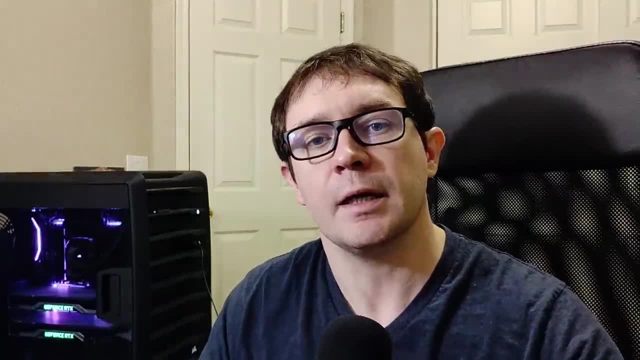 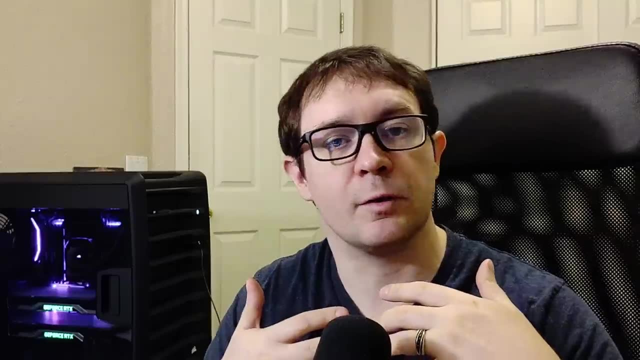 right and shoot by fixed discrete intervals, fixed amounts right In other environments like, say, robotics. the robots can move a continuous amount, So it can move in anywhere from you know, zero to one, minus one to plus one, anything along a continuous number interval. 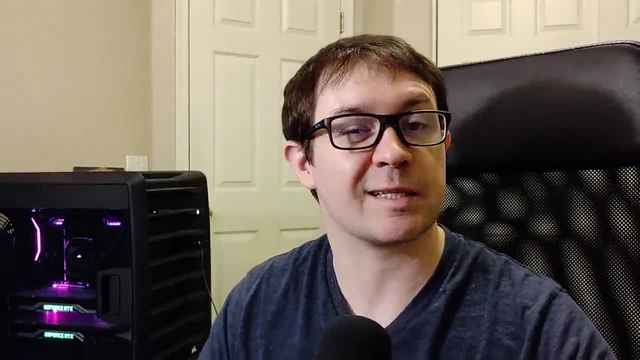 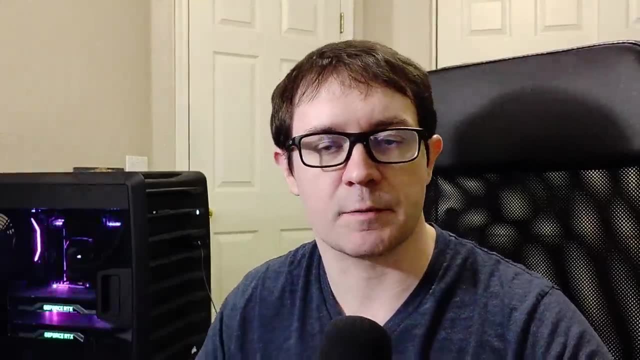 And this poses a problem for most deep reinforcement learning methods, like, say, Q-learning, which works spectacularly well in discrete environments but cannot tackle continuous numbers. So it's a problem for most deep reinforcement learning methods. continuous action spaces: Now, if you don't know what any of this means, don't worry. 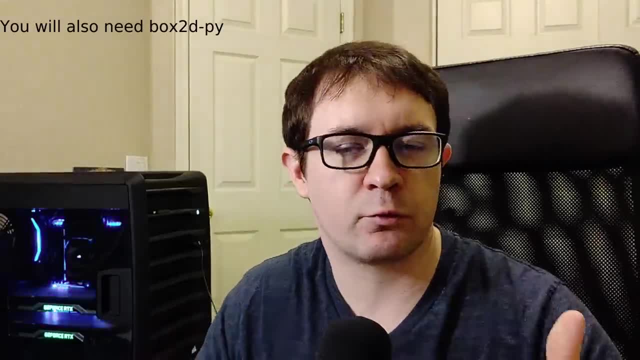 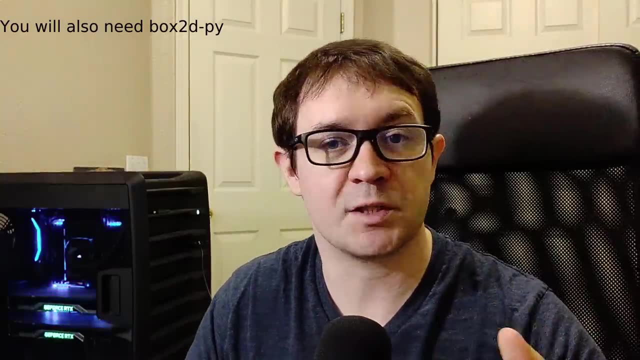 I'm going to give you the rundown here in a second, But for this set of tutorials you're going to need to have installed the OpenAI GIM. you'll need Python 3.6, and you also need TensorFlow and PyTorch. Other packages you'll need include: 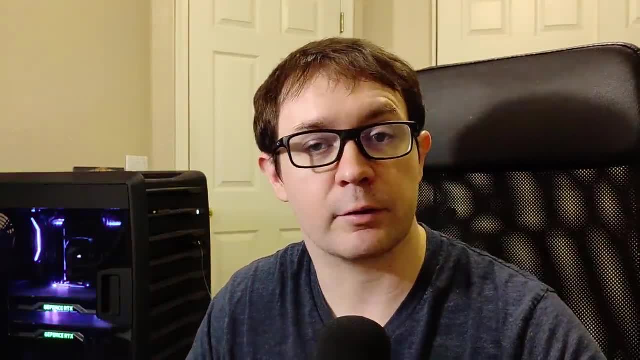 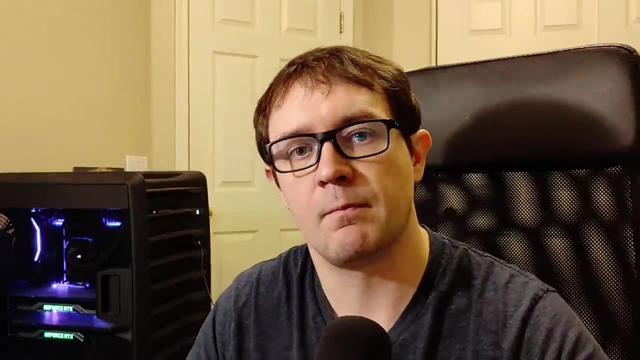 Matplotlib to handle the plotting of the learning curve, which will allow us to see the actual learning of the agent, as well as NumPy to handle your typical vector operations. Now here I'll give you a quick little rundown of reinforcement learning. So the basic idea is: 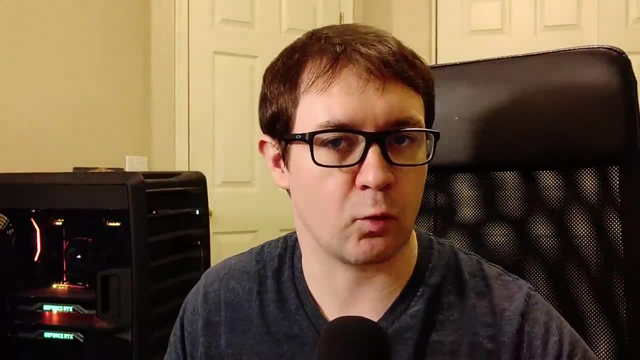 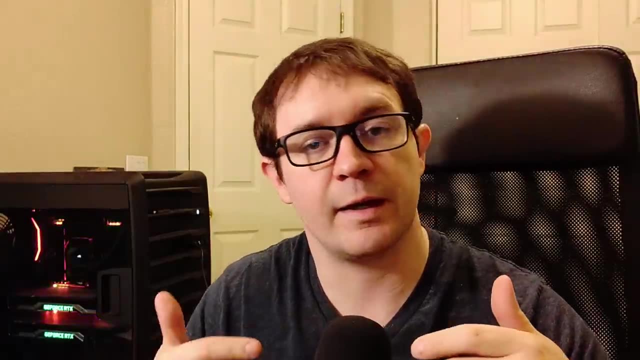 that we have an agent that interacts with some environment and receives a reward. The rewards kind of take the place of labels in supervised learning, in that they tell the agent what is good, what is it that it is shooting for in the environment, And so the agent will attempt to. 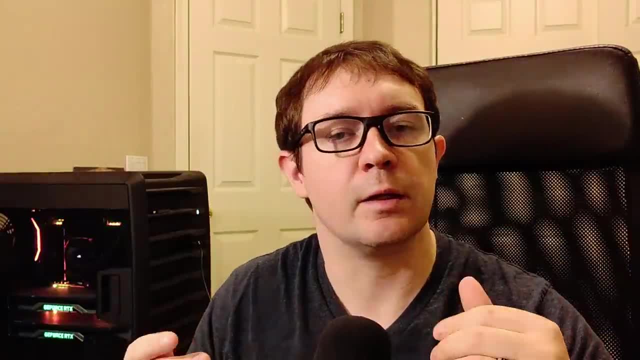 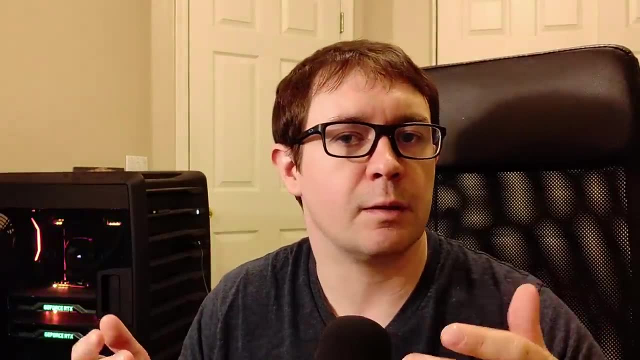 maximize the total rewards over time by solving something known as the Bellman equation. We don't have to worry about the actual mathematics of it, but just so you know for your future research. the algorithms are typically concerned with solving the Bellman equation. 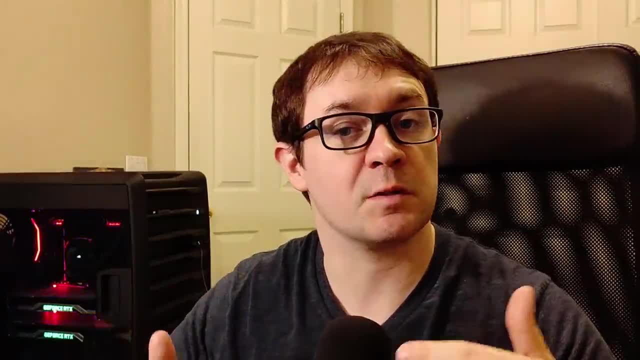 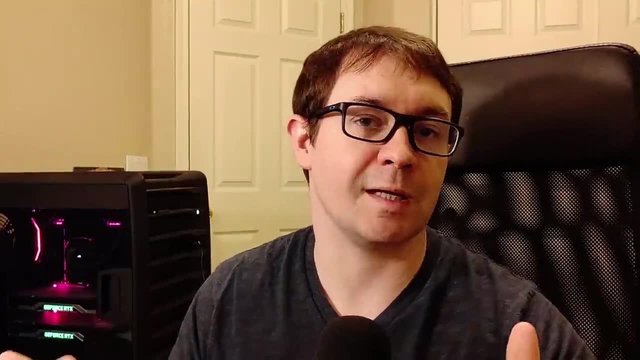 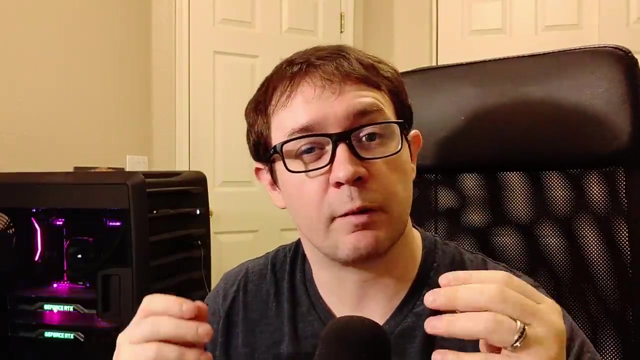 which tells the agent the expected future returns, assuming it follows something called its policy. So the policy is the probability that the agent will take a set of actions, given it's in some state. S, It's basically probability distribution. Now, many types of algorithms, such as Q-learning, will attempt to solve the 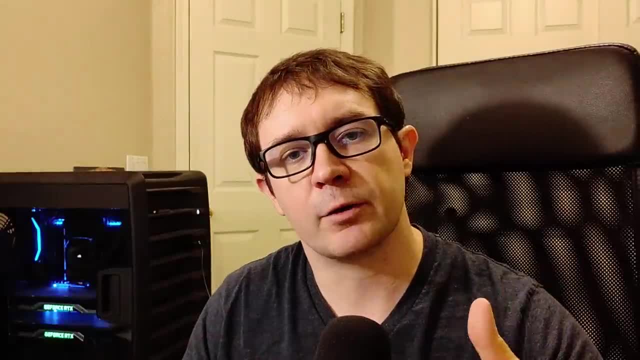 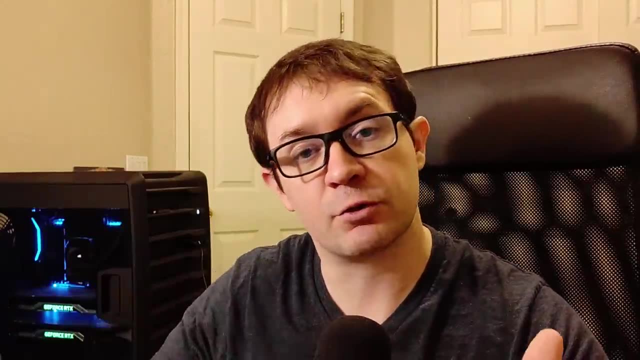 Bellman equation by finding what's called the value function. The value function, or the action value function in this case, maps the current state and set of possible actions to the expected future returns the agent expects to receive. So in other words, the agent says, hey, I'm in some state, meaning some configuration of pixels. 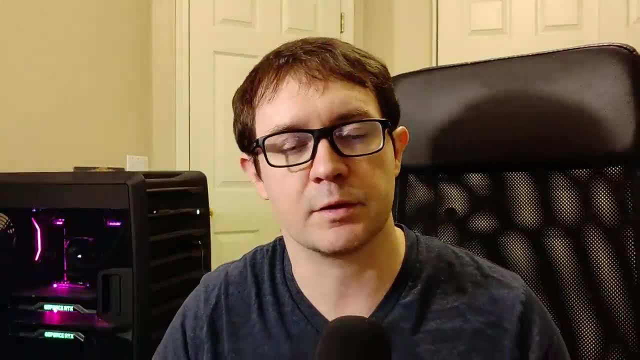 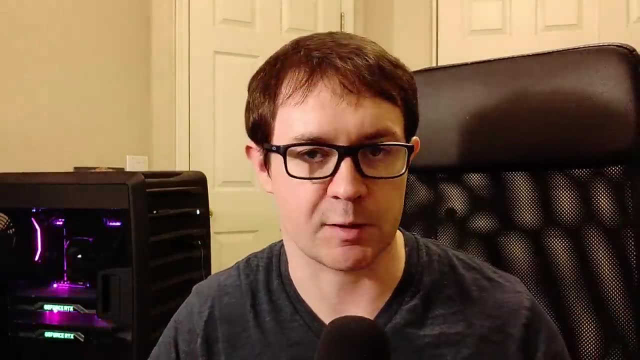 on the screen- in the case of the Atari library, for instance- and says: okay, if I take one or another action, what is the expected future return, assuming that I follow my policy? Actor-critic methods are slightly different in that they attempt to learn the policy directly. 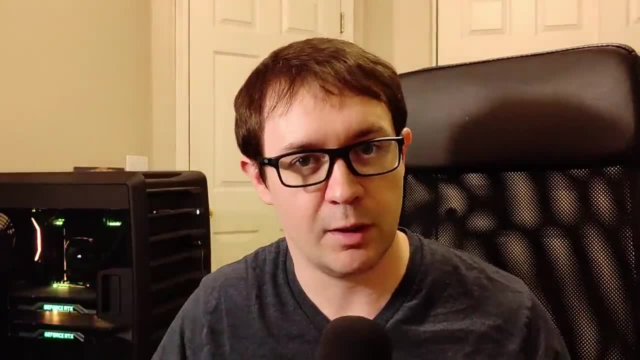 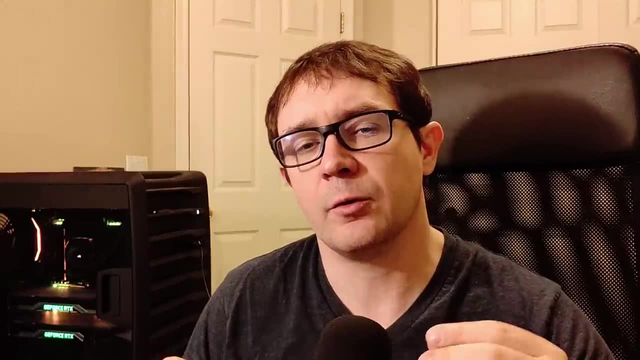 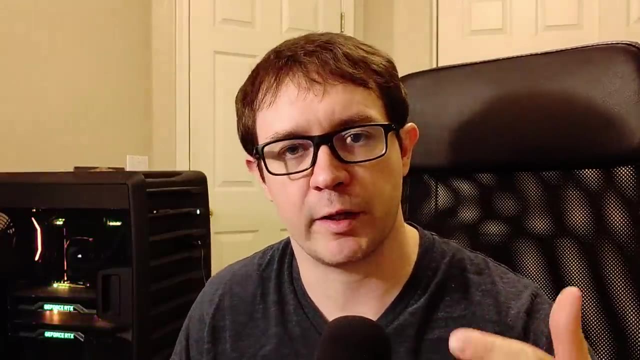 And recall the policy is a probability distribution that tells the agent what the probability of selecting an action is, given it's in some state S. So these two algorithms have a number of strengths between them, and deep deterministic policy gradients is a way to marry the strengths of these two algorithms into something that does. 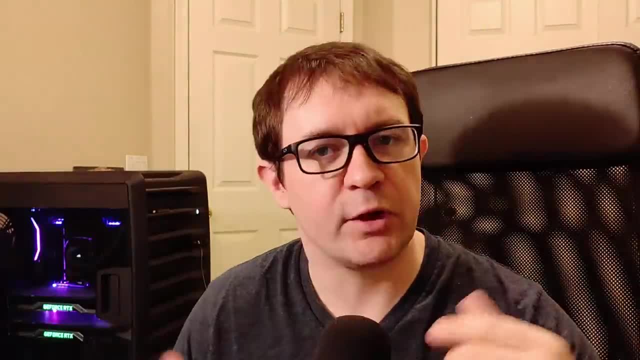 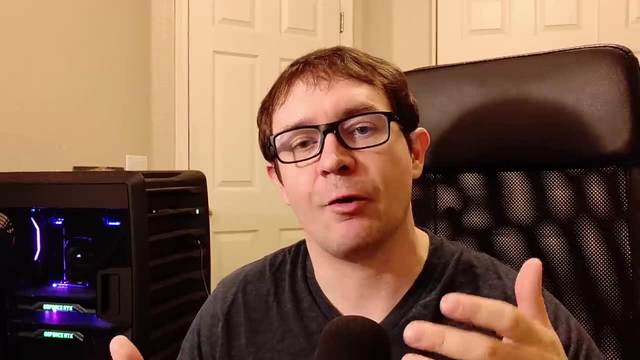 really well for discrete action- sorry, continuous action spaces. You don't need to know too much more than that. Everything else you need to know I'll explain in the respective videos. So in the first video you're going to get to see how I go ahead and read papers, and then 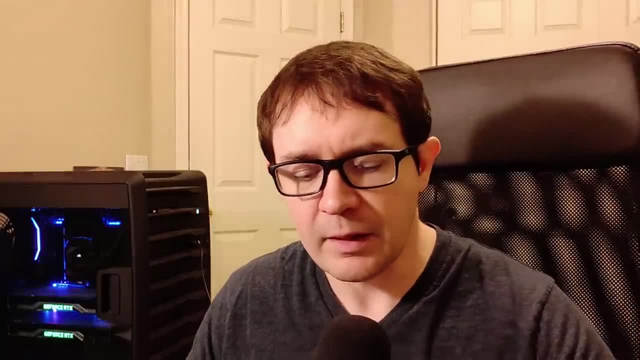 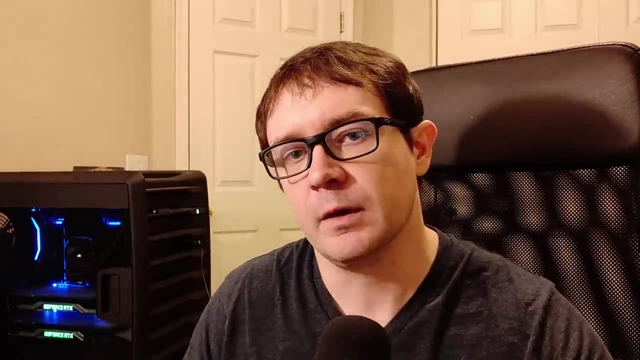 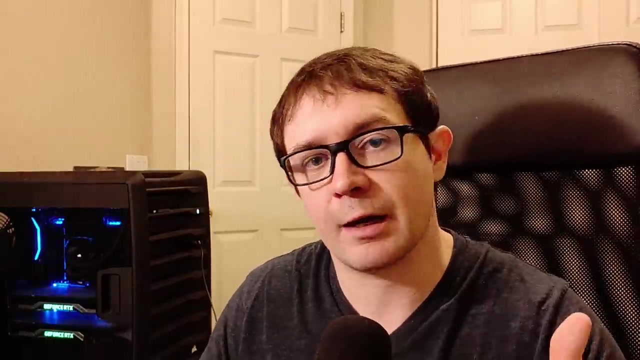 implement them on the fly, And in the second video you're going to see the implementation of deep deterministic policy gradients in PyTorch, in a separate environment. Both these environments are in. both these environments are continuous, and so they will demonstrate the power of the 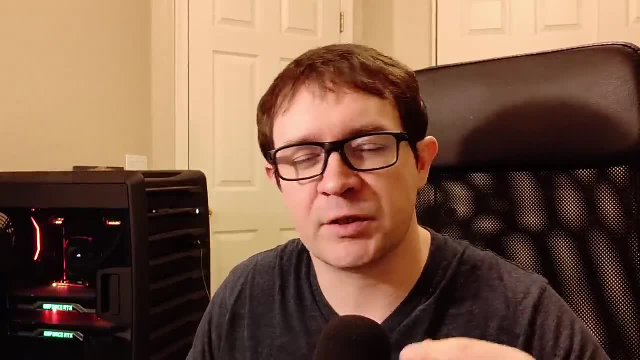 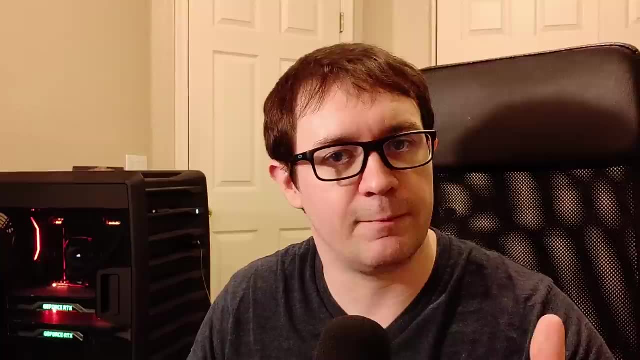 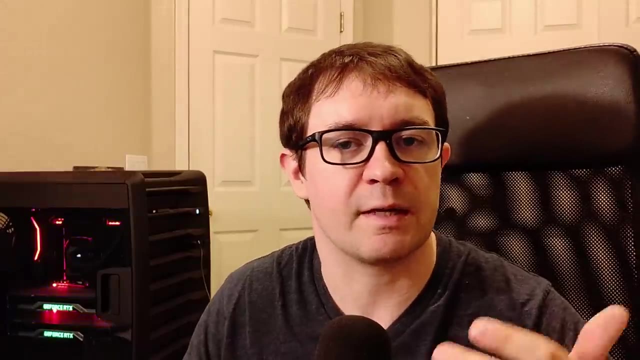 algorithm quite nicely. You don't need a particularly powerful GPU, but you do need some kind of GPU to run these, as it does take a considerably long time even on a GPU, So you will need at least a like, say, a Maxwell class GPU or above, So something from the 700 series on. 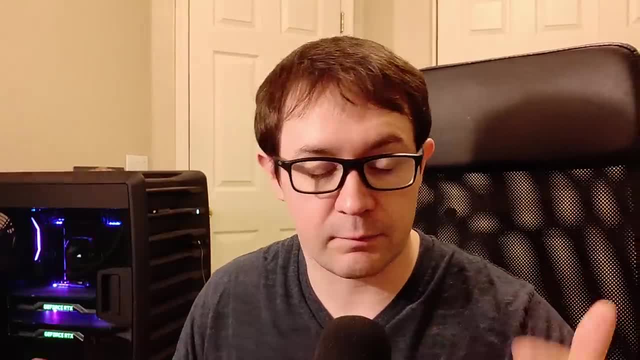 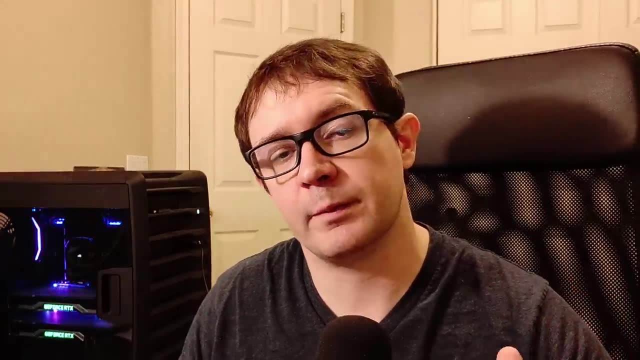 Nvidia side. Unfortunately, neither of these frameworks really work well with AMD cards, So if you have those, you would have to figure out some sort of kludge to get the OpenCL implementation to transcompile to CUDA. That's just a technical detail. I don't have any information on that. 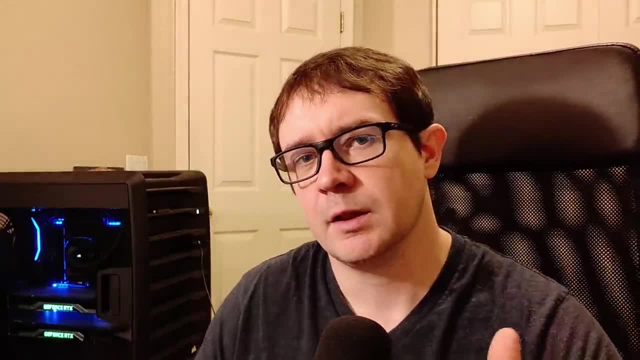 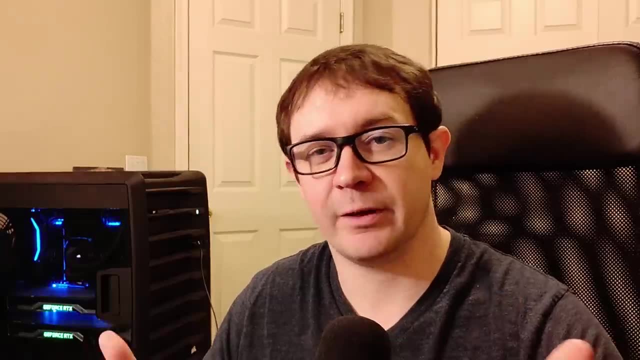 so you're on your own, sorry. So this is a few hours of content. Grab a snack, a drink and watch it. It's best to watch it in order. I actually did the videos in a separate order. a reverse order on. 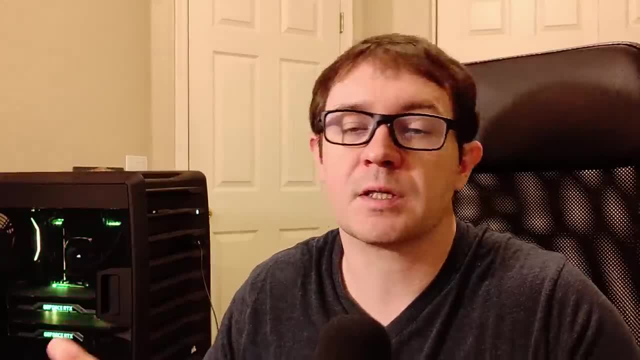 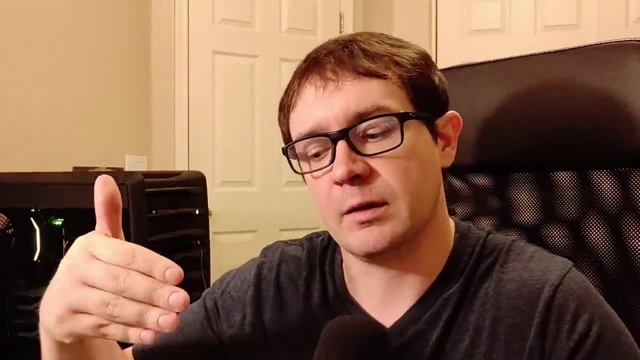 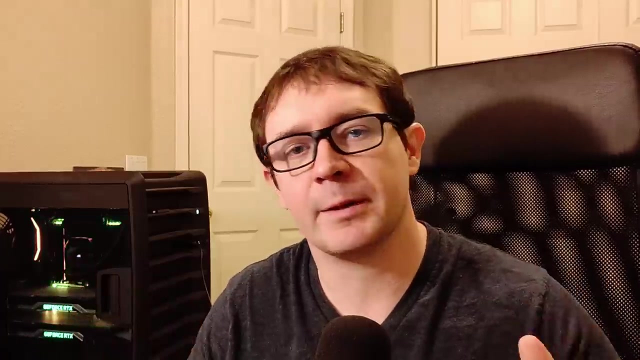 my channel just so I could get it out. So I did the implementation of PyTorch first and then the video on implementing the paper in TensorFlow second. But it really is best for a new audience to go from the paper video to the PyTorch video. So I hope you like it. Leave any comments. 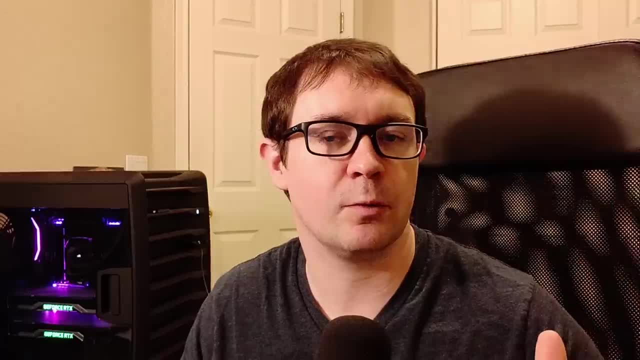 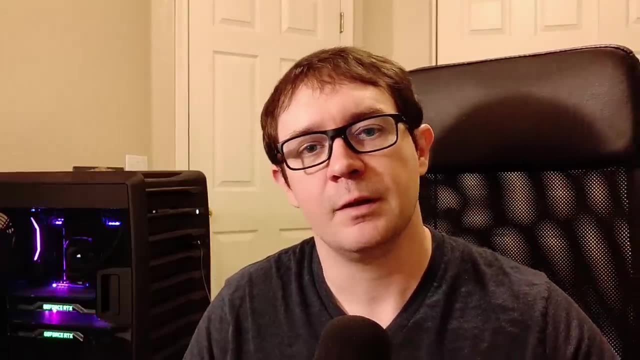 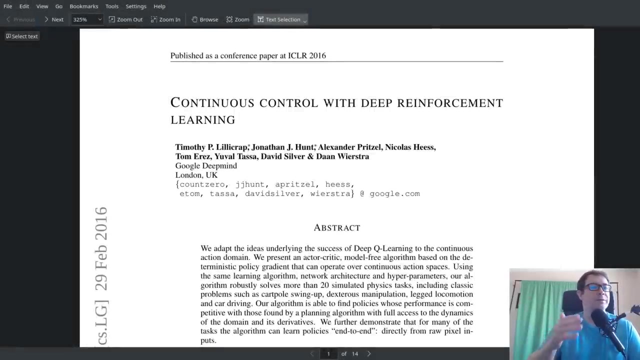 questions, suggestions, issues down below. I'll try to address as many as possible. You can check out the code for this on my GitHub And I'll see you guys in the next video. Have a great day. Bye-bye, What is up, everybody? In today's video we're going to go from the paper on deep deterministic 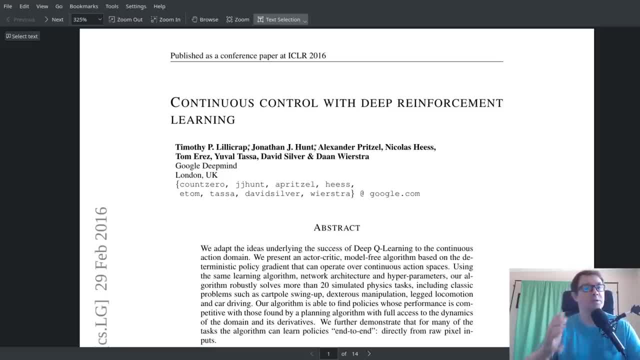 policy gradients all the way into a functional implementation in TensorFlow. So you're going to see how to go from a paper to a real-world implementation all in one video. Grab a snack, a drink, because this is going to take a while. Let's get started. 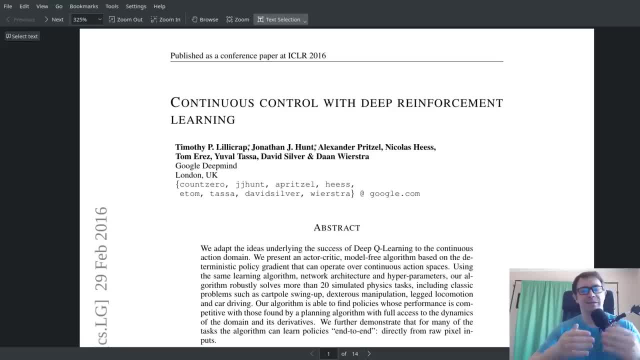 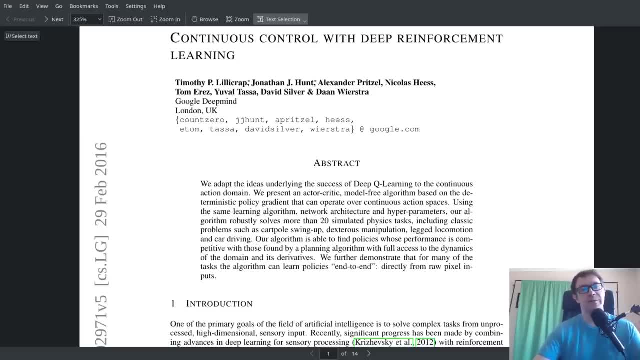 So the first step in my process really isn't anything special. I just read the entirety of the paper, Of course, starting with the abstract. The abstract tells you what the paper is about at a high level. It's just kind of an executive summary. Introduction is where the authors will. 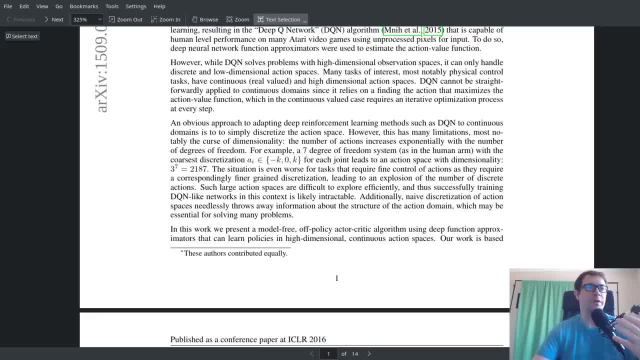 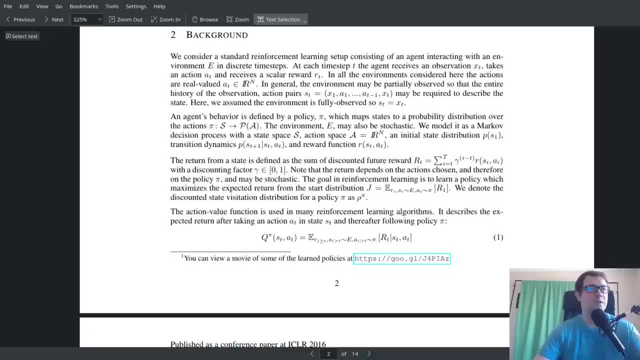 pay homage to other work in the field, kind of set the stage for what is going to be presented in the paper as well as the need for it. The background kind of expands on that And you can see here it gives us a little bit of mathematical equations. 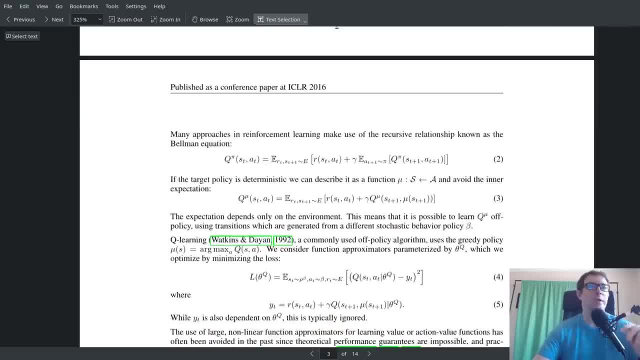 And you will get a lot of useful information here. This won't talk too much about useful nuggets on implementation, but it does set the stage for the mathematics you're going to be implementing, which is, of course, critical for any deep learning, or, in this case, 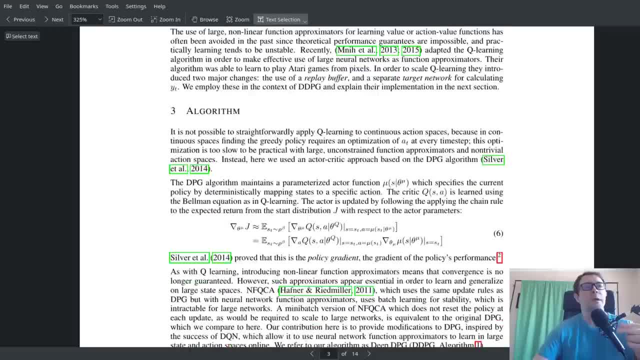 deep reinforcement learning paper. implementation- The algorithm is really where all the meat of the problem is. It is in here that they lay out the exact steps you need to take to implement the algorithm right. That's why it's titled that way. So this is the section we want to talk about. 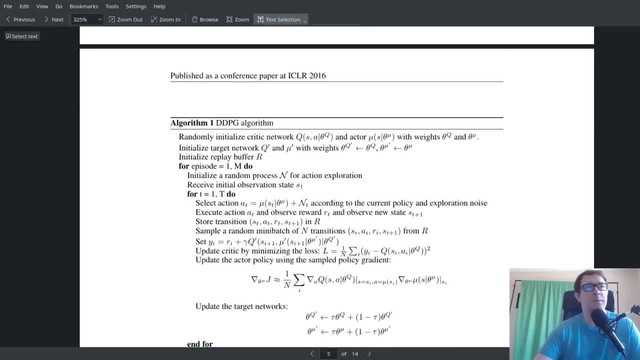 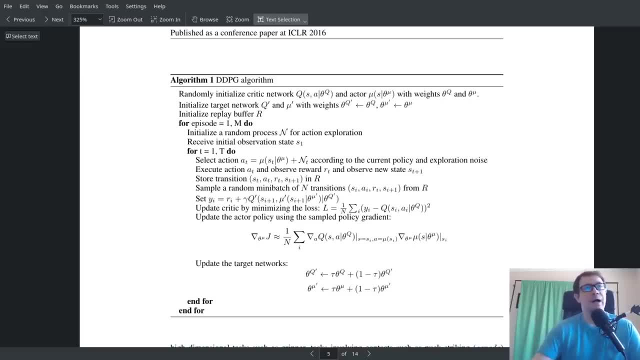 And then, of course, they will typically give a table where they outline the actual algorithm. And oftentimes, if I'm in a hurry, I will just jump to this, because I've done this enough times that I can read this- what is called pseudocode. If you're not familiar with that, pseudocode is: 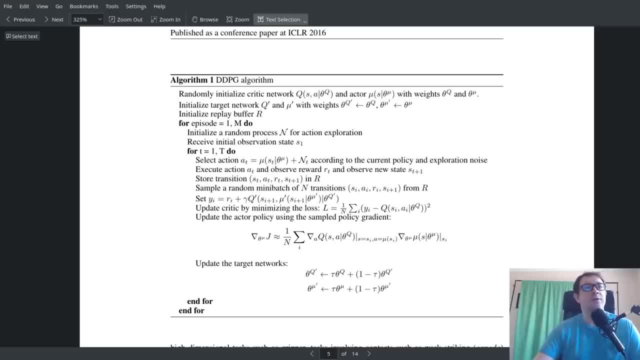 just an English representation of computer code, So we will typically use that when we outline a problem, And it's often used in papers, of course. So typically I'll start here reading it and then work backward by reading through the paper to see what I missed. But 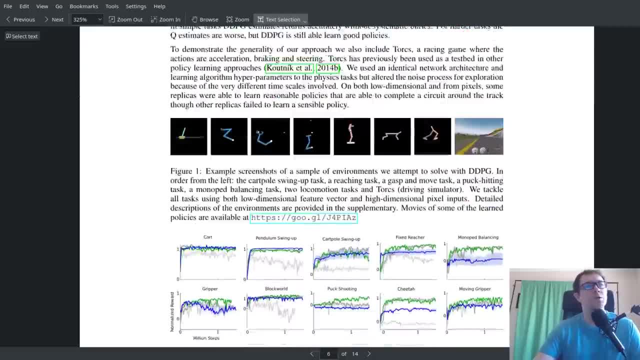 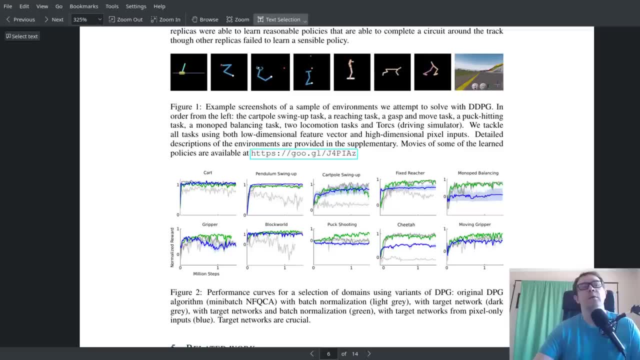 of course it talks about the performance across a whole host of environments, And of course all of these have in common that they are continuous control. So what that means is that the action space is a vector whose elements can vary on a continuous real number line. 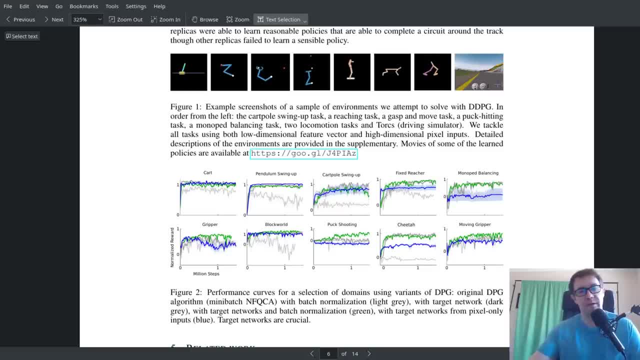 instead of having discrete actions of 0,, 1,, 2,, 3,, 4, or 5.. So that is the motivation behind deep deterministic policy gradients that allows us to use deep reinforcement learning to tackle these types of problems. And in today's video we're going to go ahead and 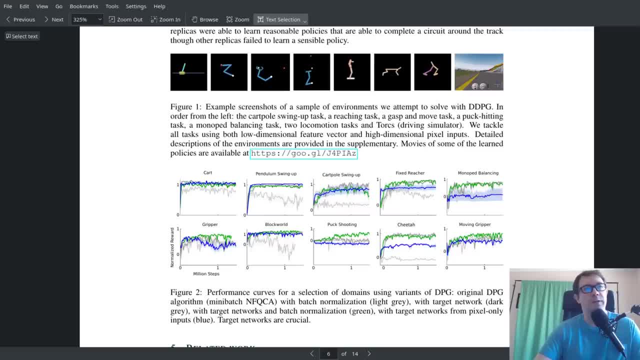 tackle the- I guess- pendulum swing up, also called the pendulum problem. Reason being is that, while it would be awesome to start out with something like the bipedal walker, you never want to start out with maximum complexity. You always want to start out with something very. 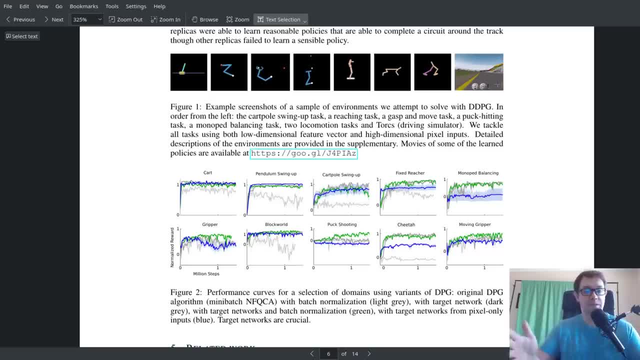 very small and then scale your way up, And the reason is that you're going to make mistakes And it's most easy to debug quick, to debug very simple environments that execute very quickly. So the pendulum problem only has, I think, three elements in its state vector and only a single action. So, or maybe, 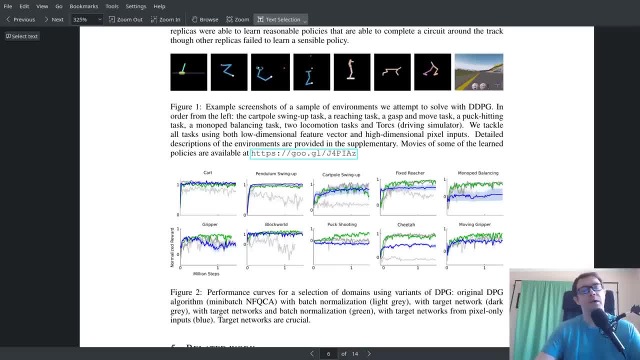 it's two actions, I forget, But either way it's a very small problem relative to something like the bipedal walker or many of the other environments. You could also use the continuous version of the card poll or something like that. That would be perfectly fine. I've just chosen the. 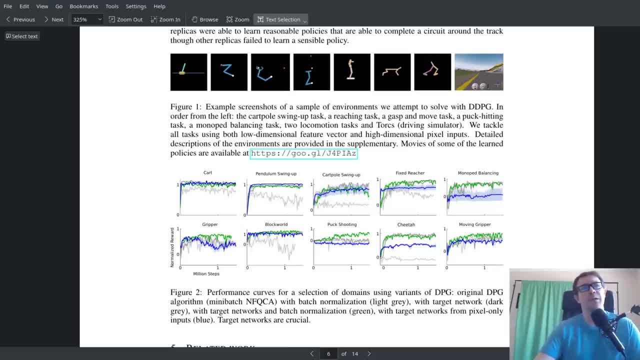 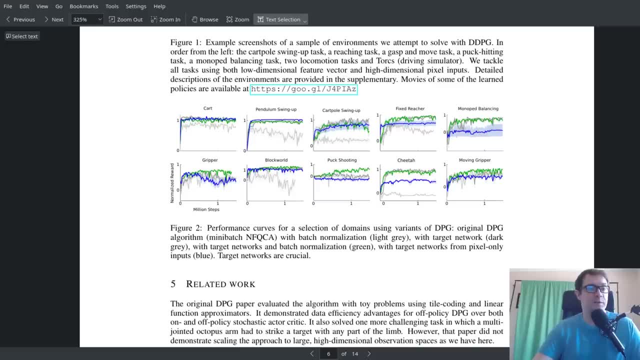 pendulum for this particular video, because we haven't done it before, So it's in here that they give a bunch of plots of all of the elements. So I'm going to go ahead and start out with all of the performance of their algorithm, with various sets of constraints placed upon it, and 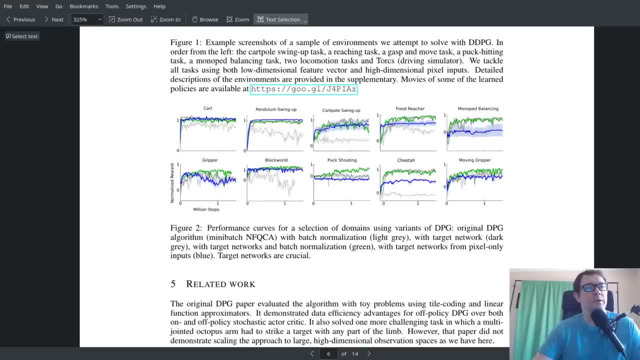 different implementations so you can get an idea. And one thing you notice right away: it's always important to look at plots because they give you a lot of information visually, right. It's much easier to gather information from plots than it is text. You see that right. 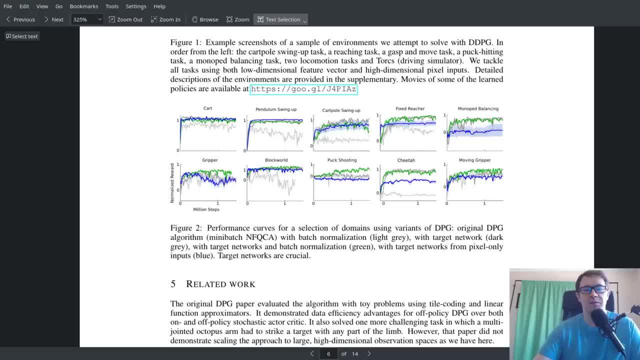 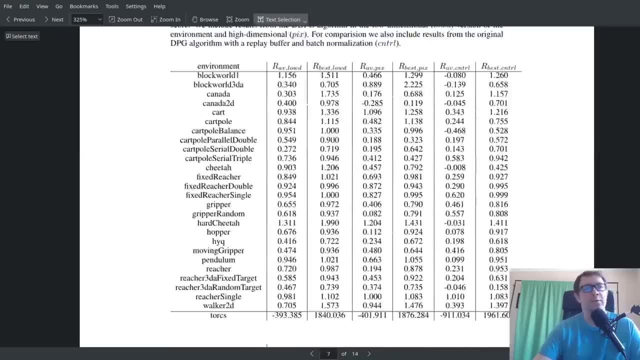 away. they have a scale of one, So that's telling you it's relative performance and you have to read the paper to know relative to what. I don't like that particular approach. They have similar data. I don't like that particular approach. They have similar data. 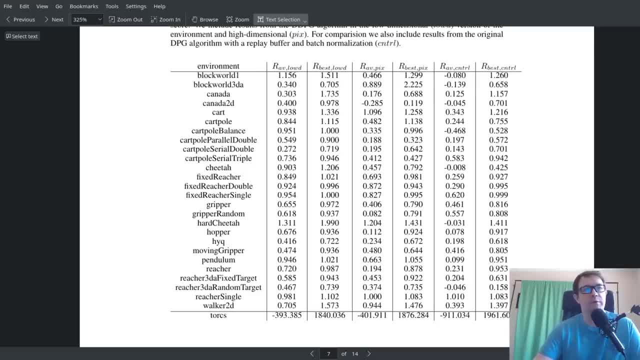 that are right here. This is a table form and here you see a whole bunch of environments they used and there's a broad, broad variety. They wanted to show that the algorithm has a wide arena of applicability, which is a typical technique In papers. they want to show that this is relevant. 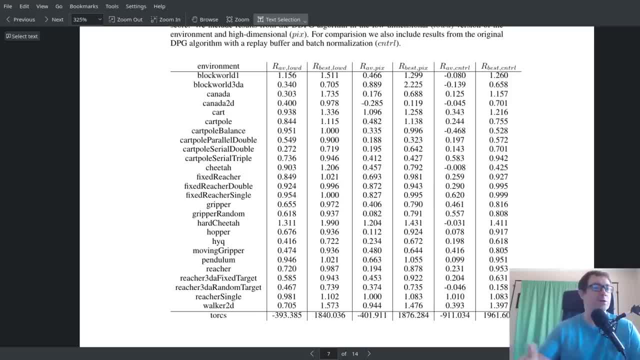 right. If they only showed a single environment, people reading it would say: well, that's all, well and good, You can solve one environment, but what about these dozen other environments? right, And learning is generality. Can we model real learning in biological systems such that it? 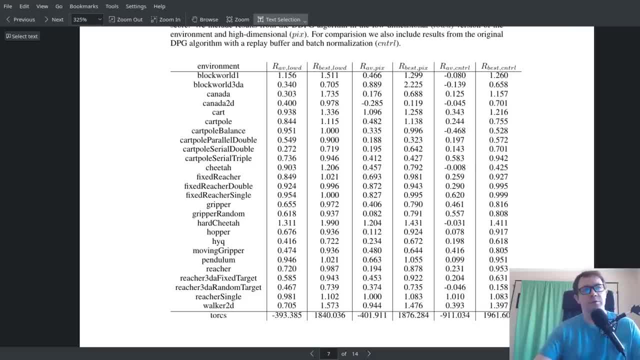 mimics the generality of biological learning. One thing you notice right away is that these numbers are not actual scores, So that's one thing I kind of take note of and causes me to raise an eyebrow. So you have to wonder the motivation behind that. Why would the authors 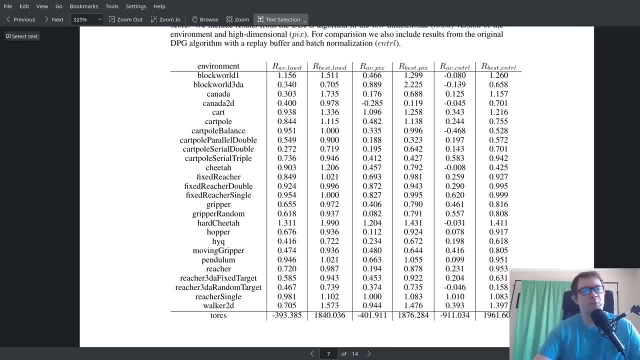 express scores in a ratio. There's a couple different reasons. One is because they want to just to make all the numbers look uniform. Maybe the people reading the paper wouldn't be familiar with each of these environments, so they don't know what a good score is And that's a perfectly. 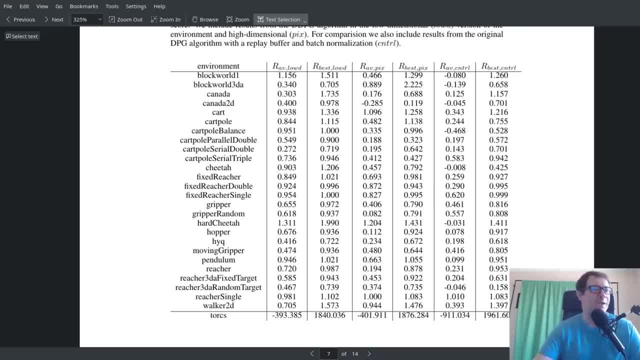 valid reason. Another possibility is they want to hide poor performance. I don't think that's going on here, but it does make me raise my eyebrow whenever I see it. One exception is the torques, which is a totally open race car simulator environment. I don't know if we'll get to that. on. 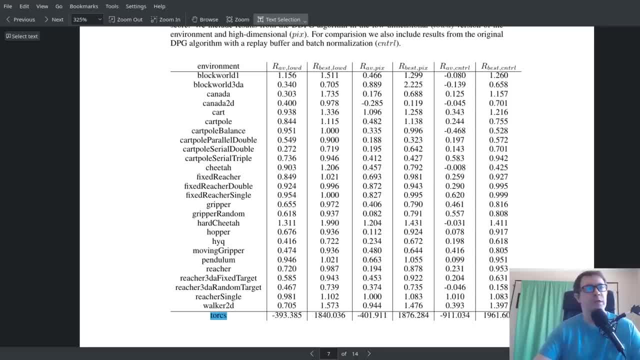 this channel. That would be a pretty cool project but that would take me a few weeks to get through. But right away you notice that they have a whole bunch of environments. These scores are all relative to one, and one is the score that the agent gets on a planning algorithm, which they 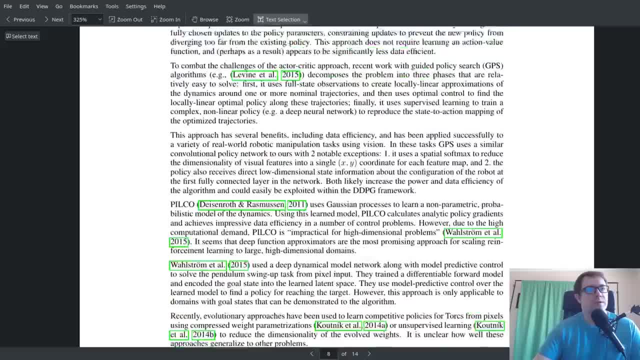 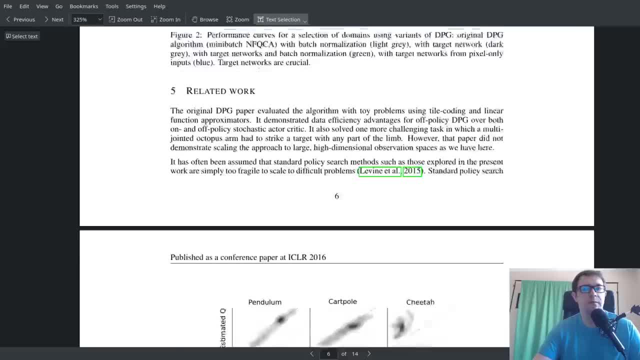 also detail later on. So those are the results and they talk more about. I don't think we saw the headline, but they talk about related work, which talks about other algorithms that are similar and their shortcomings. right, They don't ever want to talk up other algorithms. You always want to. 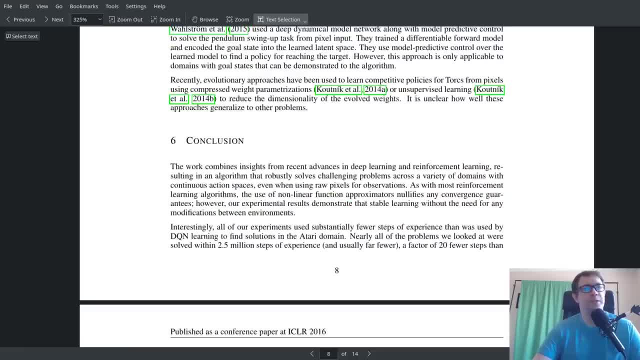 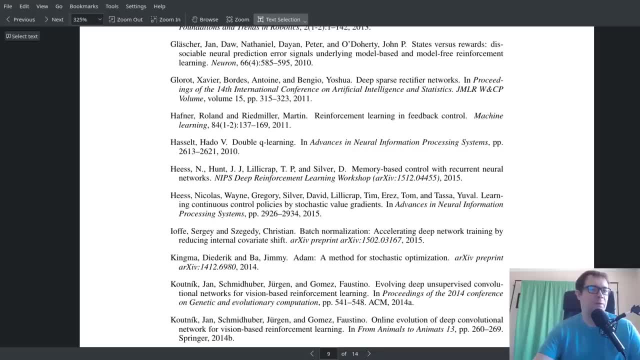 talk up your own algorithm to make yourself sound good. Um, you know, why else would you be writing a paper in the first place? And, of course, the conclusion, to tie everything together: References. I don't usually go deep into references. Um, if there is something that I feel I really, really need to know, I may look at a 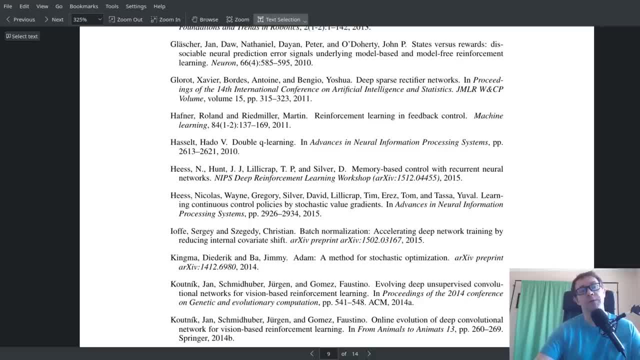 reference, but I don't typically bother with them. Uh, if you were a PhD student, then it would be who you to go into the references, because you must be an absolute expert on the topic. And for us we're just, you know, hobbyists. I'm a YouTuber, so I don't go into too much depth with the 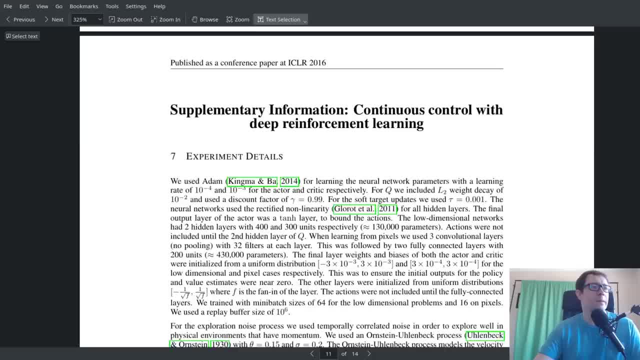 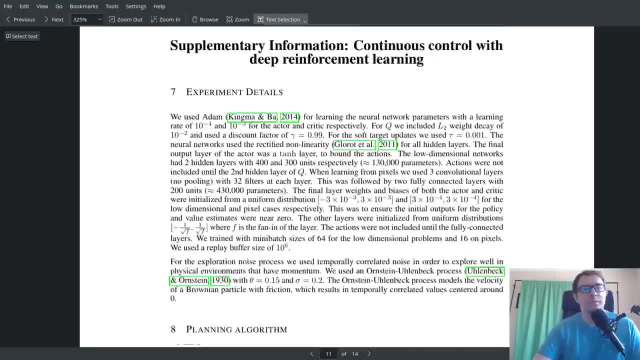 background information. I'm just going to go into the background information. I'm going to go into the background information And the next most important bit of the paper are the experimental details, And it is in here that it gives us the parameters and architectures for the networks. So 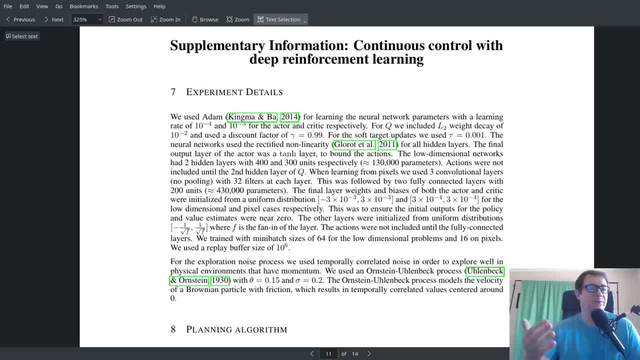 this is where, if you saw my previous video where I did the implementation of DDPG and PyTorch and the continuous lunar lander environment, this is where I got most of this stuff. It was almost identical with a little bit of tweaking. I left out some stuff from this paper, but uh pretty. 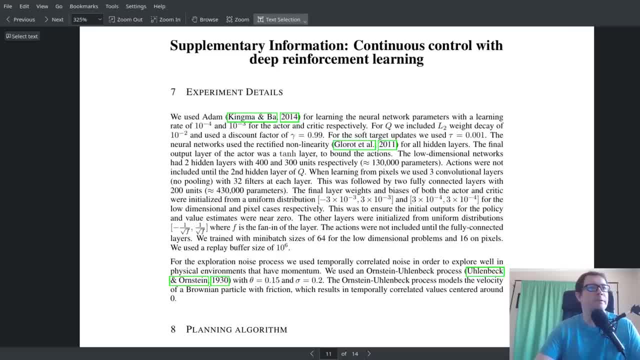 much all of it came from here, In particular, the hidden layer sizes, 400 and 300 units, uh, as well as the initialization of the parameters from uniform distribution of the given ranges, Uh. so just to recap, uh, this was a really. 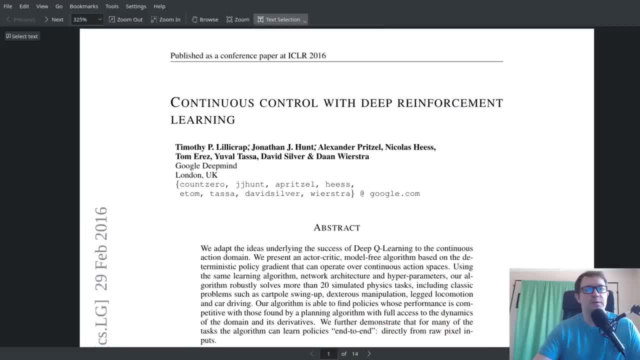 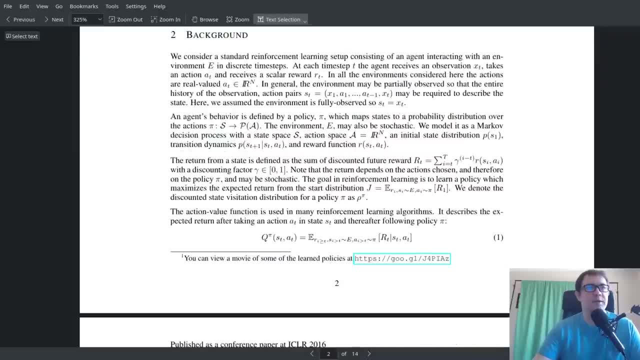 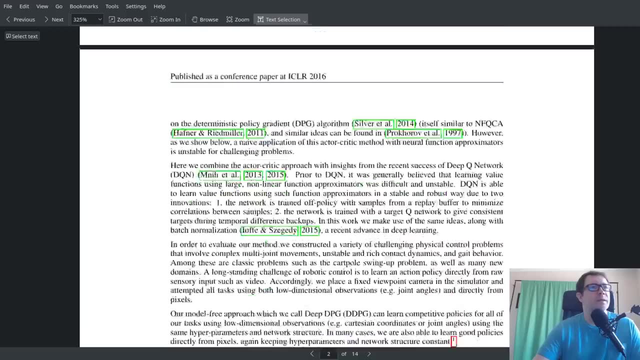 quick overview of the paper. uh, just showing my process of what I look at. Uh, the uh most important parts are the details of the algorithm as well as the experimental details. So as you read the paper, um, like I said, I gloss over the introduction because I don't really 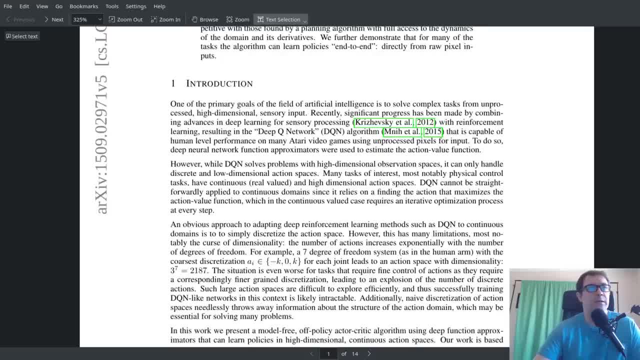 I kind of already understand the motivation behind it. I get the idea It says, basically tells us that, um, you can't really handle, uh, continuous action spaces with deep Q networks- Uh, we already know that. And it says: you know you can discretize the state space, but then you end up. 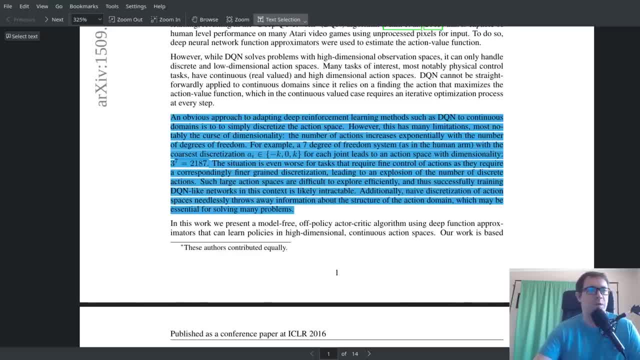 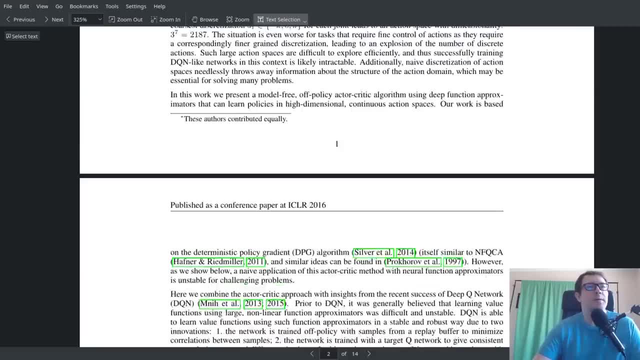 with really, really huge actions. Sorry, You can discretize the action space, but then you end up with a whole boatload of actions. you know what is it? 2,187 actions. So it's intractable anyway, And they say what we present, you know. 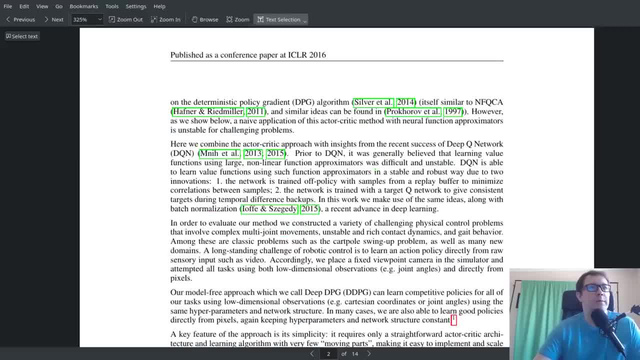 a model free off policy algorithm. And uh, then it comes down to this section where it says the network is trained off policy with samples from a replay buffer to minimize correlations- Very good- And train with the target Q network to give consistent targets during temporal difference. 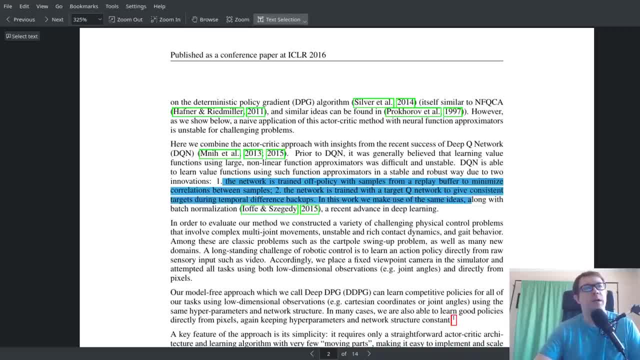 backups. So in this work, we make use of the same ideas, along with batch normalization. So let's talk about the used data, of the data, And I'm going to go ahead and take a second to read this. Yeah, So what we're going to do is we're going to show you М. 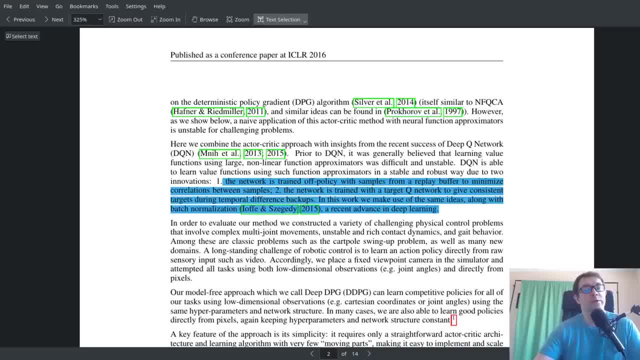 we're going to show you the data of the data that we've on the screen, So you can always have the data as well, even if it's in a text, and this is why you want to read the whole paper, because sometimes they'll embed stuff in there that you may not otherwise catch. So, uh, as I'm 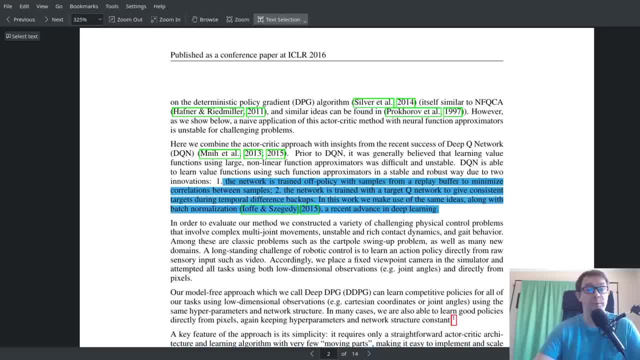 reading the paper. what I do is I take notes, and you can do this in paper, you can do it in you know text document. In this case, we're going to use the editor, so that way I can show you what's. 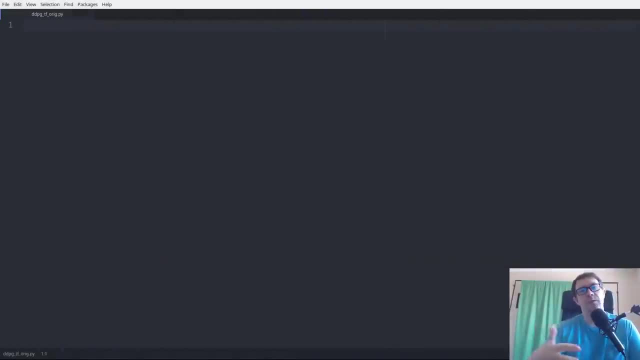 going on, And it's a natural place to put this stuff, Cause that's where we're going to implement the code. Anyway, let's hop over to the editor. Yeah them. So the paper mentioned a replay buffer as well as a target queue network. So the target queue. 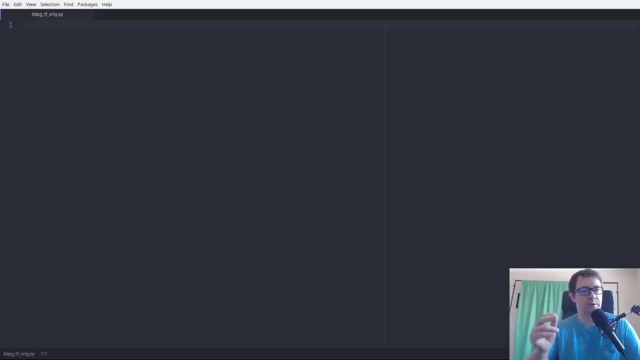 network. for now we don't really know what it's going to be, but we can write it down. So we'll say we'll need a replay buffer class and need a class for a target queue network. Now I would assume that if you're going to be implementing a paper of this advanced difficulty, you'd already 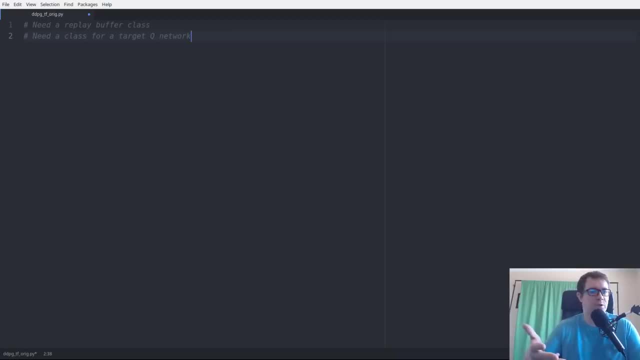 be familiar with queue learning, where you know that the target network is just another instance of a generalized network. The difference between the target and evaluation networks are: you know the way in which you update their weights. So right off the bat, we know that we're going to. 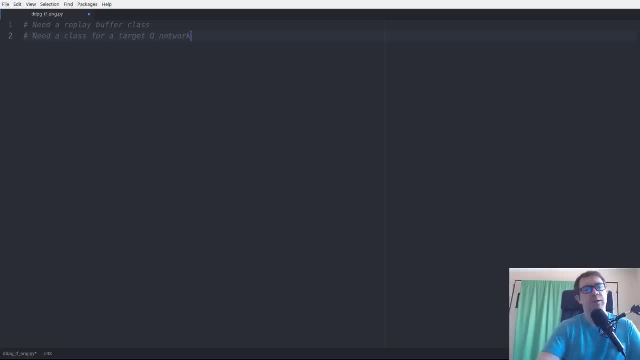 have a single class, at least one. If you know something about actor-critic methods, you'll know that you'll probably have two different classes, one for an actor, one for a critic, because those two architectures are generally a little bit different. 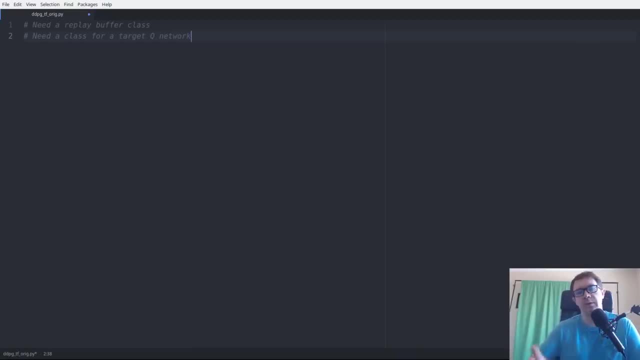 But what do we know about queue networks? We know that queue networks are state action value functions. right, They're not just value functions. So the critic in the actor-critic methods is just a state value function in general, Whereas here we have a queue network which is going to be a 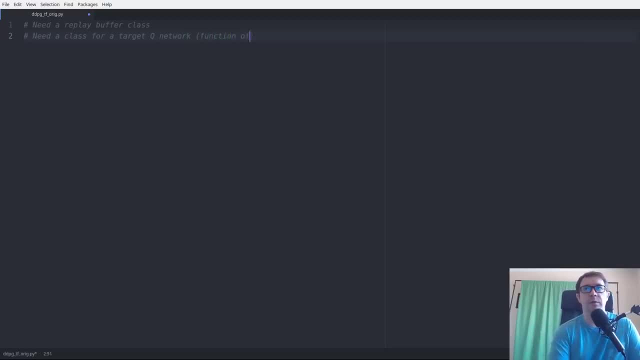 function of the state and action. So we know that it's a function of s and a. So we know right off the bat it's not the same as a critic, It's a little bit different. And it also said: we will. 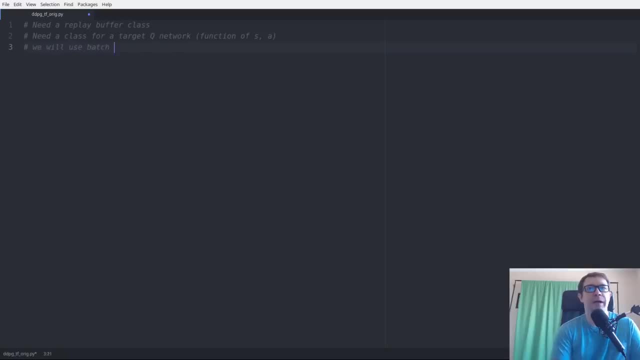 use. we will use batch norm. So batch normalization is just a way of normalizing inputs to prevent divergence in a model. I think it was discovered in 2015,, 2014, something like that. So then we use that, So we'll need that in our network, So we know at least right off the bat a little bit of an. 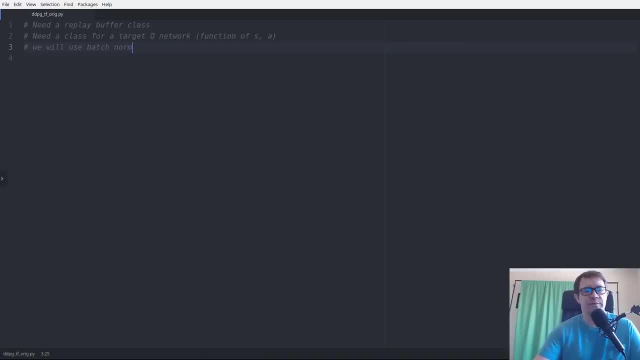 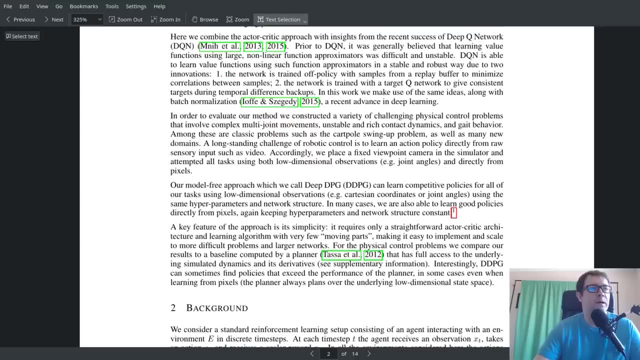 idea of what the network is going to look like. So let's go back to the paper and see what other little bits of information we can glean from the text before we take a look at the algorithm Reading along, we can say blah, blah. they say. key feature: simplicity. it requires only a straightforward actor-critic. 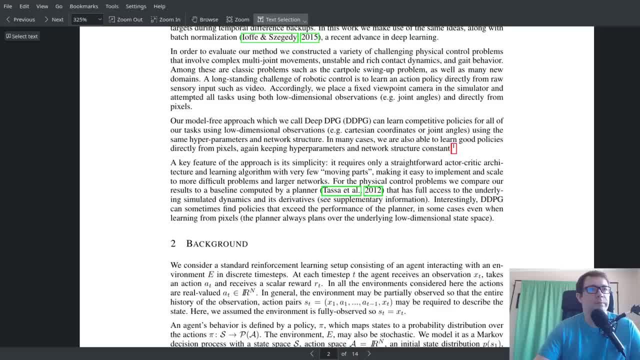 architecture and very few moving parts. And then they talk it up and say: can learn policies that exceed the performance of the planner. you know the planning algorithm, even learning from pixels, which we won't get to in this particular implementation. So then, okay, no real other. 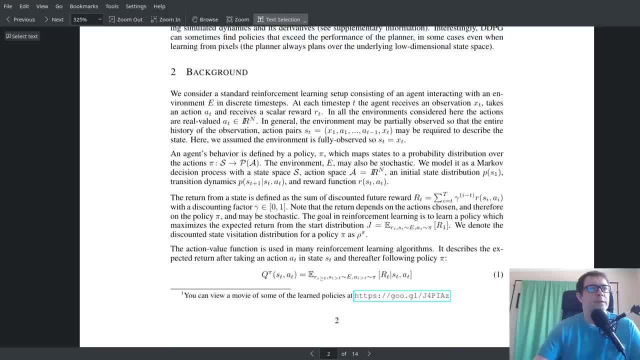 nuggets there. The background talks about the mathematical structure of the algorithm, So this is really important if you want to have a really deep, in-depth knowledge of the topic. If you already know enough about the background, you would know that you know the formula for discounted. 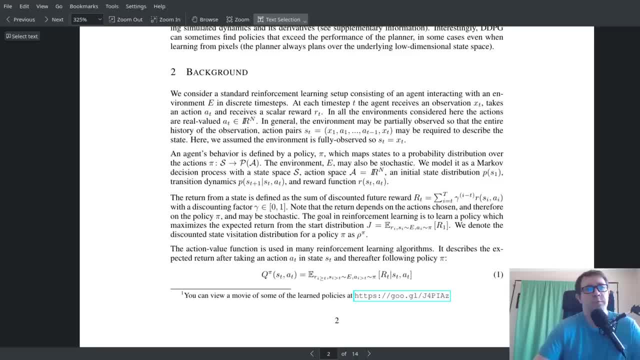 future rewards. you should know that if you've done a whole bunch of reinforcement learning algorithms. If you haven't, then definitely read through this section to get the full idea of the background and the motivation behind the mathematics. Other thing to note is it says the 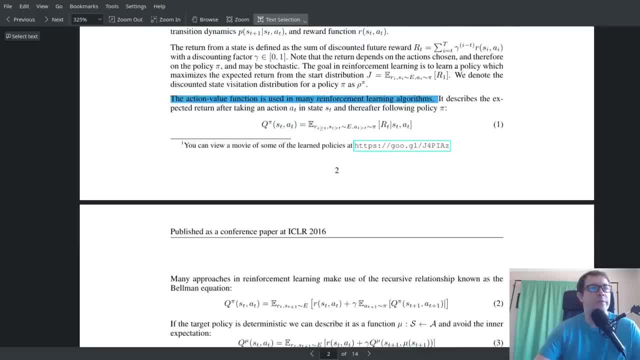 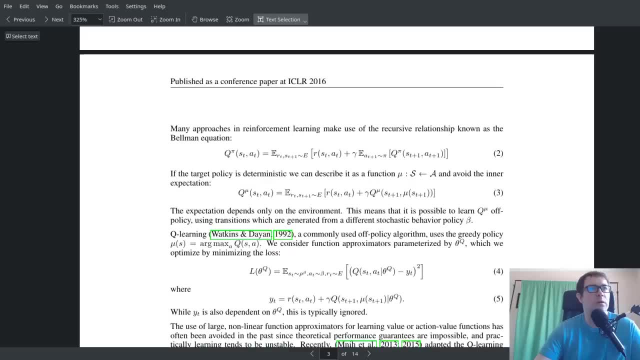 action value function is used in many algorithms. We know that from deep Q learning. And then it talks about the recursive relationship known as the Bellman equation. that is known as well. Other thing to note: what's interesting here- and this is the next nugget- is if the target policy is deterministic, we can describe it as a function. 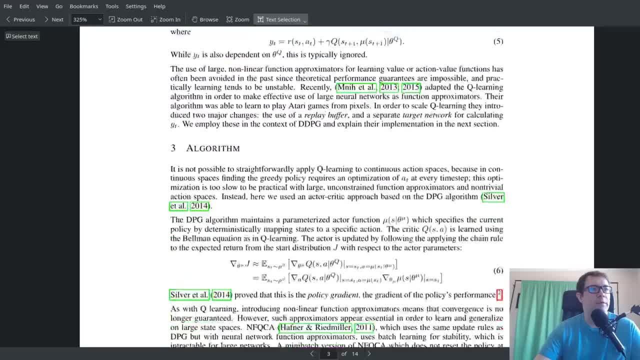 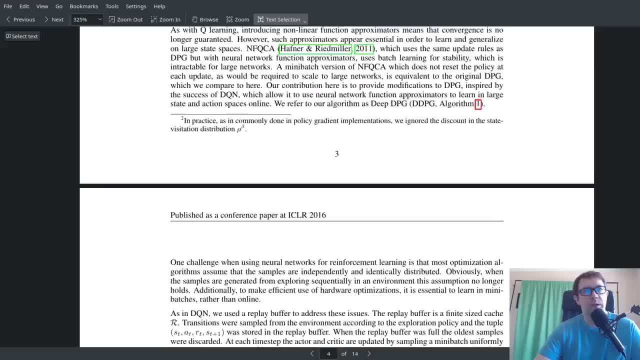 mu. And so you see that in the remainder of the paper, like in the algorithm, they do indeed make use of this parameter mu. So that tells us right off the bat that our policy is going to be deterministic. Now, if you've done a whole bunch of reinforcement learning algorithms, you're going to 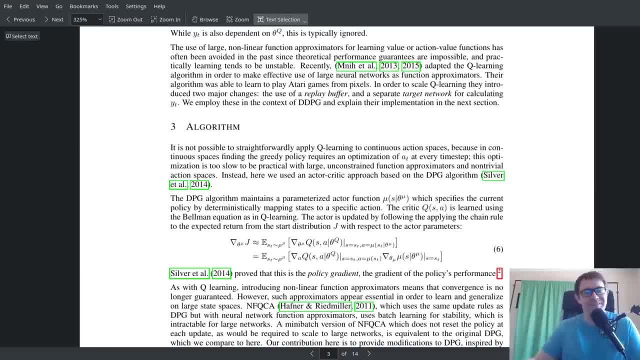 have. you could probably guess that from the title, right, Deep deterministic policy gradients, right. So you would guess from the name that the policy is deterministic. What does that mean exactly? So a stochastic policy is one in which the software maps the probability of taking an. 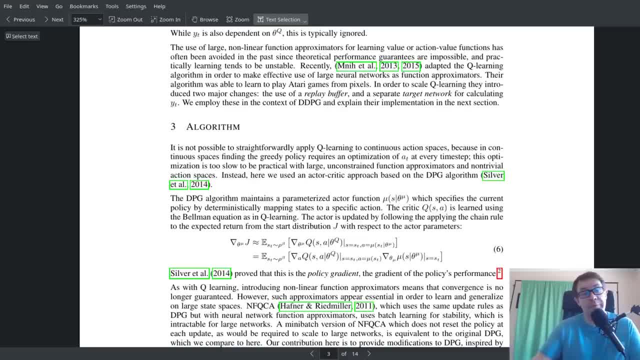 action to a given state. So you input a set of state and outcomes, a probability of selecting an action, and you select an action according to that probability distribution. So that right away bakes in a solution that's going to be deterministic. So if you've done a whole bunch of reinforcement, 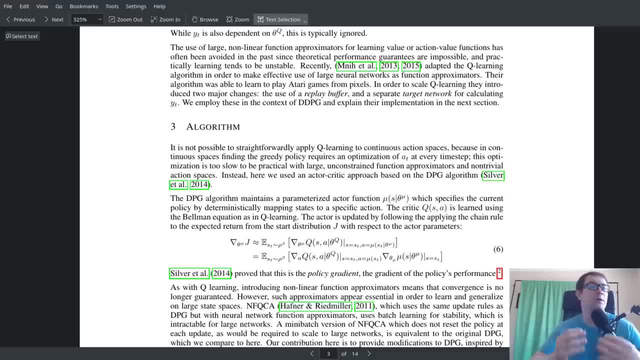 learning algorithms. you're going to have a set of state and outcomes bakes in a solution that's going to to the explore-exploit dilemma. so long as all probabilities are finite, right? So as long as a probability of taking an action for all states doesn't go to zero, there is some element of 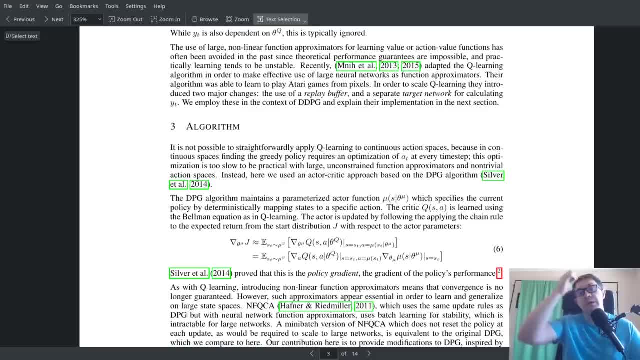 exploration involved in that algorithm. Q-learning handles the explore-exploit dilemma by using epsilon greedy action selection, where you have a random parameter that tells you how often to select a random number- sorry, a random action- and then you select a greedy action. the remainder, 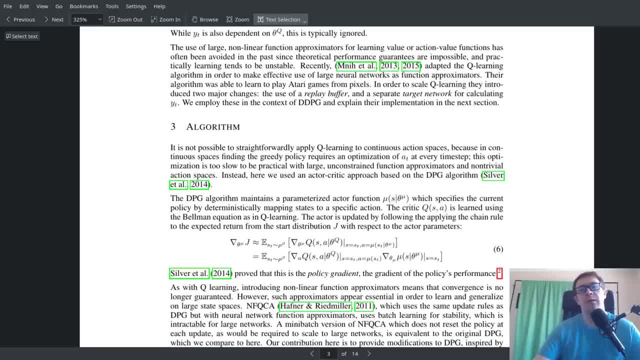 of the time. Of course, policy gradients don't work that way. So if you've done a whole bunch of work that way, they typically use a stochastic policy. but in this case we have a deterministic policy. So you have to wonder right away: okay, we have a deterministic policy, how are we going? 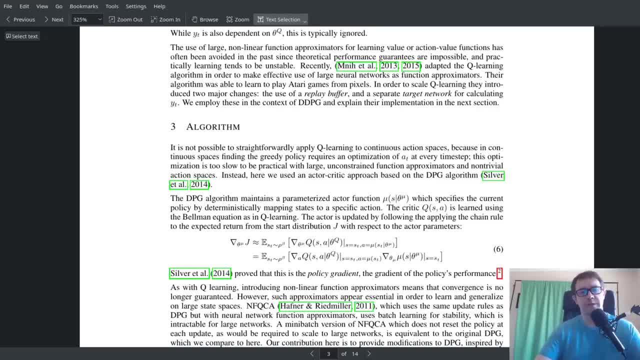 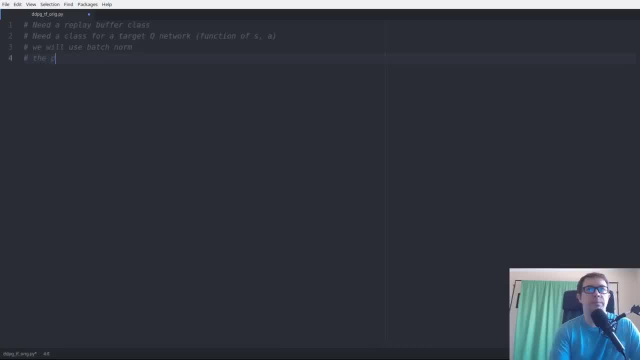 to handle the explore-exploit dilemma. So let's go back to our text editor and make a note of that. So we just want to say that the policy is deterministic: how to handle explore-exploit. And that's a critical question, right? Because if you only take 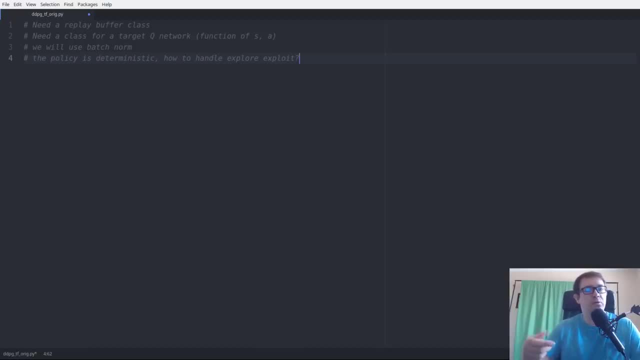 what are perceived as the greedy actions. you never get a really good coverage of the parameter space of the problem and you're going to converge on a suboptimal strategy. So this is a critical question we have to answer in the paper. So let's head back to the paper and see how they handle it. 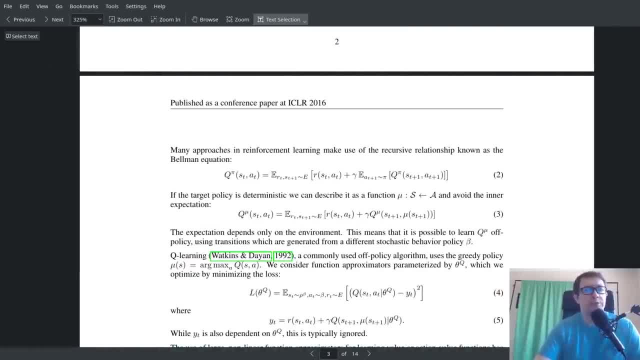 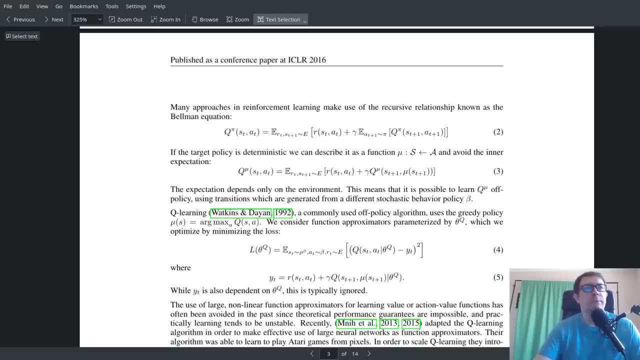 So we're back in the paper and you can see the reason they introduced that deterministic policy: is to avoid an inner expectation, or maybe that's just a byproduct. I guess it's not accurate to say that's the reason they do it. But what's neat is it says the expectation depends only on the. 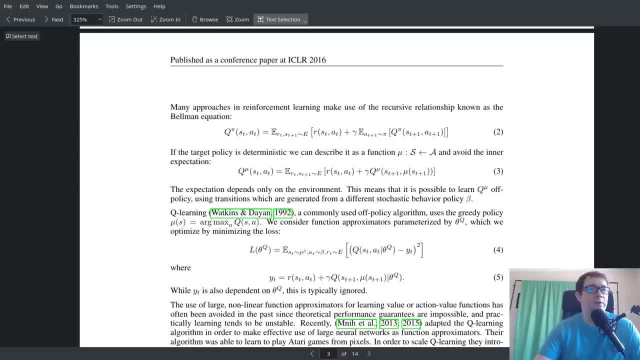 environment. It means it's possible to learn and it's possible to avoid and it's possible to learn Q to the mu meaning. Q is a function of mu off policy using transitions which are generated from a different stochastic policy beta. So right there we have off policy learning. 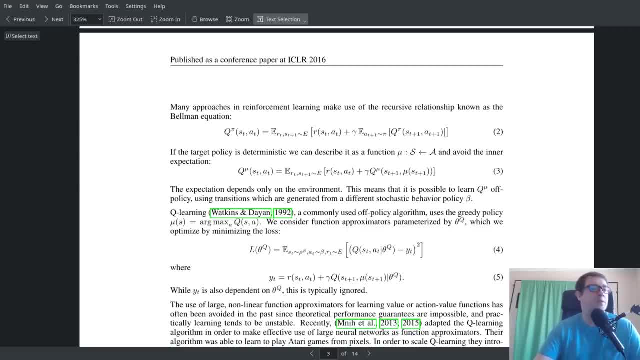 which is say explicitly with a stochastic policy. So we are actually going to have two different policies in this case. So then, this already answers the question of how we go from a deterministic policy to solving the explore-exploit dilemma, And the reason is that 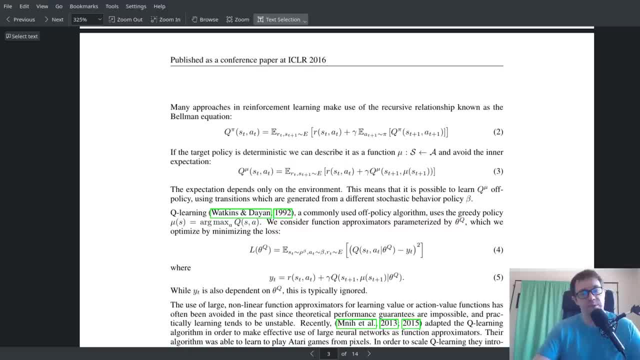 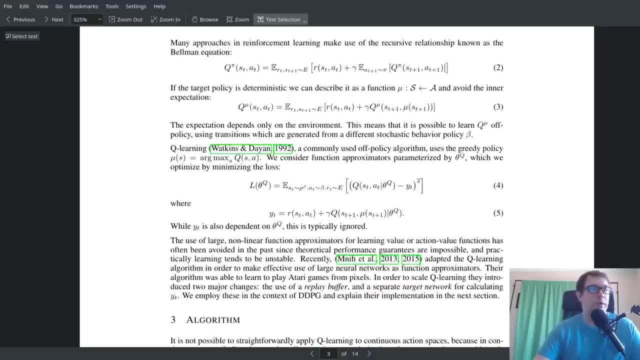 we're using a stochastic policy to learn the greedy policy or a- sorry, a purely deterministic policy. And of course they talk about the parallels with Q-learning, because there are many between the two algorithms And you get to the loss function, which is 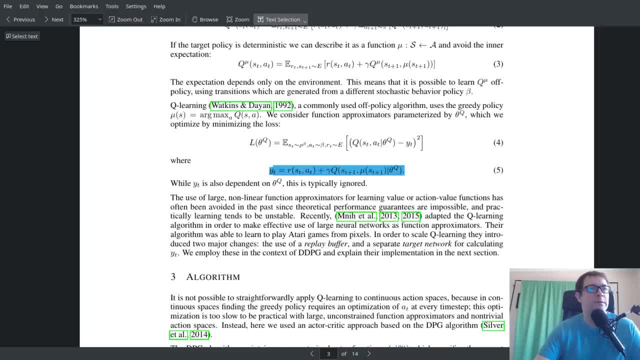 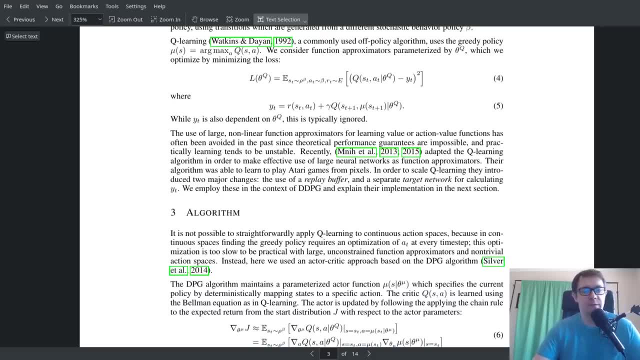 of course, critical to the algorithm and this Y of T parameter. Then, of course, they talk about what Q-learning has been used for. They make mention of deep neural networks, which is, of course, what we're going to be using. That's where the deep comes from And it talks about. 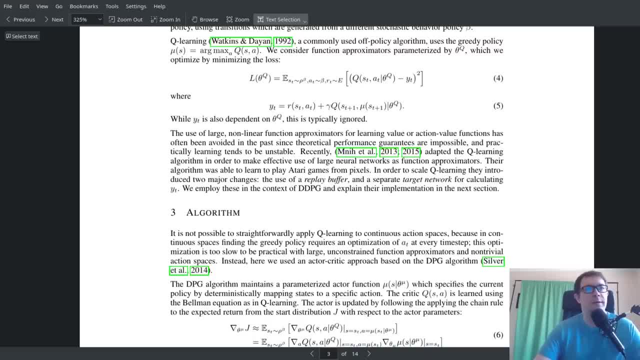 the Atari games, Which we've talked about on this channel as well, And, importantly, they say, the two changes that they introduce in Q-learning, which is the concept of the replay buffer and the target network, which, of course, they already mentioned before. 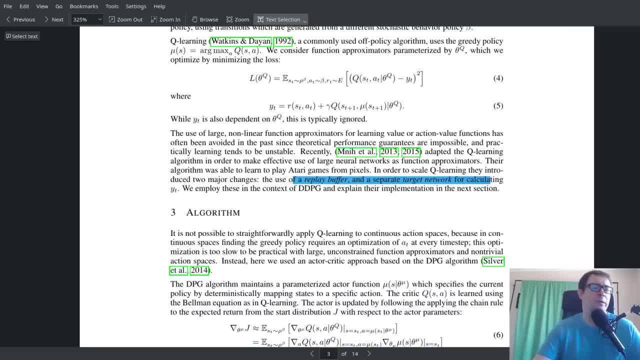 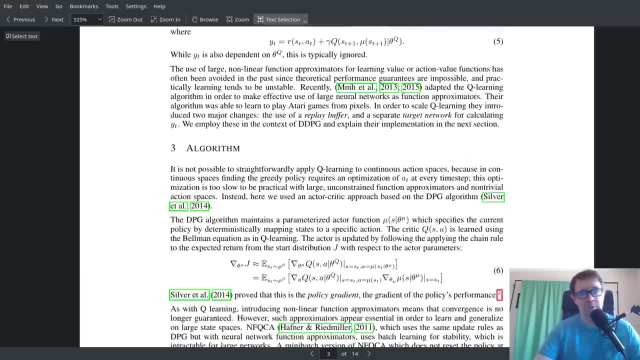 They're just reiterating and reinforcing what they said. That's why we want to read the introduction and background type material to get a solid idea of what's going to happen. So now we get to the algorithmic portion, and this is where all of the magic happens. 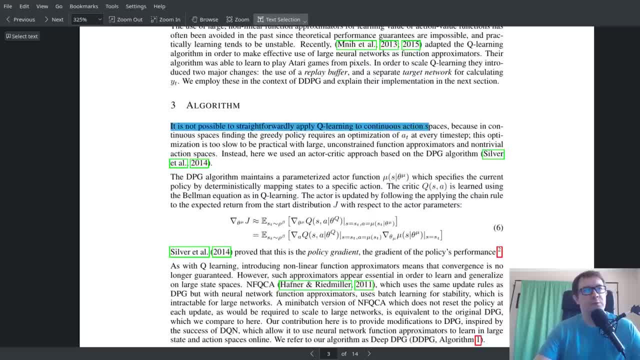 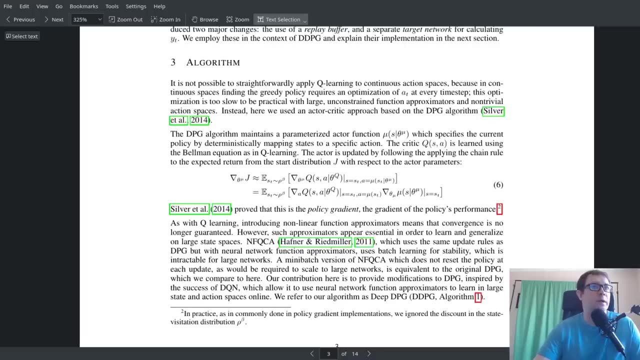 So they again reiterate that it's not possible to apply Q-learning to continuous action spaces, Because you know reasons. It's pretty obvious. You have an infinite number of actions. That's a problem. And then they talk about the deterministic policy gradient algorithm, which we're not going to go too deep into. 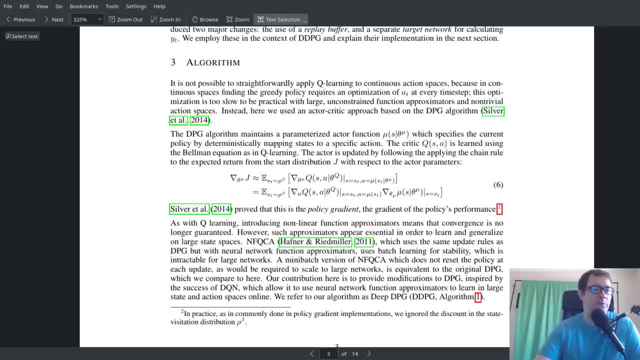 For this video. we don't want to do a full thesis, We don't want to do a full doctoral dissertation on the field. We just want to know how to implement it and get moving. So this goes through and gives you an. 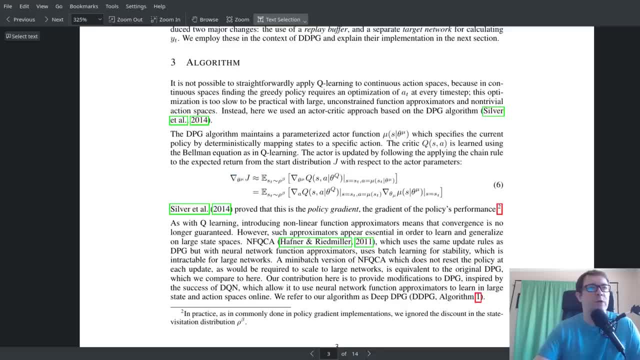 update for the gradient of this parameter j and gives it in terms of the gradient of q, which is the state action value function, and the gradient of the policy, the deterministic policy, mu Other thing to note here is that this gradients, these gradients, are over two different. 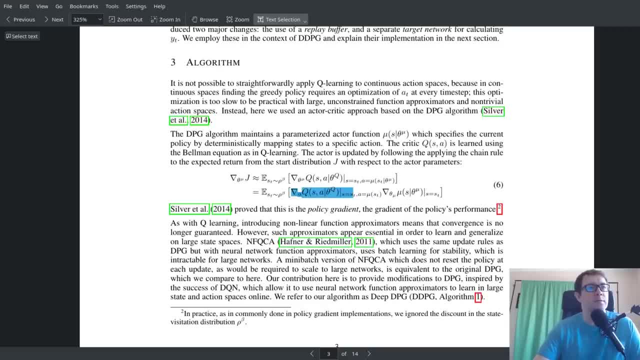 parameters. So the gradient of q is with respect to the actions, such that the action a equals mu of s of t. So what this tells you is that q is actually a function not just of the state but is intimately related to that policy mu. So it's not. it's not an action chosen according. 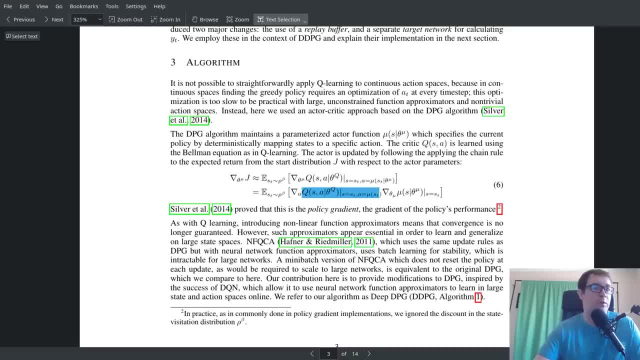 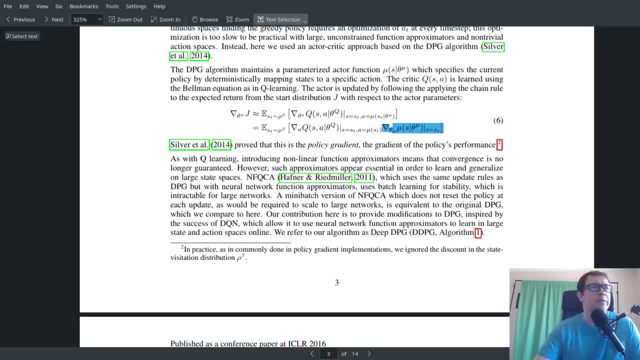 to an argmax, For instance, it's an action short chosen according to the output of the other network, And for the update of mu, it's just the gradient with respect to the weights, which you would kind of expect. So they talk about another algorithm, NFQCA. I don't know what that is, honestly. 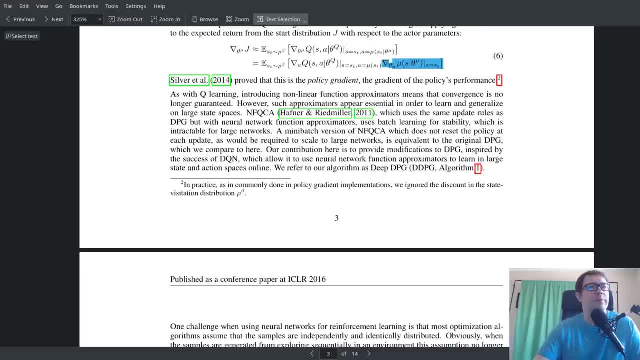 mini batch version: blah blah blah. Our contribution here is to provide modifications to DPG inspired by the success of DQN, which allowed us neural network function approximators to learn in large state and action spaces online. We call it DDPG- very creative, As they say. 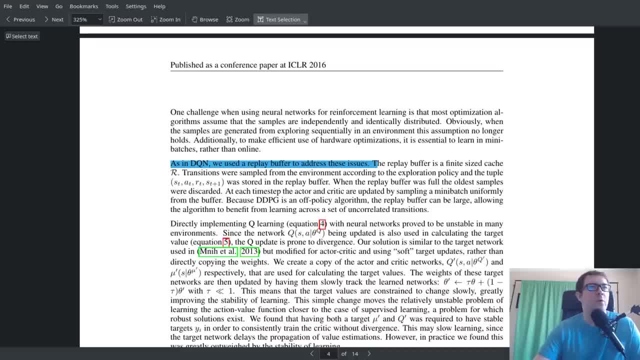 again, we use a replay buffer to address the issues of correlations between samples generated on subsequent steps within an episode. finite size, cache size, are transition sample from the environment. So we know all of this. So, if you don't know all of it, what you need to know here, 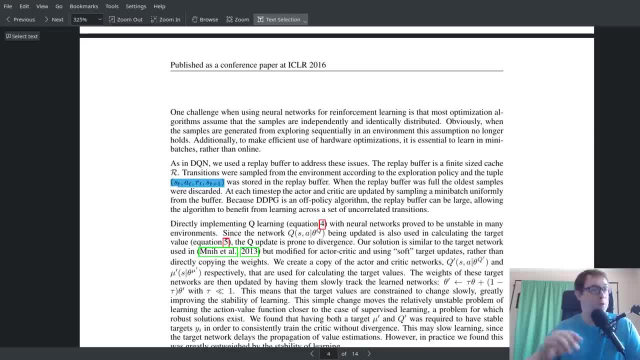 is that you have state action, reward and then new state transition. So what this tells the agent is: started in some state s, took some action, receive some reward and ended up in some new state. Why is that important? It's important because in in anything that isn't, 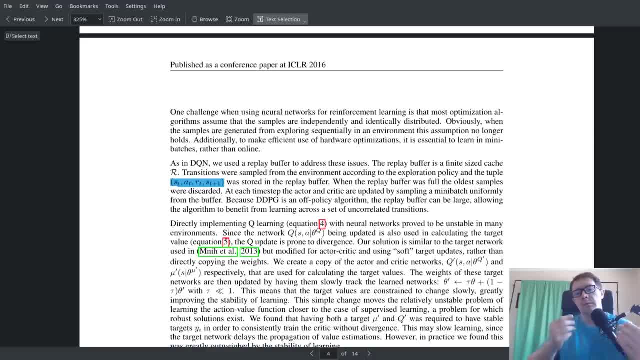 dynamic programming. you're really trying to learn the state probability distributions. you're trying to learn the probability of going from one state to another and receiving some reward along the way. If you knew all those beforehand, then you could just simply solve a set of very, very large set of equations, for that matter, to arrive at the optimal solution. 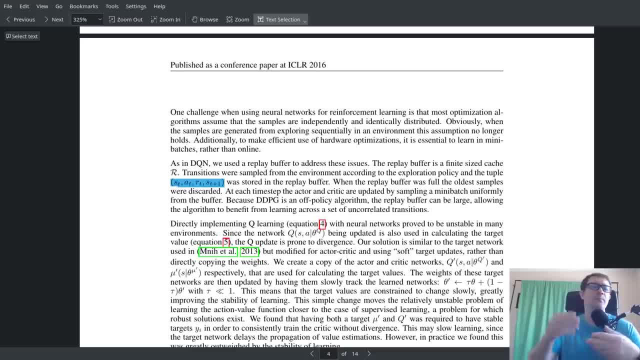 right. If you knew all those transitions. you say, okay, if I start in this state and take some action, I'm going to end up in some other state, with certainty. then you'd say, well, what's the most advantageous state? What state is going to give me the? 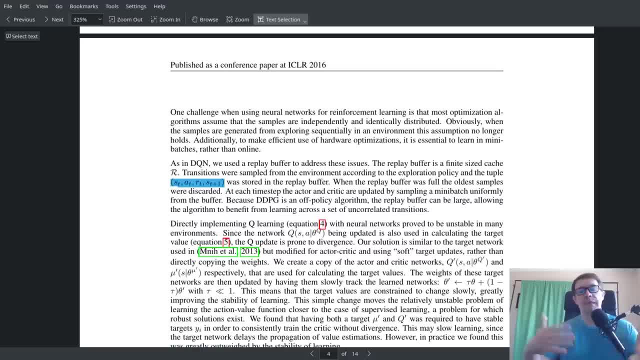 largest reward, And so you could kind of construct some sort of algorithm for traversing that set of equations to maximize your reward over time. Now, of course, you often don't know that, And that's the point of the replay. buffer is to learn that through experience and interacting with the 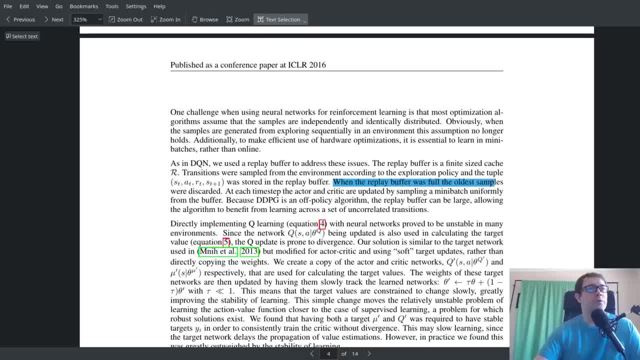 environment. And it says: when the replay buffer was full, all the samples were discarded. Okay, that makes sense. It's finite size. it doesn't grow indefinitely. At each time, step actor and critic are updated by sampling a mini batch uniformly from the buffer. So it operates exactly. 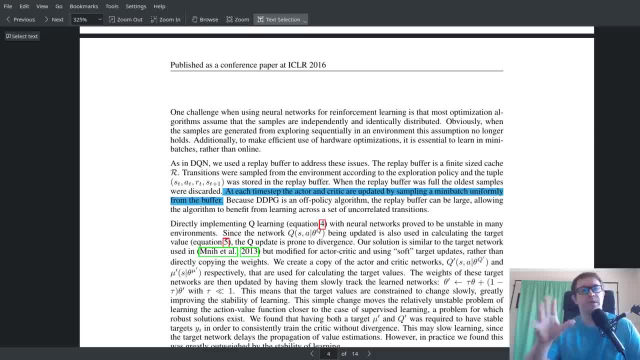 according to Q learning, it does a uniform sampling- random sampling of the buffer- and uses that to update the actor and critic networks. What's critical here is that- combining this statement with the topic of the previous paragraph- is that when we write our replay, 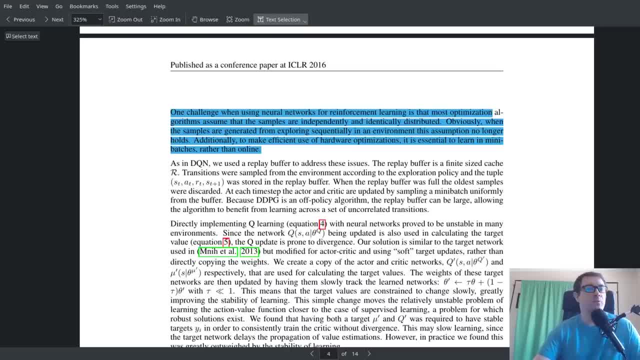 buffer class, it must sample states at random. So what that means is you don't want to sample a sequence of subsequent steps, And the reason is that there are large correlations between those steps, right as you might imagine, And those correlations can cause you to get trapped. 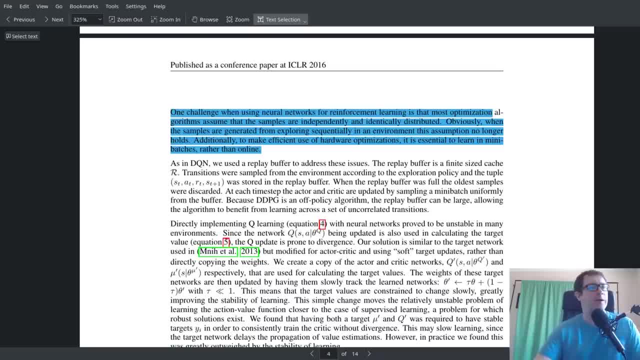 in little nicks, nooks and crannies of parameter space and really cause your algorithm to go wonky. So you want to sample that uniformly. So that way you're sampling across many, many different episodes to get a really good idea of the- I guess, the breadth of the parameter space. 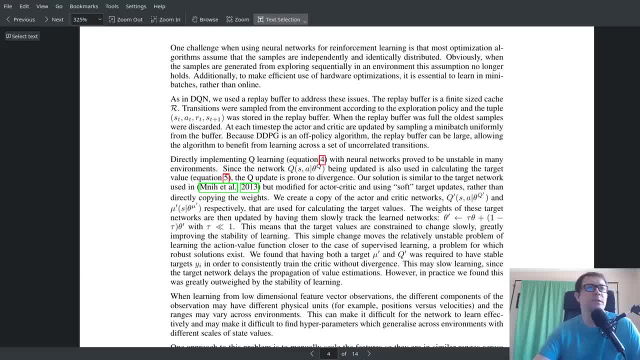 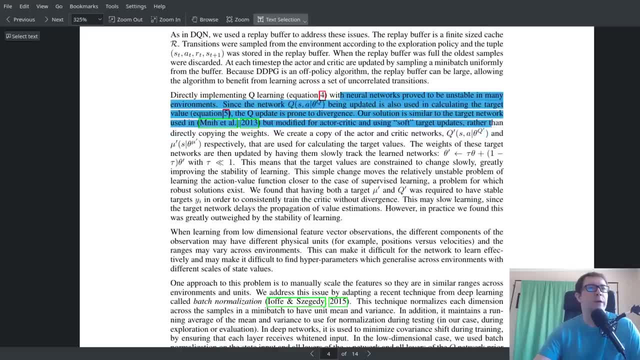 to use kind of loose language. And then it says: directly implementing Q learning with neural networks prove the unstable many environments. And they're they're going to talk about using the, the target network. okay, but modified for actor critic using soft target updates. 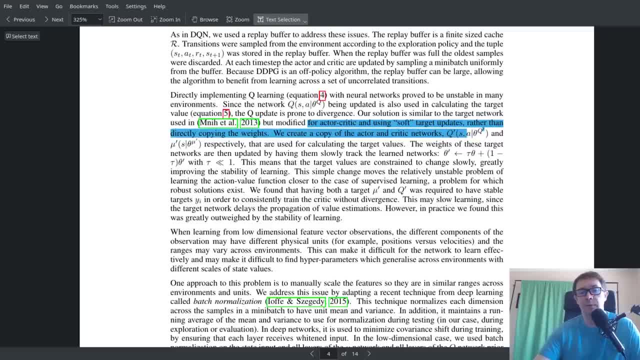 rather than directly copying the weights. So in Q learning we directly copy the weights from the evaluation to the target network. Here it says we create a copy of the actor and critic networks- Q prime and mu prime respectively- that are used for calculating. 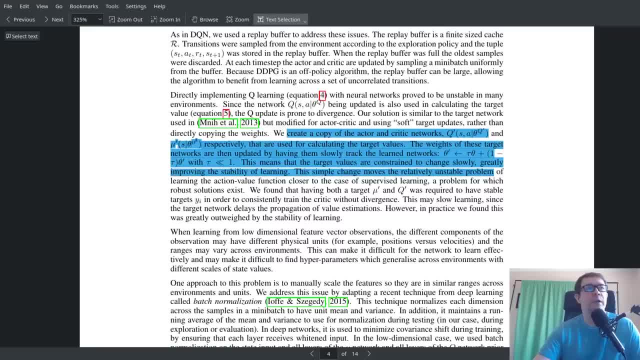 the target values. The weights of these target networks are then updated by having them slowly track the learn networks. theta prime goes to theta. theta times tau plus one minus tau times theta prime with tau much, much less than one. This means that the target values are constrained to change slowly, greatly improving. 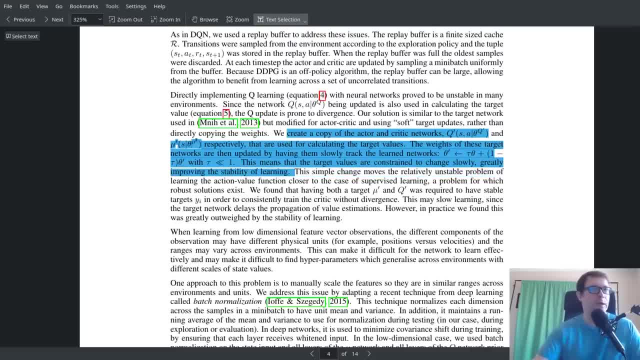 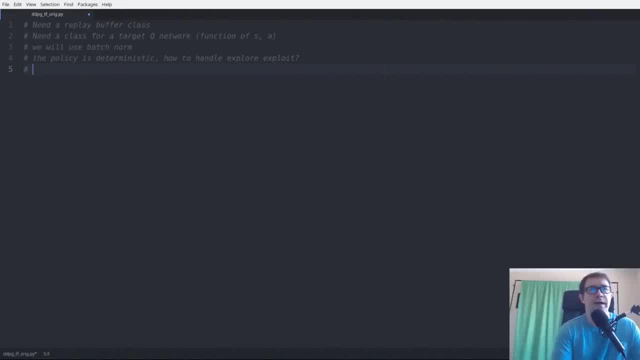 the stability of learning. Okay, so this is our next little nugget, So let's head it over to the paper and make to our text editor and make note of that. What we read was that the we have to not in caps. we don't want to shout. we have two networks: target networks and 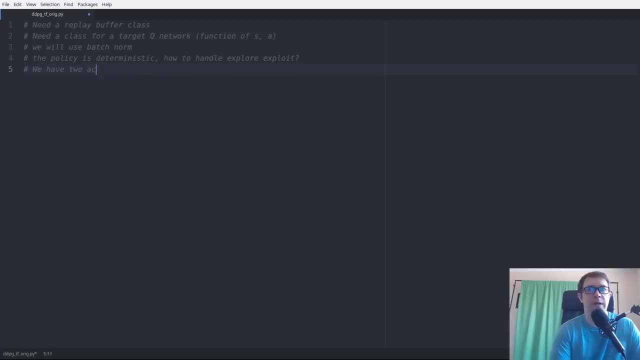 critics. Sorry, we have two actor and two critic networks, a target for each. Updates are soft according to: theta equals tau times theta plus one minus tau times theta prime. So sorry, this should be theta. So this is the update rule for the parameters of our target networks And we have two target. 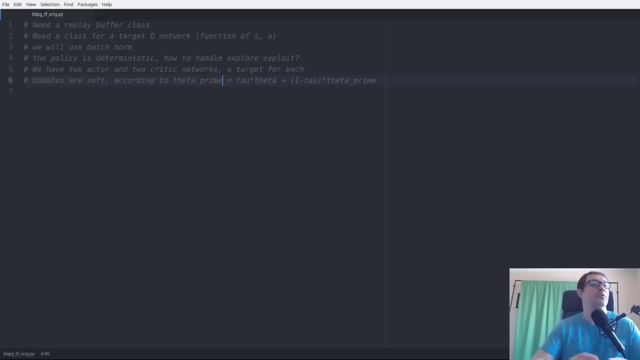 networks, one for the actor and one for the critic, So we have a total of four deep neural networks, And so this is why the algorithm runs so slowly. even on my beastly rig It runs quite slowly even in the lunar lander and continuous lunar lander environment. I've 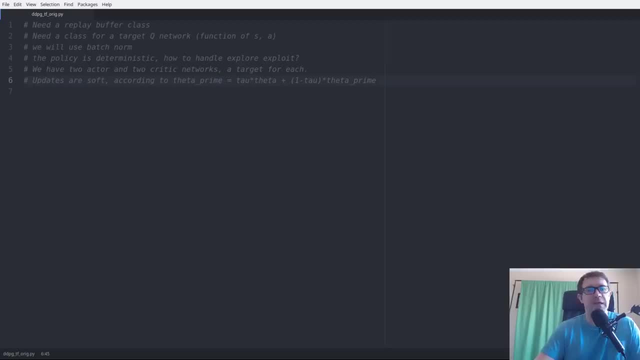 done the bipedal Walker and it took about 20,000 games to get something that approximately approximates a decent score. So this is a very, very slow algorithm And that 20,000 games took, I think, about a day to run. So quite slow but nonetheless quite powerful. 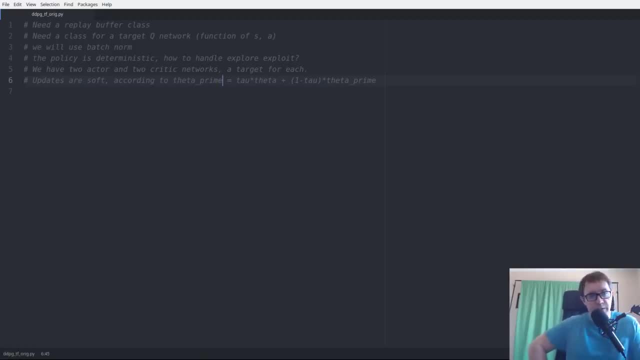 It's the only method we have so far of implementing a deep reinforcement, learning and continuous control environments. So, Hey, you know beggars can't be choosers, right? But we know, just to recap, that we're going to use four networks: two that are on policy and two off policy. 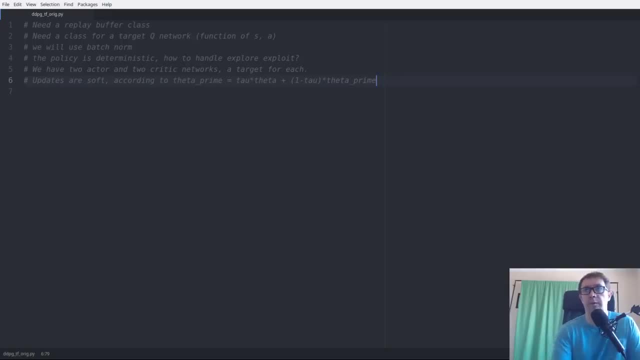 The updates are going to be soft with tau. much less than 1.. If you're not familiar with mathematics, this double less than or double greater than sign means much less than or much greater than respectively. So what that means is that tau is going to be of order 0.01 or smaller right. 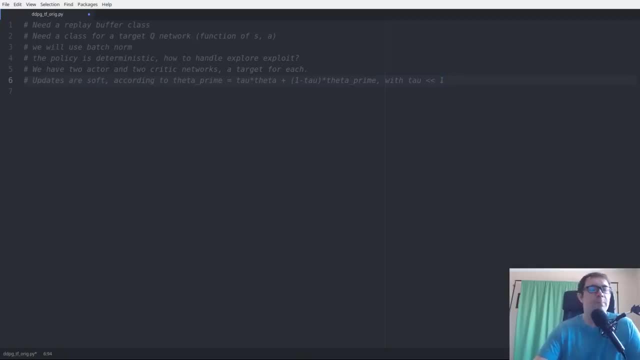 0.1 isn't much smaller. That's kind of smaller 0.01. I would consider much smaller They use. we'll see in the details. we'll see what value they use, but you should know that it's of order 0.01 or smaller. 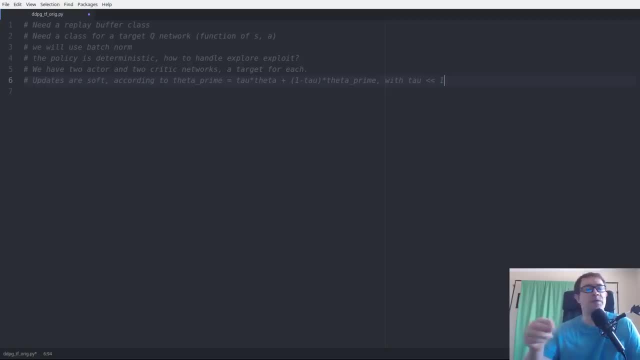 And the reason they do this is to allow the updates to happen very slowly, to get good convergence, as they said in the paper. So let's head back to the paper and see what other nuggets we can glean before getting to the outline of the algorithm. 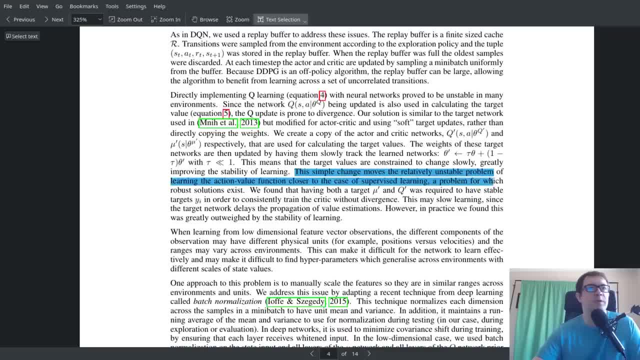 And then, in the very next sentence, they say: This simple change moves the relative unstable problem of learning the action value function closer to the case of supervised learning, a problem for which it robustly, We found that having both the target mu prime and q prime was required to have stable targets yi. 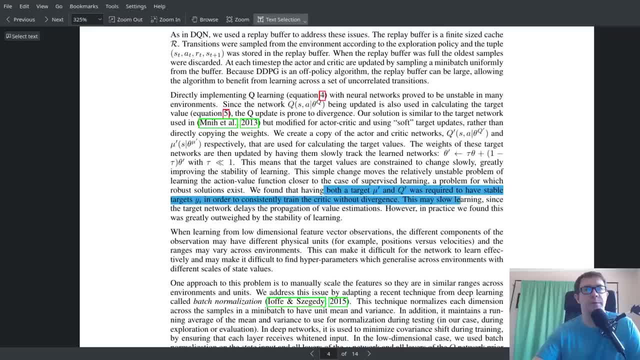 in order to consistently train the critic without divergence. This may slow learning, since the target networks delay the propagation of value estimates. However, in practice, we found this was always greatly outweighed by the stability of learning, And I found that as well. 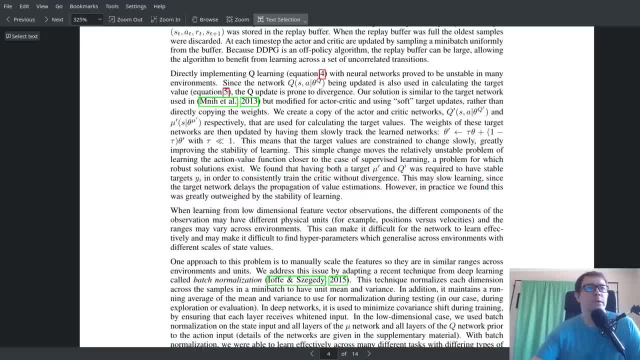 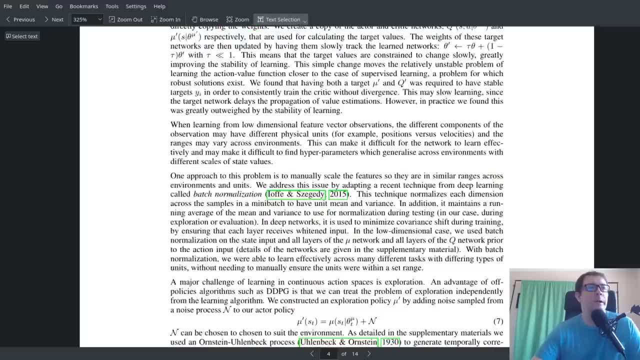 You don't get a whole lot of divergence, but it does take a while to train. Then they talk about learning in low dimensional and higher dimensional environments, And they do that to talk about the Need for feature scaling. So one approach to the problem, which is the ranges of variations in parameters, right. 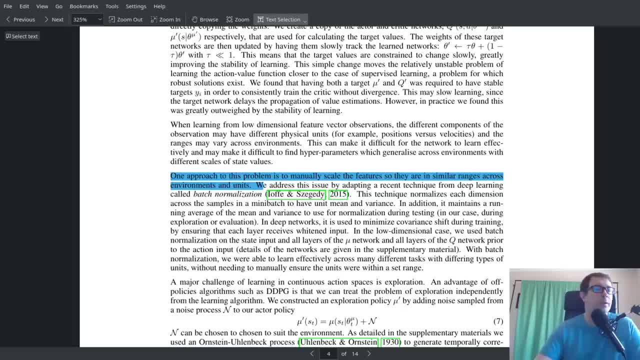 So in different environments, like in a mountain car, you can go from plus minus 1.6, minus 1.6 to 0.4, something like that, And the velocities are plus minus 0.07.. So you have a two order magnitude variation there in the parameters. 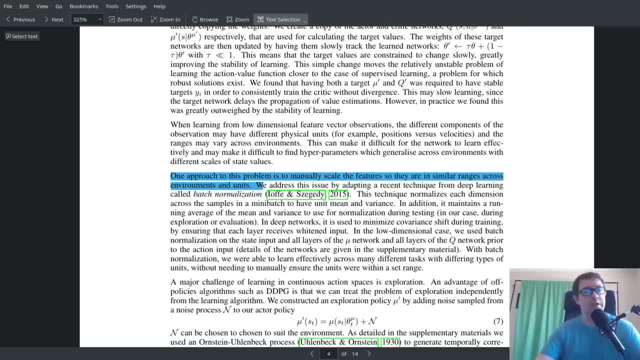 That's kind of large even in that environment. And then when you compare that to other environments where you can have parameters that are much, much larger, in the order of hundreds, you can see that there's a pretty big issue with the scaling of the inputs to the neural network. 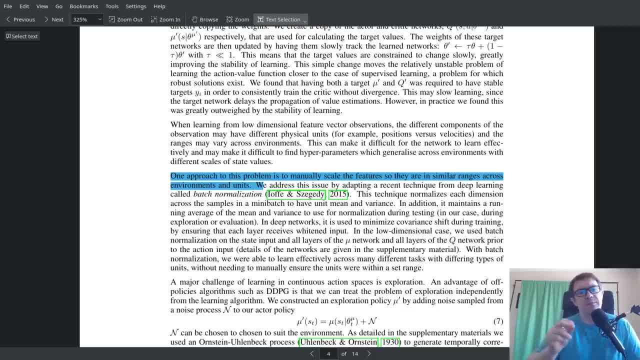 which we know from our experience that neural networks are highly sensitive to the scaling between inputs, So they're. solution to that problem is to manually scale the features So they're in similar across environments and units, And they do that by using batch normalization. 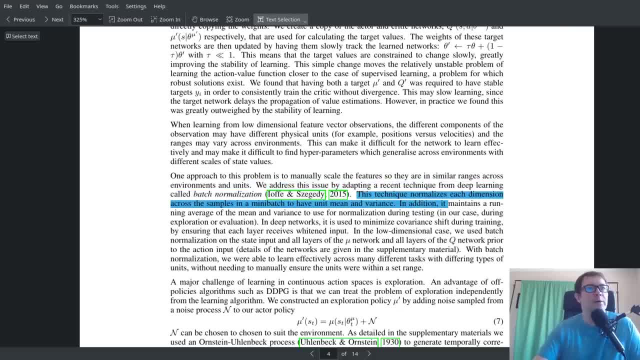 And it says: this technique normalizes each dimension across the samples in a mini batch dev unit- Mean and variance- and also maintains a running average of mean and variance use for normalization during testing, during exploration and evaluation. So in our case, training and testing are slightly different than in the case of supervised learning. 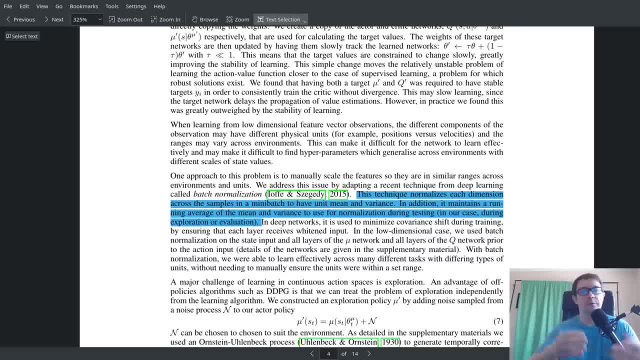 So supervised learning. you've maintained different data sets or shuffled subsets of a of a single data set to do training and evaluation And, of course, in the evaluation phase you perform no weight updates of the network. you just see how it does based on the training. 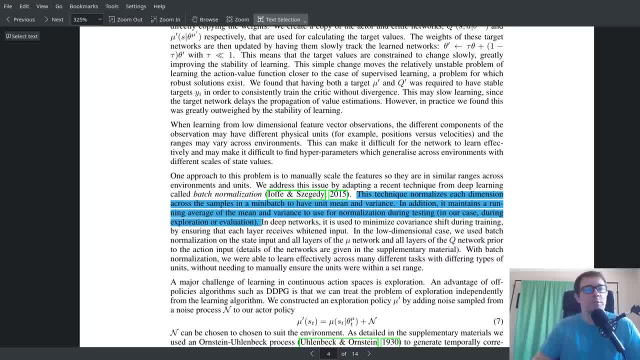 And reinforcement learning. you can do something similar where you have a set number of games where you train the agent to achieve some set of results And then you turn off the learning and allow it to just choose actions based upon whatever policy it learns. And if you're using batch normalization in pytorch in particular, there are significant differences in how batch normalization is used in the two different phases. 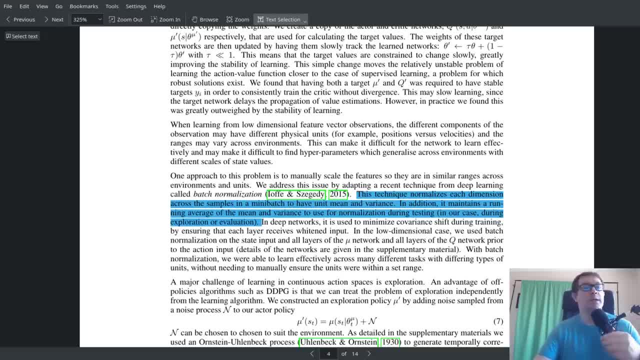 So you have to be explicit in setting training or evaluation mode. In particular, in pytorch they don't track statistics in evaluation mode, which is why, when we wrote the DDPG algorithm in pytorch, we had to call the eval and train functions so often. 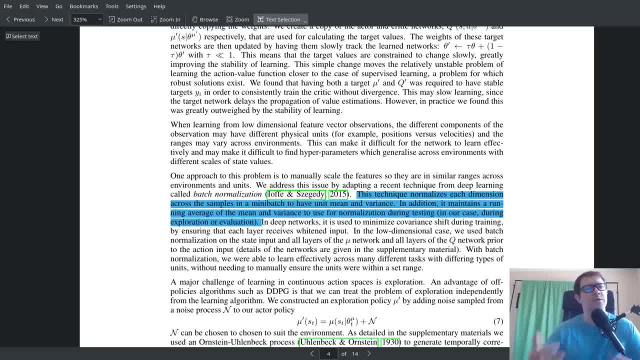 Okay, so we've already established we'll need batch normalization, So everything's kind of starting to come together. we need a replay network, batch normalization. we need four networks. right, we need to. we need to each of a target of an actor and to each of a critic. 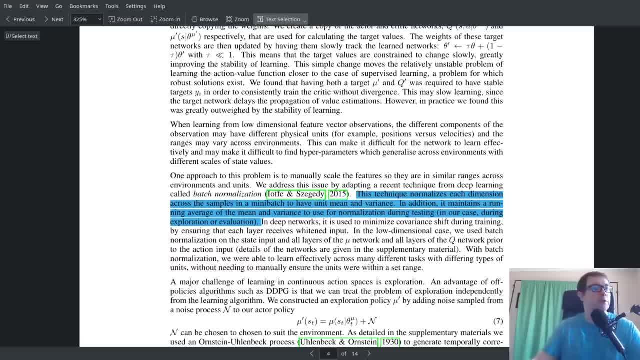 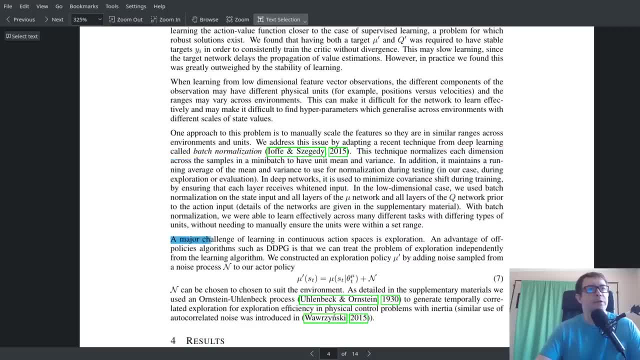 Okay, Half of those are going to be used for on policy and half of them are going to be used for off policy, for the targets. And then it says, if you scroll down, a major challenge of learning in continuous action spaces is exploration. 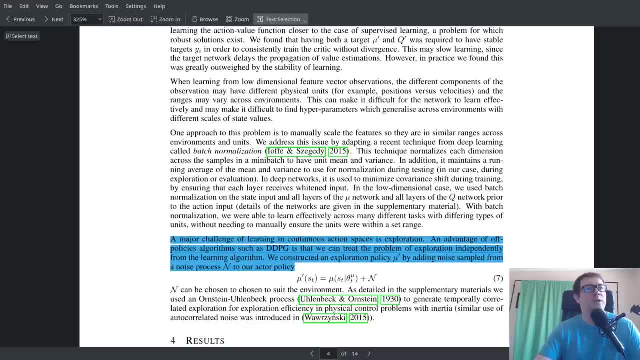 An advantage of off policy algorithms such as DDPG is that we can treat the problem of exploration independently from the learning algorithm. We constructed an exploration policy, mu prime- by adding noise sampled from a noise process n to our actor policy. Okay, so right here it's telling us what the basically the target actor function is. it's mu prime is basically mu plus some noise n. 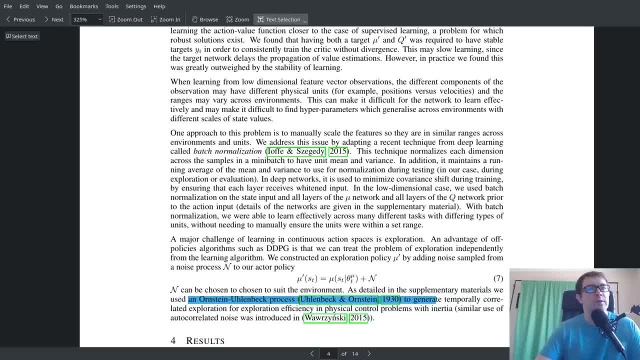 n can be chosen to suit the environment, as detailed in the supplementary materials we use in Orenstein-Uhlenbeck process to generate temporally correlated exploration for exploration efficiency and physical control. problems with inertia. If you're not familiar with physics, inertia just means the 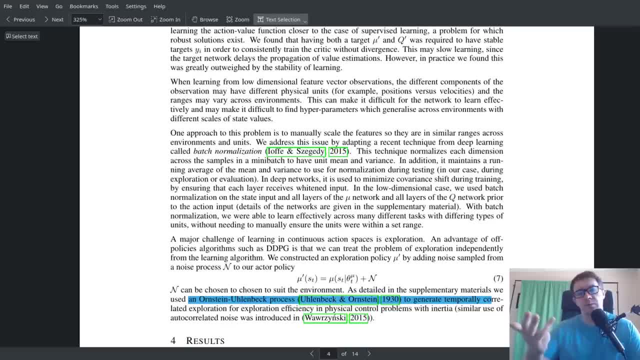 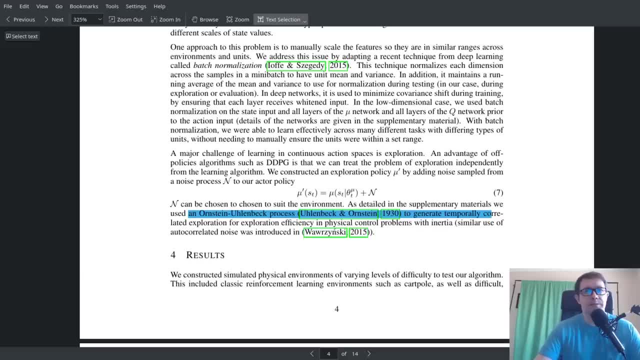 Tendency of stuff to stay in motion has to do with like environments that move, like the walkers, the cheetahs, stuff like that, the ants. Okay, so we've kind of uh got one other nugget to add to our text editor. 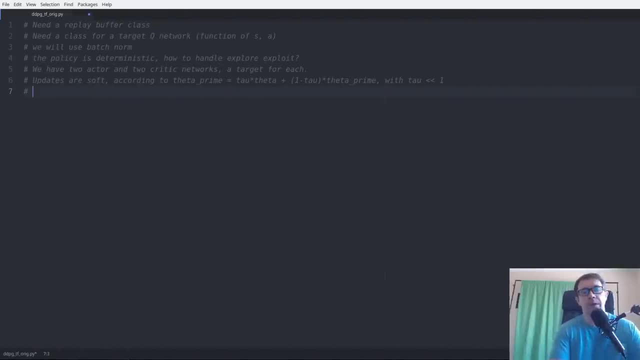 Let's head back over there and write that down, Okay, so, uh, the target uh actor is just the um, evaluation. We'll call it that for like of a better word: evaluation actor plus some noise process. they used ornstein, uh, ulan beck, i don't. 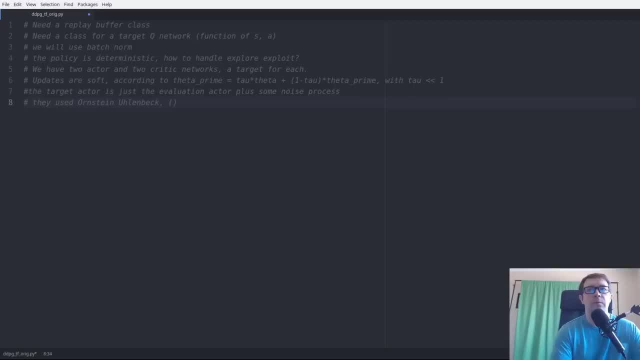 think i spelled that correctly. um, we'll need to look that up. uh that i've already looked it up. um, my background is in physics, so it made sense to me. it's basically, uh, a noise process that models the motion of browning particles, which are just particles that move around, uh, under the influence. 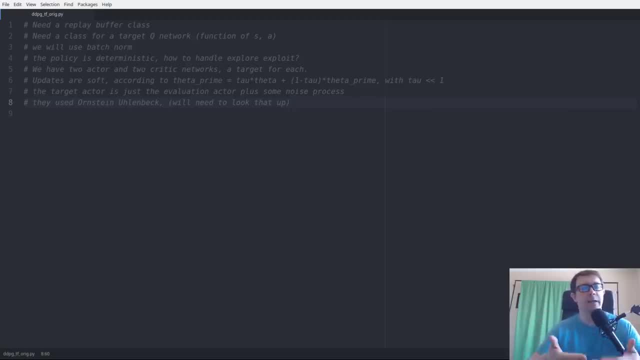 of their interaction with other particles in some type of medium, like a lossless medium, like a, a perfect fluid or something like that. um, and in the ornstein ullenbeck case, they are temporally correlated, meaning each time step is related to the time step prior to it. and i hadn't thought. 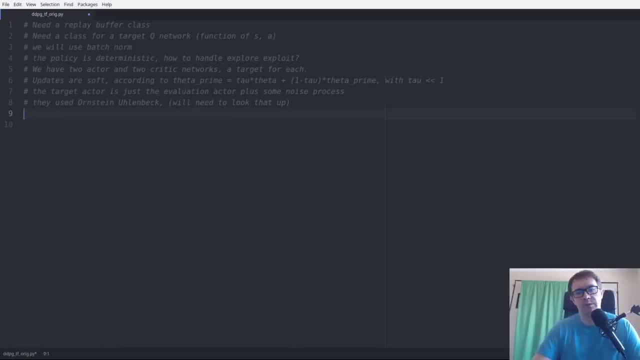 about it before, but that's probably important for the case of markov decision processes, right? so in mdps the current state is only related to the prior state and the action taken. you don't need to know the full history of the environment. so i wonder if that was chosen that way. if 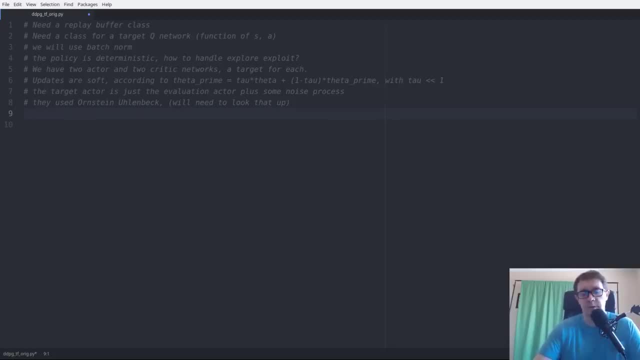 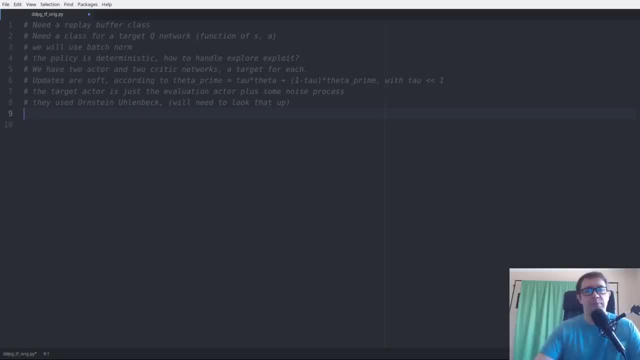 my head. i don't know the answer to that. if someone knows, hey, drop the answer in the comments. i would be very curious to see the answer. so, uh, we have enough nuggets here. so just to summarize: we need a replay buffer class. uh, we'll also need a class for the noise, right? so we'll need a. 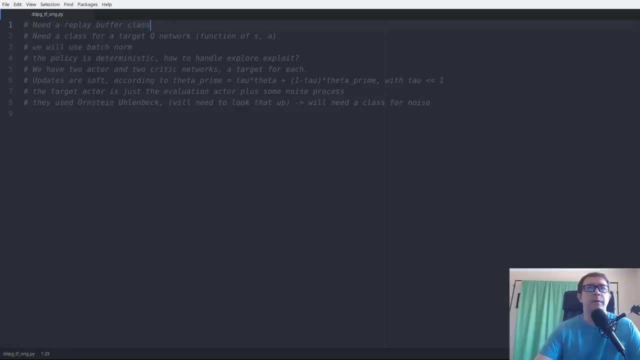 class for noise, a class for the replay buffer? uh, we'll need a class for the target queue now. uh, we'll need a class for the target queue now. we'll need a class for the target queue now. and we're going to use batch normalization. uh, the policy will be deterministic. so what that means. 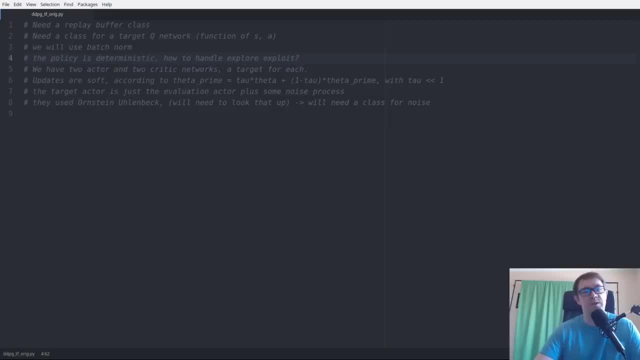 in practice is that the policy will output the actual actions instead of the probability of selecting the actions. so the policy will be limited by whatever the action space of the environment is, so we need some way of taking that into account. so so deterministic policy means outputs the actual action instead. 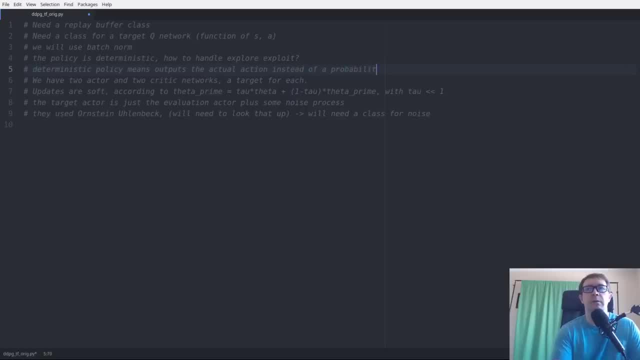 of a probability. we'll need a way to bound the actions to the environment, environment limits and, of course, these notes don't make it into the final code. these are just kind of things you think of as you are reading the paper. uh, you would want to put all your questions here. uh, i don't have. 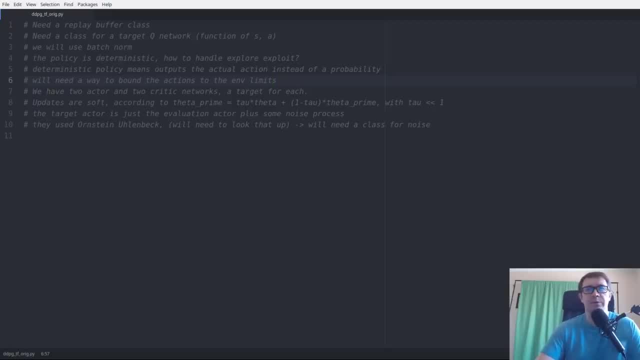 questions, since i've already implemented it, but this is kind of my thought process as i went through it the first time. um, as best as i can model it after having finished the problem, and that it's pretty simplified and uh as go, chatters are a little more complicated. 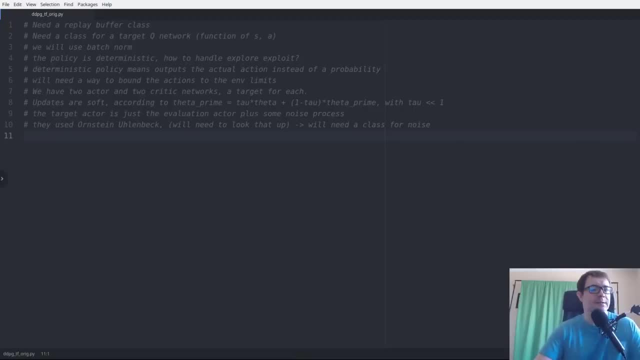 but you could also use a sheet of paper with some kind of magic about writing stuff down on paper, but we're going to use the code editor because i don't want to use an overhead projector to show you guys a freaking sheet of paper. this isn't grade school here, so let's head back to the 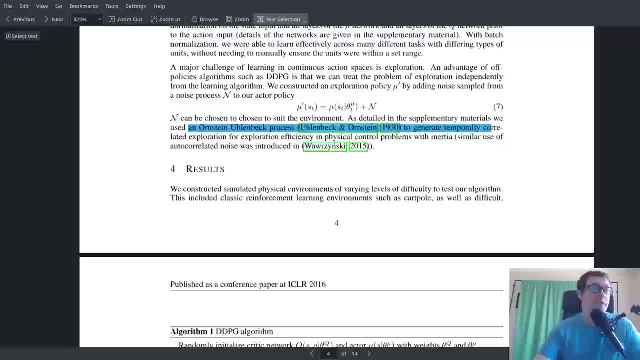 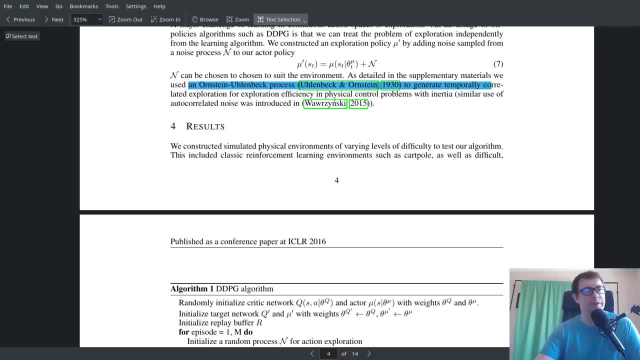 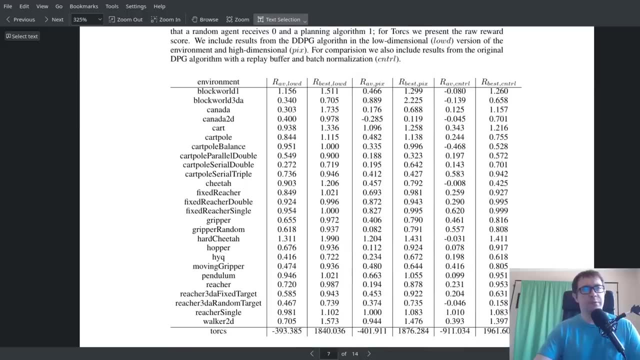 paper and uh, take a look at the actual algorithm to get some real sense of what we're going to be implementing the. the results really aren't super important to us yet. uh, we will use that later on if difficult, right? so scroll down to the data really quick so they give another thing to note. i didn't 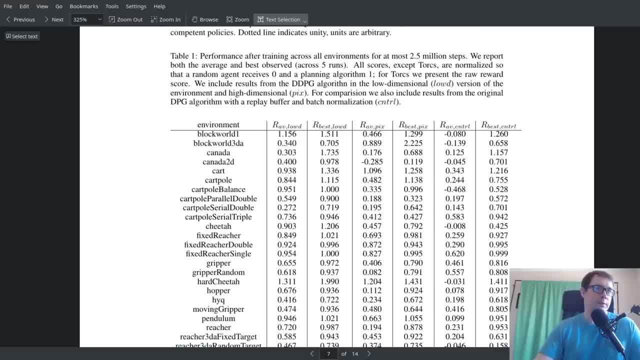 talk about this earlier, but i guess now is a good time. is the stipulations on this? on this, performance data says performance after training across all environments for at most 2.5 million steps. so i said earlier i had to train the bipedal walker for around 20 000 games. that's around um times. 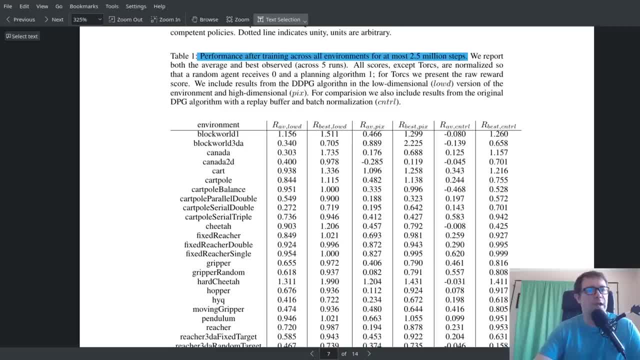 i think that's around about about two and a half million steps or so. i think it was actually on 15 000 steps, so maybe around three million steps, something like that. we report both the average and best observed across five runs, so why would they use five runs? so this was a super duper. 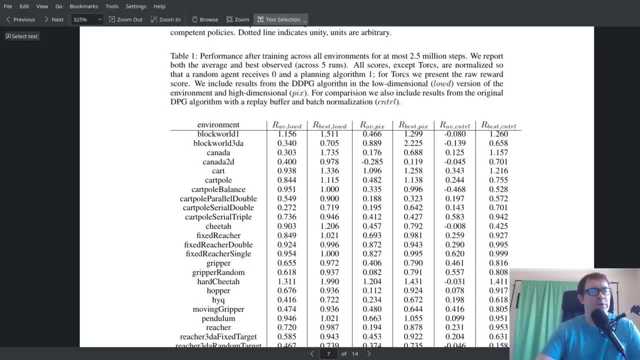 algorithm and which none of them are. this isn't a slight on their algorithm. this isn't meant to be snarky or anything. what it tells us is that they had to use five runs because there is some element of chance involved. so you know, in one problem with deep learning is the problem of, uh, replicability. right, it's hard to. 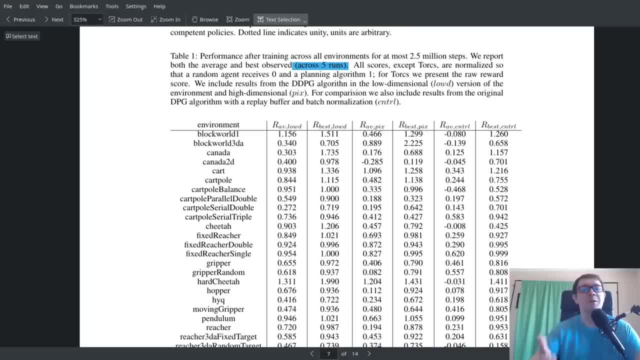 replicate other people's results. if, particularly if you use system clocks as seeds for random number generators- right, using the system clock to to seed the random number generator guarantees that, if you run the simulation at even a millisecond later, right, uh, that you're going to get different results because you're going to be starting with different sets of parameters now you. 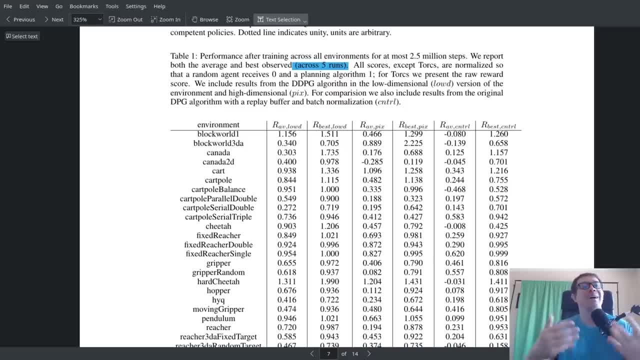 you'll be able to repeat the, the general idea of the experiments, but you won't get the exact same results. um, it's kind of what. it's an objection to the whole deep learning phenomenon. it makes it kind of not scientific. but whatever it works, uh has an enormous success. so we won't quibble about. 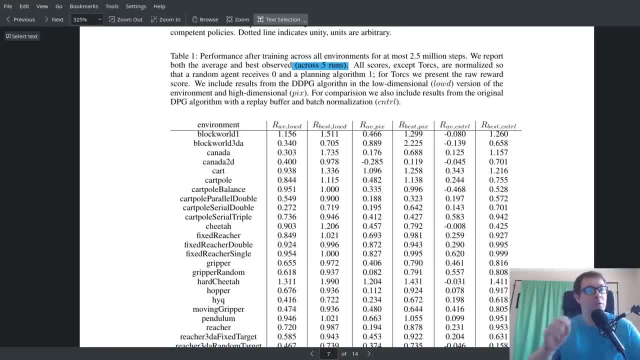 semantics or you know philosophical problems, but we just need to know for our purposes that even these people that invented the algorithm had to run it several times to get some idea of what was going to happen, because the algorithm is inherent to the algorithm and it's not going to. 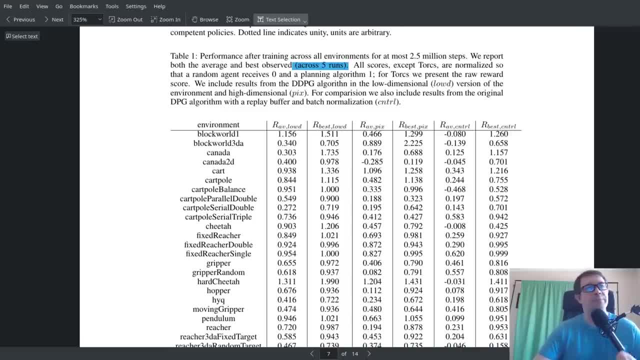 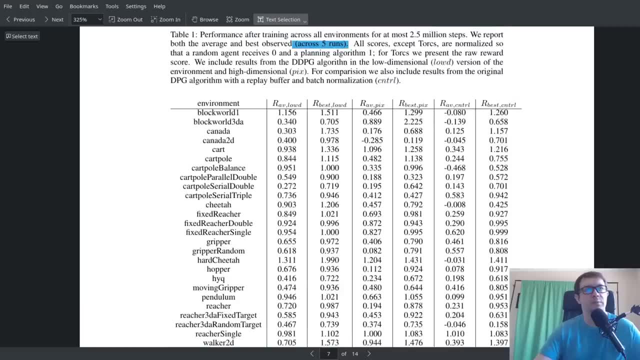 be inherently probabilistic, and so they report averages and best case scenarios. so that's another little tidbit. and they included results for both the low dimensional cases, where you receive just a state vector from the environment, as well as the pixel inputs. we won't be dealing with pixel. 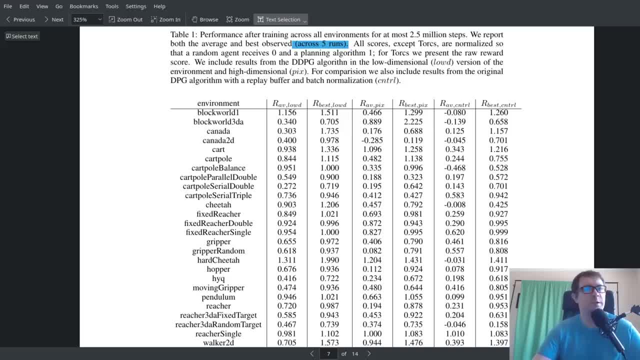 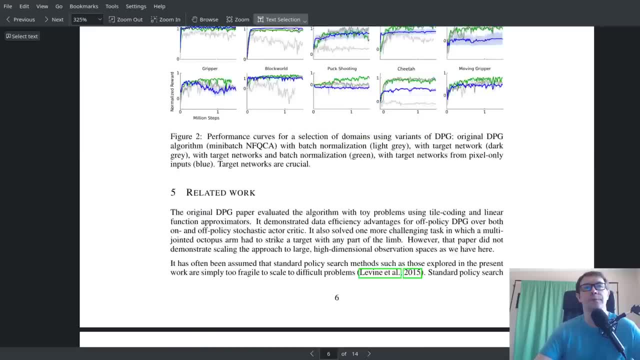 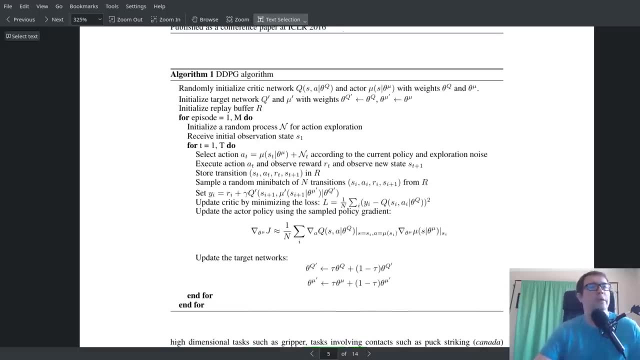 inputs for this particular video, but maybe we'll get to them later. i'm trying to work on that as well. so these are the results, and the interesting tidbit here is that it's probabilistic it's going to take five runs, so okay, fine, other than that, we don't really care about results. uh, for now. we'll take a look later, but uh, that's not. 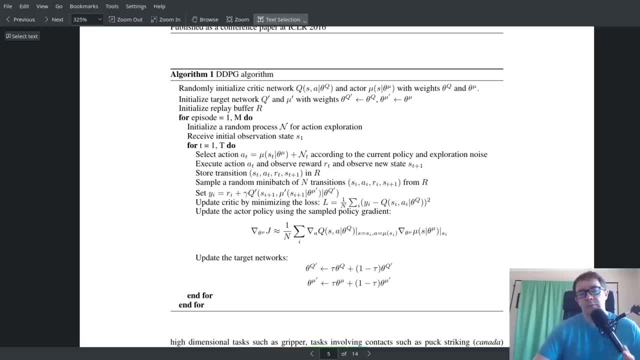 really our concern at the moment. so now we have a series of questions. we have answers to all those questions. we know how we're going to handle the explore exploit dilemma. we know the purpose of the target networks. we know how we're going to handle the noise. we know how we're going to handle 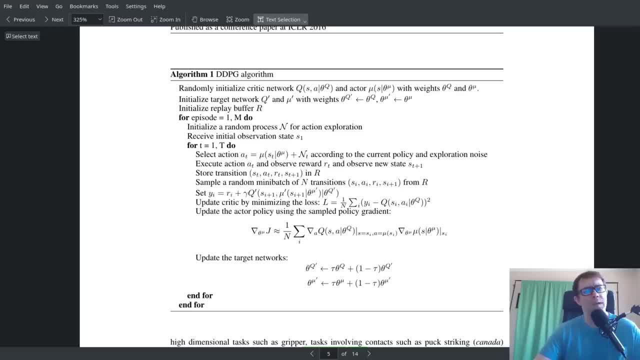 the replay buffer, um, and we know what the policy actually is going to be. it's the actual prop, it's the actual actions the agent is going to take. so we know a whole bunch of stuff. so it's time to look at the algorithm and see how we fill in all the details. so randomly initialize a critic network. 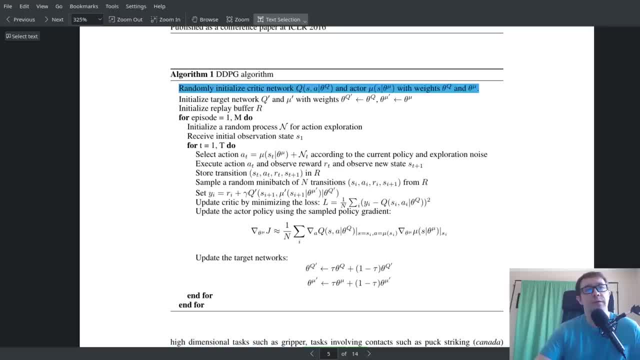 and actor network with weights: theta super q, theta super mu. so, uh, this is handled by whatever library you use, you don't have to manually initialize weights. but we do know from the supplemental materials that they do constrain these updates to be within- sorry, these initializations to be within some range. so put a note in the back of your mind that you're going to have to. 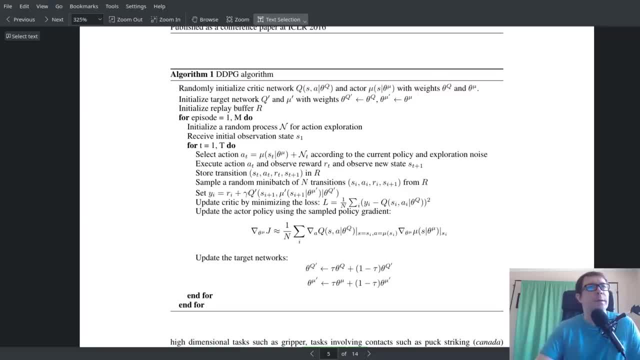 train these a little bit. and then it says: initialize target network q prime and mu prime with weights, uh that are uh equal to the original networks. so theta super q prime gets initialized with theta super q and theta mu prime gets initialized with theta super mu. so, uh, we will. 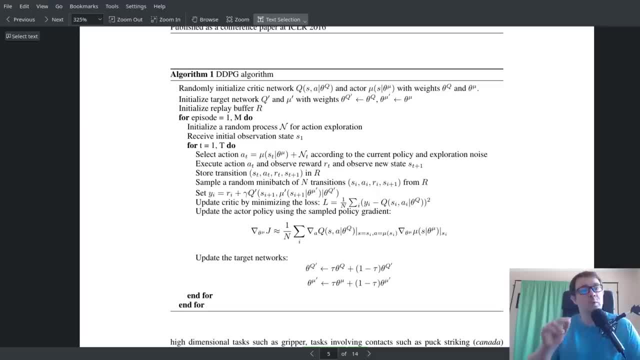 be updating the weights right off the bat for the target networks with the evaluation networks and initialize a replay buffer r. now this is an interesting question: how do you initialize that replay buffer? so i've used a couple different methods. uh, you can just initialize it with all. 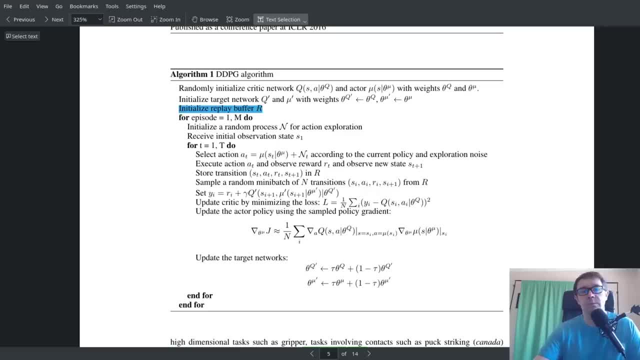 zeros. and then, if you do that, when you perform the learning you want to make sure that you have a number of memories that are greater than or equal to the mini batch size of your training, so that way you're not sampling the same states more than once. right, if you have 64 memories in? 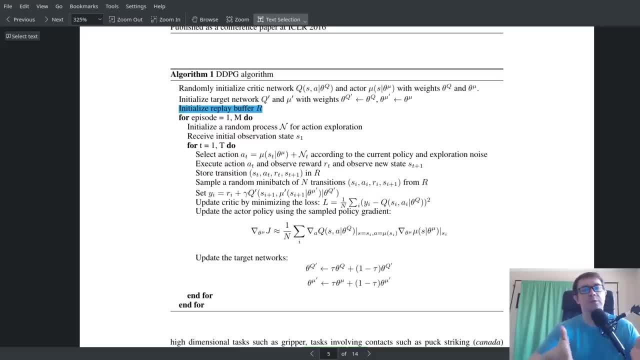 a batch that you want to sample, but you only have 10 memories, you're going to have to initialize in your replay buffer. then you're going to sample, let's say, 16 memories and you're going to sample each of those memories four times, right? so then that's no good. so the question becomes: if you 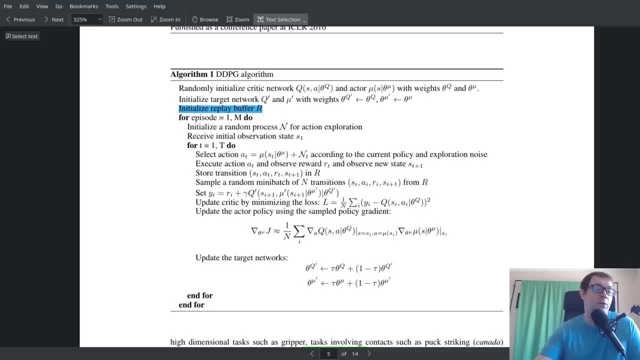 update. if you initialize your replay buffer with zeros, then you have to make sure that you don't learn until you exit the warm-up period, where the warm-up period is just a number of steps equal to your replay buffer- uh, your buffer sample size- or you can initialize it with the actual environmental. 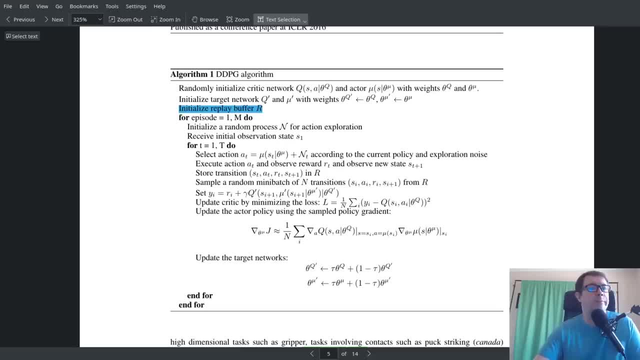 play. now this takes quite a long time. uh, you know, the replay buffers are border a million. so if you let the uh the algorithm take lane steps at random, then it's going to take a long time. i always use zeros and then, you know, just wait until the agent fills up the mini batch size of memories. just a minor detail there. 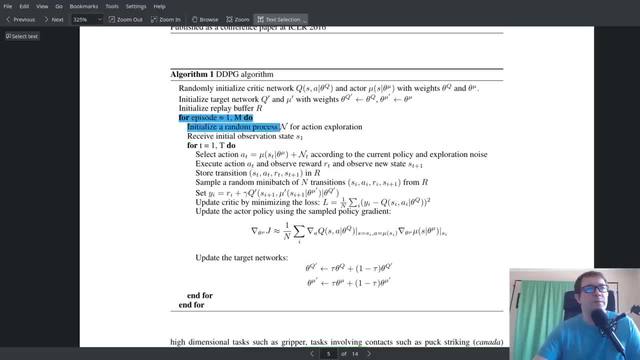 then it says: for some number of episodes due, so a for loop, initialize a random process, end for action: exploration. so this is something. now, reading it, i actually made a little bit of a mistake. so i'm going to initialize it with a for loop and then i'm going to initialize it with a. 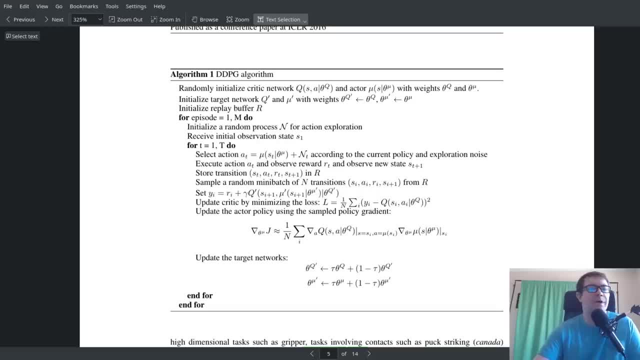 so, uh, in my previous implementation i didn't reset the noise process at the top of every episode, uh, so it's explicit here. i must have missed that line. um, and i've looked at other people's code. um, some do, some don't. uh, but it worked. uh, within uh, how many episodes was it? 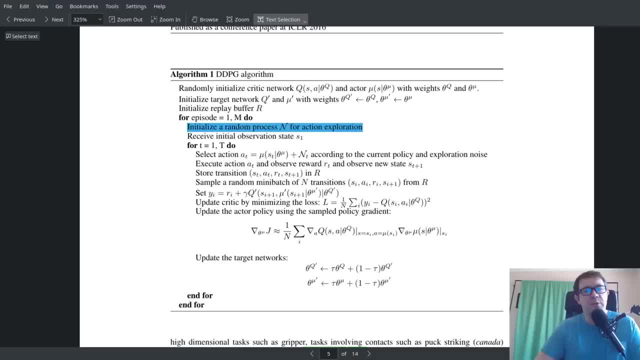 within a, uh, under a thousand episodes, the agent managed to beat the continuous lunar environment. so is that critical? maybe not. um, and i think i mentioned that in the video, receive your initial state, observation s1. so for each step of the episode, t equals one to capital t. 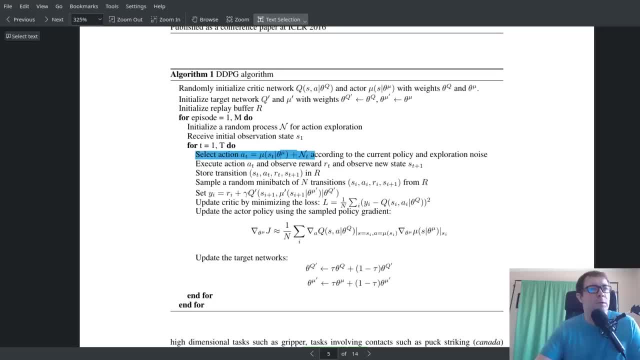 do select the action. a sub t equals mu. the policy plus n sub t, according to the current policy and exploration noise. okay, so that's straightforward, just use just feed the state forward. what does that mean? it means feed the state forward through the network, receive the vector output of the. 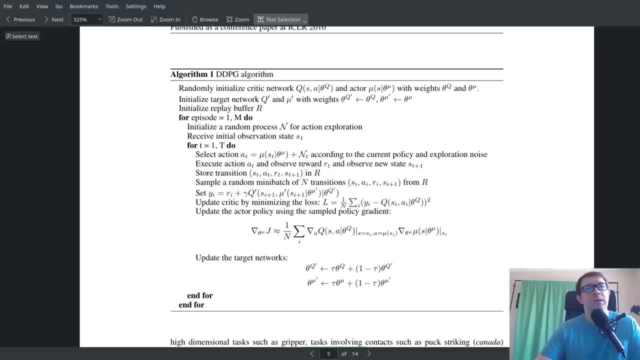 action and add some noise to it. okay, execute that action and receive and observe reward and new state. simple store that transition. you know the old state, action reward, a new state in your replay buffer are. okay, that's straightforward. each time step sample a random mini batch of n transitions from the replay buffer and then you 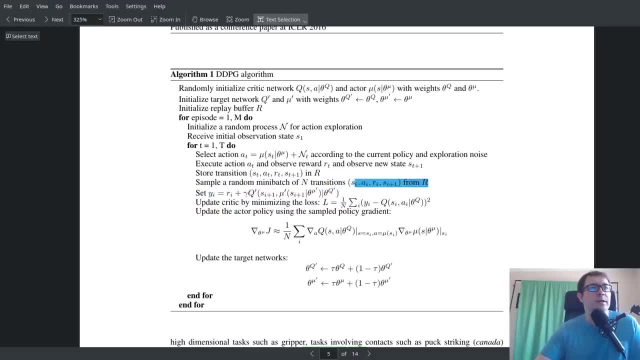 want to use that set of transitions to set y sub i equals. so i is sorry having difficulties here. so i is each step of that, uh, is each element of that mini batch of transitions. so you want to basically loop over that set or do a vectorized implementation. looping is more. 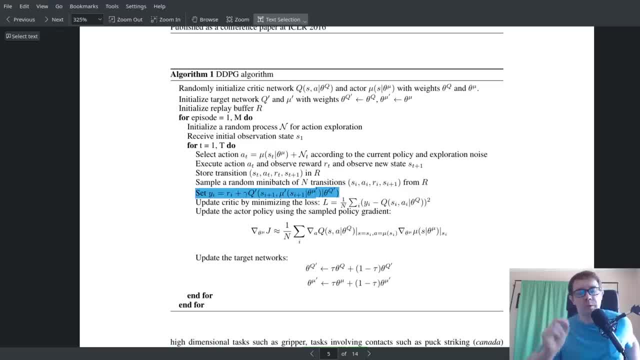 straightforward. that's what i do. i always opt for the most straightforward and not necessarily most efficient way of doing things the first time through, because you want to get it working first and worry about implementation- uh sorry, efficiency later. so set y sub i equals r sub i. 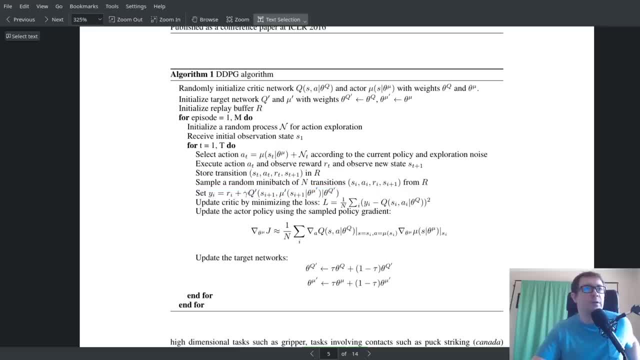 plus gamma, where gamma is your uh discount factor, times q prime of the new state s sub i plus one uh times uh, where the action is chosen according to mu prime. uh, given some weights: theta super mu prime and theta super q prime. so, uh, what's important here is that, and this isn't immediately, 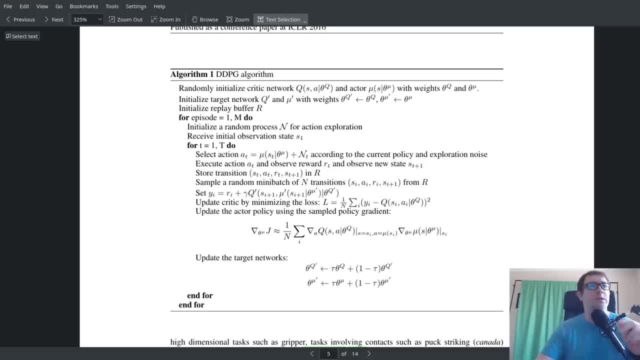 clear, if you're reading this for the first time, what's? this is a very important detail. so it's the action. uh must be chosen according to the target actor network, so you actually have q as a function of the state as well as the output- excuse me- of another network. that's very important update. 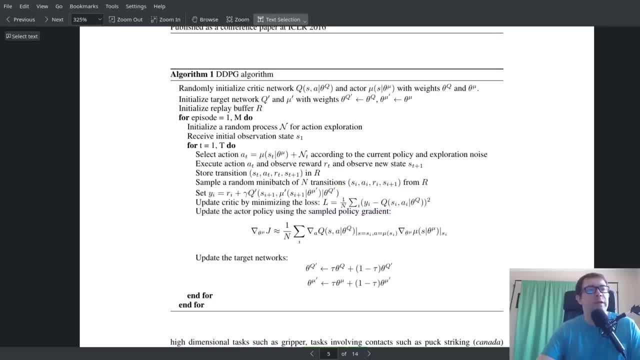 the critic by minimizing the loss. uh, basically a weighted average of that y sub i minus the output from the actual q network, where the a sub i's are from the actual q network. so that's actually the actions you actually took during the course of the episode. so this a sub i is from. 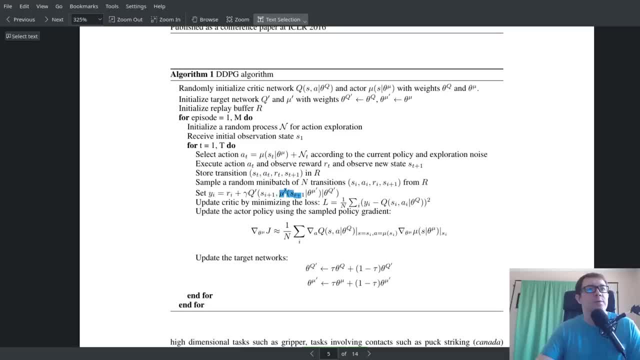 the replay buffer and these actions right are chosen according to the target actor network. so for each learning step you're going to have to do a feed forward pass of not just this target q network but also the target actor network as well as the evaluation critic network, i hope. i. 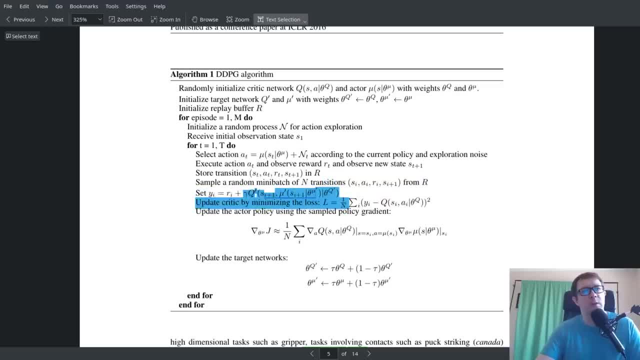 said that, right. so the feed forward pass of the target critic network as well as the target actor network and the evaluation critic network as well, and then it says: update the actor policy using the sample policy gradient. this is the hardest step in the whole thing. this is the most confusing part. so this is the gradient. 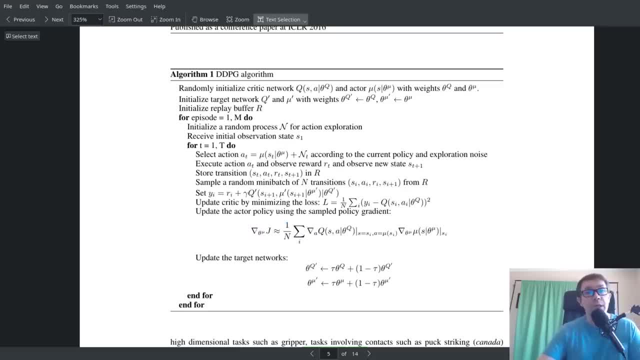 is equal to one over n times the sum, so a a mean. basically, whenever you see one over n times the sum, that's a mean. the gradient with respect to actions of q? uh, where the actions are chosen according to the policy mu of the current states s times. a gradient with respect to the weights of mu? uh, where the you. 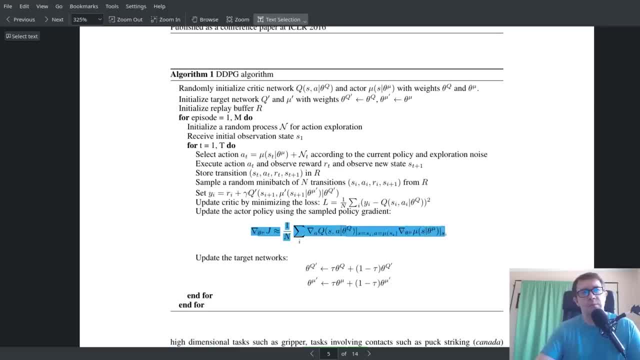 just input the set of states, okay, so that'll be a little bit tricky to implement. so- and this is part of the reason i chose tensorflow for this particular video- is because tensorflow allows us to calculate gradients explicitly. uh, in pytorch, you may have noticed that all i did was uh set q. 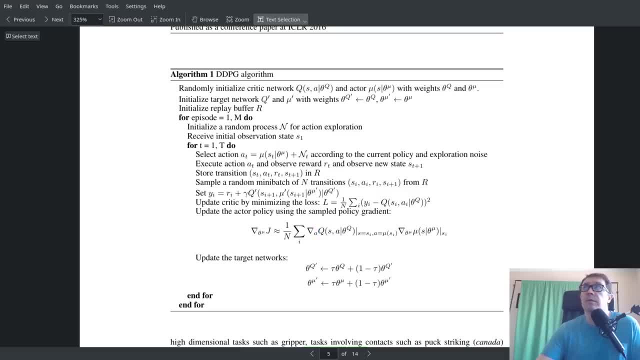 to be a function of the um, the current state as well as the network, and so i allowed pytorch to handle the chain rule. this is effectively a chain rule, so let's, let's scroll up a little bit to look at that, because this kind of gave me pause. the first 10: 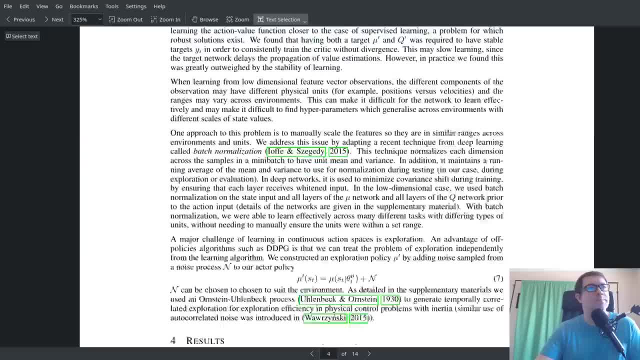 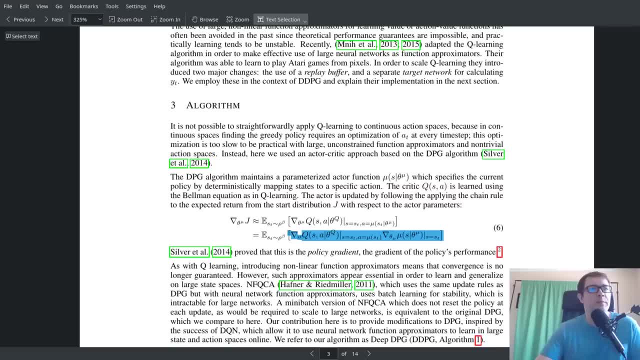 times. i read it so, uh, this is the hardest part to implement. if you scroll up, you see that this exact same expression appears here, right, and this is in reference to this. so it's a gradient with respect to the weights, theta, super mu of q, of s and a, uh, such that you can see that this is the gradient. 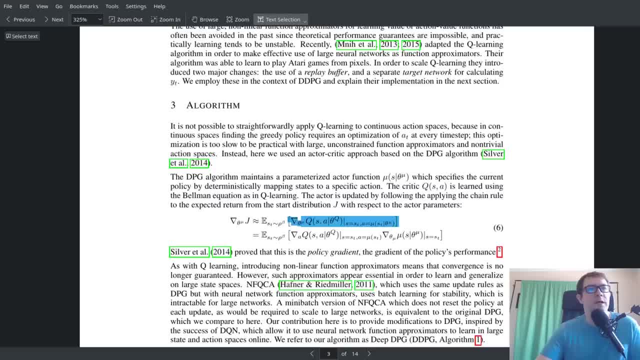 of q of s and a, such that you can see that this is the gradient of q of s and a, such that you can. you're choosing an action a according to the policy mu. so, really, what this is is the chain rule. so it's the uh. this gradient is proportional to a gradient of this quantity times the gradient. 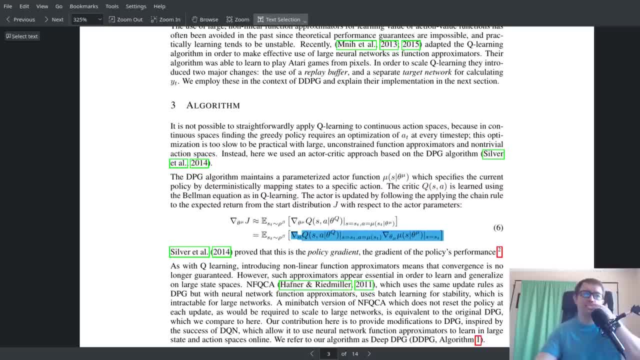 of the other quantity. it's just a chain rule from calculus. so, um, in the in the pytorch paper we implemented this version and these are. these are equivalent. it's perfectly valid to do one or the other. so in pytorch we did this version. today we're going to do this particular version. 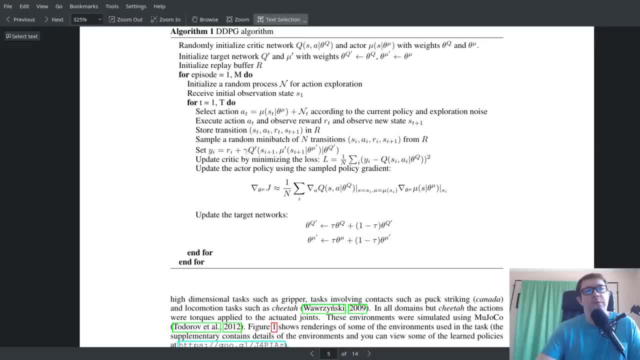 so that's good to know. all right. so next step: on each time step, you want to update the target networks according to this soft update rule. so theta super q prime gets updated as tau times theta super q plus one minus tau theta super q prime, and likewise for theta super mu prime. 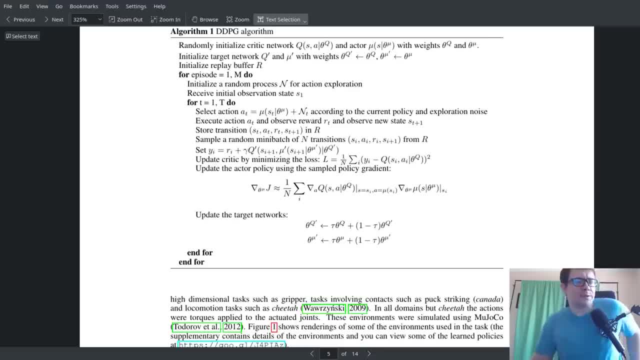 and then just end the two loops. so in practice, this looks very, very simple, but what do we know off the bat? we need a class for our replay network, we need a class for our noise process, we need a class for the actor and a class for the critic. now you could think. 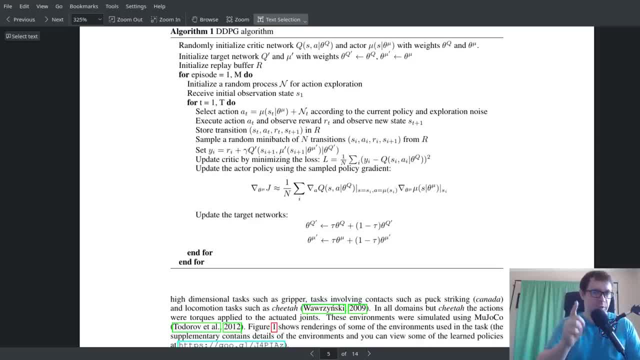 that perhaps they're the same. but when you look at the details, which we're going to get to in a minute, you realize you need two separate classes. so you need at least one class to handle the deep neural networks. so you have at least three classes, and i always add in an agent class on top as kind. 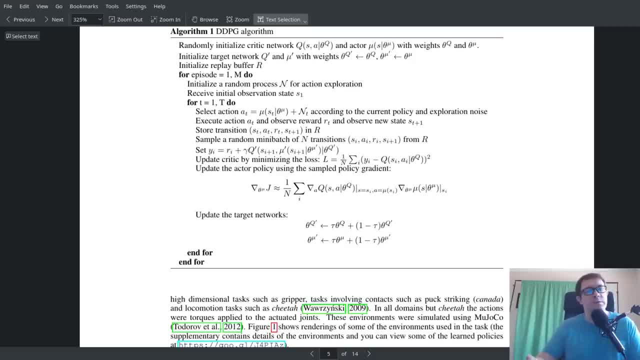 of an interface between the environment and the deep neural networks. so that's four, and we're gonna end up with five, but that's four right off the bat. so now we know the algorithm. let's take a look at the supplemental details- uh, supplemental information to see precisely the architectures. 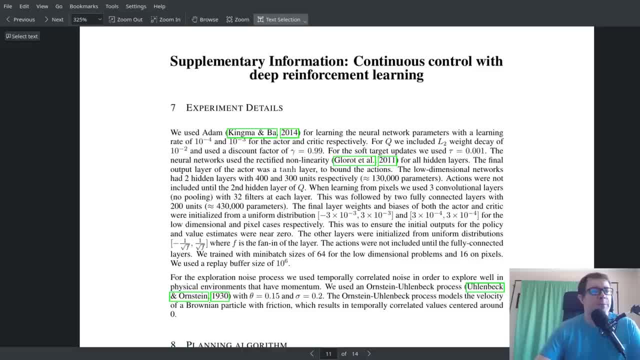 and parameters used. so we scroll down. so here are the experimental details. uh, these atom for learning, the neural network parameters, with a learning rate of 10 to the minus 4 and 10 to the minus 3 for the actor and critic respectively. so they tell us the learning rates 10 to the minus. 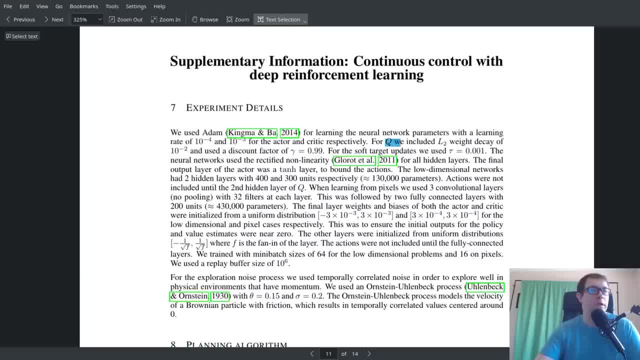 4: 10 to the minus 3 for actor critic. for q the critic. we included l2 weight decay of 10 to the minus 2 and use a discount factor of 10 to the minus 2 and we're going to use a discount factor. 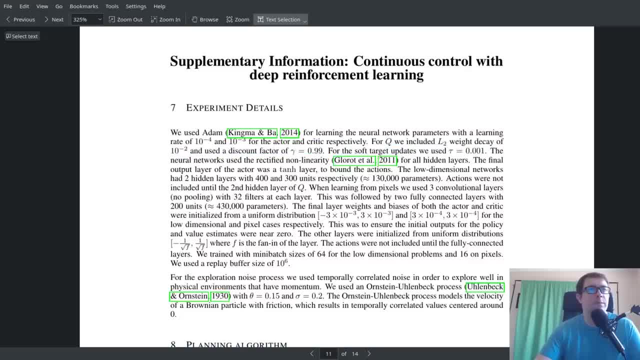 of gamma 0.99, so that gamma is pretty typical. but this important thing is that for q- and only q, not mu- we included l2 weight decay of 10 to the minus 2. use a discount factor of gamma of 0.99. that's an. 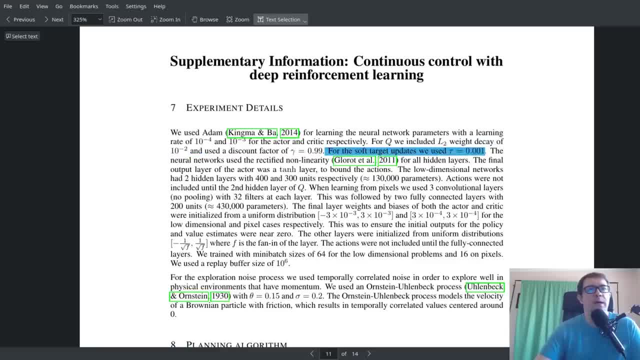 important detail for the soft target updates we use. tau equals 0.001, so one part in a thousand. that is indeed very, very small. okay, fine, the neural networks use the rectified non-linearity for all hidden layers. okay, the final output layer of the actor was a tangent hyperbolic layer to bound the actions now. 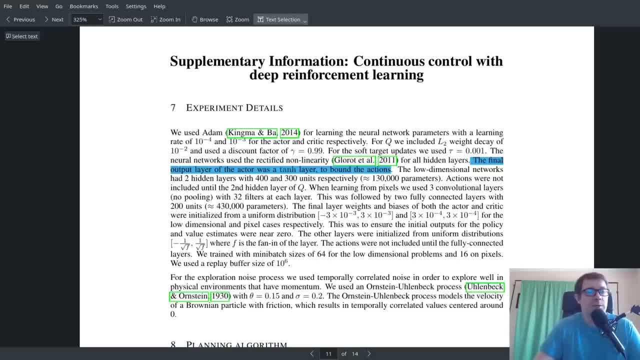 tan hyperbolic goes from minus 1 to plus 1. so in environments in which you have bounds of plus or minus 2, let's say, you're going to need a multiplicative factor. so that's just something to keep in mind. the low dimensional networks: 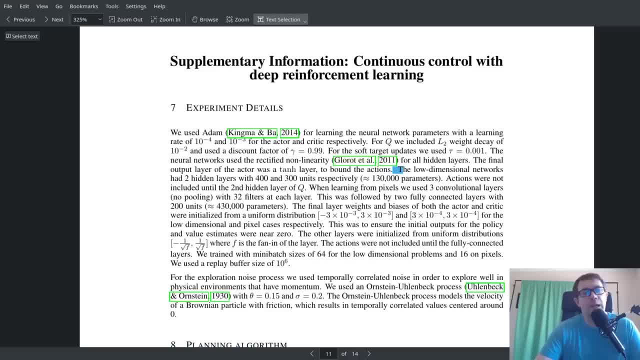 but that doesn't um, that doesn't impact the tangent hyperbolic, it just means there's a multiplicative factor and they're related to your environment. the low dimensional networks had two hidden layers with 400 and 300 units respectively, about 130 000 parameters. actions were not included until the second hidden layer of q. 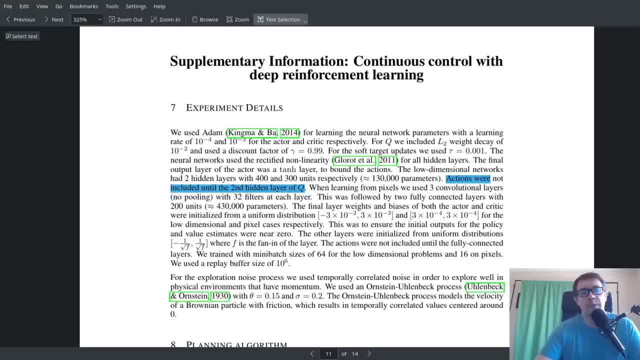 so when you're calculating the critic function q, you aren't actually passing forward the action from the very beginning. you're including it as a separate input at the second hidden layer of q. that's very important. that's a very important point and that's why we're going to talk about. 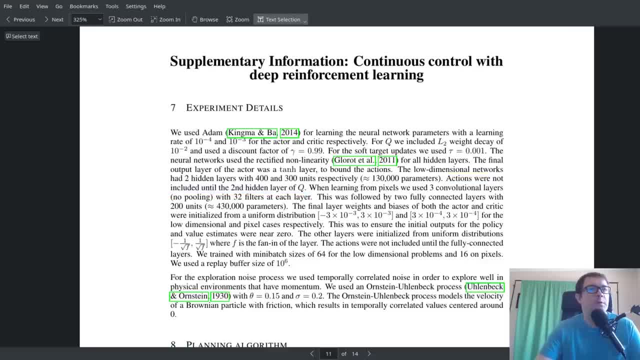 it in a little bit more detail, in a little bit more detail, in a little bit more detail, and this is when learning from pixels. we use three convolution layers- which we don't need to know right now- we're not using pixels yet- and followed by two fully connected layers. 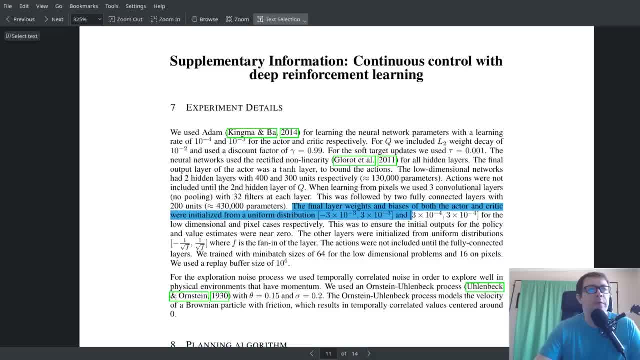 the final layer, weights and biases of both the actor and critic were initialized from a uniform distribution of plus or minus 3 by 10 to the minus 3 for the low dimensional case this was. this was to ensure that the initial outputs for the policy and value estimates were. 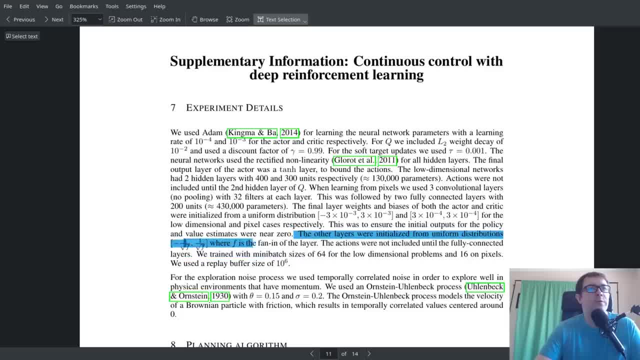 near zero. the other layers were initialized from uniform distribution of plus or minus 1 over square root of f, where f is the fan end of the layer. fan end is just the number of input units and the other layer- oh, i already read that- the um, the. 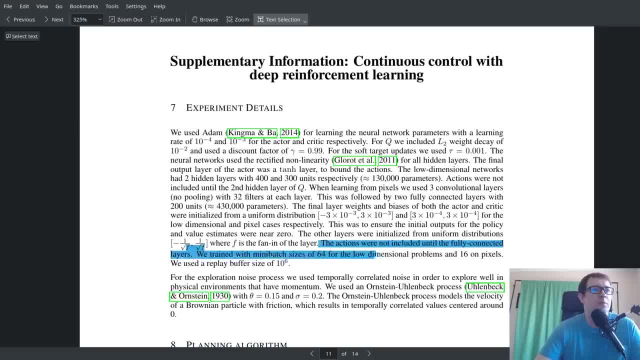 the actions were not included into the fully connected layers. that's for the convolutional uh case. so here right now, i'm experiencing some confusion reading this. so, um, it says the other layers were initialized from uniform distributions related to the fan end. the actions were not included into the fully connected layers, so i'm guessing, since they're. 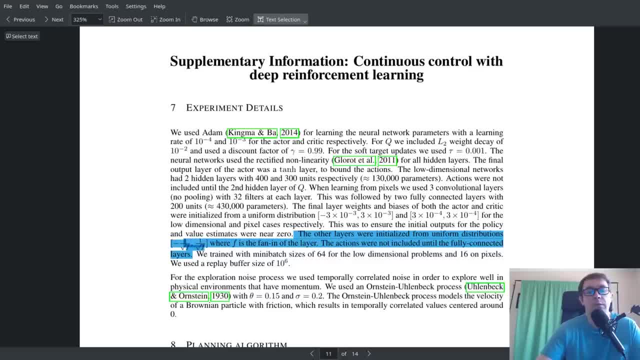 talking about fully connected layers. they're talking about the pixel case, right, because otherwise they're all fully connected. you know, wouldn't make sense to say specify fully connected layers, uh, so this gives me a little bit of confusion. is this statement referring to the way i initially interpreted it? uh, it is referring to both cases for the state vector. 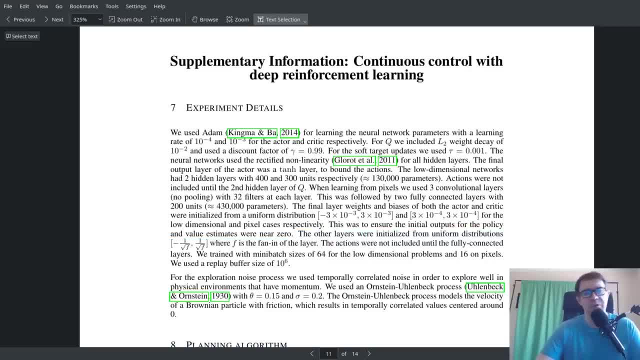 and pixel case. but whatever, i'm going to interpret it that way because it seemed to work. but there's ambiguity there and this is kind of an example of how reading papers can be a little bit confusing at times because the wording isn't always clear. maybe i'm just tired, maybe i've been. 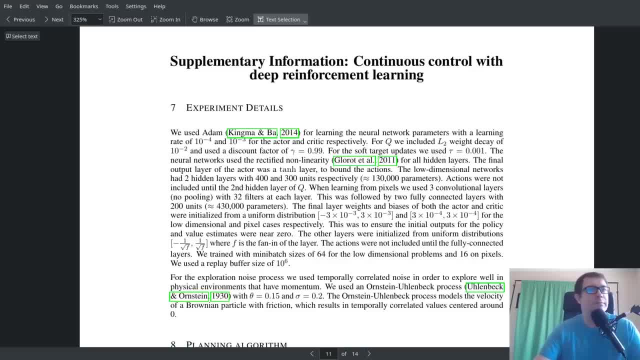 rambling for about 50 minutes and, uh, my brain's turning to mush. that's quite probable, actually, but anyway. we trained with mini match sizes- of 64 for the low dimensional problems and 16 on pixels, with a replay buffer of 10 to the 6th. 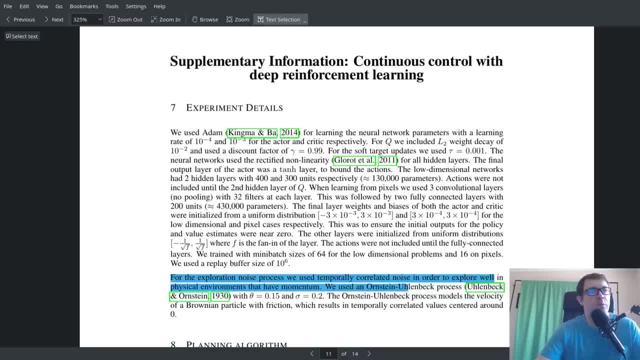 for the exploration noise process. we use temporally correlated noise in order to explore well in physical environments that add momentum or unseen. uhlenbeck process with theta equals 0.15 and sigma equals 0.2, and it tells you what it does. all well and good. okay, so these are the implementation. 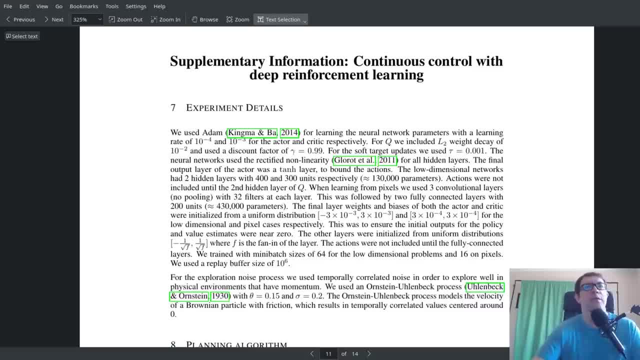 details: we need 400 units and 300 units for our hidden layers. atom optimizer: 10 to the minus 4 for the actor, 10 to the minus 3 for the critic. for the critic, we need an l2 weight decay of 10 to the. 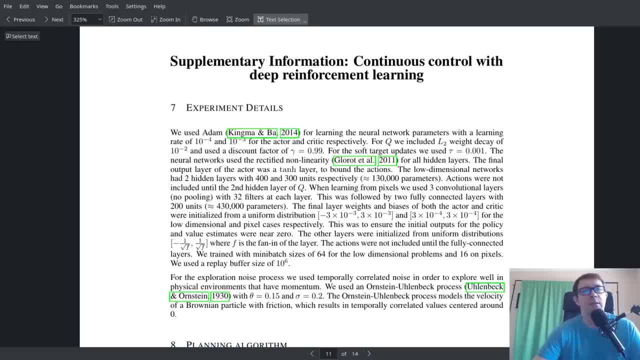 minus 2 discount factor of gamma 0.99 and for the soft update factor we need an l2 weight decay of 0.001 and we need updates. uh, we need initializations that are proportional to the one over the square root of fanon for the lower layers and plus minus 0.003. uh, 0, 0, yeah, 0 0, 3 for. 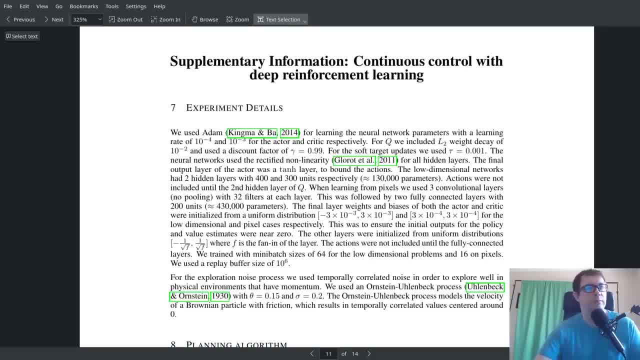 the final output layers of our fully connected networks. okay, so that's a lot of details. we have everything we need to start implementing the paper. uh, and that only took us about 50 minutes, um, which is much shorter than when i read. it took me quite a while, so, uh, let's head back up to the 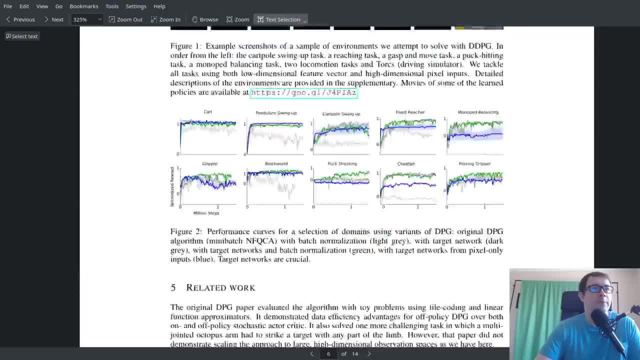 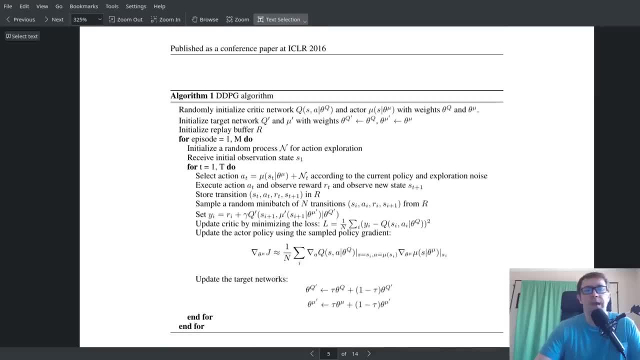 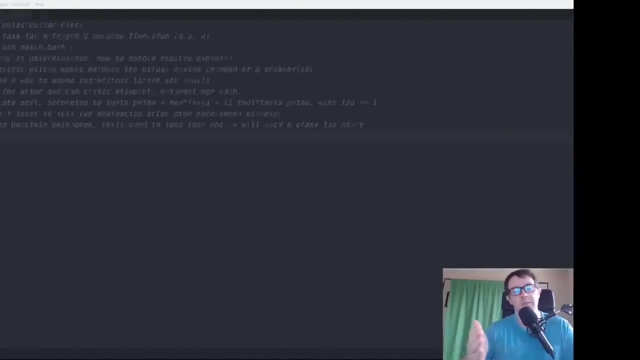 algorithm here, and we'll keep that up as reference for the remainder of the video, because that's quite critical. so, um, let's go ahead and head back to our uh code editor and start coding this up. we'll start with the easy stuff first. so let's start coding and we will start with the probably. 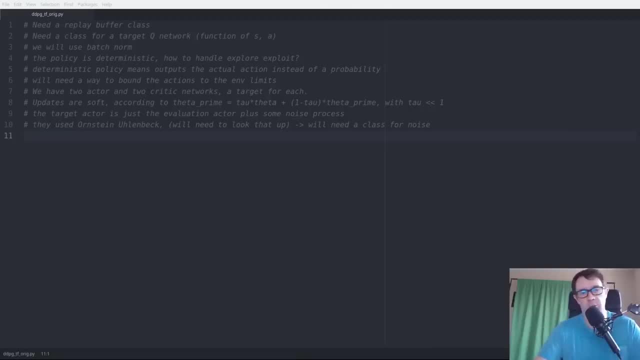 one of the most confusing aspects of the problem with the orenstein uhlenbeck action noise. now you can go ahead and do a google search for it and you'll find a wikipedia article that talks a lot about the physical processes behind a lot of mathematical derivations. 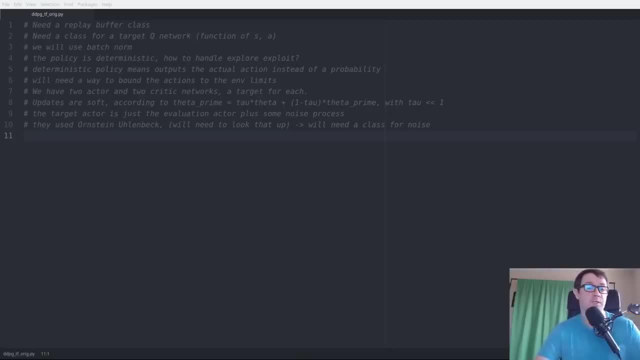 and that's not particularly helpful. so if you want to be a physicist, i invite you to read that and check it out. it's got some pretty cool stuff. it took me back to my grad school days, but we have a different mission in mind for the moment. the mission now is to find a code implementation. 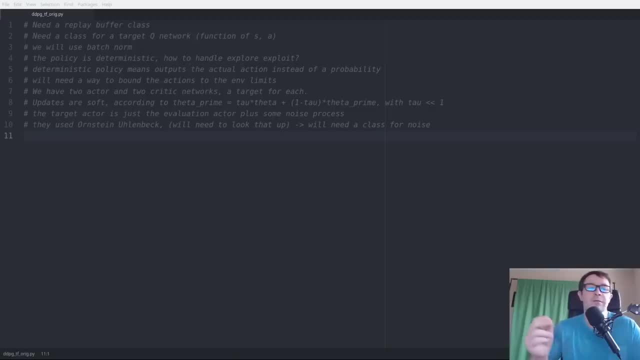 of this that we can use in our problem. so if you then do a google search for orenstein olenbeck github, as in you want to find someone's github example for it, you end up with a nice example from the orenstein olenbeck action noise and you'll find a nice example from the orenstein olenbeck. 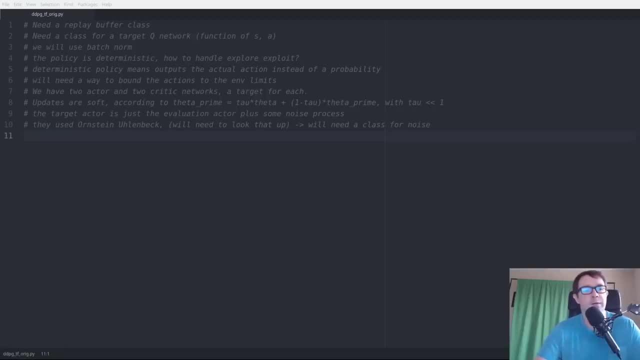 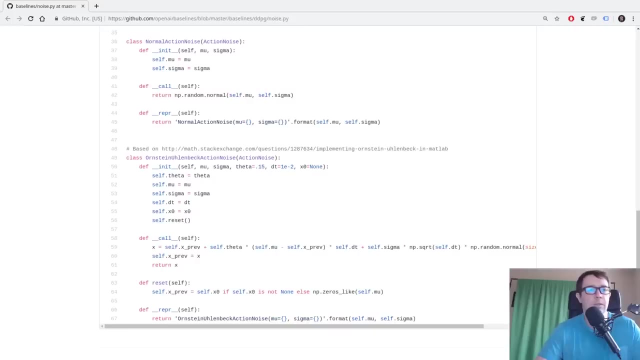 example from the orenstein olenbeck action noise. and you'll find a nice example from the orenstein olenbeck, the open ai baseline library. that shows you the precise form of it. so let me show you that one second so you can see it here. uh, in the in the github, uh, there is a whole class for this right. 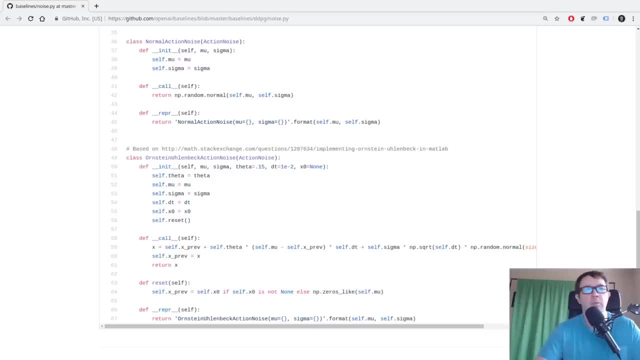 here that i've highlighted. uh, and this looks to do precisely what we want. it has a previous plus a delta term and a dt term, so it looks like it's going to create correlations through this x previous term. there's a reset function to reset the noise, which we may 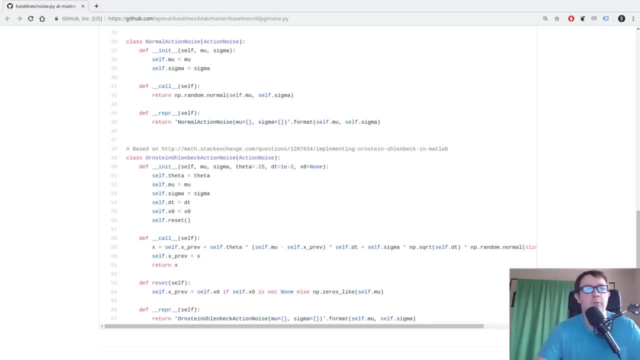 want to use. uh, and there's this representation, which we'll probably skip because we know what we're doing and it's not really critical for this particular application, though it would be nice if you were writing a library, as these guys were. so they included the representation method. so 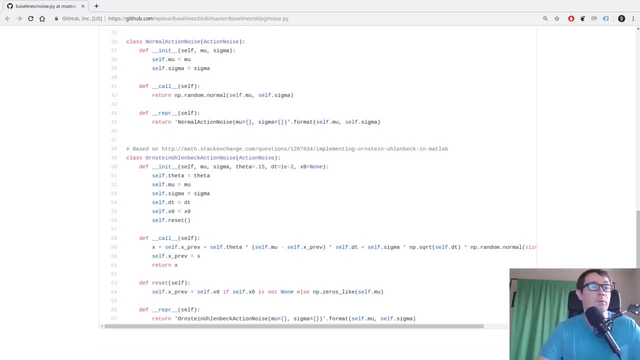 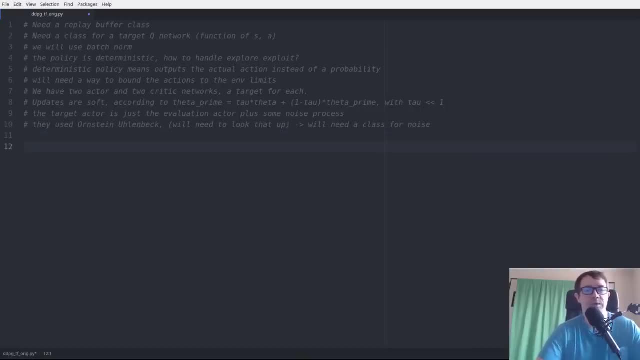 so let's go ahead and code that up in the editor and that will tackle our first class. so i'm going to leave the notes up there for now. they do no harm. they're just comments at the top of the file. so the first thing we'll need is to import: numpy is. 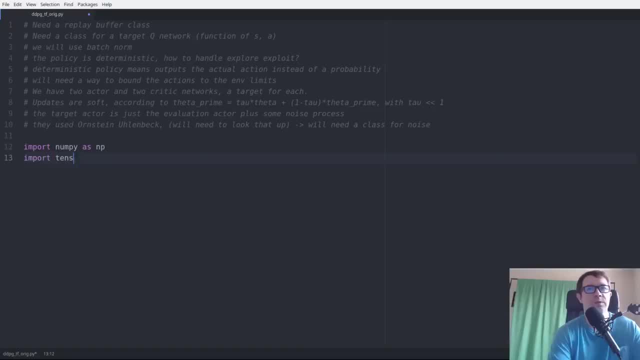 uh, we know, we can go ahead and start and say: import tensorflow, stf, we're going to need tensorflow, um, we may need something like os to handle model saving, so we can go ahead and import that as well. just a fun fact: it is considered good practice to. 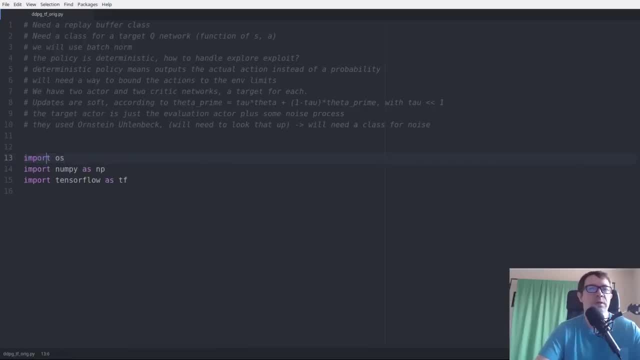 import your system level packages first and followed by your library packages second, in numerical order, followed by your own personal code in numerical order. um, so that's the imports that we need. to start, let's go ahead and code up our class. we'll call it ou action noise, and that'll just be derived from the base object. so the initializer will. 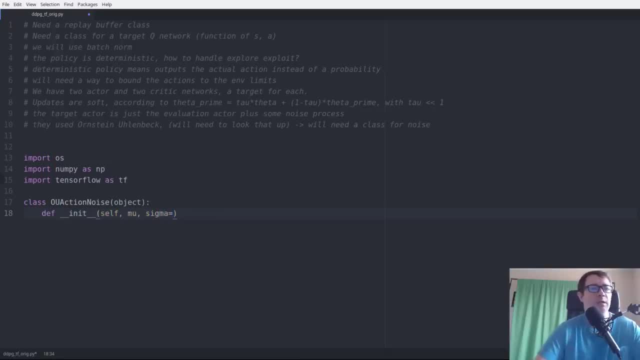 take a mu, a sigma. now they said they used a default value of, i believe, 0.15 and a theta of 0.2, a dt term something like 1 by 10 to the minus 2 and our x naught. we'll save as none. and again, if you have any doubts on 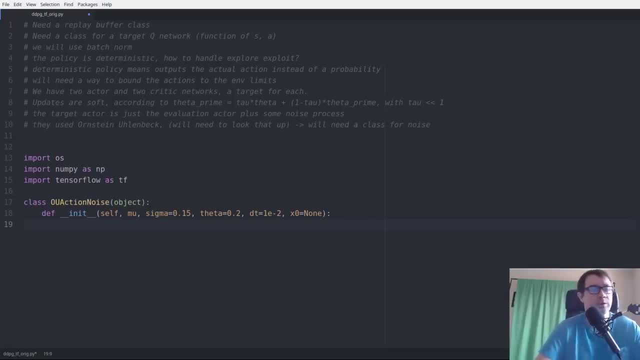 that. just go check out the open ai baselines for it. their implementation is probably correct, right? i'll give them the benefit of the doubt, so go ahead and save your parameters as usual. so we have a mu, a theta, a dt, a sigma and x- 0, and we'll go ahead and call the reset function at the top. now they override the call. 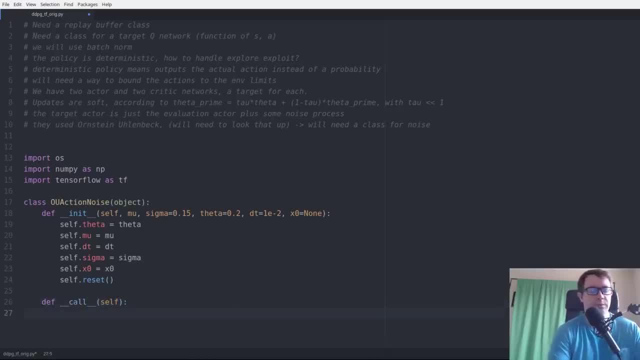 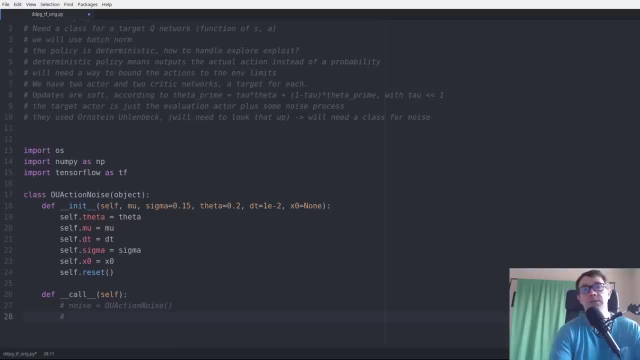 method and what this does is it enables you to say noise equals ou action noise, and then, when you want to get the noise, you just say our noise equals noise. you can use the parentheses. that's what overall writing call does. that's a good little notification if you get the noise, and then what? 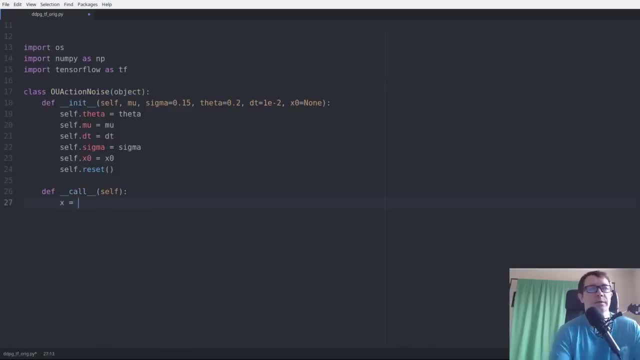 you do is you want to call the reset function the reset function over here and then, when you do that tidbit, to know. so we want to implement the equation that they gave us. it's L, self, dot, X previous plus self, dot. theta times mu minus X previous times self. 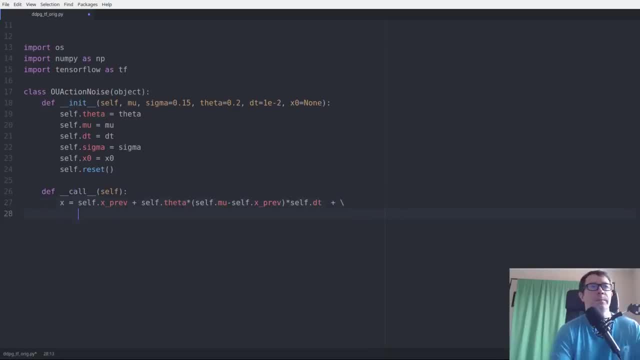 dot DT plus Sigma times numpy dot square root self dot DT times numpy random normal for the size of mu and set the X previous to the current value. that's how you create the temporal correlations and return the value of the noise. so we don't have a value for X previous, so we have to set that with the reset. 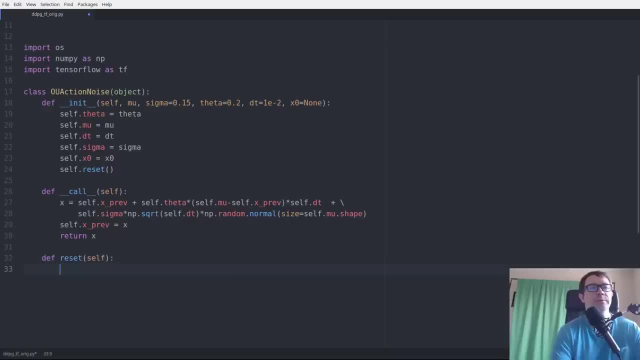 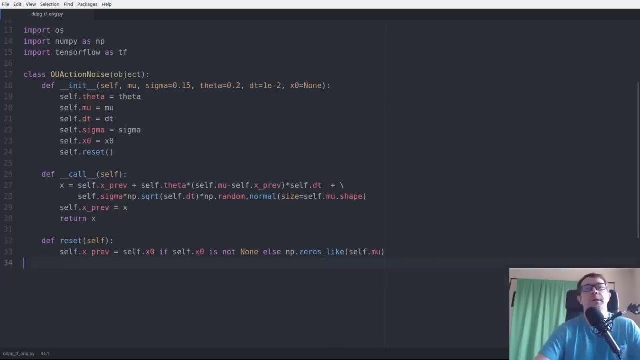 function which takes no parameters, so that X previous equals X, not if self dot X, no is not, none else numpy zeros like selfmute. and that's it for the noise function. that's pretty straightforward, so that's all well and good. so we have one, one function down, so we've taken care of. 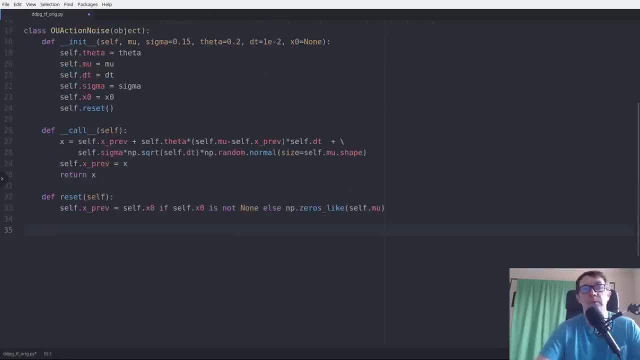 the noise. sorry, one class. now we've taken care of the noise and now we can move on to the replay buffer, so this will be something similar to what i've implemented in the past. there are many different implementations and ways of implementing this. many people will use a built-in python data. 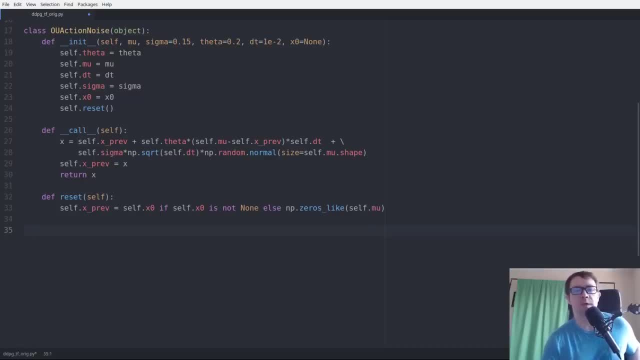 structure called a dq or a deck. i think it's dq is the pronunciation. basically it's a q that you fill up over time and that's perfectly valid. you can do that. there's no reason not to. i prefer using a set of arrays and using numpy to facilitate that, the reason being that we can tightly control. 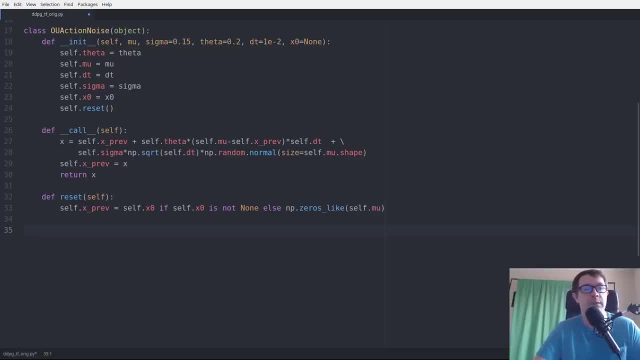 the data types of the stuff that we're saving for this pendulum environment it doesn't really matter. but as you get more involved in this field you will see that you are saving stuff that has varying sizes. so if you're trying to save images, let's say, from the one of the atari libraries or a mujoko. 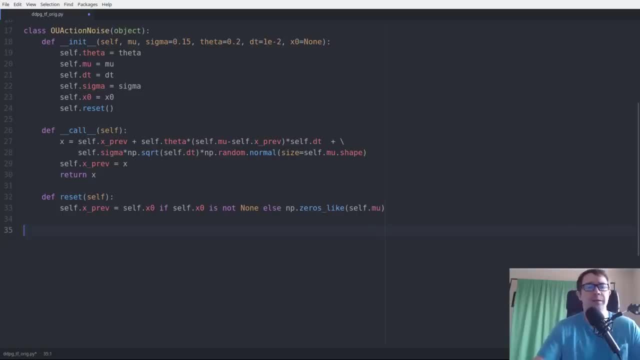 environment or something like that. i hope i pronounced that correctly. uh, you'll see that this memory can explode quite quickly. you can eat into your ram. so the ability to manipulate the information- whether you want to use single or double precision for either your floating point numbers or your integers- is critical to memory management. as well as taking advantage of some 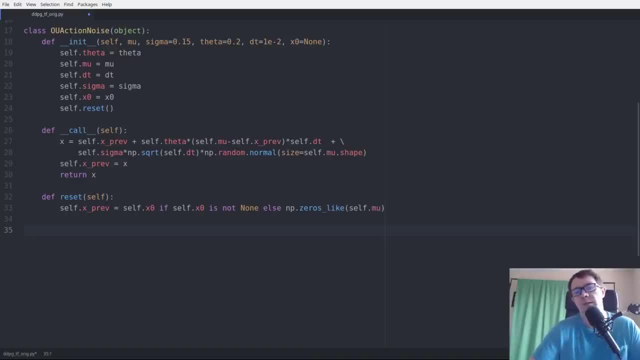 other optimizations for nvidia gpus in the touring class and above. so i always use the numpy arrays because it's a clean implementation that allows manipulation of data types. you can use the dq if you want. it's perfectly valid. so our separate class has its own initializer. 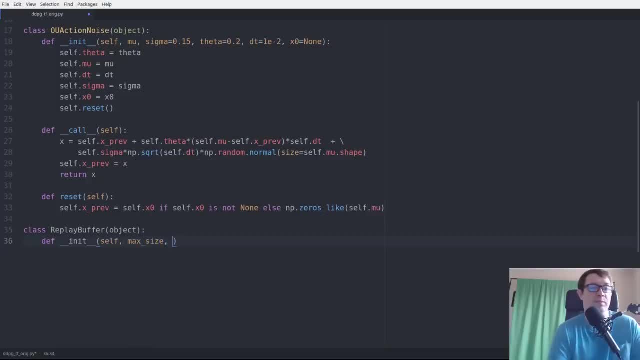 of course. so we're going to want to pass in a maximum size the input shape and the number of actions right, because we have to store the state action reward and new state tuples. we're also going to want to facilitate the use of the done flag, so we'll have an extra parameter in here. 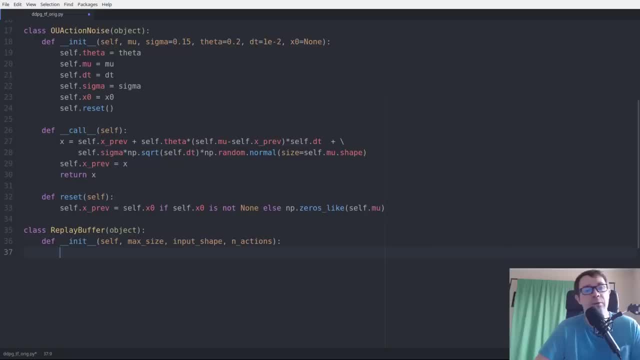 and the reason behind that is intimately related to how the, uh, how the bellman equation is calculated. it took me a second to think of that, uh, at the end of the episode. the agent received no further rewards, and so the expected feature reward, the discounted feature reward, if you will. 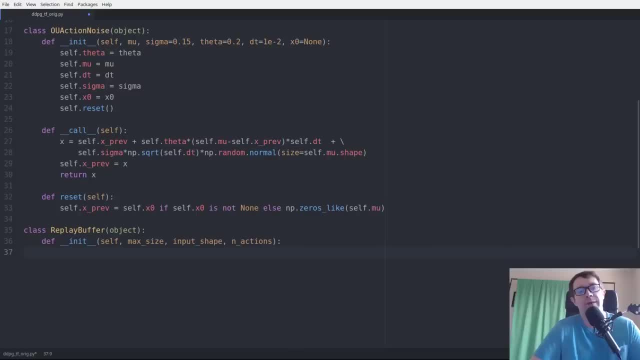 is identically zero. so you have to multiply the uh reward for the next state by zero if that next state follows the terminal state, if your current state is terminal and the next state is following the terminal state, so you don't want to take into account anything from that. the expected future. 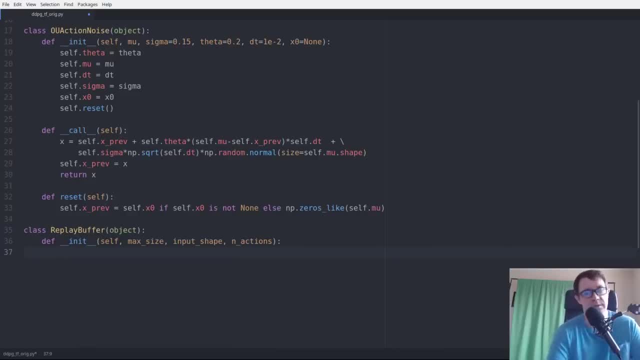 rewards because they're identically zero. so we need a done flag, is all i wanted to say. uh, so we save our parameters? um, uh, yeah, we don't even need to say that. we can say selfmem: counter equals zero and that'll keep track of the position of our most recently saved memory state memory, an array of numpy zeros. 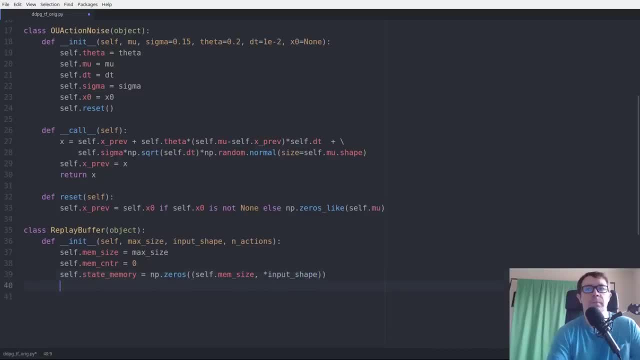 mem size by input shape. uh, new state memory- same same deal. you know, it's just just totally the same, good grief. okay, so now we have the say action memory, and that's numpy zeros. selfmem size by selfn actions. uh, we didn't save inactions, did we? so we'll just call it inactions. 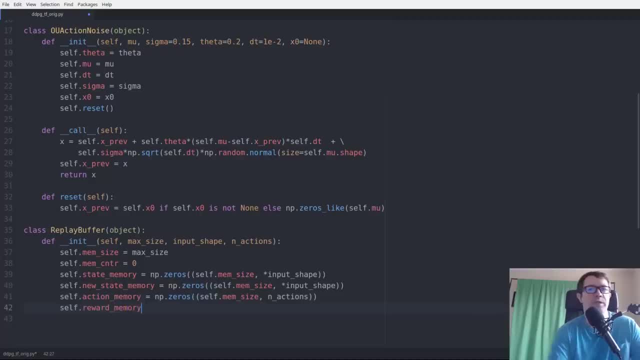 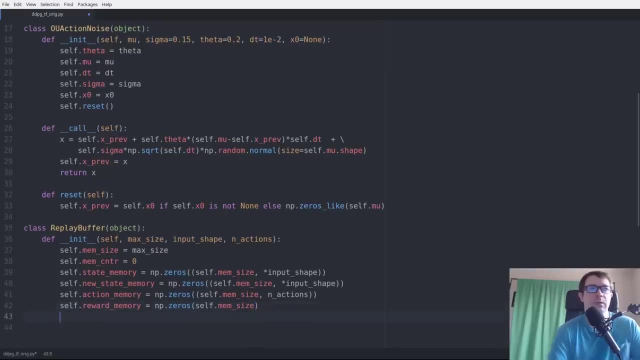 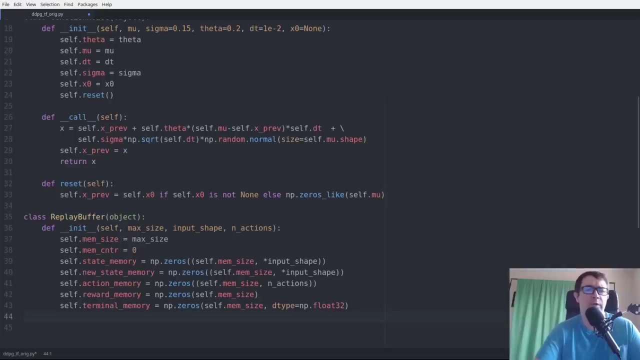 we have the reward memory and that's just a scalar value so that only gets shape self mem size. we also need the terminal memory, terminal memory and that'll be shape selfmen size and i have a numpy flow: 32 if i recall correctly. that is due to the data types in the pytorch. 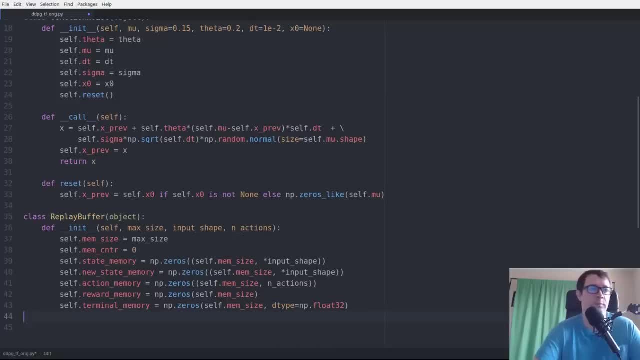 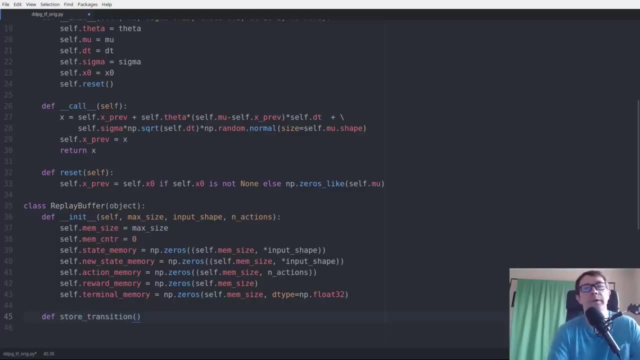 implementation is probably not necessary here in the tensorflow implementation, but i left it the same way just to be consistent. it doesn't hurt anything. so next we need a function to store a current transition, so that'll take a state, action, reward, new state and a done flag as input, so the index of where we want to store that memory. 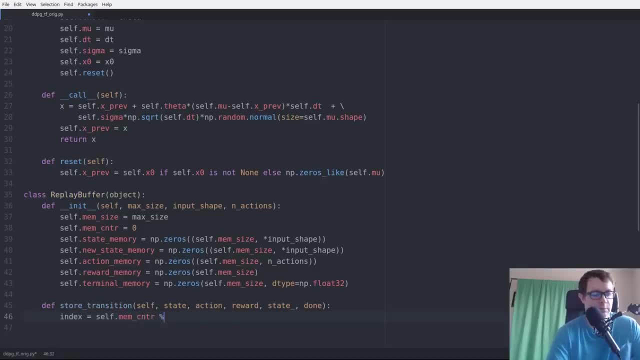 is the memory counter modulus the mem size. so for any mem counter less than mem size, this just returns mem counter. um, for anything larger than mem size, it just wraps around. so if you have a million memories, all the way up from zero to nine hundred ninety thousand 999, it will be a number of. 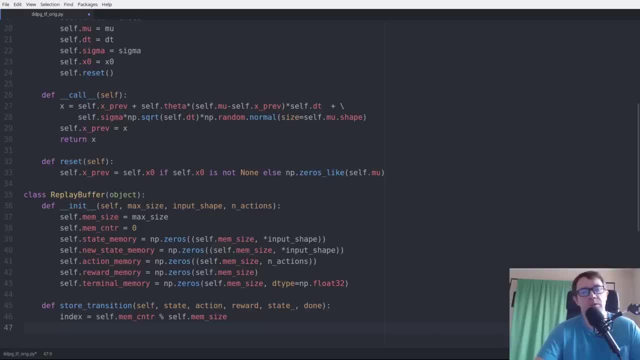 uh, that number, and then once it's a million, it wraps background to zero, and then one and two and so on and so forth, and so that way you're overriding memories at the earliest part of the array with the newest memories, precisely as they describe in the paper, if you're using the dq. 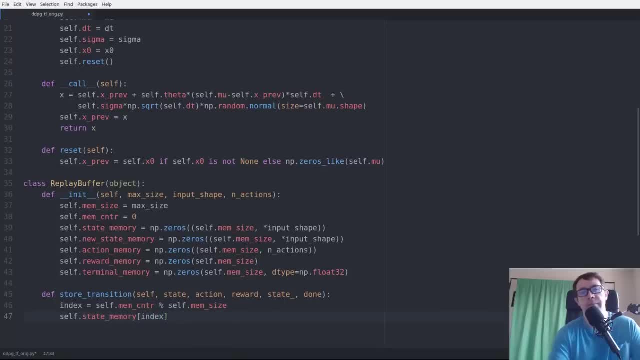 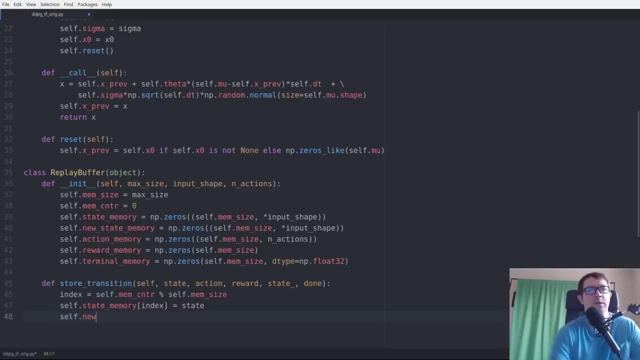 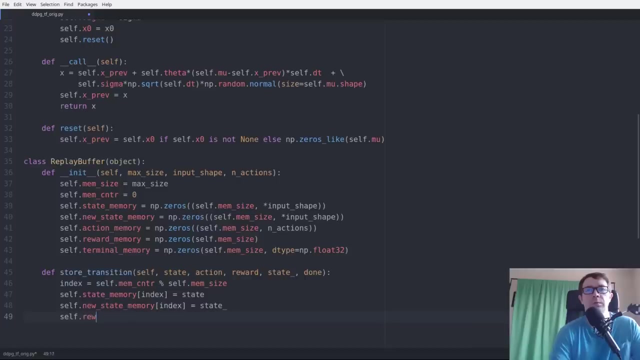 method, then i believe you would just pop it off of the left, i believe. now don't quote me because i haven't really used that implementation, but from what i've read, that's how it operates. new state memory subindex equals state underscore. reward memory equals subindex. 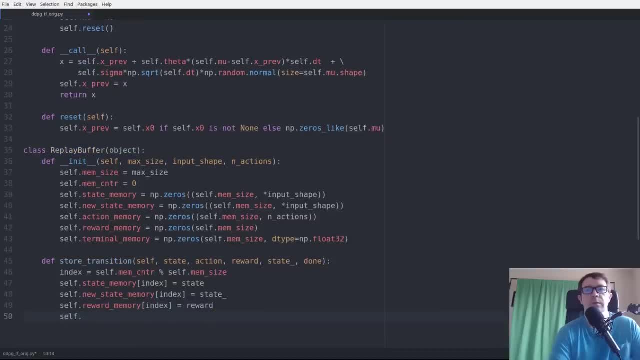 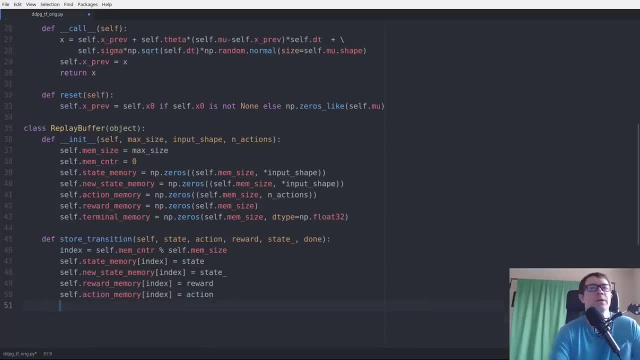 is reward as action memory. now keep in mind that the actions in this case are arrays themselves, so it's an array of arrays. just keep that in the back of your mind so that you can visualize the problem we're trying to solve here. you next up, we have the terminal memory. now a little twist here is that we want this to be. 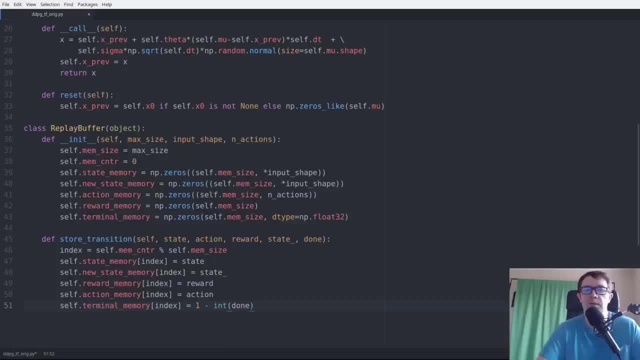 one minus int of done. so done is either true or false, so you don't want to count the rewards after the episode has ended. so when done is true, you want to multiply by zero. so one minus int of true is one minus one, which is zero, and when it's not over, it's one minus zero, which is. 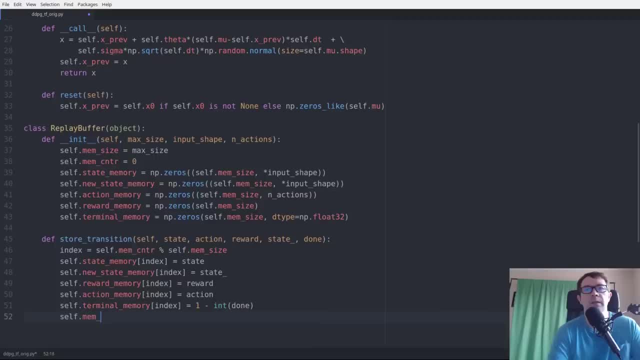 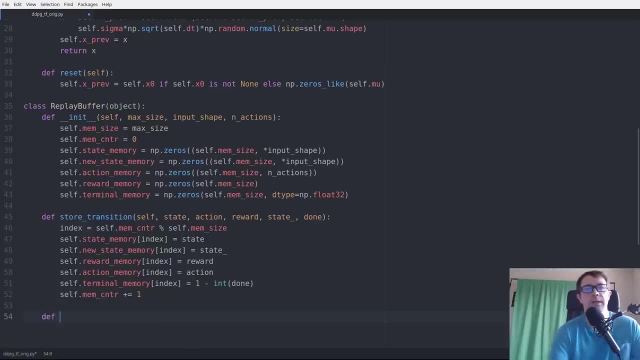 just one. so it's precisely the behavior we want. and finally, you want to increment memcounter by one every time you store mnu memory. next, we need a function to sample our buffer and we want to pass in a batch size. alternatively, you could make batch size a member variable of this class. it's not really a big deal. 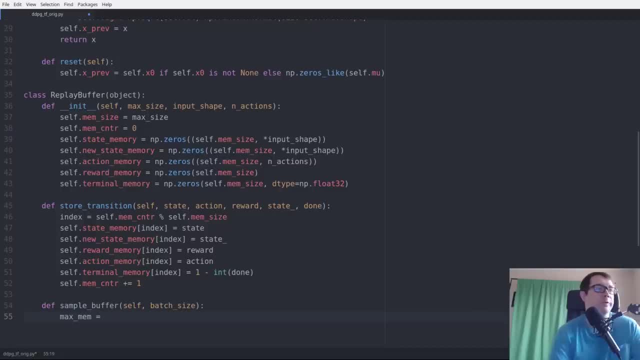 i just did it this way. for whatever reason, i chose to do it that way. so what we want to do is we want to find the minimum either. so let's back up for a second. so what we want is to sample the memories from either the zero. 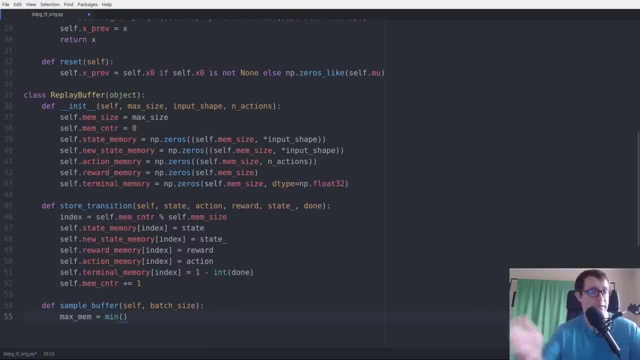 position all the way up to the most filled memory, the last filled memory. so if you have less than the max memory, you want to go from zero to mem counter, otherwise you want to sample anywhere in that whole interval. so max mem equals the minimum of either mem counter or mem size. and the reason 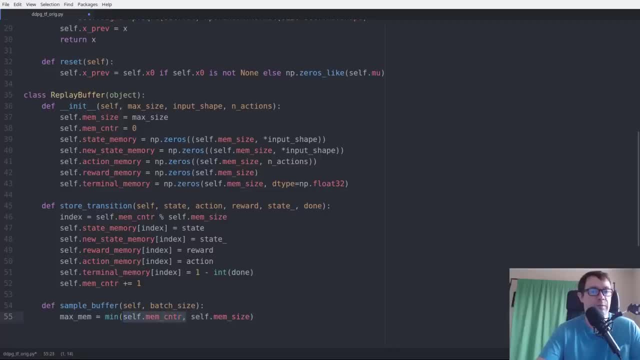 you don't want to just use mem counter is that mem counter goes larger than mem size. so if you try to tell it to select something from the range mem counter when mem counter is greater than mem size, you'll end up trying to access elements of the array that aren't there, and it'll 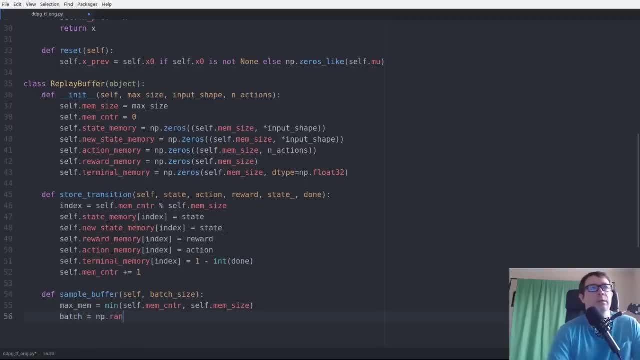 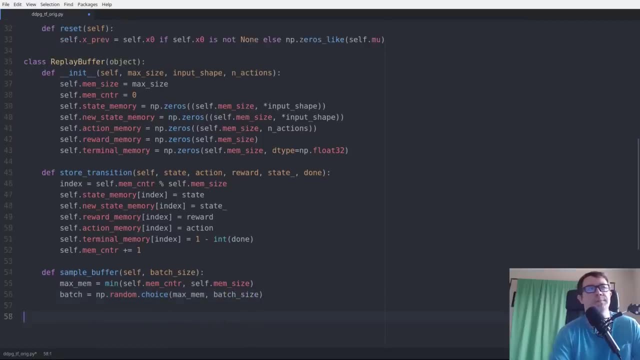 throw an error. so that's why you need this step. next, you want to take a random choice from zero to max mem of size, batch size. so then you just want to gather those states from the range of the mem counter and then you want to select the space version that you want to. 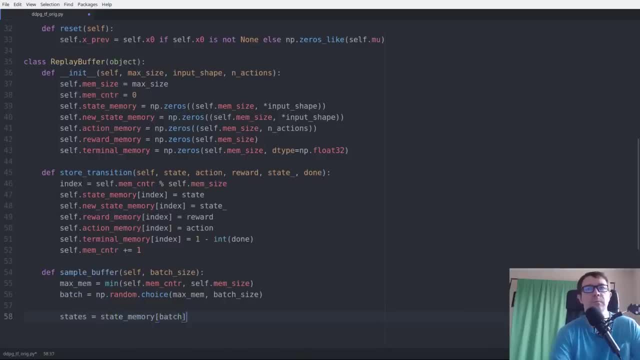 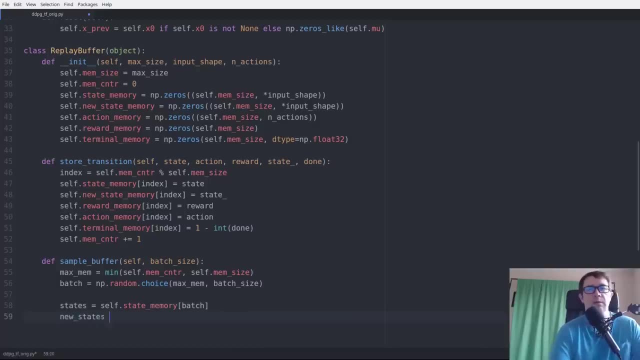 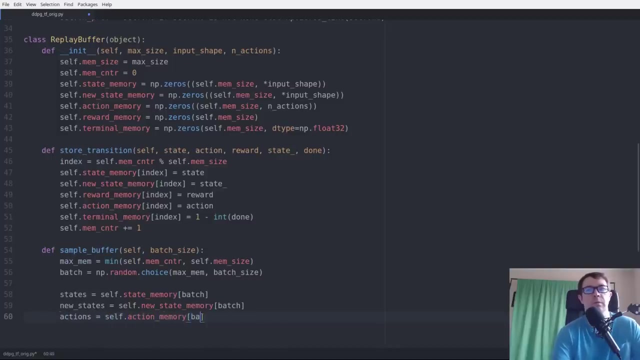 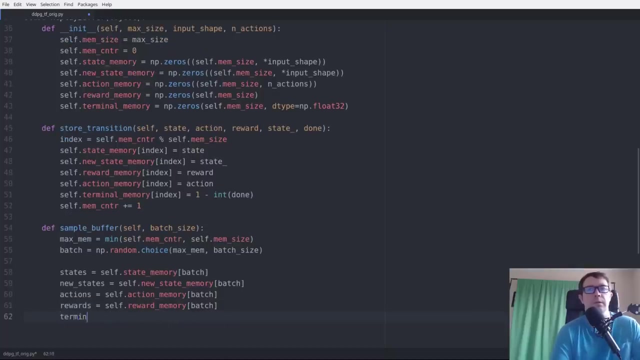 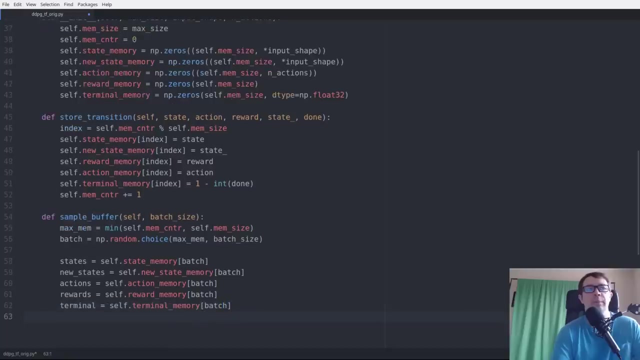 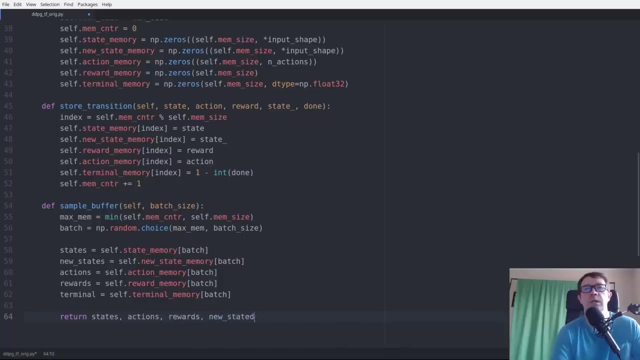 the appreciation of the mem counter and the size of the mesh block isn't going to change. so you're like respective arrays, like, so I forgot the self, of course- new states, actions, rewards and terminal batch. I believe that's everything And you want to return the states, actions, rewards, new states and. 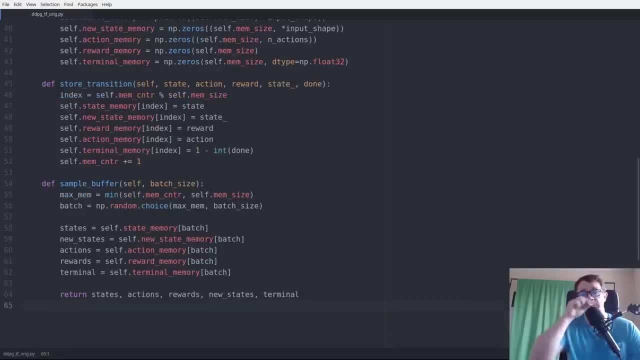 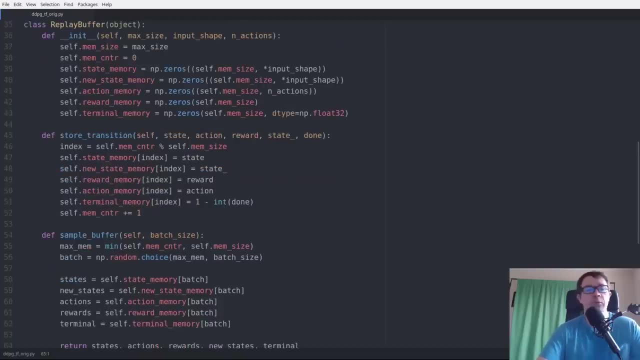 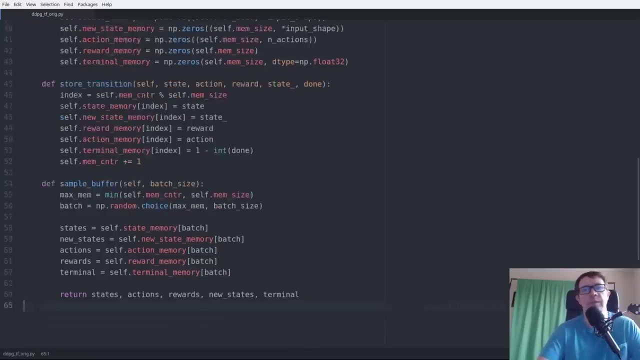 terminal. Okay, so now we are done with the replay buffer class. So that's actually pretty straightforward And if you've seen some of my other videos on deep Q learning then you've seen pretty much the same movement implementation. I just typically kept it in the agent class. then we're kind of refining my approach, getting more. 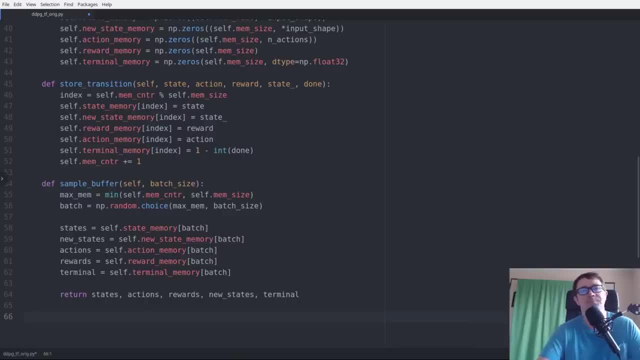 sophisticated over time, So it makes sense to stick it in its own class. So we're already like 40% of the way there. we got five classes in total, So that's good news. So next up, we have to contend with the actor and critic networks. So 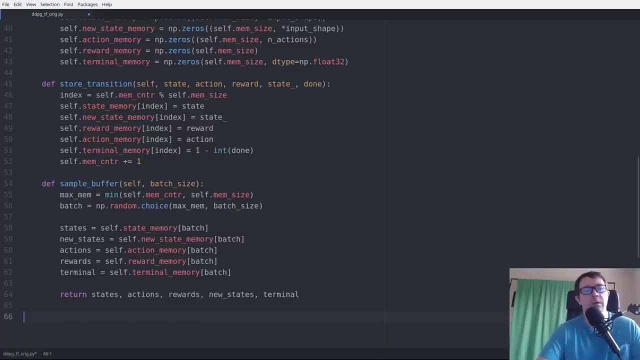 we'll go ahead and start with the actor And from there, keep in mind that we have two actor networks And we're going to go ahead and do a little bit more repaired code on these And with, TensorFlow likes to do stuff, So let's get started. 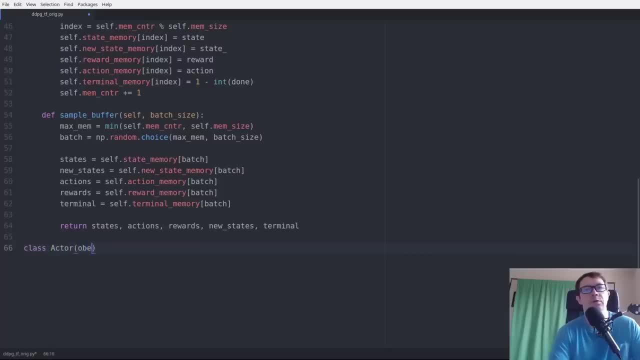 the actor. And of course, in TensorFlow you don't derive from any particular class around pytorch, you would derive from an end up module. Don't know what I'm doing there. definite, So we'll need a learning rate, number of actions, a name, and the name is there to. distinguish the regular actor network from the target actor network. So we'll need to look at that for real quick. So we'll go ahead and check out the actual actor network So we can see the action rates, the number of actions that are there. And for the actual actor network we're 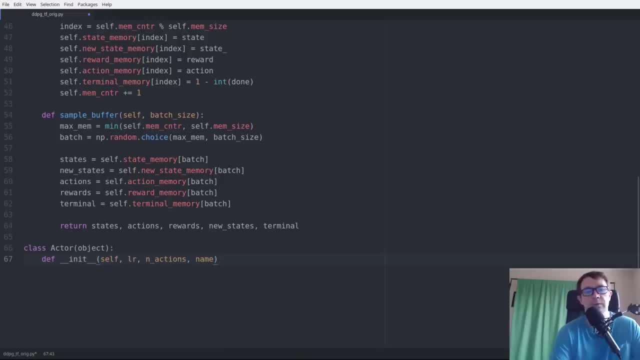 And the name is there to distinguish the regular actor network from the target actor network. Input DIMMs. We're going to want to pass it a session, So TensorFlow has the construct of the session which houses the graph and all the variables and parameters and stuff like that. 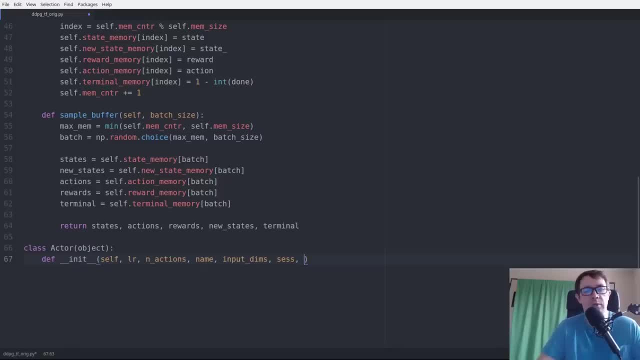 You can have each class having its own session, but it's more tidy to pass in a single session to each of the classes A number of dimensions for the first fully connected layers. So of course that should be 400.. If we're going to implement the paper precisely, FC2 DIMMs is 300.. 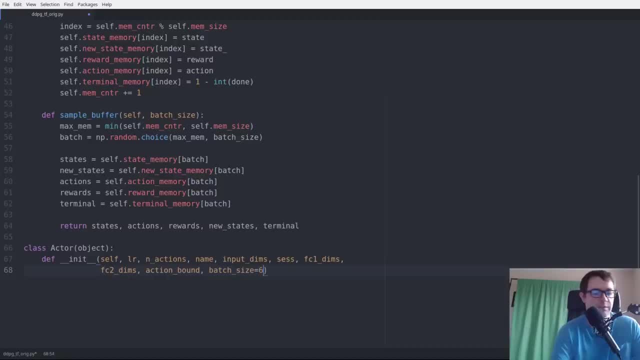 An action bound, a batch size That defaults to 64.. A checkpoint directory, And the purpose of that is to save our model, And in the case of the pendulum it doesn't really matter because it's so quick to run. 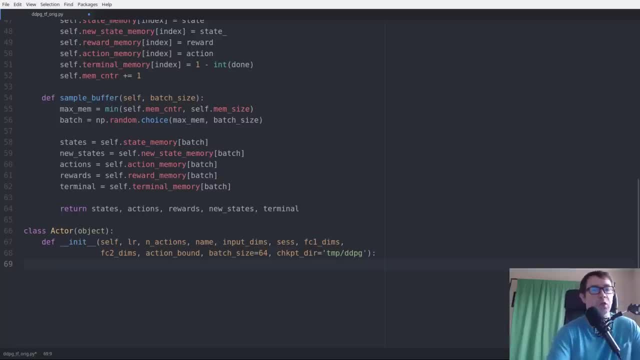 But in general, you want a way of saving these models because it can take a long time to run. So we'll save our learning rate, Number of actions And all of the parameters we passed in fc1DIMMS- fc1DIMMS. 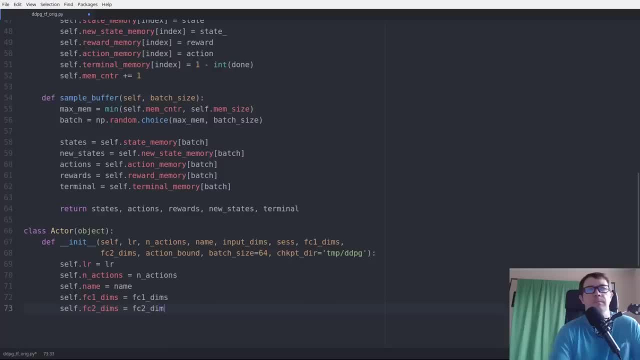 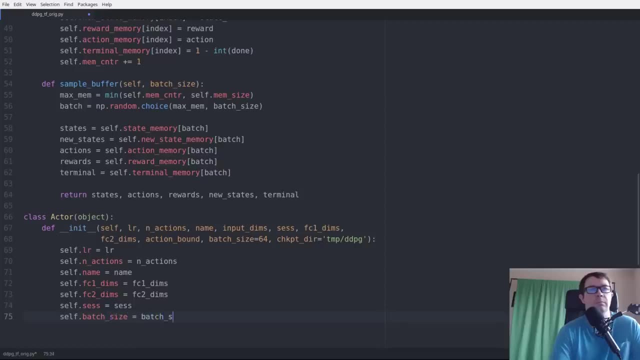 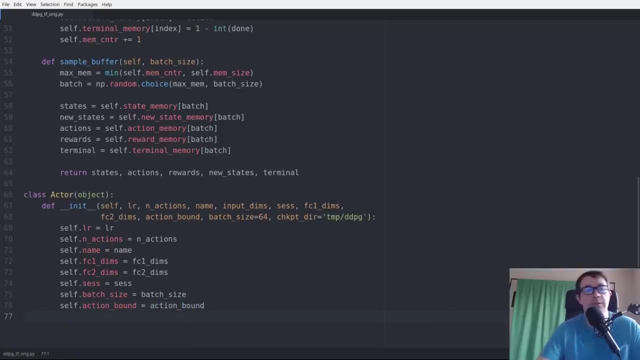 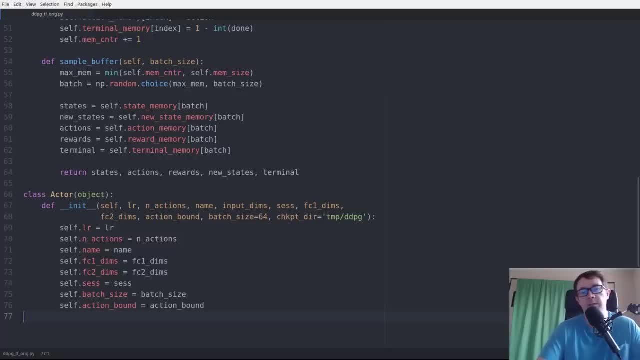 So if you can go from plus or minus two, the tangent hyperbolic is only going to sample like half your range, right from plus minus one, And so you want to have an action bound and there is a multiplicative factor to make sure that you can sample the full range of actions available to your agent. 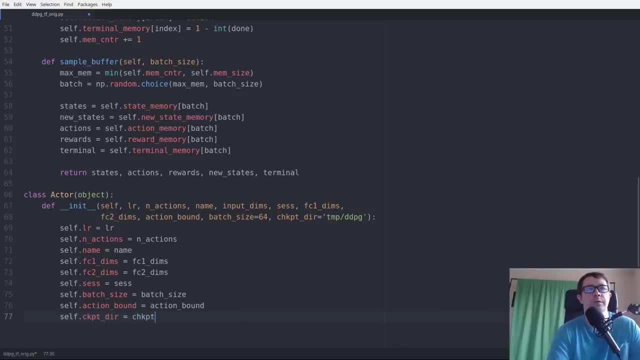 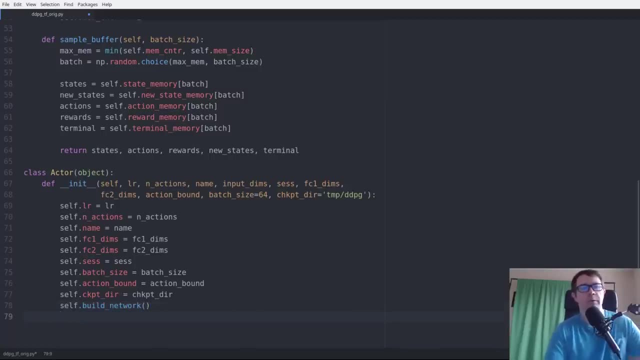 And we need to say that- checkpoint dir. And finally, we want to call a build network function. That's not final but we'll call the build network function Next up since we have to do the soft cloning, the soft update rule for the target actor class and target critic. 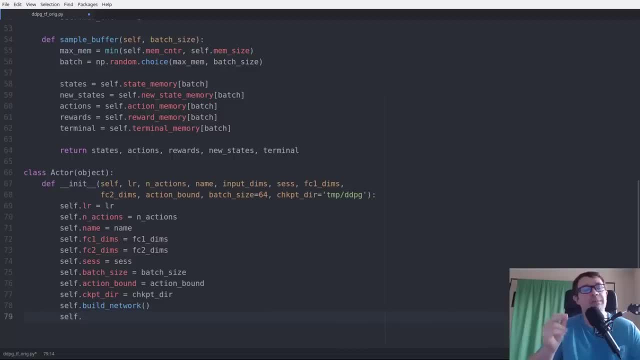 then we know that we have to find a way of keeping track of the parameters in each network. So we're going to keep track of them here in the variable params, And it's tensorflowtrainable variables with a scope of selfname. So we have a single session, a single graph, and you're going to have multiple deep neural networks within that graph. 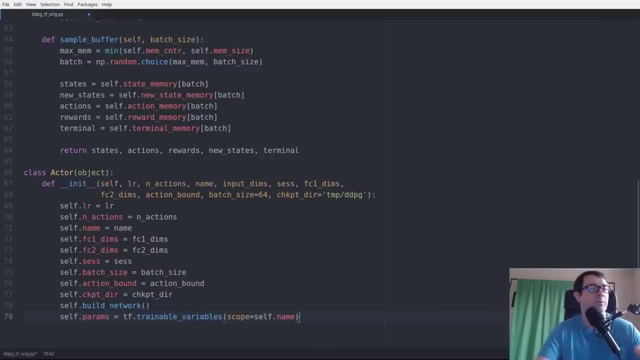 We don't want to update the critic network when we're trying to do the actor network and vice versa. right, We want those to be independent, And so we scope them with their own name, so that TensorFlow knows. hey, this is a totally different set of parameters from this one. 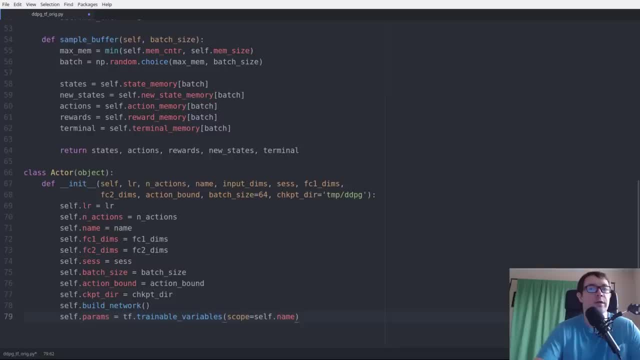 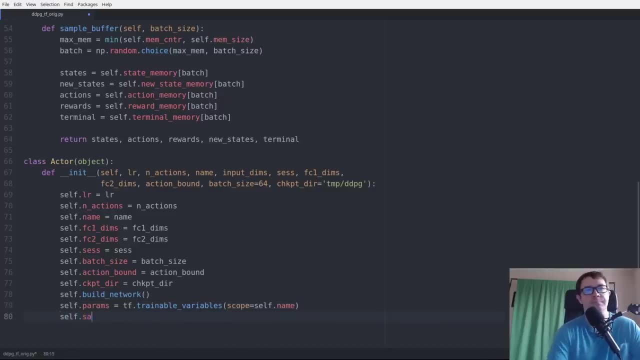 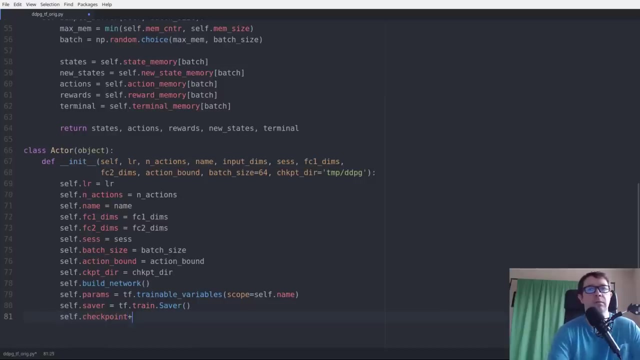 And that will aid in copying stuff later And it also makes sure that everything is nice And tidy, And the scope is what facilitates that. We'll also need a saver object to save the model. Let's make a checkpoint file, And that's where we use OS. 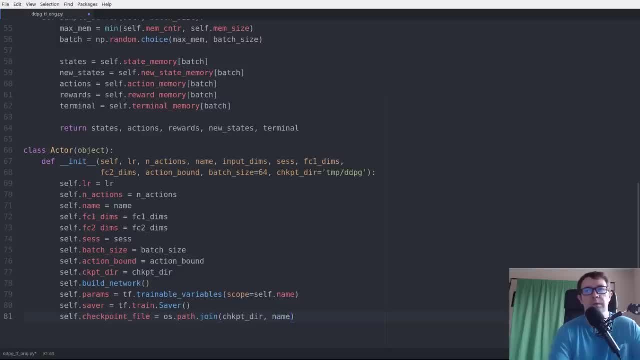 And that will clone into checkpointer and the name plus underscore ddpgcheckpoint, So this will automatically scope the save files, So that way we don't confuse the parameters for the target actor and actor or critic and target critic, or even actor and critic, for that matter. 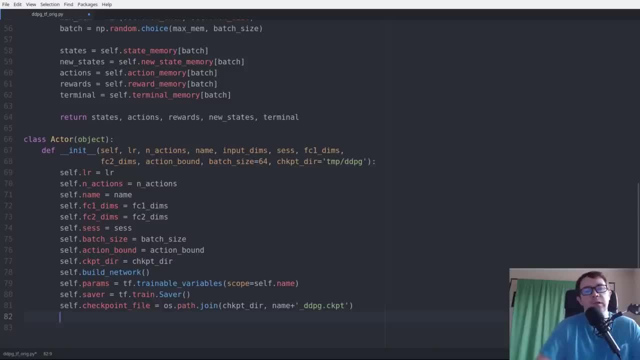 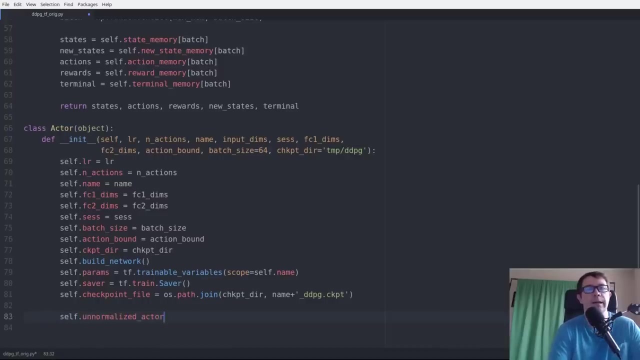 Very important. So we're going to have to calculate some gradients, And we're going to do that by hand, So we're going to need a series of functions that will facilitate that, And the first of which is the unnormalized actor gradients. 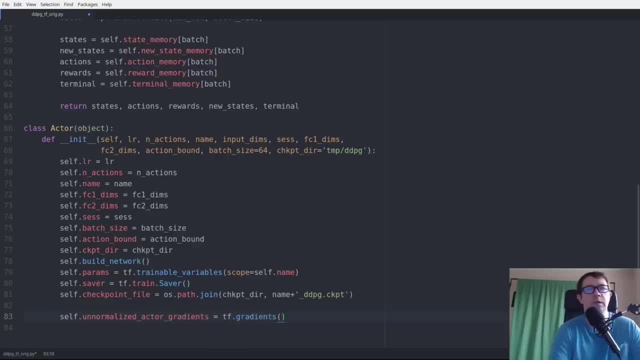 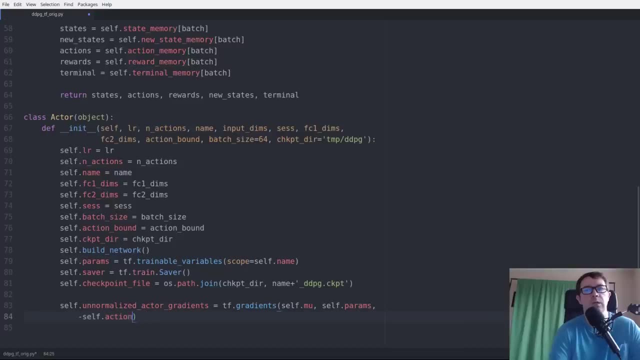 And that is Given my tensorflowgradients, selfmu, selfparams and minus selfactiongradient. So we're going to calculate. So mu will be the mu from the paper. the actual actions of the agent Params are our network parameters. 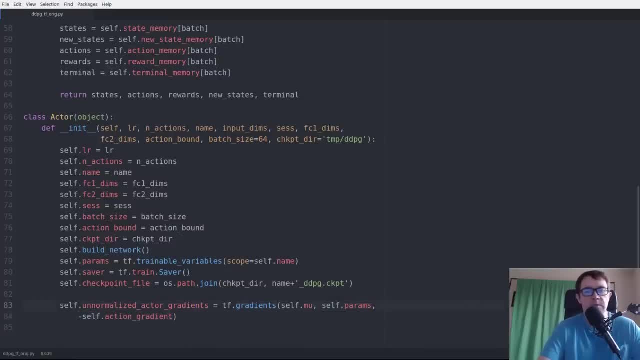 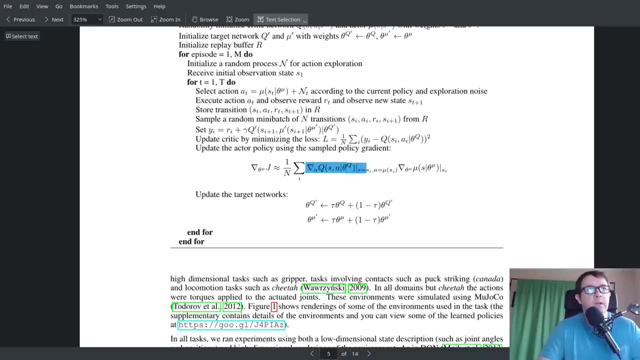 And this action gradient. So let's go back to the paper for a second so we can get some idea what I'm talking about here. So if we look at the algorithm, we can see that we're going to need these Gradients of the critic function with respect to the actions taken. 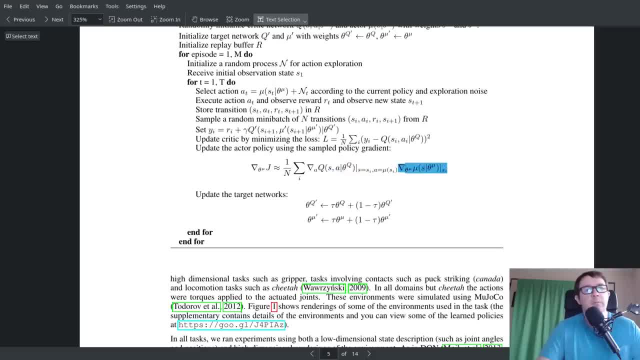 We're also going to need the gradient of the actual mu with respect to the weights of the network. So we're passing in into tensorflow gradients this function, mu, the parameters to get the gradient with respect to those parameters, And then we're going to have to calculate the gradient of the critic with respect to the actions taken. 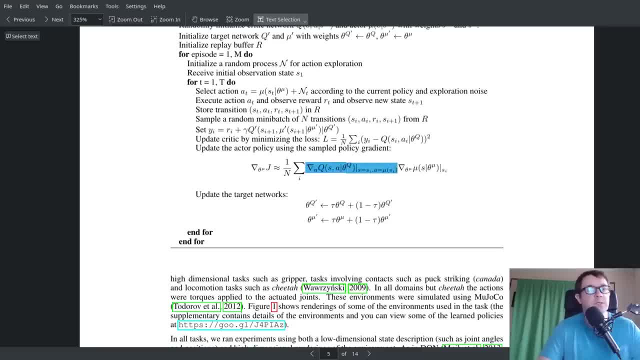 So we'll have to calculate this later. That's a placeholder, That's the minus selfaction gradient, And we're going to calculate that in the learning function. But that's where all of that comes from. So now let's go back to the code editor and continue. 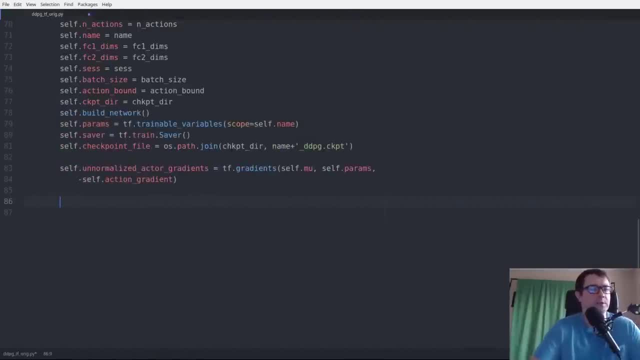 So that's our unnormalized actor gradients, and unnormalized is just because we're going to take one over the sum, one over n times a sum. We need a function for performing that normalization. So the actor gradients has to be this parameter has to be a list. 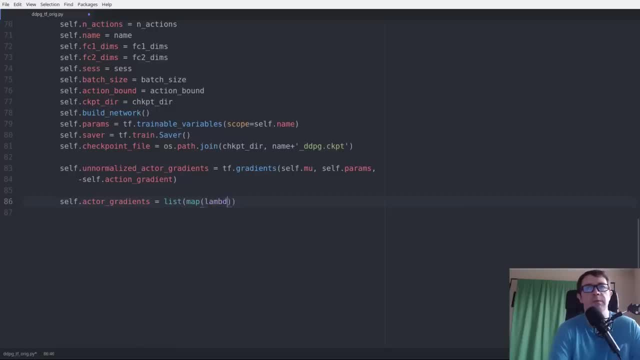 So we cast it as a list and we're just going to map a lambda function And to x, tfdiv, x and batch size. No big deal there. So optimize is our optimization step And of course that's the atom optimizer. We want to optimize with a learning rate of self dot learning rate. 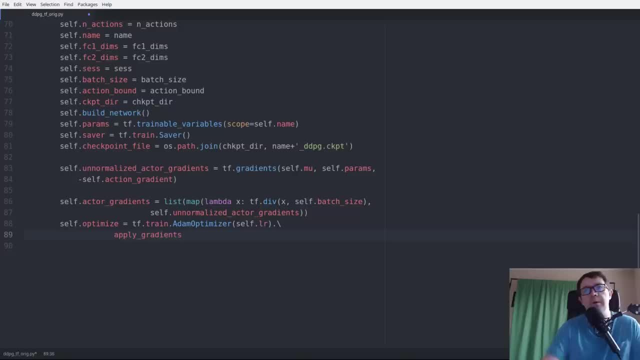 And we want to apply gradients. So typically we'd use dot minimize loss. But in this case we're calculating our grades manually, So we need to apply those gradients. And what do we want to apply? want to apply the actor gradients to the params. 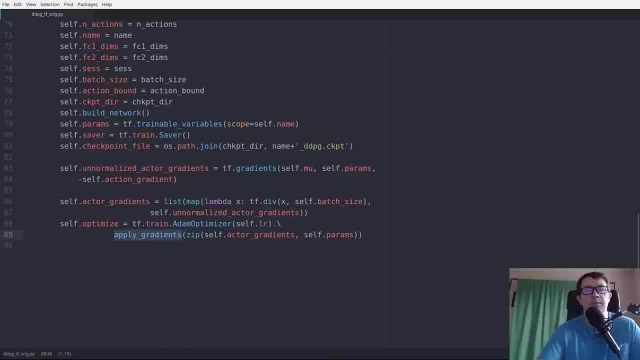 And I would encourage you to go look at the TensorFlow code for all of these. the video is getting a little bit long. we're already up to like an hour and 20 hour and 1020 minutes, something like that, So I'm not going to go through all the documentation for TensorFlow. 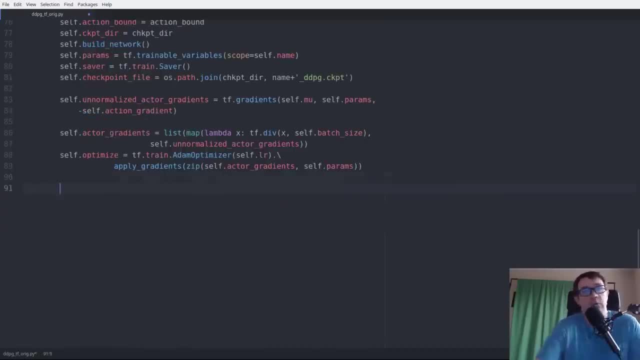 Feel free to look that up. I had to when I was building this out. So next up, we need to build our network. So this is how we're going to handle the scoping: tf, dot, variable, underscore, scope, self dot names. that way, every network gets its own scope. 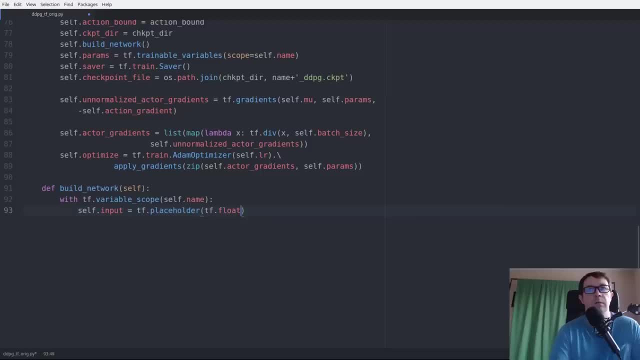 We need a placeholder for the input. That'll be a 32 bit floating number, shape of none, which is batch size. So we're going to do that And we're going to give it a name. it's not critical. the name parameter is just for debugging if something goes wrong and then you can kind of trace where it went wrong. makes life a little bit easier. 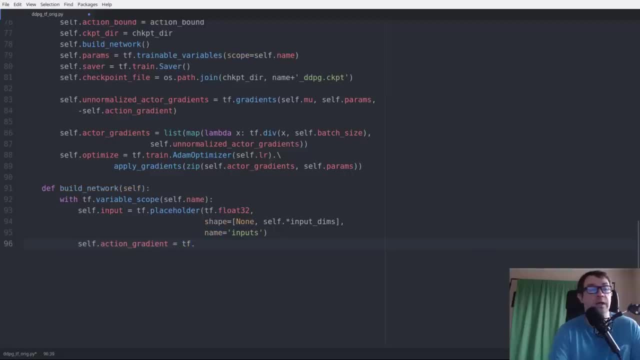 The action gradient is also a placeholder. That is what we're going to calculate in the learn function for the agent And that gets a shape of none by an actions. So it'll be the gradient of q with respect to each action. So it has number of dimensions, which is of actions. 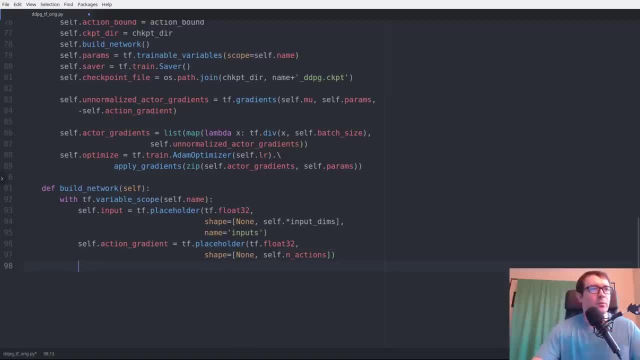 And so those are our two placeholder variables. Now we get to construct the actual network. So let's handle the initialization first. So f1 is the fan in it's one divided by numpy square root. FC one dims And our dense one 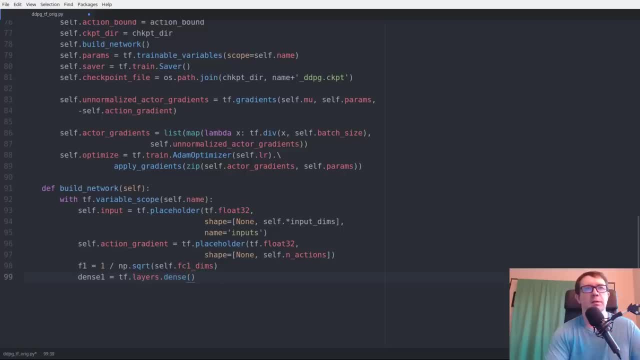 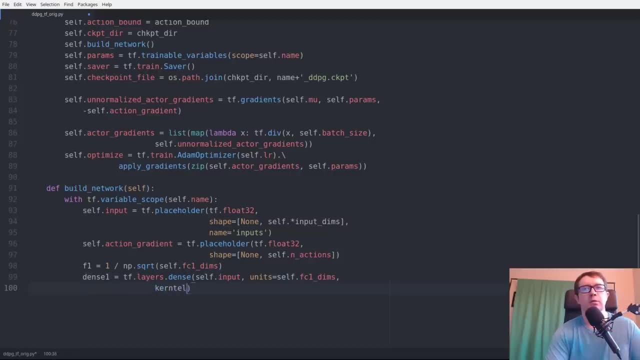 So tf layers, not dense, And that takes self dot input as input with self dot FC, one dims as units. Our kernel initializer equals random. I forgot it in imports. It's random uniform, One second minus f1 to f1.. And the bias initializer: 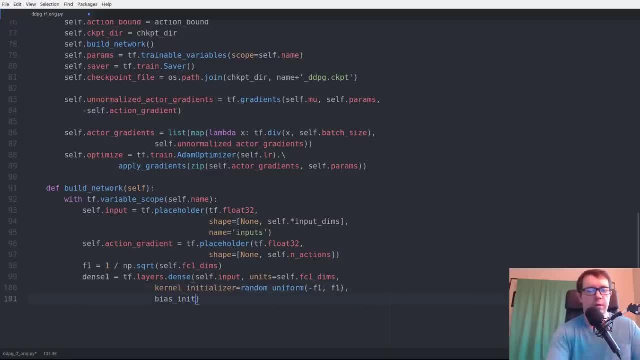 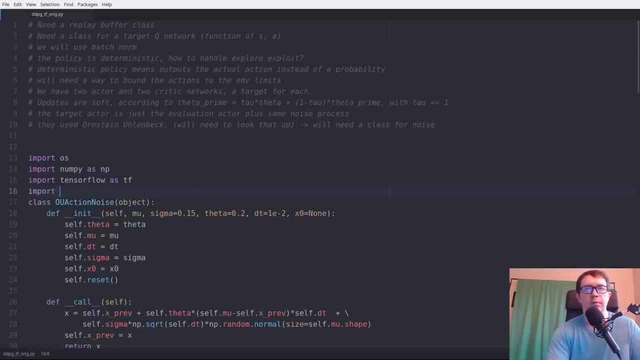 current tell: no, that's not right. Kernel bias initializer: Random uniform minus f1 to f1, that gets two parentheses. So we have to come back up to our imports: Import tensor flow dot initializers: No. So we have to come back up here and say: from tensor flow dot initializers initial. 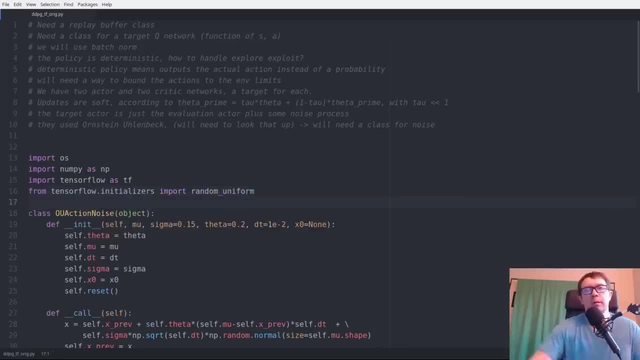 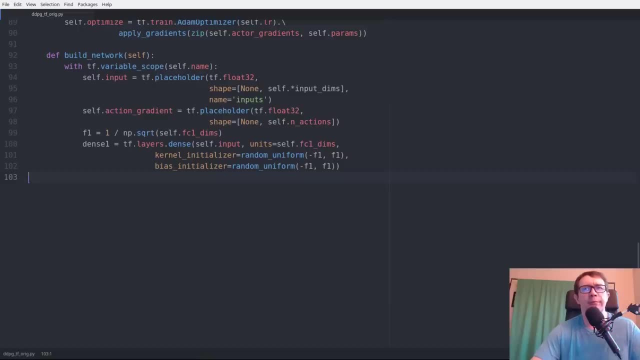 isers, Import random, uniform, and now we're good to go. Let's come back down here. Um, we have dense one. Now we want to do the batch normalization. So batch one equals tf layers, batch normalization, dense one. and 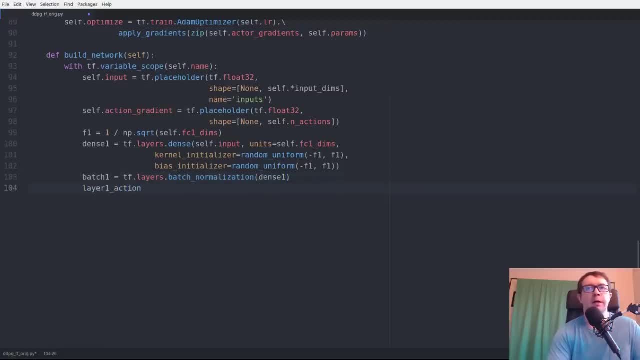 that doesn't get initialized. So now let's uh activate our first layer And that's just the relu activation of the batch normal batch normed. Now it is an open debate, uh, from what I've read online, about whether or not 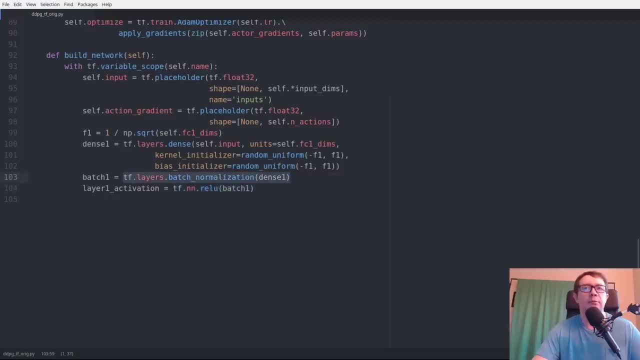 you should do the activation before or after the batch normalization. I'm in the camp of doing it after uh, the activation after the batch norm. That's because um the relu activation function, at least in uh, at least in the case of relu. So in relu you lop off everything lower than zero. So in relu you lop off everything lower than zero. So your statistics might get skewed to be positive instead of maybe they're zero, maybe they're negative, Who knows. So I think the batch norm is probably best before the activation. 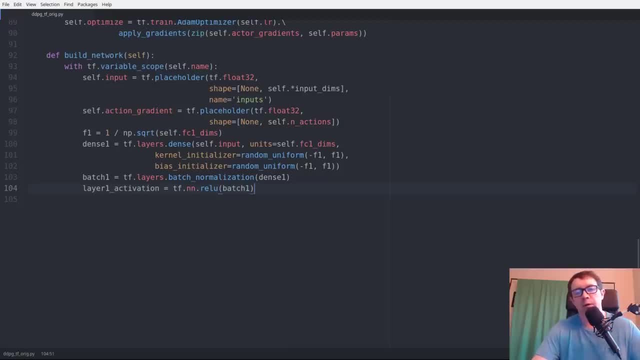 And indeed this works out. This is something you can play with, Uh, so go ahead and fork this repo and play around with it and see how much of a difference it makes for you. Maybe I missed something when I tried to do it the other way. 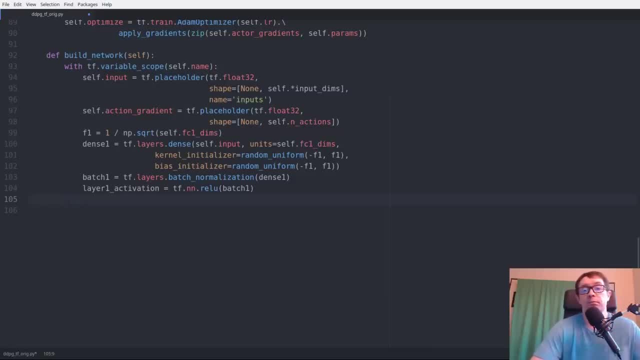 It's entirely possible. I miss stuff all the time, Uh, so you know it's something you can improve upon. Uh, that's how I chose to do it, Uh, and it seems to work and, who knows, maybe other implementations. 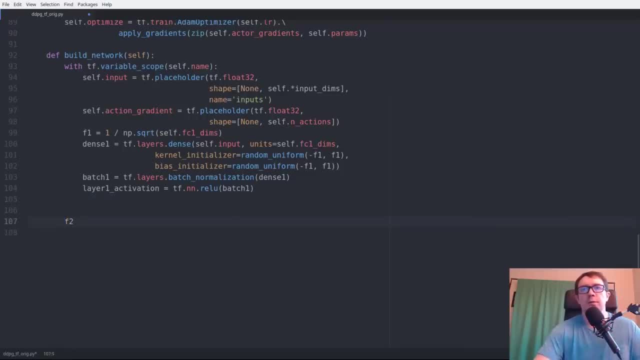 Yeah, Work as well. So now let's add some space. So F two is one over square root, SC two DIMMs. dense two is similar. That takes layer one activation as input with SC two DIMMs. You don't need that. I'm going to come up here and copy this. 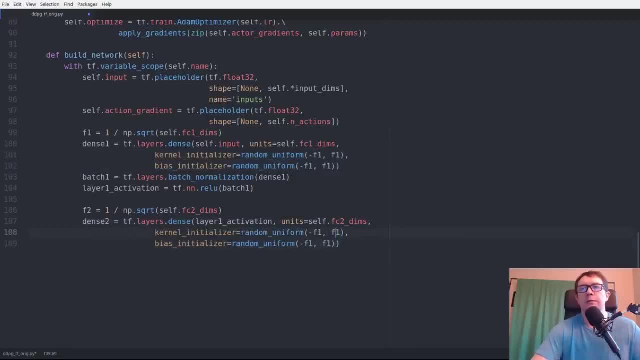 There we go, Except we had to change F one to F two. Perfect. Then we have batch two, and that takes dense two as input here to activation batch two. Now, finally, we have the output layer, which is the actual policy of our agent. 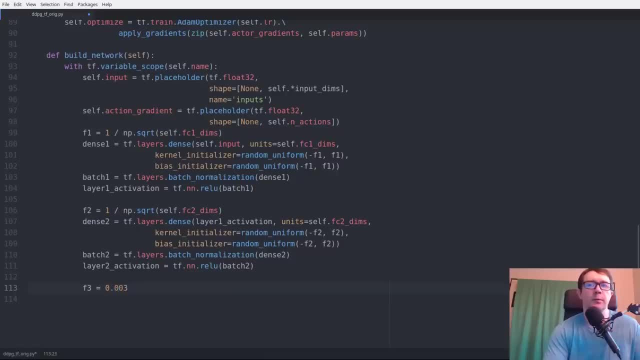 the deterministic policy, of course, and from the paper that gets initialized with the value of 0.003, uh, and we're going to call this mu, that gets layered to activation as input and that needs an actions as the number of output units. 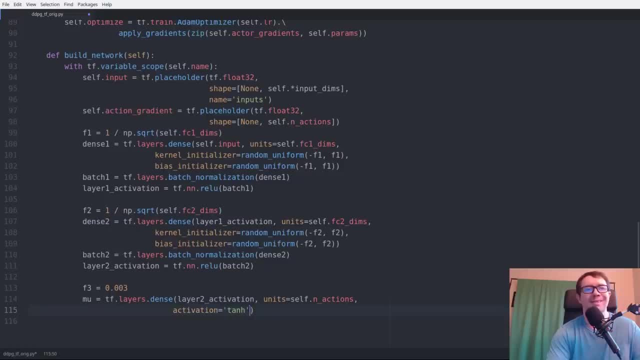 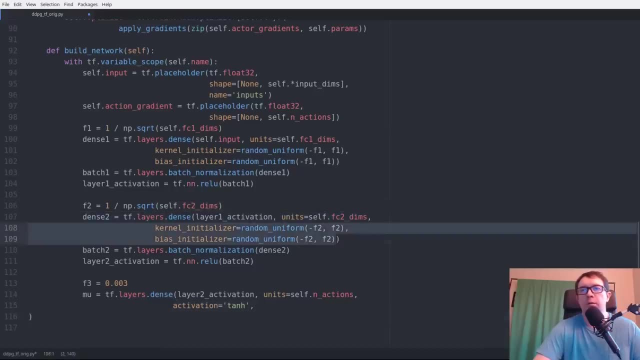 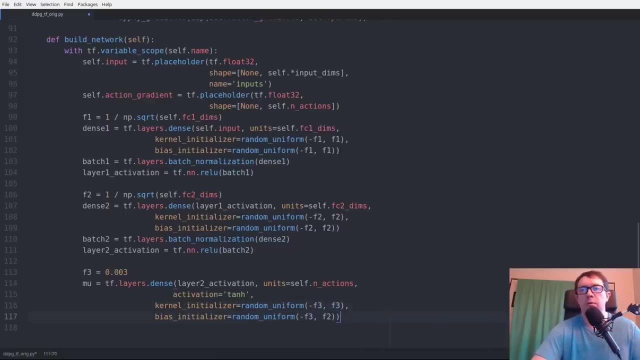 What's our activation? That is tangent hyperbolic tanch and I will go ahead and copy the initializers here. Of course that gets F three, not F two. Perfect, Can I tab that I can? Okay, So that is mu. 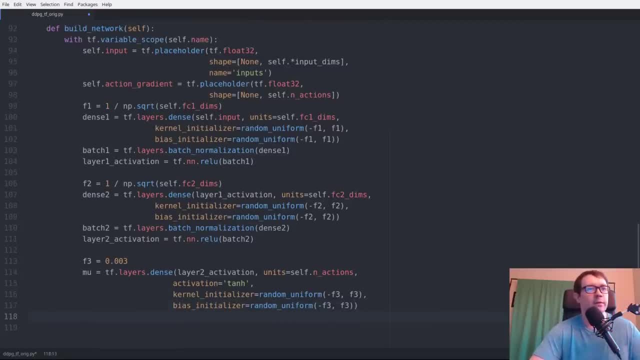 Uh. and then we want to take into account the fact that our environment may very well uh require Actions that have values plus uh, greater than plus or minus one. So self dot mu is TF dot. multiply with mu and the action bound and action bound will be, you know. 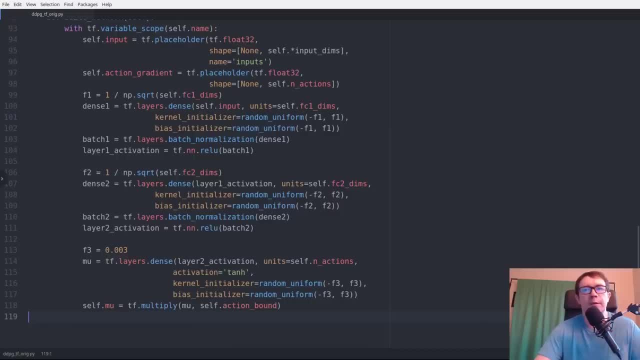 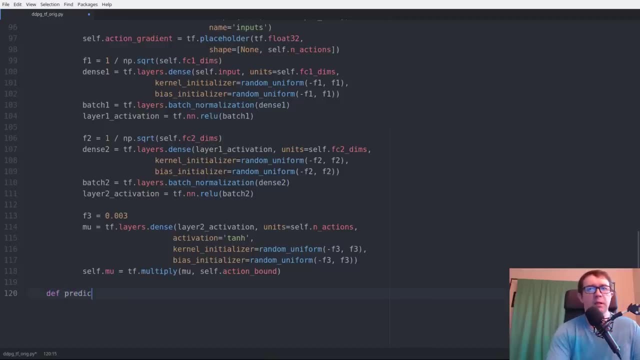 something like two: It needs to be positive, So that way you don't flip the actions. Uh, but that's pretty straightforward. So now we've built our network, built our network. Next thing we need is a way of getting the actual actions out of the network. 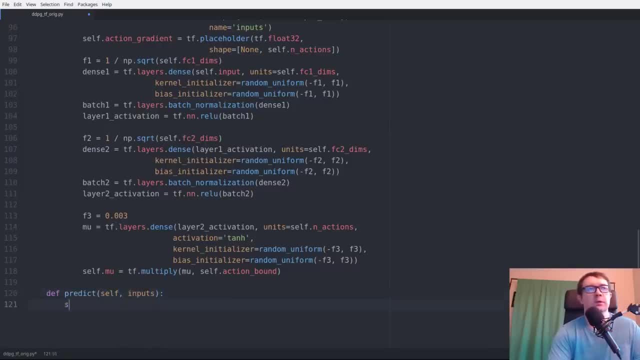 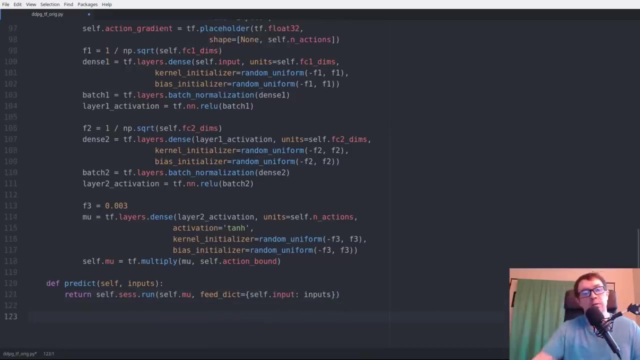 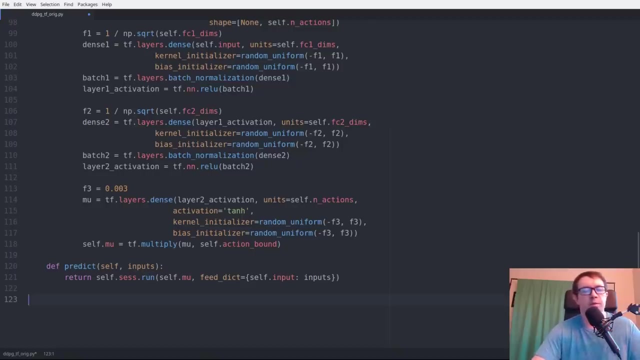 So we have a prediction function. Okay, That takes some inputs and you want to return self dot, cess, dot run, self dot mu with a feed dictionary of uh, self dot input and pass in inputs. That's all that is. there is to uh passing the doing the feed forward. kind of an interesting contrast to how PyTorch does it with um, the explicit construction of the feed forward function. 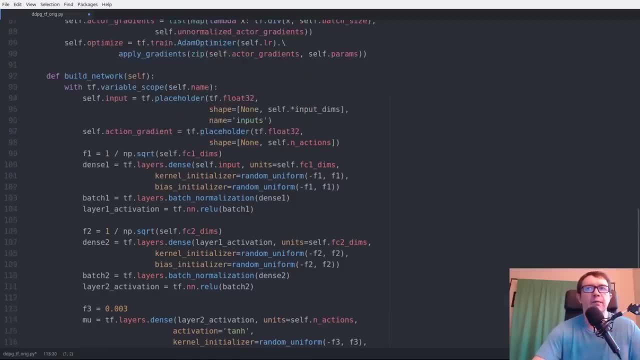 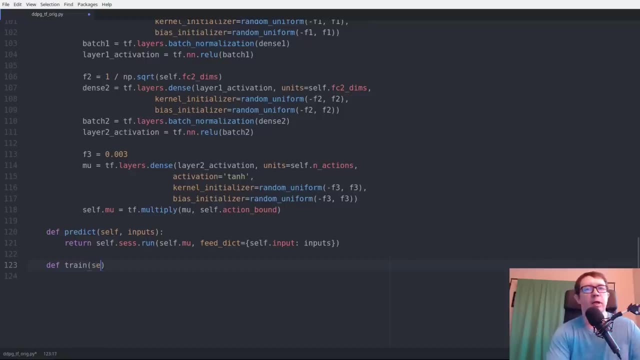 This just runs the session on this and then goes back and finds all the associations between the Uh respective variables. nice and simple. Now we need a function to train uh and that'll take inputs and gradients. This is what will perform the actual back propagation through the network. 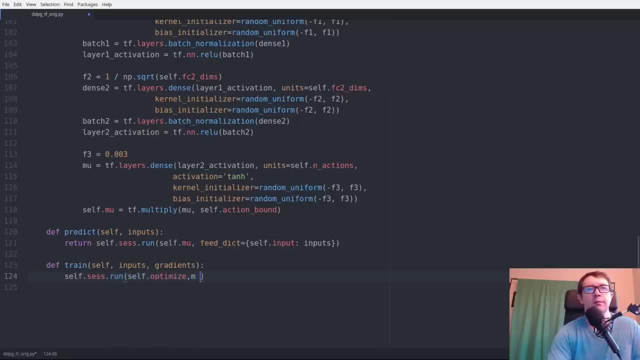 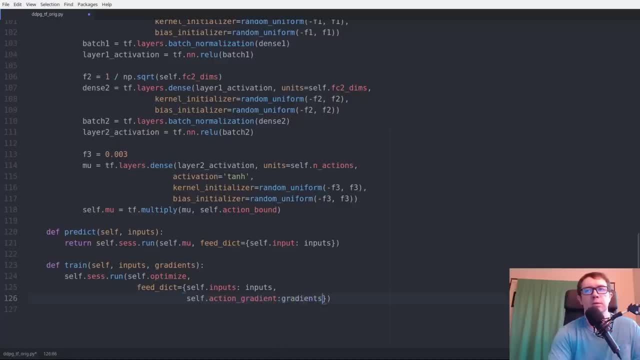 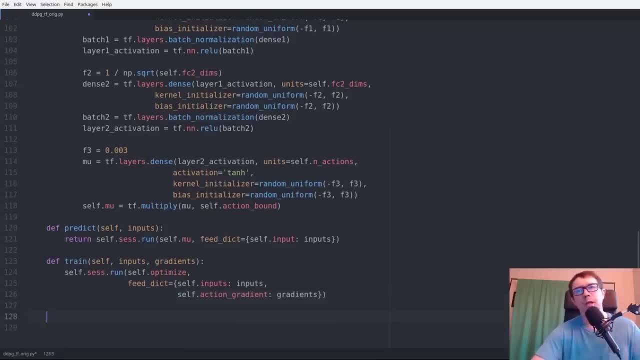 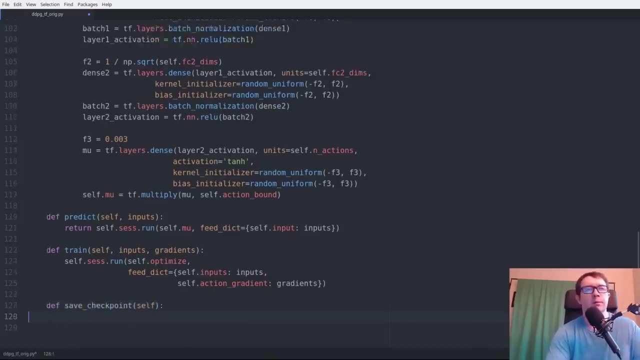 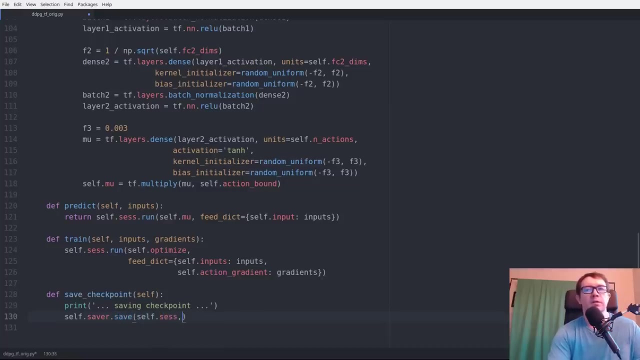 All right. So that is our training function. Next, we need two functions to accommodate the loading and the saving of the model. So define: save, checkpoint print. Okay. then you want to say selfsaversave, very creative, you want to save the current session. 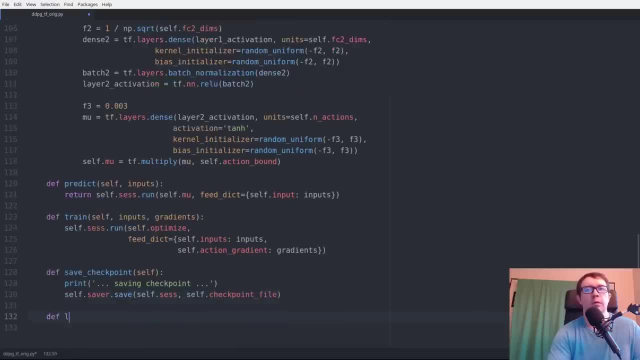 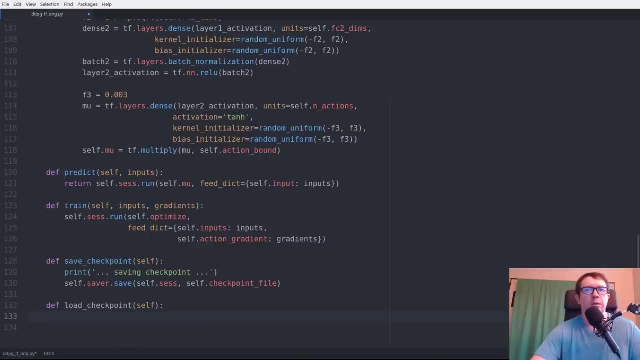 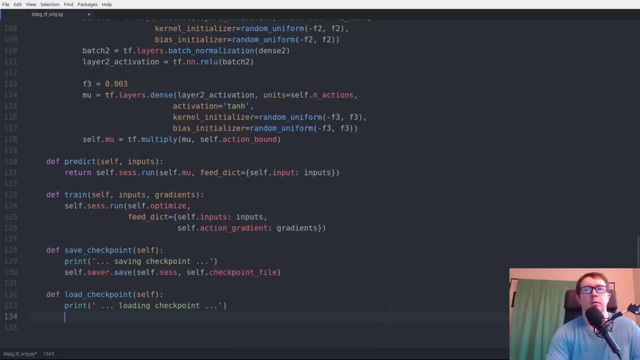 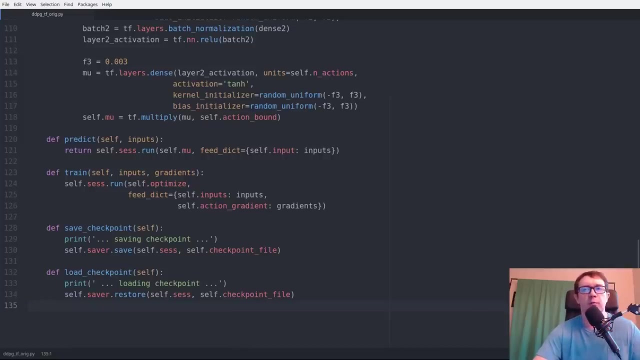 to the checkpoint file and the load checkpoint function is the same thing, just in reverse. so here we want to print loading checkpoint, selfsaverrestoresession and the checkpoint file, so that will. you can only call this after instantiating the agent, so it will have a default session with some initialized values and you want. 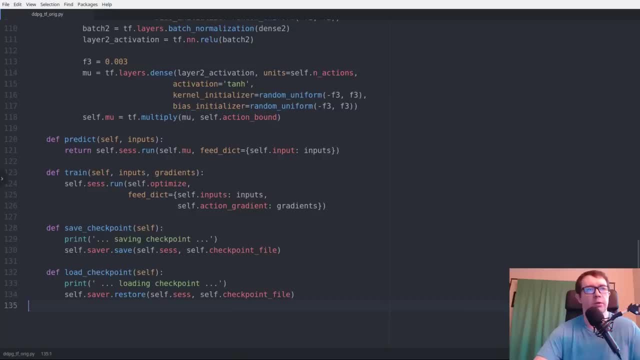 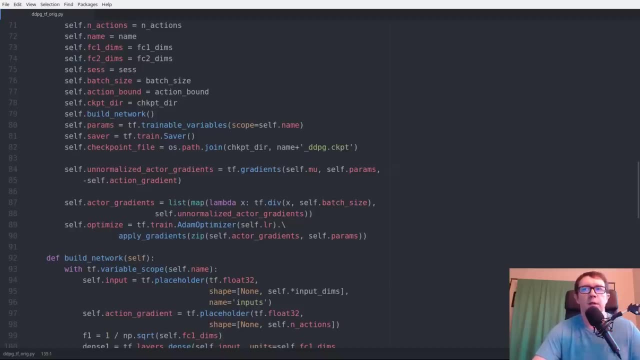 to load the variables from the checkpoint file into that checkpoint, and that is it for the actor class. this is reasonably straightforward. the only real mojo here is the you actor gradients, and this is just two functions that accommodate the fact that we're going to manually calculate the gradient of the critic with respect to the actions taken. so let's go. 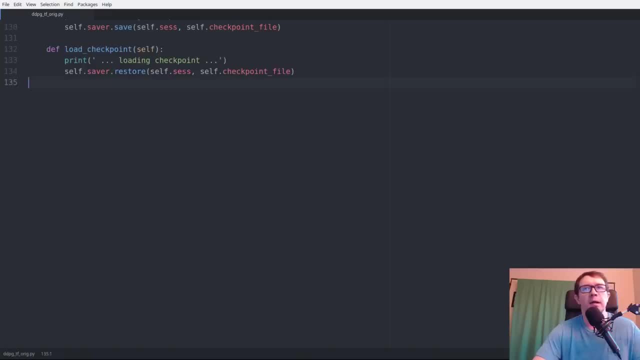 ahead and do the critic class next. that is also very similar, so that again derives from the base object gets an initializer and it's pretty much the same number of actions. a name input dims session, the no session, se1 dims, se2 dims. a batch size will default to 64 and a checkpoint der will default to this. just a note: you have to do a make der on this temp slash ddpg first, otherwise it'll bark at you. not a big deal, just something to be aware of. since it's identical, let's go ahead and copy a good chunk of this stuff here where to add the. 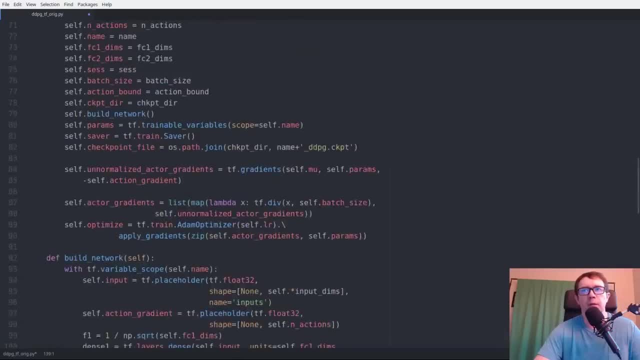 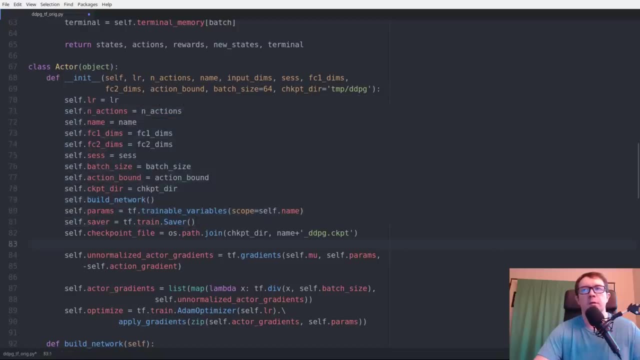 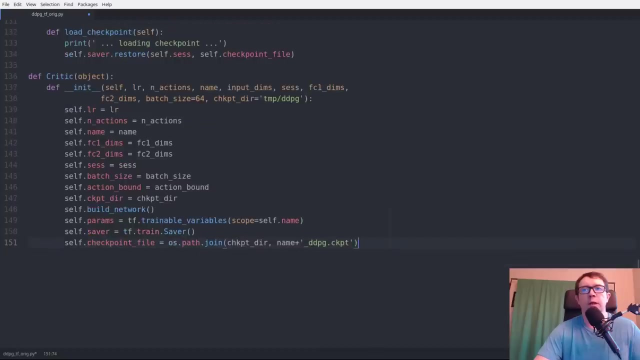 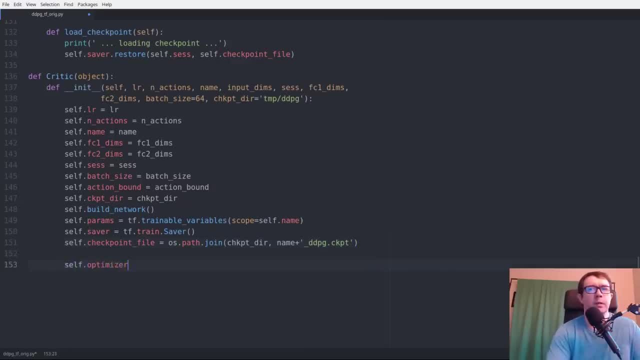 too magical about that. so now let's handle the optimizer, because we already have a- we've already called the function to build our network. we can define our optimizer, so the selfoptimize tf train dot atom optimizer, and we're going to minimize the uh, the loss which we will calculate in the build network function. and we also need uh the function to 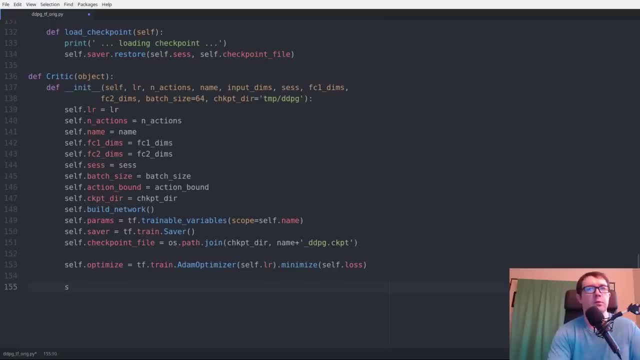 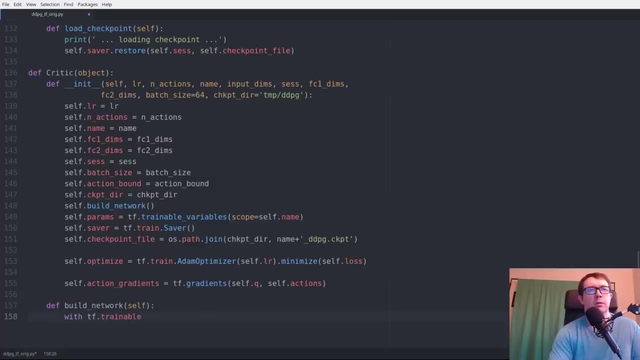 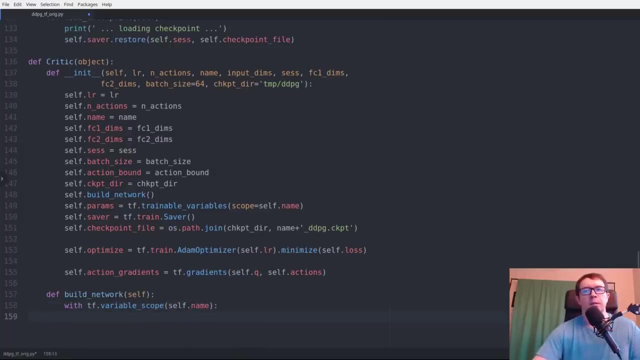 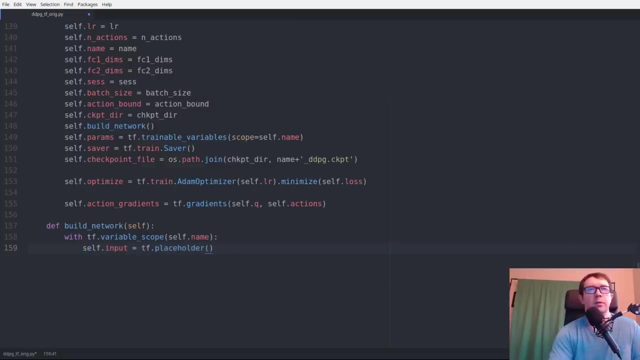 actually calculate the gradients of q with respect to a. so we have selfaction gradients, selfq and actions. let's build our network, uh, with t, sorry, tf, variable, scope, selfname. so now we need our placeholders again. we need selfinput placeholder, float 32. we need a shape, none by input dims. now 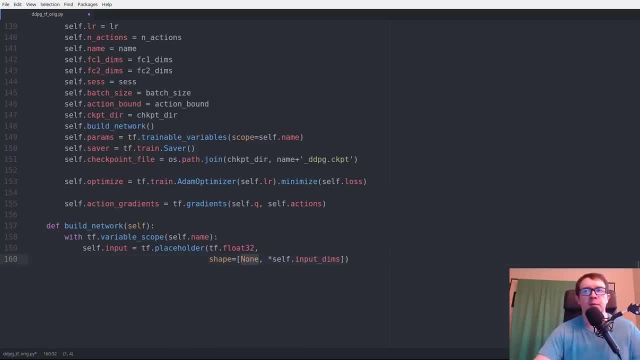 if you're not too familiar with tensorflow, specifying none in the first dimension tells sensorflow. you're going to have some type of batch of inputs and you don't know what that batch size will be beforehand, so just expect anything. and uh, let's delete that and say: 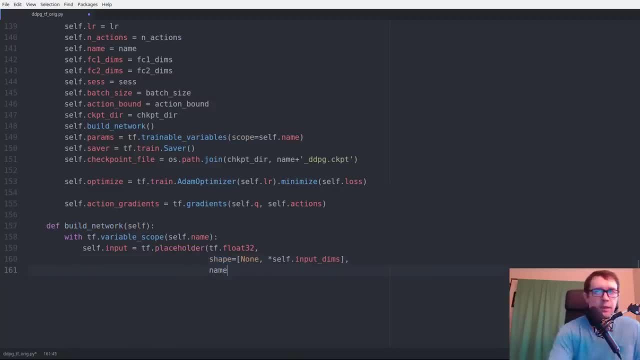 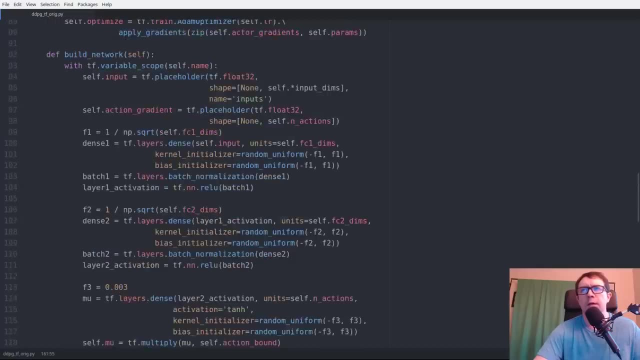 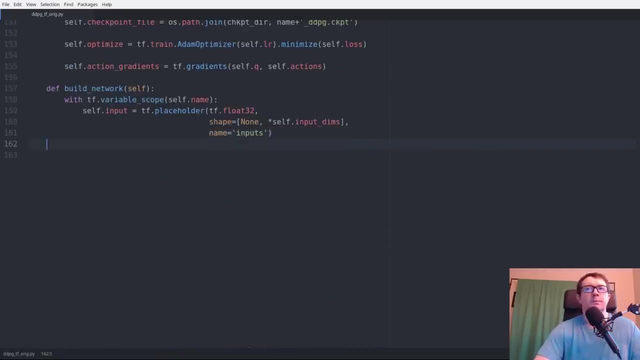 i'll need a comma, for sure, and say: name equals, uh, inputs. there we go. did i forget a comma up here? let's just make sure i did not. okay, so we also need the actions because, remember, we only take into account the actions. uh, on the second hidden layer of the critic neural network, 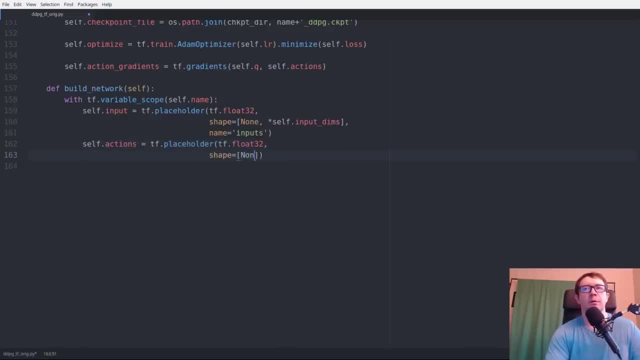 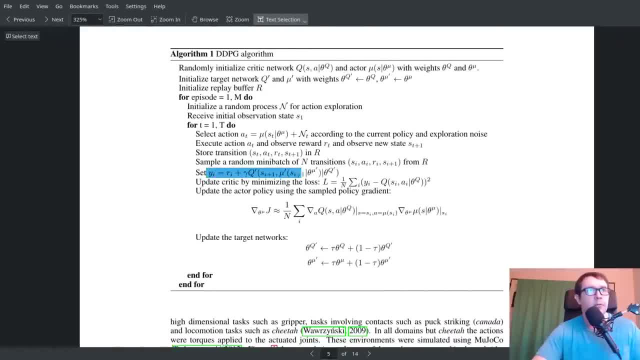 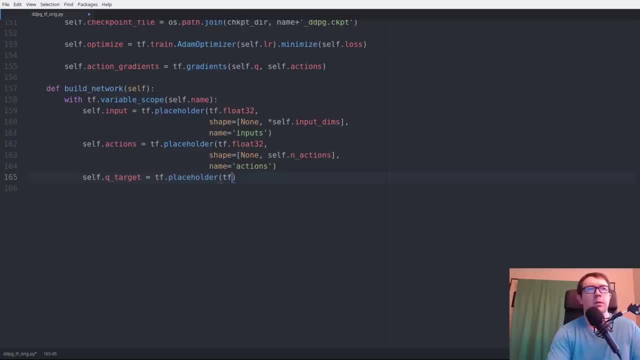 will be so that target value will be this quantity here and we will calculate that in the learning function. uh, as we, as we get to the agent class. so let's go back to the code editor and finish this up. so q target is just another placeholder and that's a floating point number. 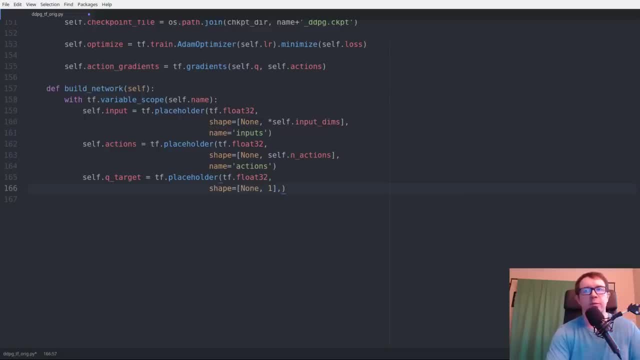 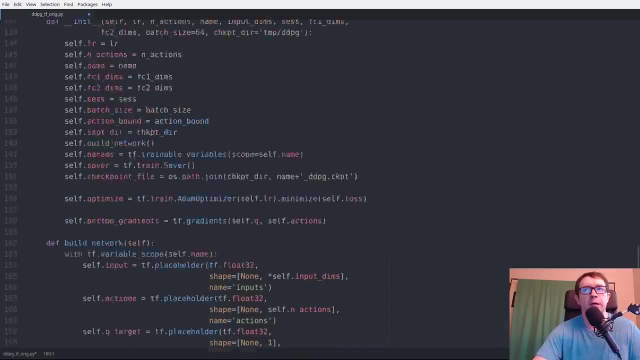 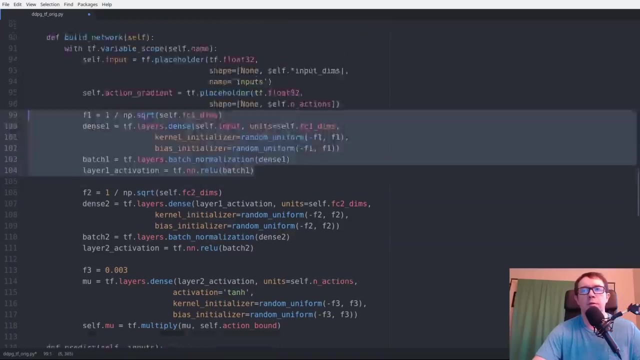 and that's the first of the main points we're about to see. so let's take a look at the and we will come up here and copy this. so it's a scalar, so it's shaped batch size by one and we will call it targets, okay, so now we have a pretty similar setup to the actor network. so let's go. 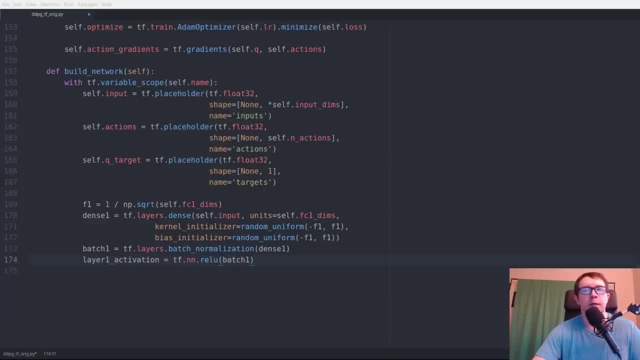 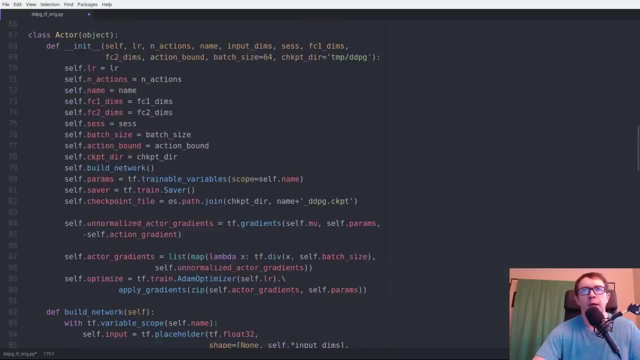 ahead and come up here and copy this. recognize. that's just the fan in. we have a dense layer for the inputs and we want to initialize that with a random number, pretty straightforward. then we can come up to f2 and copy that as as well. sorry, the second layers, it'll be a little bit different, but we'll handle that momentarily. 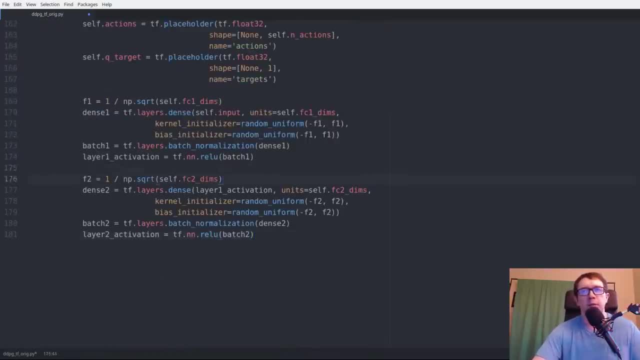 so now f2. the layer 2 is pretty similar. the only real difference is that we want to get rid of that activation. and the reason we want to get rid of that activation is because after we do the batch norm, we have to take into account the actions. so we need another layer. so action in tf layers dense. 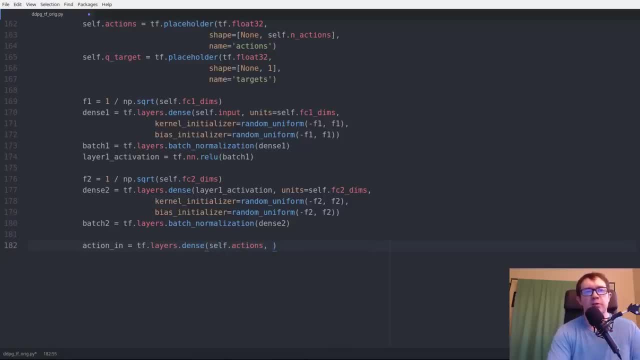 it's going to take in selfactions which will pass in from the learning function and that's going to output f2 with a value activation. so then our state actions will be the uh, the addition of the batch 2 and the action in, and then we want to go ahead and activate that. 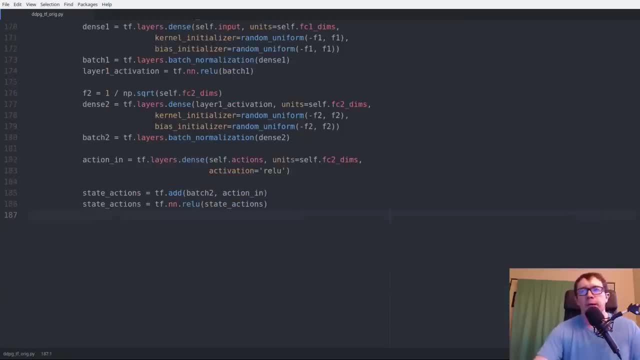 okay. so this is something else i pointed out in my pytorch video, where this is a pointed debate with the way i've implemented this. i've done it a couple different ways, i've done the different variations and this is what i found to work. i'm doing a double activation here, so i'm 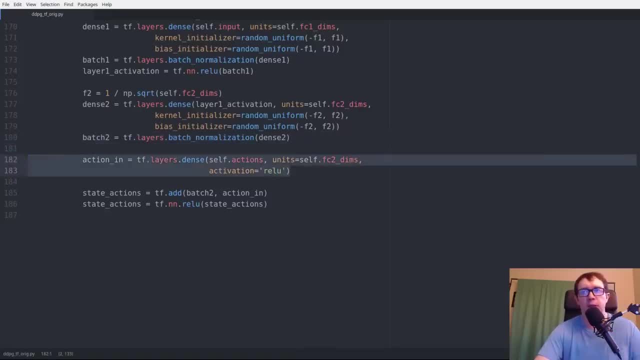 activating the value. i'm doing the value activation on the actions in on the output of that that dense layer, and then i'm activating the sum. now the um, the value function, is non-commutative with respect to the addition function, so the value of the sum is different than the sum of the values and you. 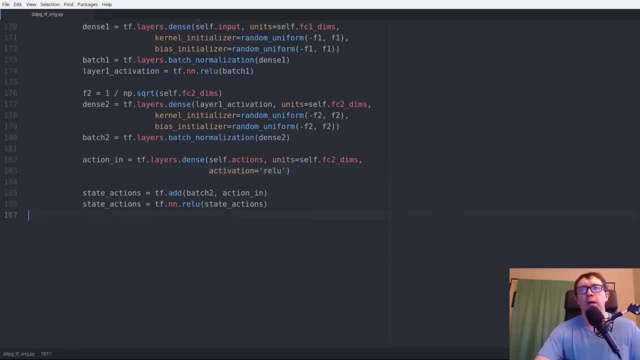 can prove that to yourself on a sheet of paper. uh, but it's debatable on whether or not the way i've done it is correct. it seems to work, so i'm going to stick with it for now. again, fork it, clone it, change it up, see how it works and improve it. for me, that would be. 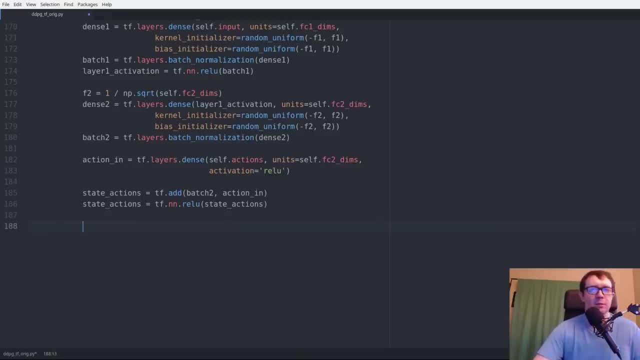 fantastic. then make a pull request and i'll disseminate that to the community. so we have our state actions. now we need to calculate the actual output of the layer and an f3 is our uniform initializer for our final layer, which is selfq. those are layersdense. that takes state actions as input, outputs a single unit and we have the. 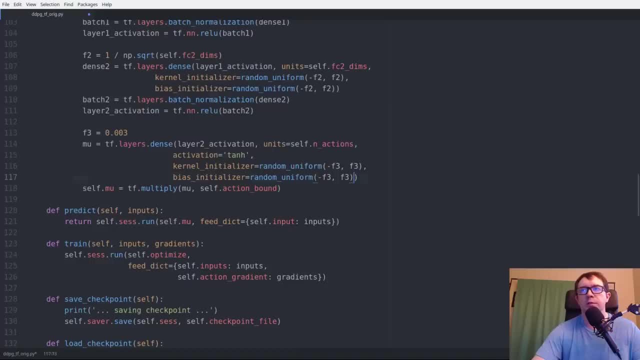 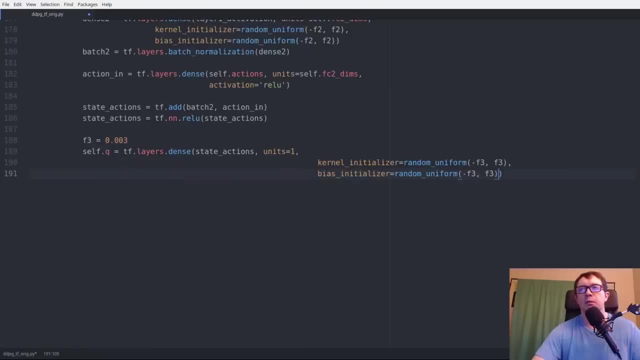 kernel initializers and bias initializers similar to up here. let's paste that. there we go. that's a little bit better. still got a whole bunch of white space there, all right. so we are missing one thing, and that one thing is the regularizer. so, as they said in the paper, they have elton regular regularization. 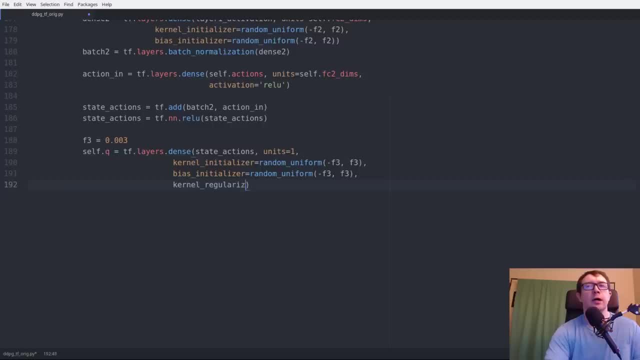 on the critic. so we do that with kernel: regularizer equals tf, charis, regularizers l2 or the value of zero, zero one, uh, zero one, sorry. so that is that for the que, and notice that it outputs one unit and it outputs a single unit. this is a scalar value. you want the value of the particular state action pair. Finally, 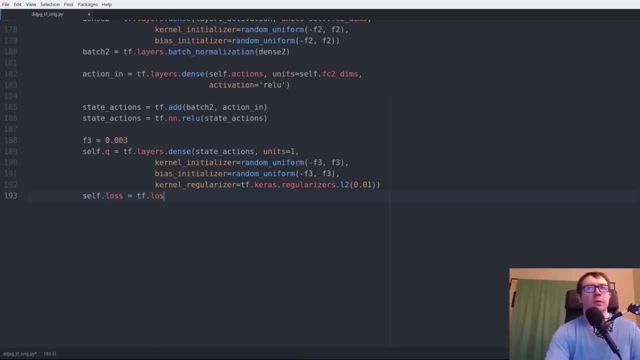 we have the loss function And that's just a mean squared error error: q target and q. So q target is the placeholder up here And that's what we'll pass in from the learn function, from the agent And self dot. q is the output of the deep neural network. Okay, so now, similar to our. 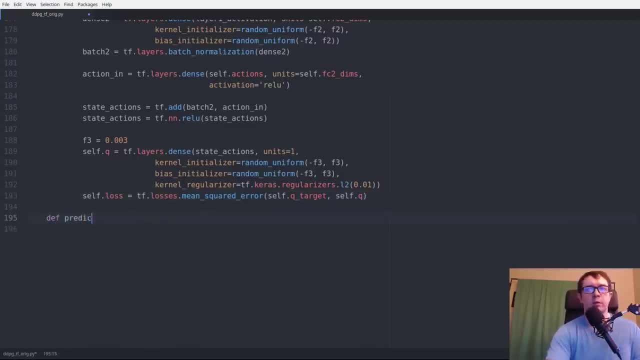 critic. we have a prediction function, takes inputs and actions And you want to return self dot, sess dot run, self dot q with a feed dictionary of sub dot input, inputs and actions. Oops. Next you need a training function And that's slightly more complicated than the actor visa. takes in the inputs, actions and a. 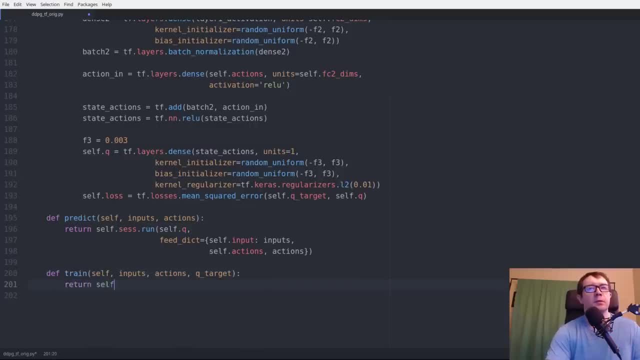 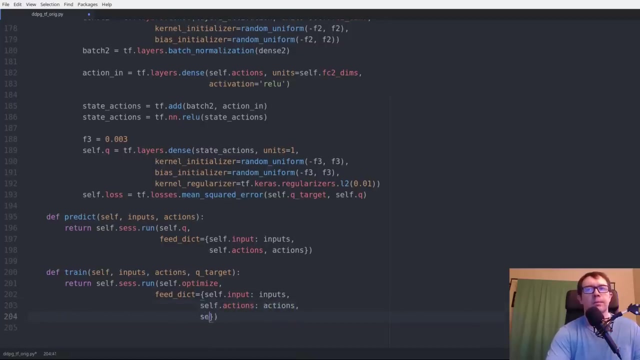 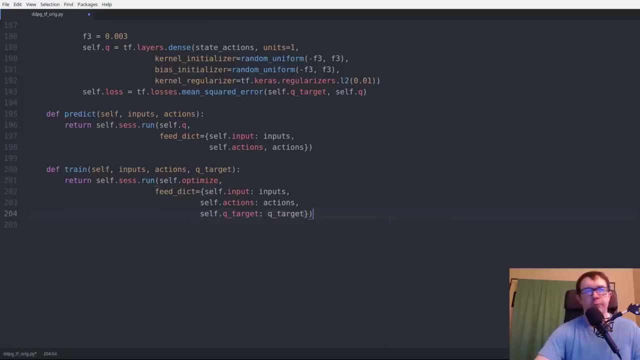 target And you want to return self assess, dot run, So to optimize with a feed dictionary of sub dot input inputs. So dot actions, actions And q target spacing on that little wonky, whatever we'll leave it, That's a training function. Next, we need a function to get the action gradients And that'll 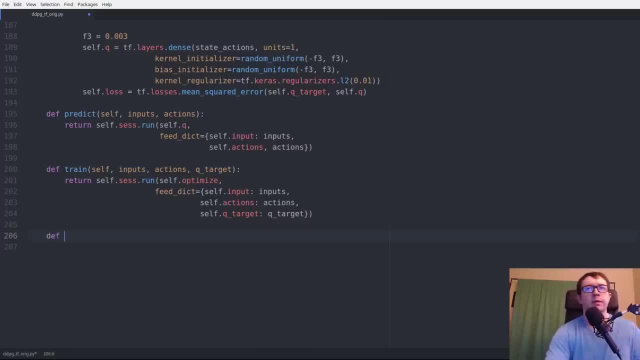 run that action gradients operation up above. So let's get that again. takes inputs and actions as input And you want to return self dot session dot run self dot action and gradients with a zone feed dictionary equals self dot input inputs and self dot actions actions. 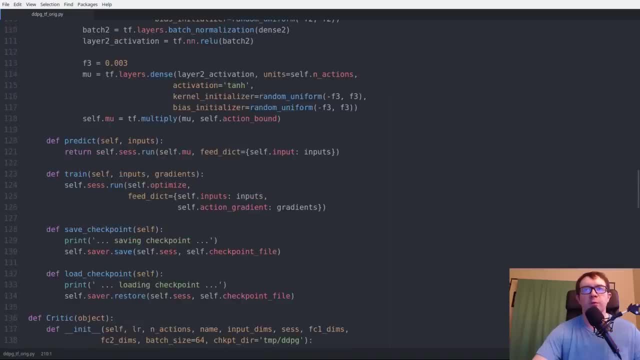 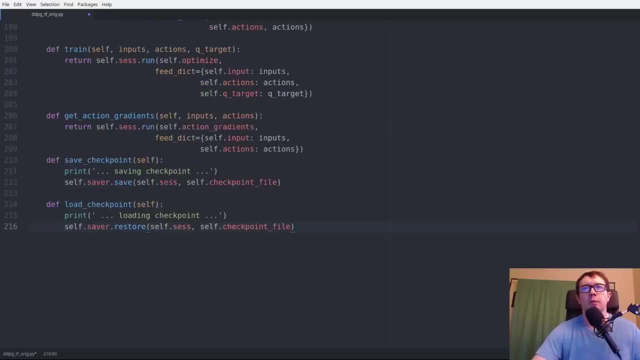 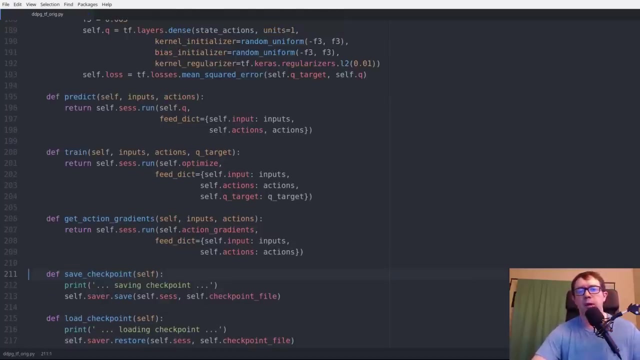 And then we also have the save and load checkpoint functions, which are identical to the actor. so let's just copy and paste those. There we go. So that is it for the critic class. So now we have most of what we need. we have our, our, our noise, our replay buffer, our 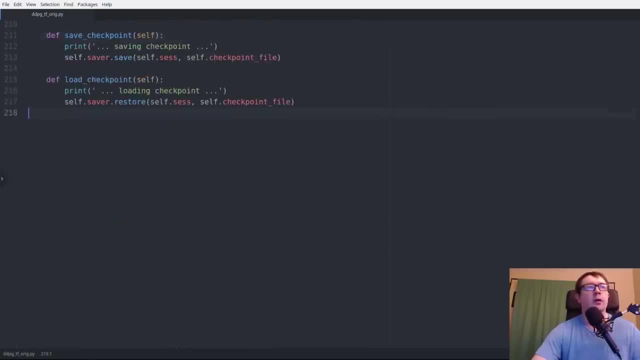 actor and our critic. Now all we need is our agent. Now, the agent is what ties everything together and handles the learning functionality. It'll house the noise, the memory Okay- And the replay buffer, as well as the four different deep neural networks. 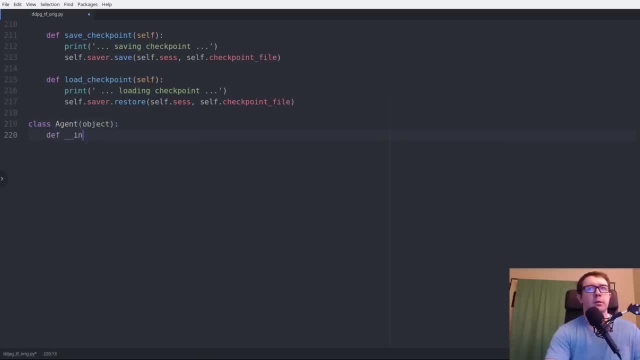 And that derives from the base. object: Initializer is a little bit long and that takes an alpha and a beta. These are the learning rates for the actor and critic respectively. Recall from what we read in the paper. they use 0 0 0 1 and 0 0 1 for both networks. 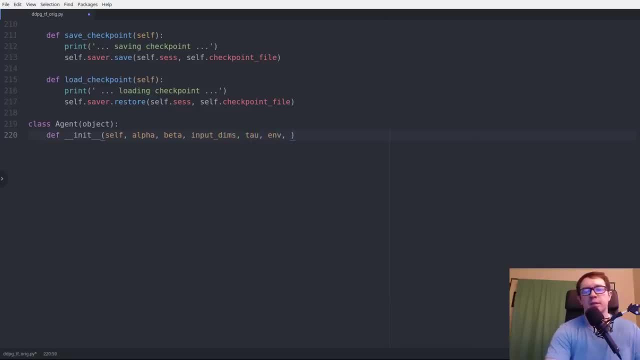 We need input, dims, tau, the environment. That's how we're going to get the actor, The action bounds, a gamma of 0.99 per the paper. In this case we need number of actions equals two um a mem size, for our memory, of 1 million. 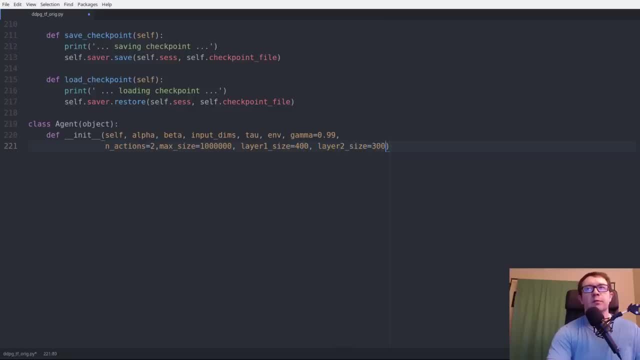 layer one size of 400 and layer two size of 300 and a batch size of 64. So of course, we want to save all of our parameters, Okay. Okay, We'll need the memory and that's just a replay buffer max size. whoops, uh, input dims and 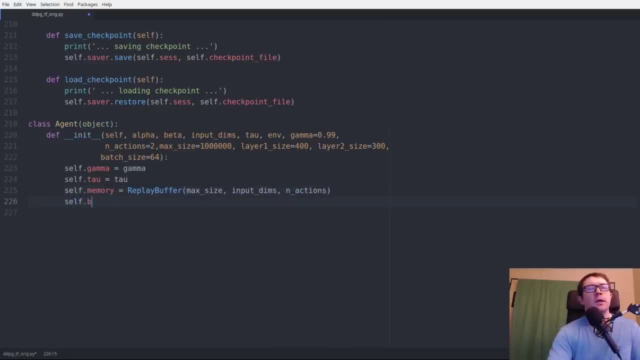 number of actions. We will need a batch size. Here's where we're going to store the session, And this is so that we have a single session for all four networks And I believe- Okay, Now I believe- don't quote me on this, but uh, I tried it with an individual network. 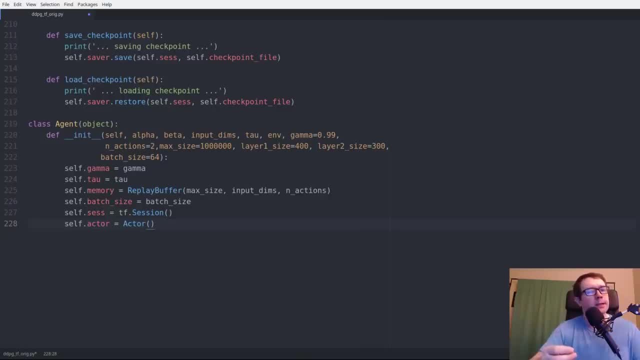 for, sorry, an individual session for each network, And it was very unhappy when I was attempting to copy over parameters from one network to another. I figured there was some scoping issues. uh, so I just simplified it by having a single session. 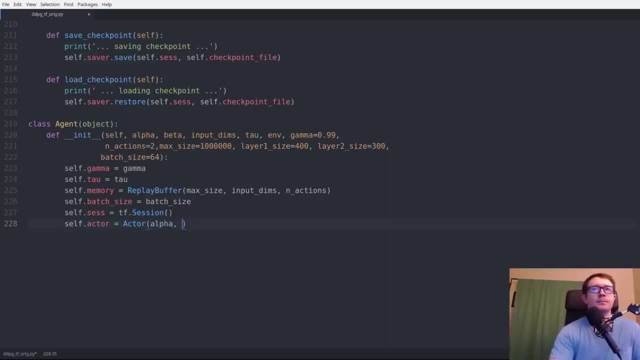 There's no real reason that I can think of to have more than one. And that is an actor that gets uh alpha number of actions. The name is just actor. Input dims The session layer. one size layer. two size action space dot high. and that's our action. 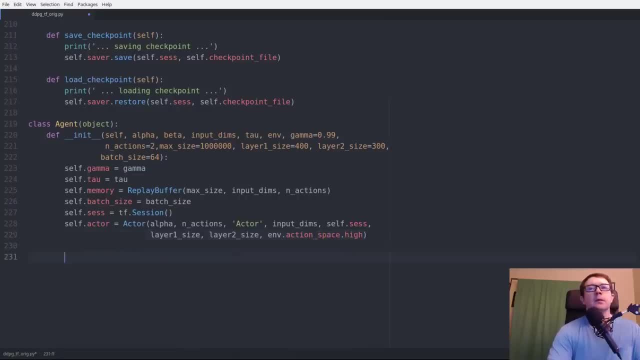 bounds: The action space dot high. Next we have a critic that gets beta and actions. Its name is just critic but dims self dot session. layer one size, layer two size: action space dot high. And that's our action bounds. 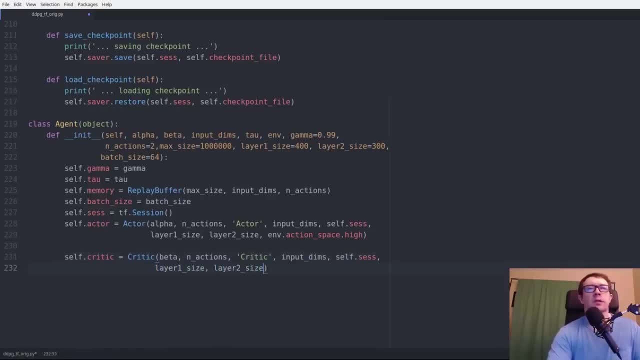 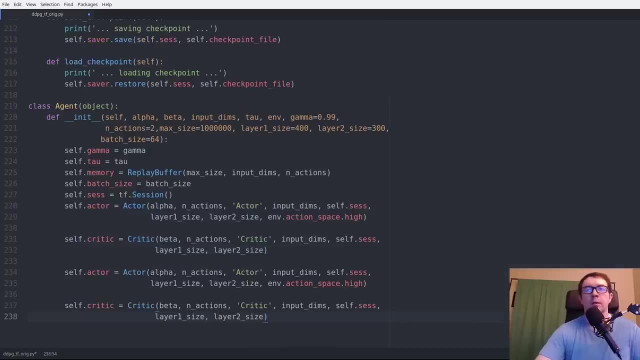 The action space dot high. Next we have a critic. It's a size layer, two size action. We don't pass in anything about the environment there. Now we can just copy these And instead of actor, it is target actor. 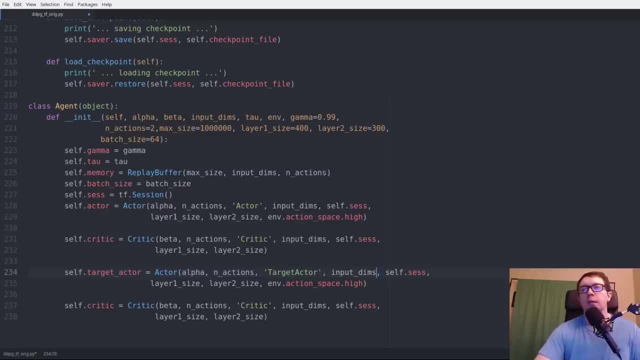 And let's go ahead and clean up and be consistent with our PetFate style guides- Always important- That actually makes you stand out. I've worked on projects where the manager was very, very helpful. So every time you come up with an action, you measure the object. 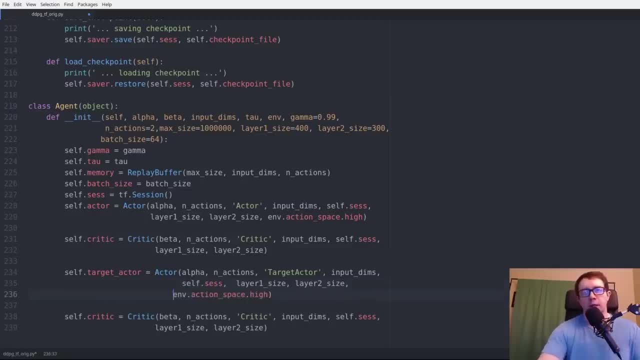 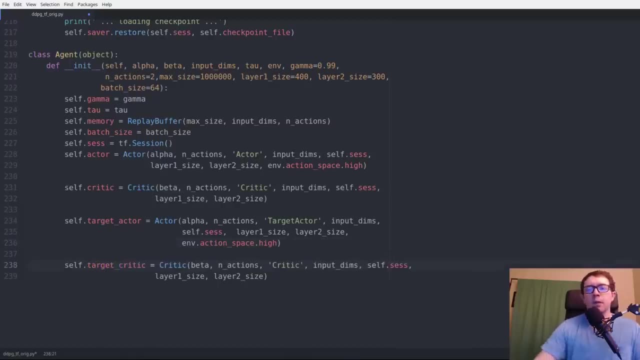 The way we did that, I was able to keep the object in and it was, you know, very, very clear, quite happy to see that i had a somewhat strict adherence to it. just something to take note of. so then we have a target critic as well. 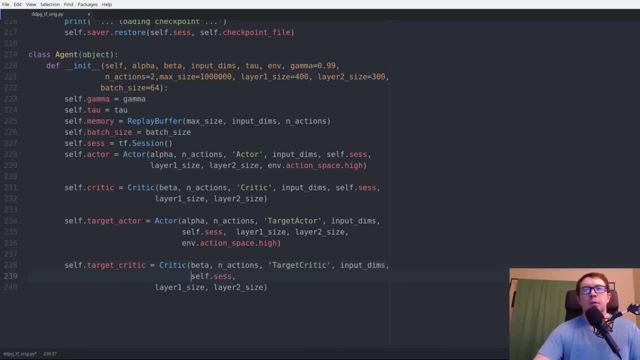 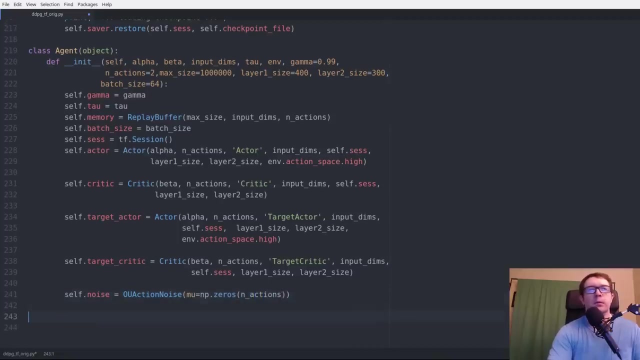 and we will clean up this. and so that is all four of our deep neural networks. that's pretty straightforward. so now we need noise that's an ou action noise with mu equals numpy zeros in the shape and actions. so now we need operations to perform the soft updates. so, uh, the first time i tried it. 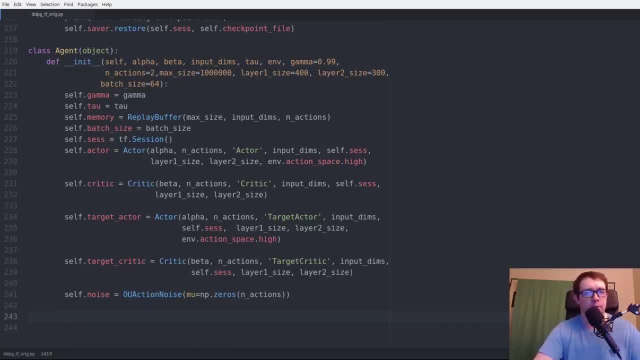 i defined it as its own separate function, and that was a disaster. it was a disaster because it would get progressively slower at each soft update, and i don't quite know the reason for that. i just know that that's what happened, and so when i moved it into the initializer and 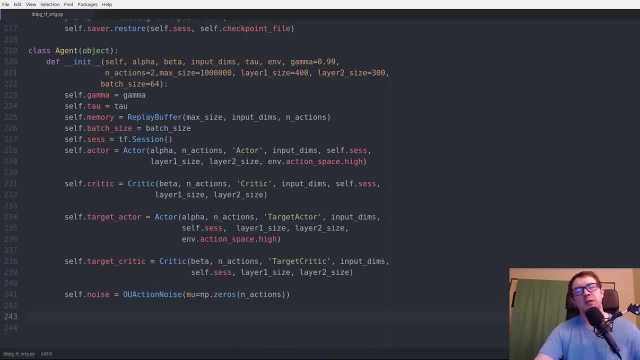 defined one operation. i'm guessing it's because it adds. every time you call it it probably adds something to the graph, so that adds overhead to the calculation. that's my guess. i don't know that's accurate. it's just kind of how i reasoned it. but anyway, let's go ahead and define our update. 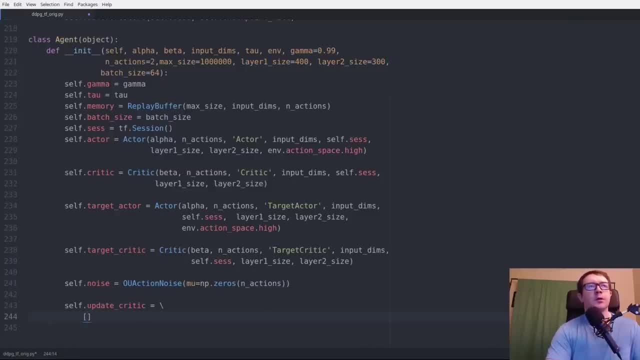 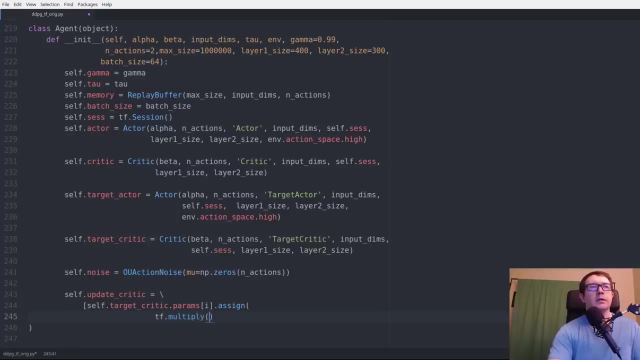 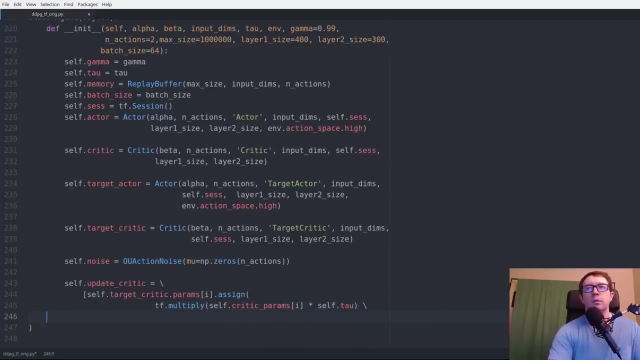 operations here. so what we want to do is iterate over our target critic parameters and call the assignment operation. what do we want to assign? we want to assign the product of critic params and self dot tau plus gif dot multiply self dot. target critic params sub i times or and. um, now that should be a sorry, a comma comma and one minus cell dot tau. 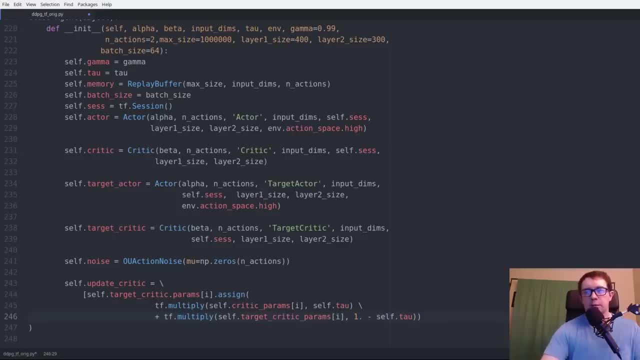 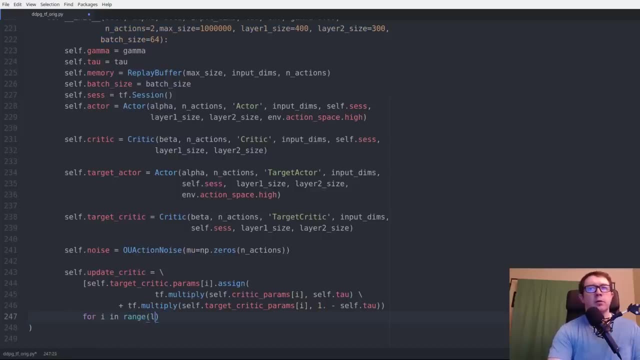 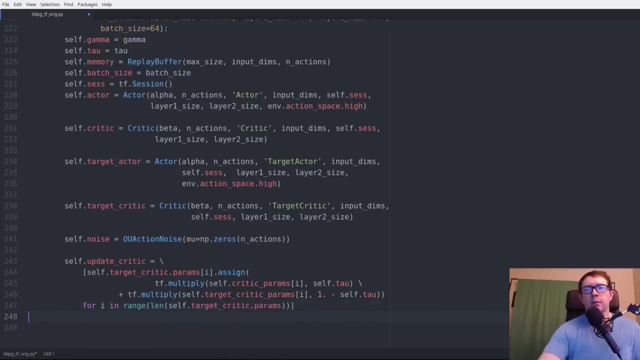 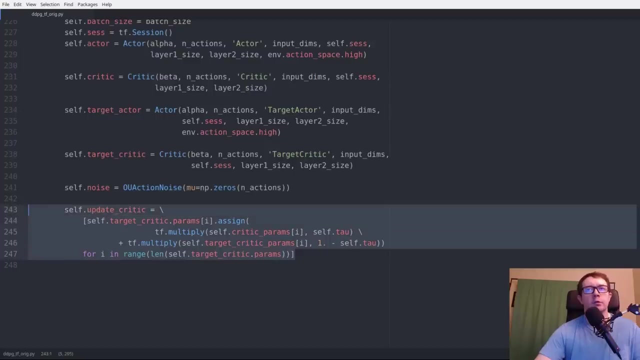 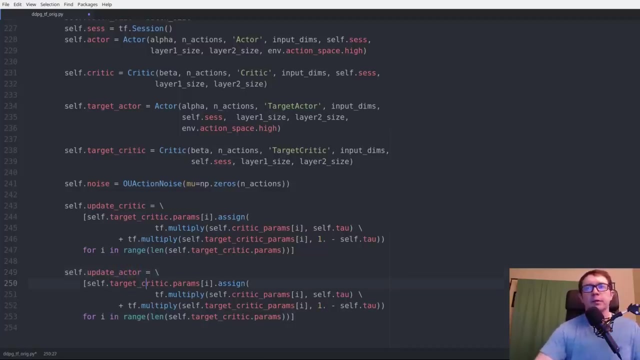 so we get two. let's hit that, and that is a list. comprehension for i in range length of target critic dot params. now it's that you don't need that? i don't believe, no. so then we have a similar operation for the actor. we just want to swap actor and critic target actor. so dot actor, uh, actor dot params, dot params. 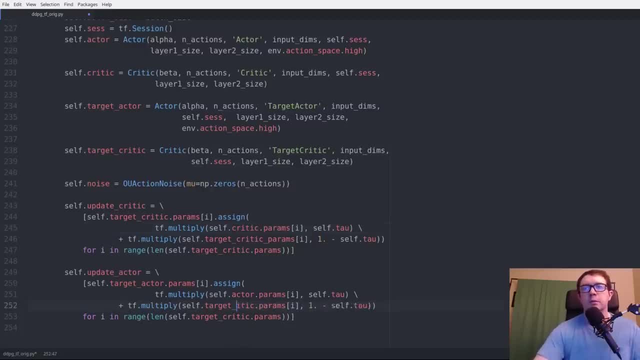 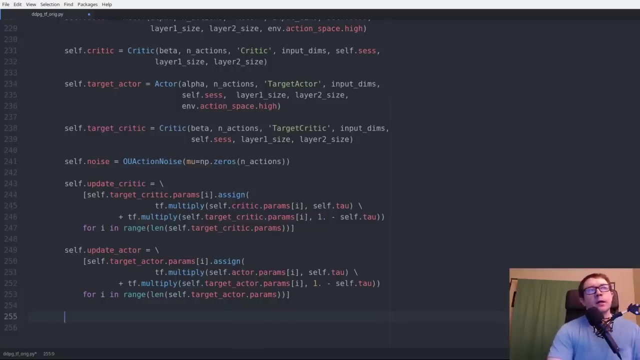 i did the same thing here, didn't i target actor and up here dot params. okay, target actor, actor and then target actor there. so now we have our update, soft update operations according to the paper. finally, we have constructed all the graphs. uh, you know, for the whole. 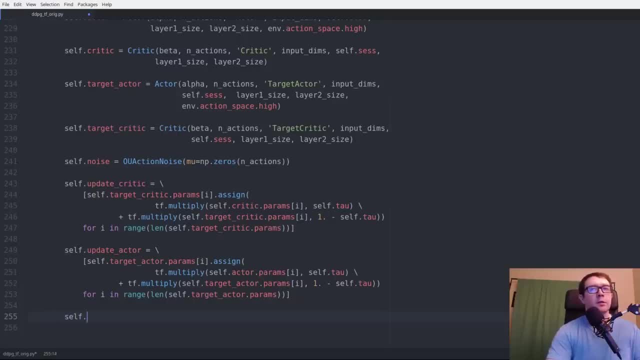 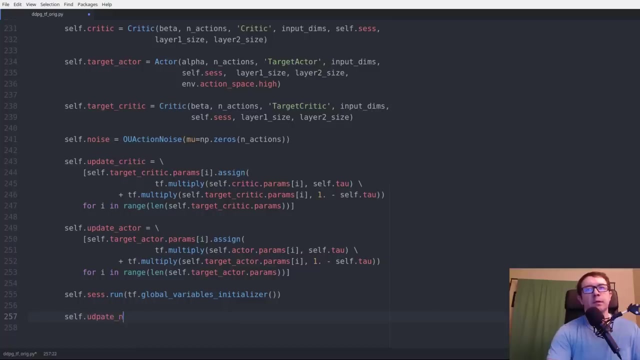 four networks. so we have to initialize our variables, selfsessionrun tf global variables initializer. you can't really run anything without initializing it and, as per the paper, at the very beginning we want to update the network parameters and at the beginning we want to pass in the 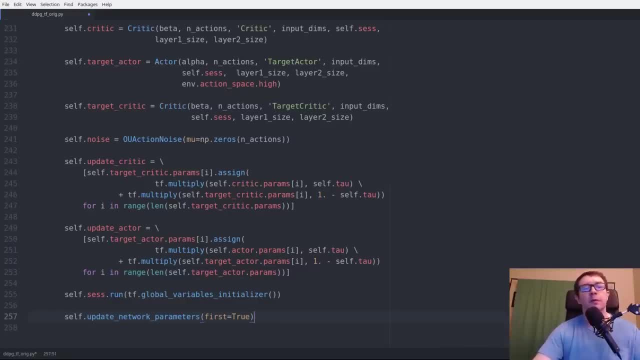 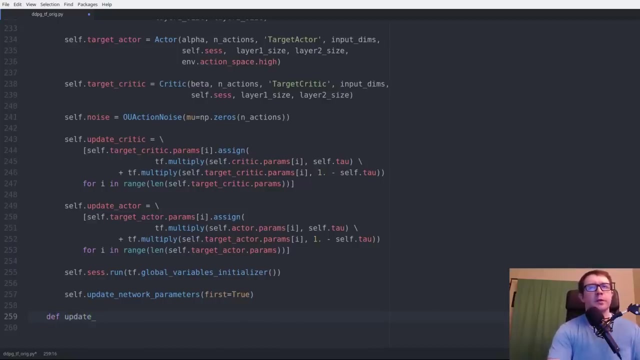 we want the target networks to get updated with the uh, full ver, the full value of the critic of the evaluation networks, and so i'm passing in a parameter of first equals true. so since it's confusing, let's do that first. that function first. update network parameters. 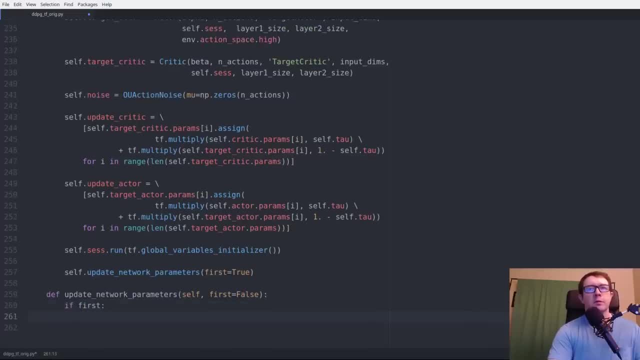 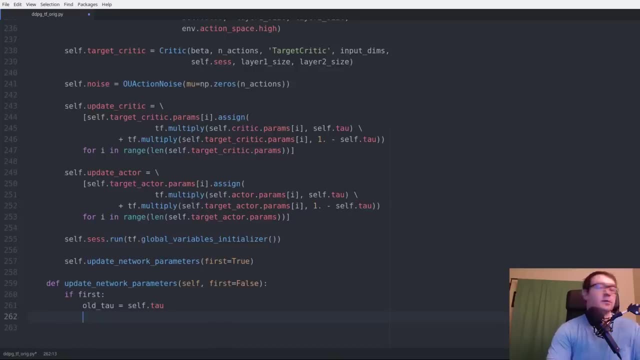 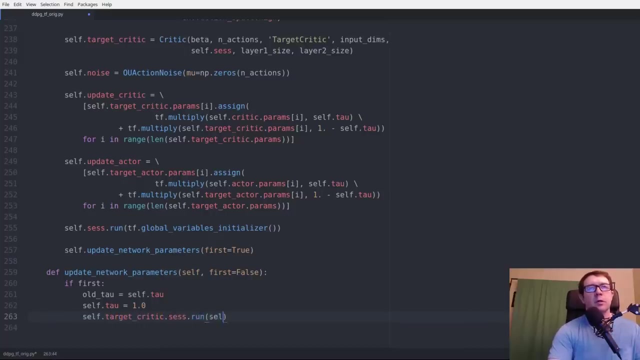 first we'll default to false. so if first we need to say old tau equals self dot tau, i need to save the old value of tau to set it again so that i can reset it. so that's how it goes. one and say selftarget, criticsessionrun, update, critic- selftargetactorsessionrun. 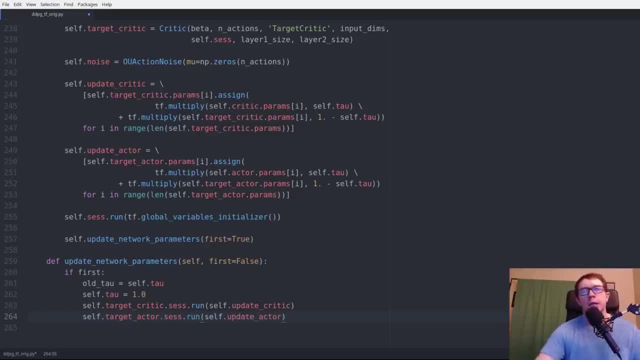 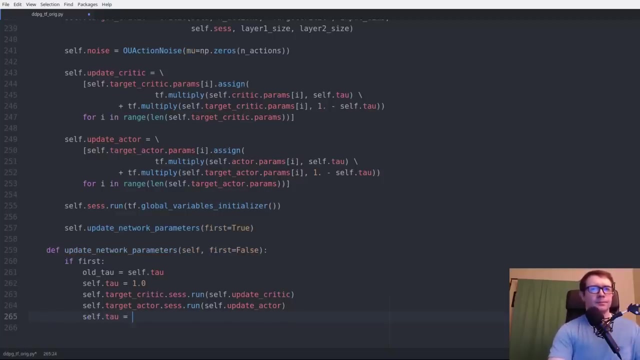 selfupdate actor and, as i recall- this is important- which session you use to run the um update, although maybe not, since i'm using only one session. if you want to play around with it, go ahead and then go ahead and reset the tau to the old value, because you only want to do this. 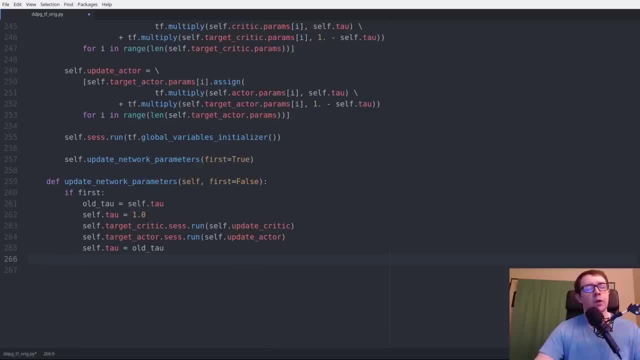 particular update where you update the target network with the original network: full values on the first term, on the first, go through, otherwise just go ahead and run the update. so next, we need a way of storing transitions: self state, action, reward, ah, new state, and done you so? selfmemorystore transition: you want to store all this stuff? this is just an interface. 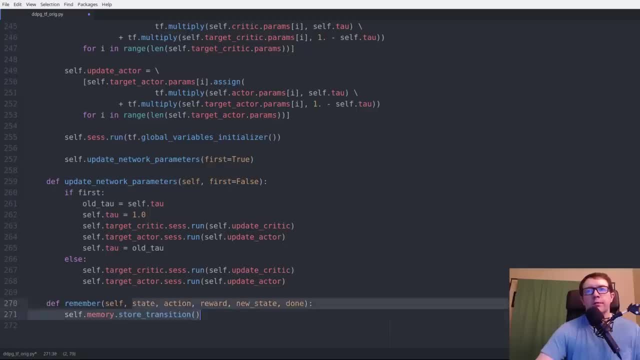 from one connection to another, so i'll stop here. this says spacing time, so stop there, because what i'll stop there is thisiking leave. we want to stop this call there. we have to do myself, stay, so i'm. this is just an interface from one class to another. you know, this may or may not be great. 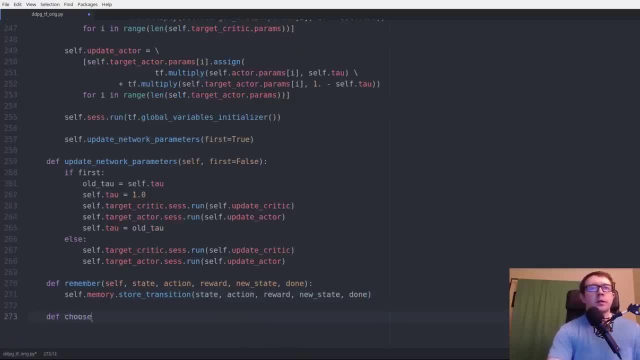 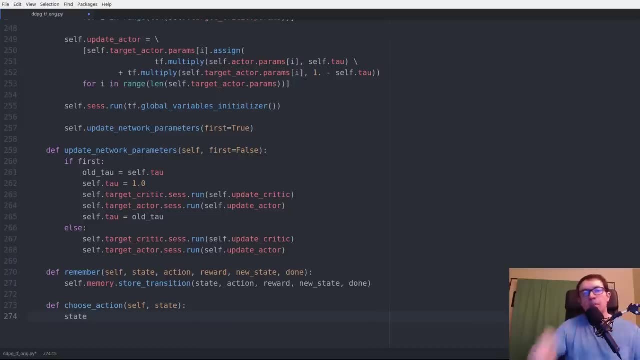 computer science practice, but it works. next, we want a way of choosing an action, and that should take a state as input, since we have defined the input variable to be shaped- batch size- by- and actions. you want to reshape the state to be one by- sorry, it should be one by the observation. 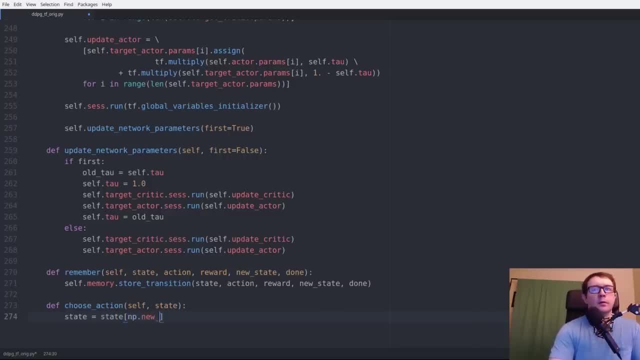 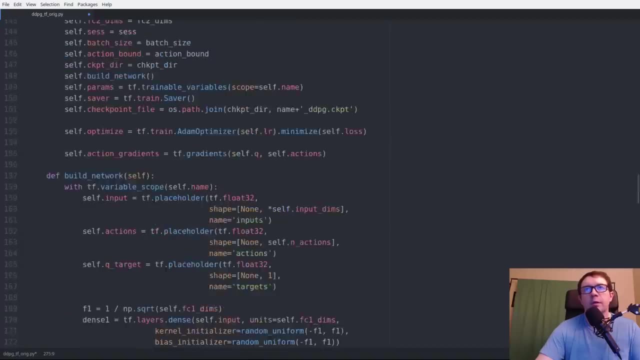 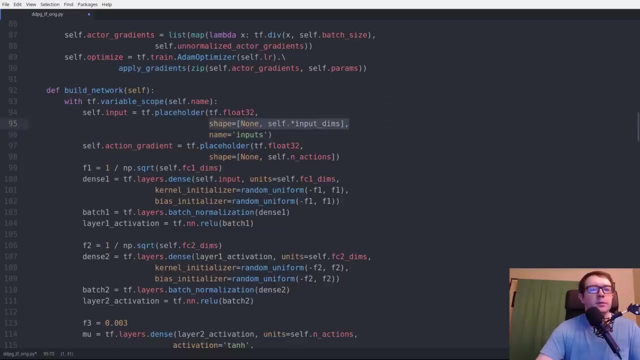 space, new access, all and that's because we have the come up here for the actor network. just so we're clear. it is because this has shaped none by input dims. so if you just pass the in the observation vector, that has shape input dims and it's going to get. it's going to get. 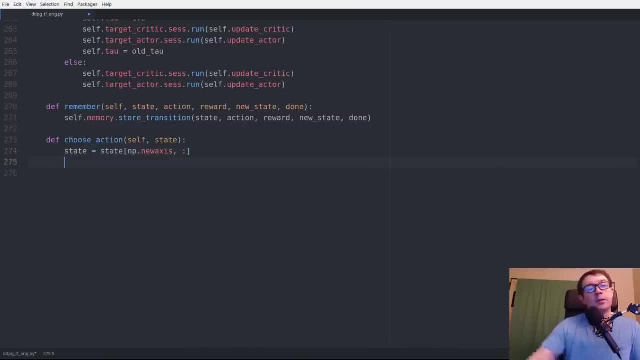 uppity with you. so you just have to reshape it because you're only passing in a single observation to determine what action to take. so mu actor dot predict state noise equals self dot noise. mu prime equals mu plus noise. return sub zero. so this returns a tuple. so you want the zeroth element. 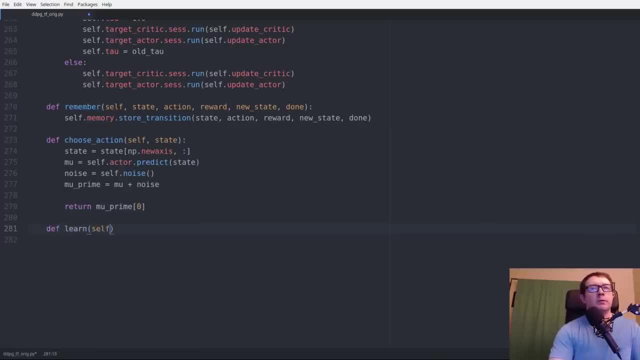 so now we have the learning function and of course this is where all the magic happens. so if you have not filled up the memory, then you want to go ahead and bail out. so otherwise you want to go ahead and sample your memory. so if that memory does sample, buffer batch size. 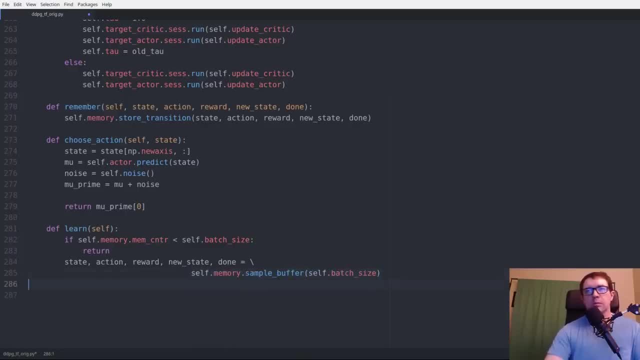 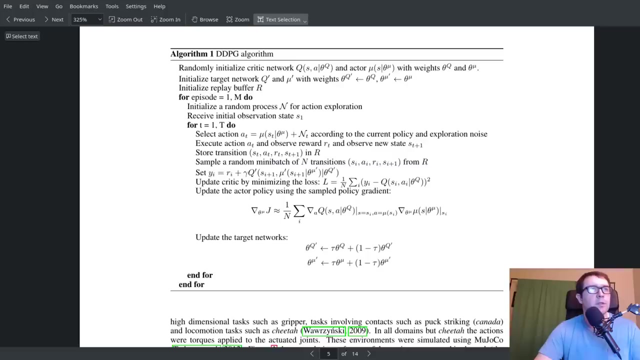 so next we need to do the update from the paper. so let's go back to the paper and make sure we are clear on that. so we need to- uh, we already sampled this- so we need to calculate this, and to do that we're going to need the q prime, the target critic network. 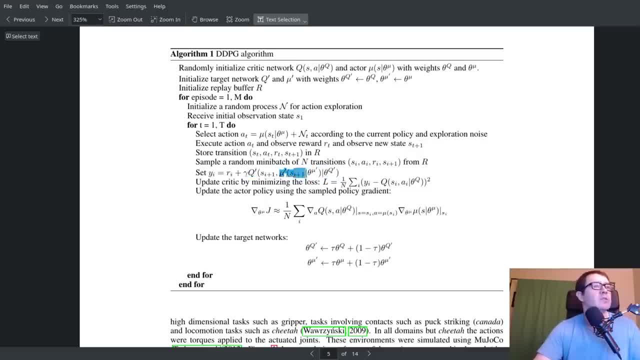 as output, as well as the output from the target actor network, and then we use that to update the loss for the critic and then we're going to need the output from the critic as well as from the actor network. so we need to basically pass states and actions through all four networks to get 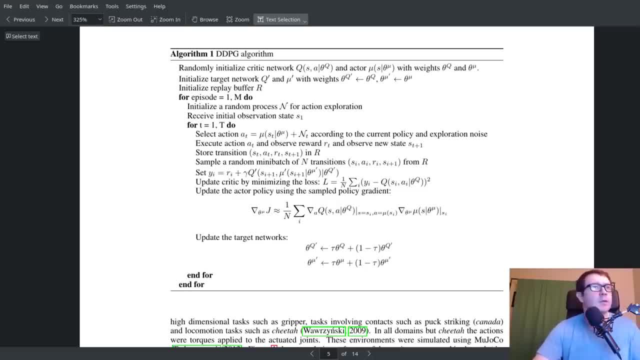 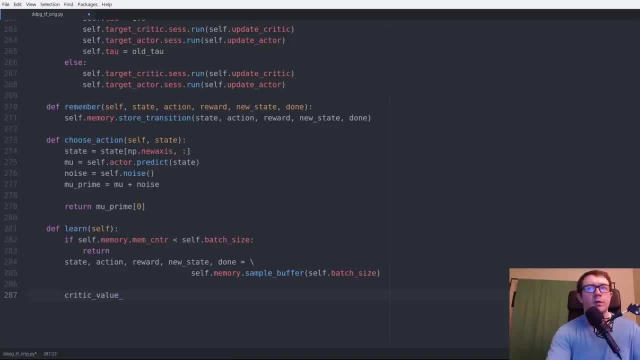 the training function, the learning function. So let's go ahead and head back to the code editor and do that. So our critic value for q prime. so q critic value, underscore, sublet, target, critic, predict. and you want to pass in the new states And you also want to pass in the actions that come. 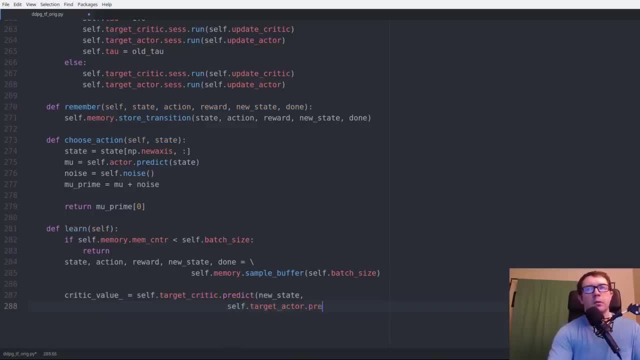 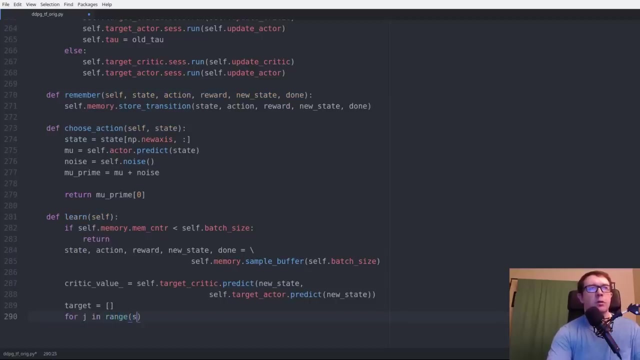 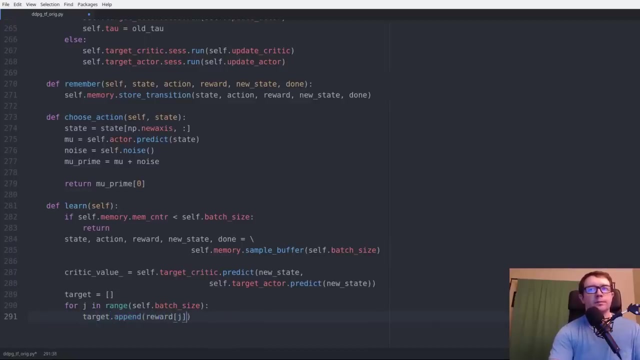 from the target actor: New state. I need one extra parentheses there. So then we want to calculate the y sub i's for the targets. So that's an empty list for j and range. So the batch size, target, dot, append reward Critic value underscore j. 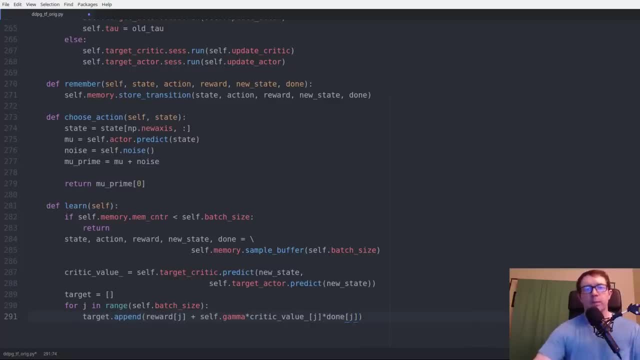 Times done sub j, And that's where the kept harping on getting no rewards after the terminal state. That's where that comes from. When done is true, then it's one minus true, which is zero. So you're multiplying this quantity by zero, So you don't take into account the value of the next. 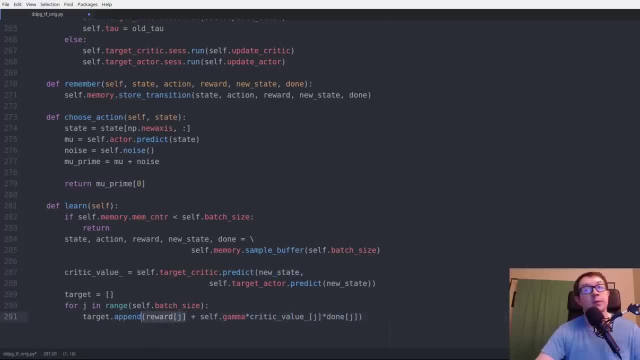 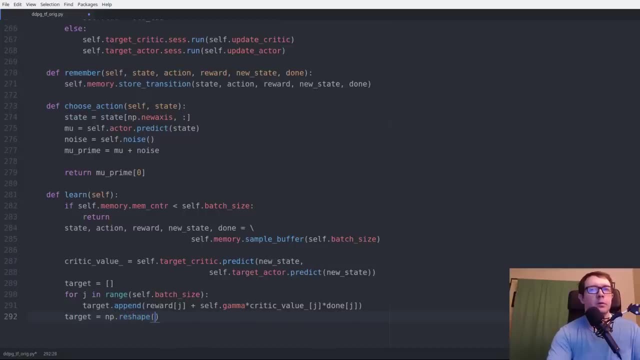 state right, which is calculated up here. you only take into account the most recent reward, as you would want. So then, we just want to reshape that Target into something that's batch size by one. that's to be consistent with our placeholders. 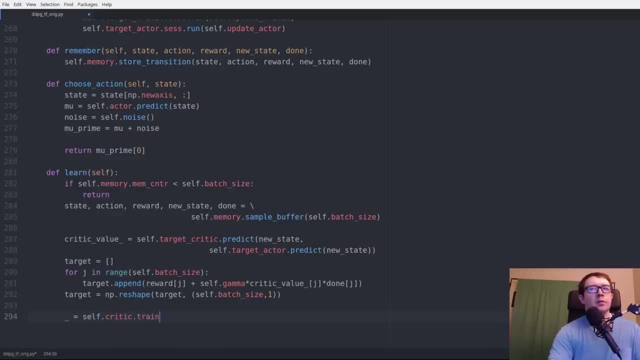 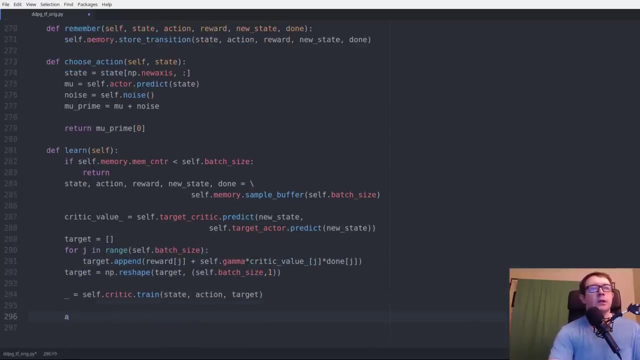 And now we want to call the critic train function Right, because we have everything we need. we have the states, actions and targets, with states and actions from the replay buffer and the target from this. calculation here Very easy. Now we need to do the actor update. So 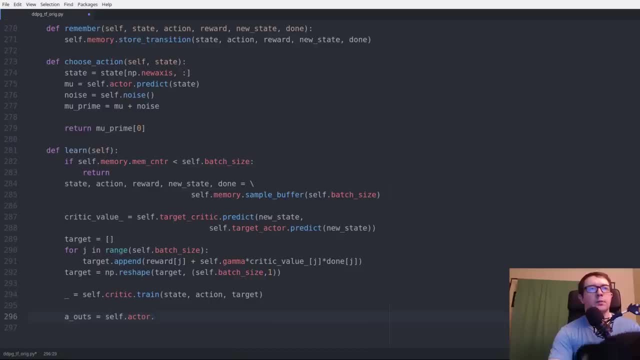 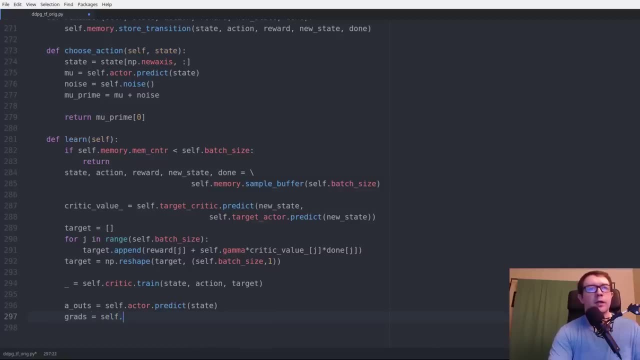 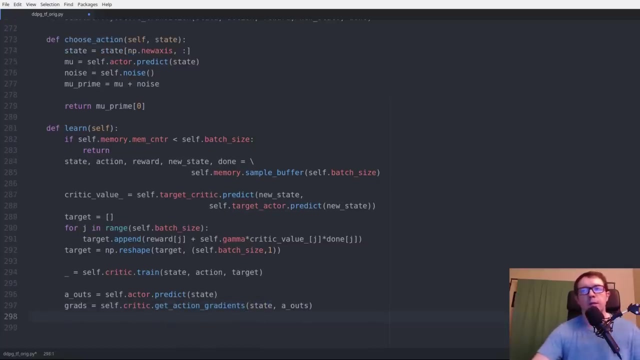 the action outs, dot actor, dot predict. we get the predictions from the actor for the states, our grads, the gradients get action gradients, state a outs that'll get the remember, that'll do a feed forward and get the gradient of the critic with respect to the actions taken. And then you want. 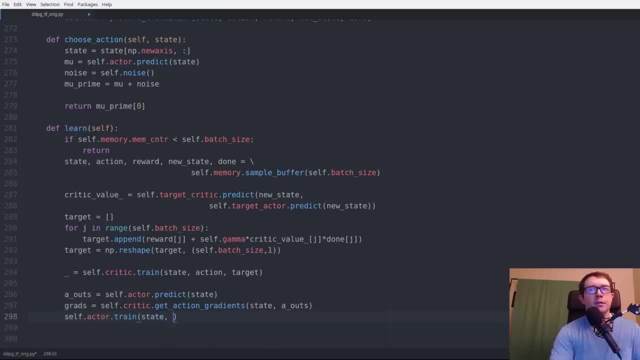 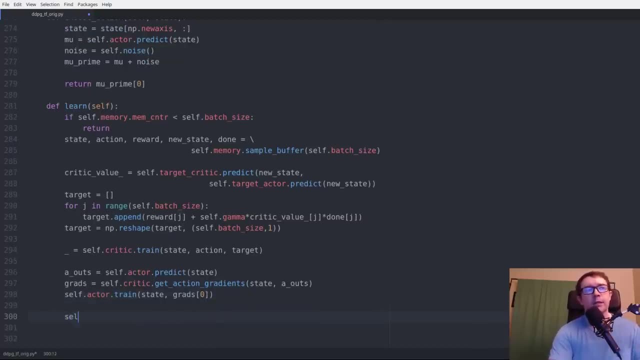 to train the actor state and grads the gradients. It's a tuple, so you want to dereference it and get the zeroth element. And then, finally, you want to update network parameters. Okay, so that is it for the learn function. Now we have two other bookkeeping functions to handle. 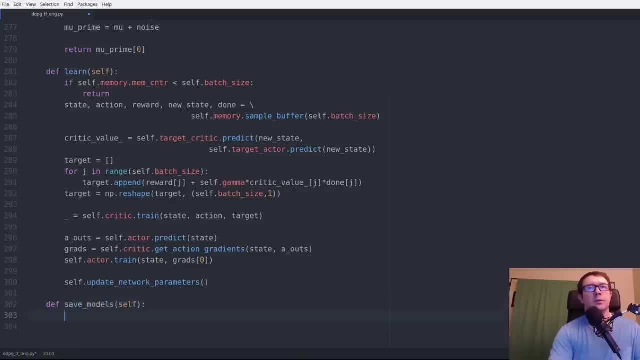 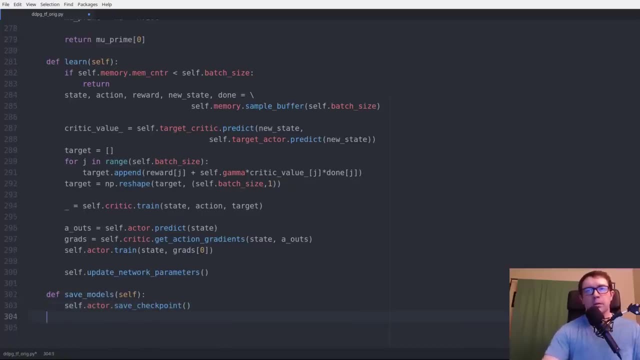 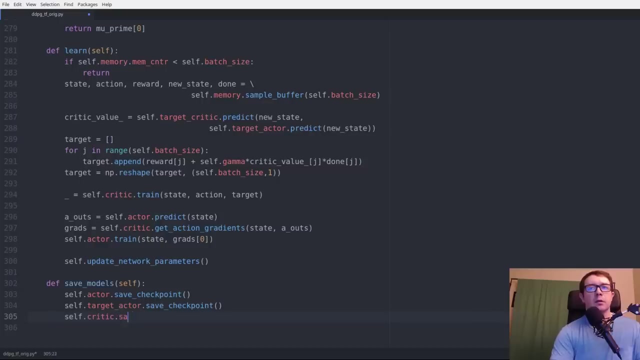 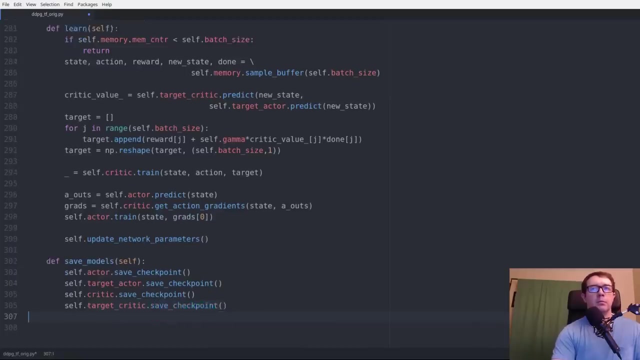 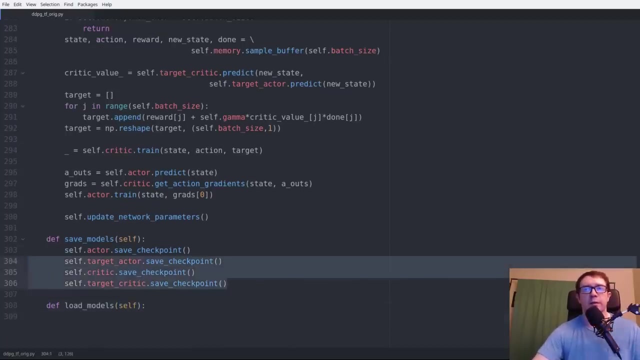 which is save models, And this will save all of our models. So self dot actor dot save checkpoint, self dot target actor- save checkpoint, self dot critic and a function to load models. Sounds like a dog find out there. So we want to load checkpoints instead of saving them. 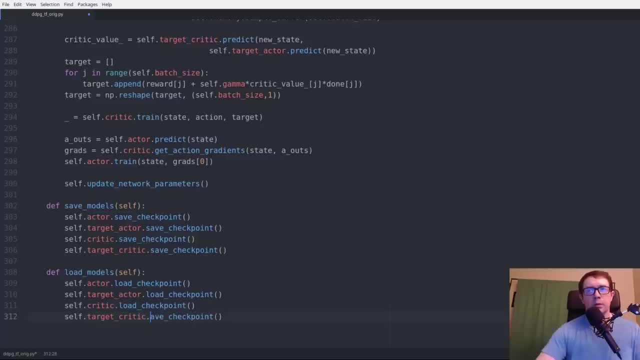 Oh, checkpoints, load and load. So that is it for the agent class. It only took about an hour, So we're up to about two hours for the video, So longest one yet. So this is an enormous amount of work. This is already. 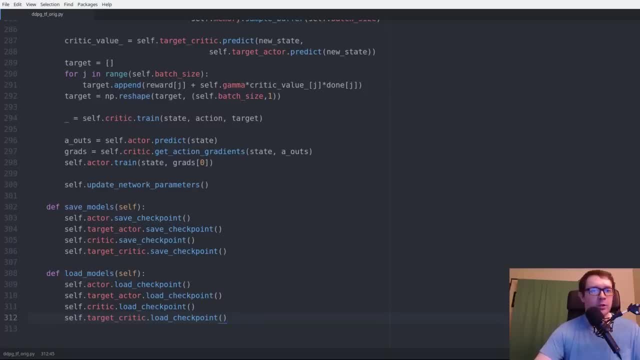 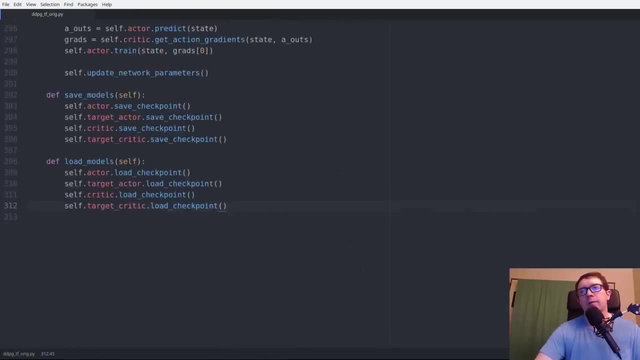 310 lines of code. If you've made it this far, congratulations. This is no mean feat. This took me a couple weeks to hammer through, but we've gotten through it in a couple hours. So this is all there is to the implementation. 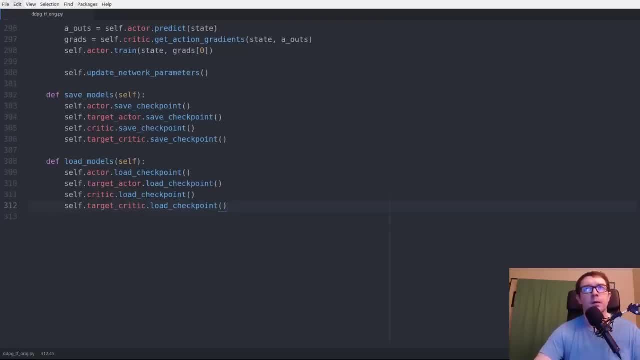 Now we have to actually test it. So let's open up a new file And save that as main TensorFlow dot pi. And what we want to do now is go ahead and test this out in the pendulum environment. Call it TensorFlow original. 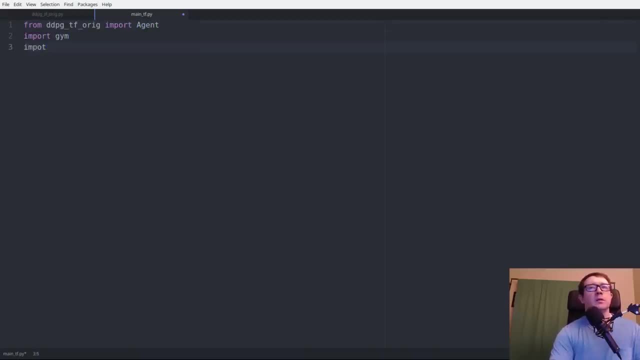 Import our agent. we need Jim, we need- do we need numpy for this? Yes, we do, We need. we don't need TensorFlow from utils import plot learning And we don't need Oh s, So we will have a score history. I know what I want to do, that Let's. 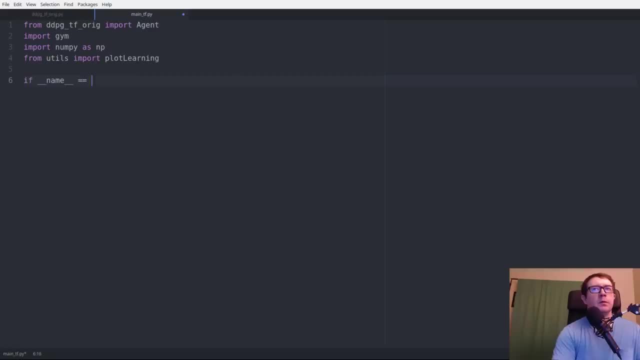 save Name equals mean. Now we want to say in v gym dot make pangu Lomb dash v. zero agent equals agent gets learning rate of 0001.. beta of T 0.. z 0.. of zero one input dims three. it was three tau zero one pass in our environment. 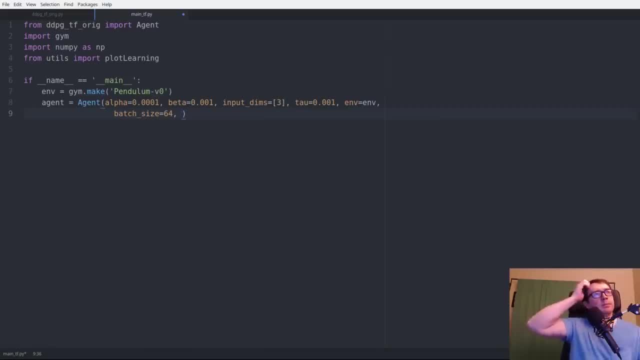 batch size 64. i'm being verbose here and it looks like when i ran this i actually used different layer sizes. well, that's an issue for hyper parameter tuning. i just want to demonstrate that this works and actions equals one. so when i got good results for this, i actually used 800 by 600. 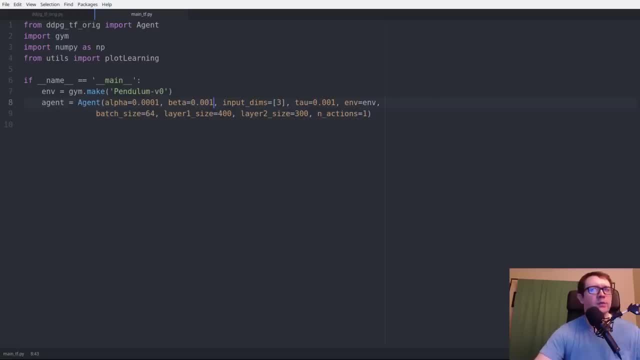 and i cut these learning rates in half, but we'll go ahead and use the values from the paper. sometimes i do hyper parameter tuning. other thing we need to do is set our random seed. you know, we can just put it here. whatever the reason we want to do this is for replicability and i have yet to see an. 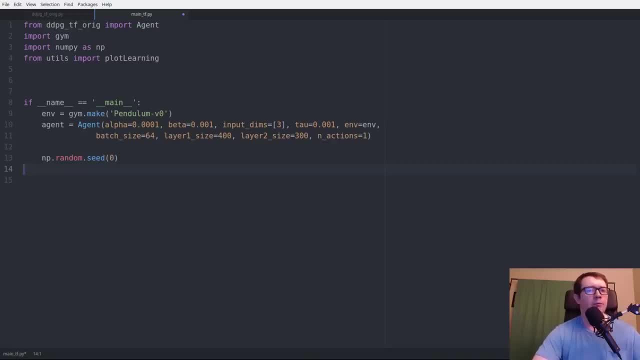 implementation of this where they don't set the random seed- and i've tried it without it and you don't get very good sampling of your replay buffer. so this seems to be a critical step and most implementations i've seen on github do the same thing. so let's go ahead and play. 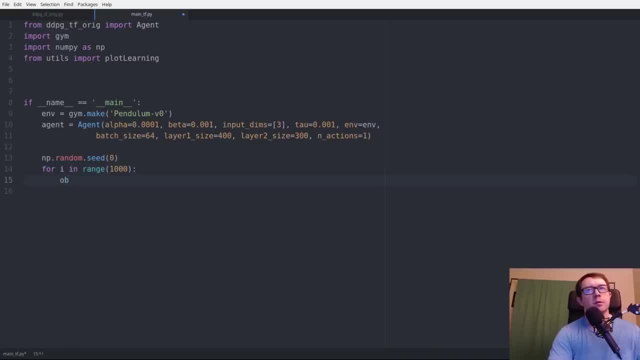 our episodes say: a thousand games envy that reset. we forgot our score history, of course. that's to keep track of the scores over the course of our games. done is false and the score for the episode is zero. let's play the episode. say act, agent, I choose action. takes OBS as input. 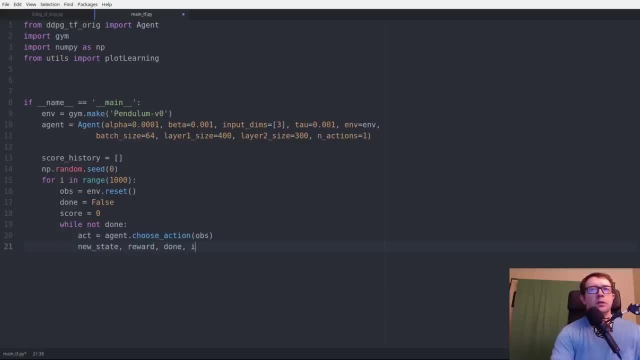 new state: reward done. info equals the envy dot. step act agent dot. remember Hobbes. act reward: new state and done. I guess the int done really isn't necessary. we take care of that in the replay buffer fun class. but you know, doesn't hurt to be explicit. and then you want to. 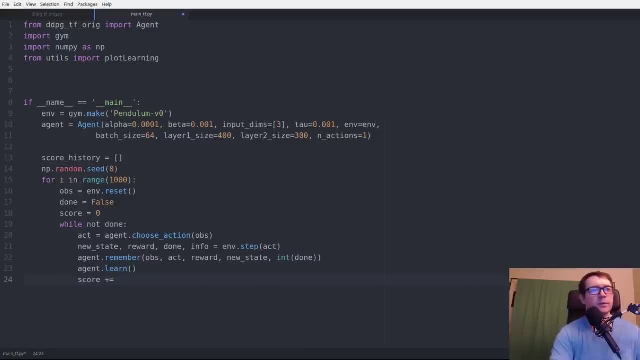 we want to learn on each time step, because this is a temporal difference method. keep track of your score and set your old state to be the new state, so that way we need to use an action on the next step. you are using the most recent information. finally, at the end of the episode we're going to 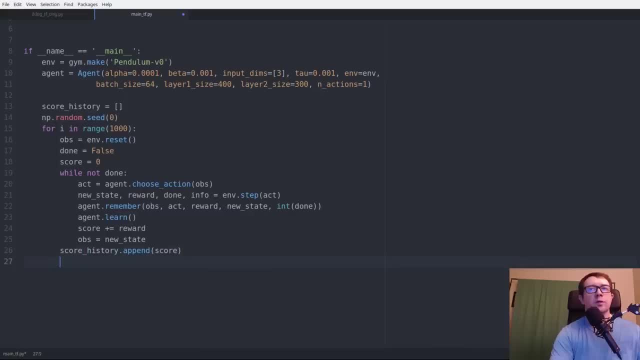 end of every episode you want to append that score to the score history and print episode. I score percent up to F score 100 game average percent out to F percent- I'm PI mean score history last hundred games minus 100 on one more and at the end equals pendulums dot png. thought learning. 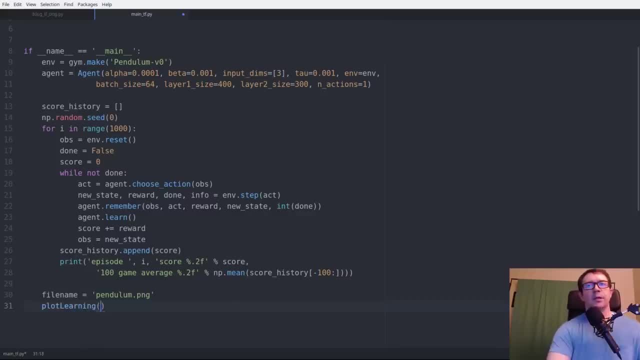 thought learning score history, file name and a window of 100. the reason I choose a window of 100 is because many environments define uh solved as trailing 100 games over some amount. the pendulum doesn't actually have a solved amount, so what we get is actually on par with some of the best results. people 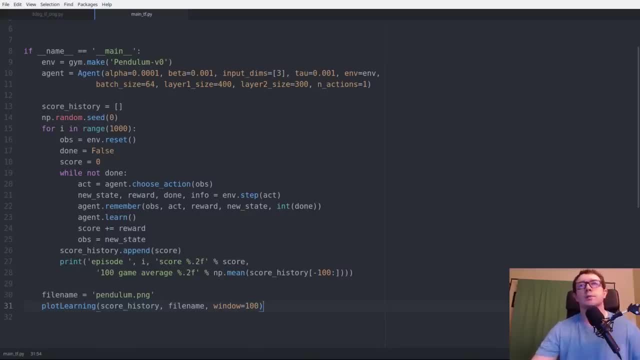 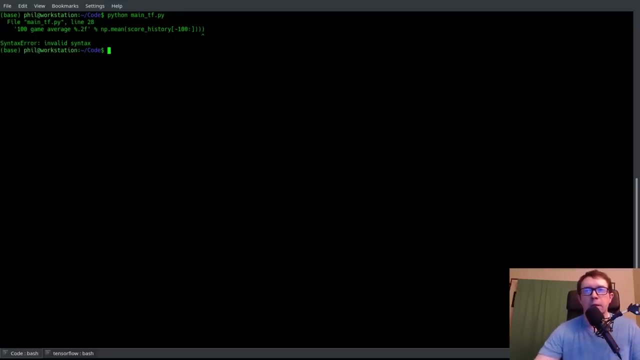 have on the leaderboard. so it looks like it does pretty well. so that is it for the main function. let's go ahead and head to the terminal and see how many typos i made. all right, here we are. let's go ahead and run the main file. uh, invalid syntax. i have an extra parenthesis. i'm just going to. 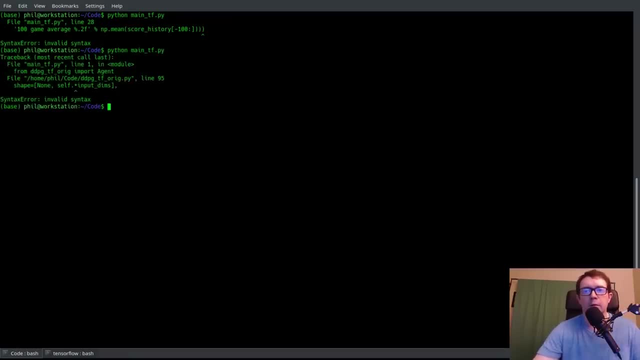 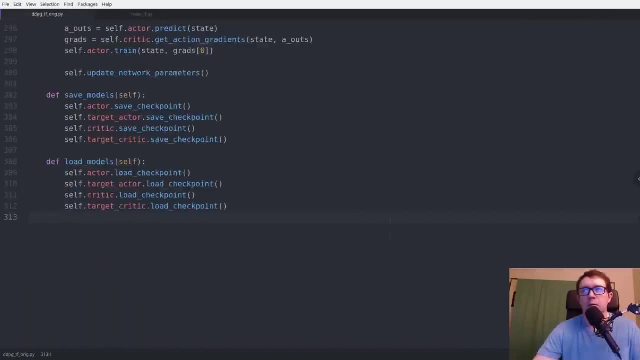 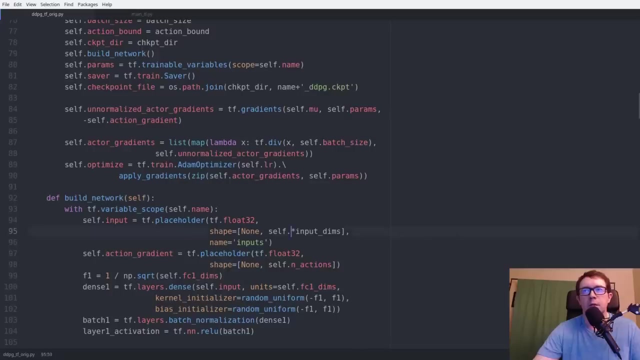 delete that really quick. run that. uh, i have the star out of place. let's go back to the code editor and handle that. so it looks like it is online 95, which is here. all right back to the terminal. all right back to the terminal. let's try it again. 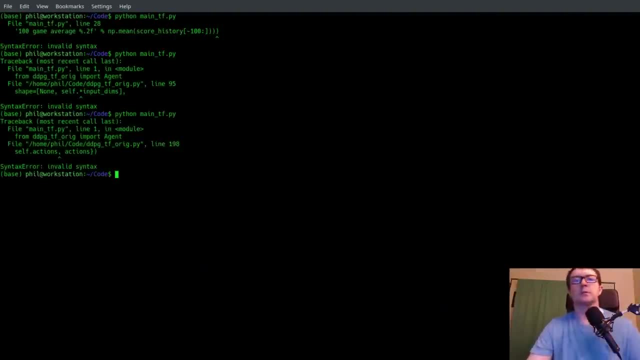 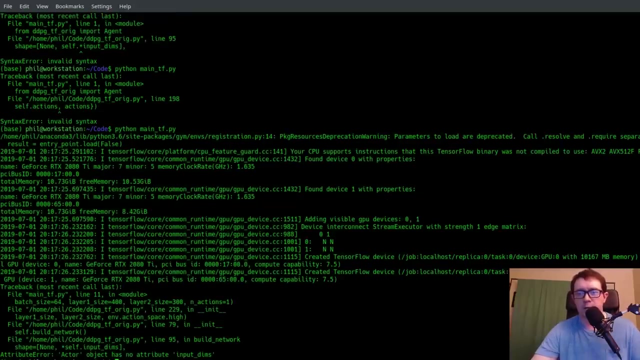 and it says: line 198: invalid syntax. oh, it's because it's a comma instead of a colon. all right, i'll fix that once more. all right, so that was close. so actor object has no attribute input. dims. line 95. ah, okay, that's easy, let's head back so it's in line 95. 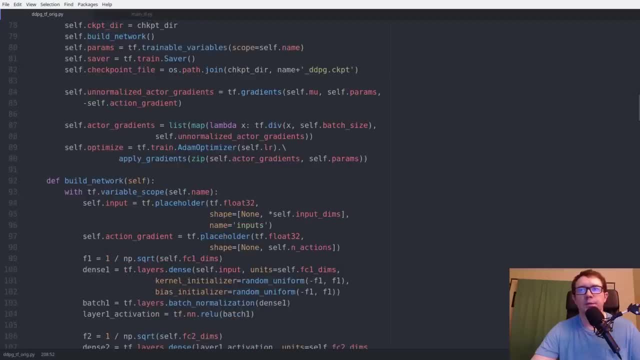 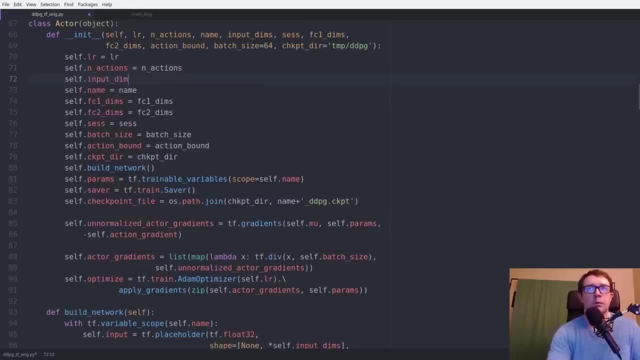 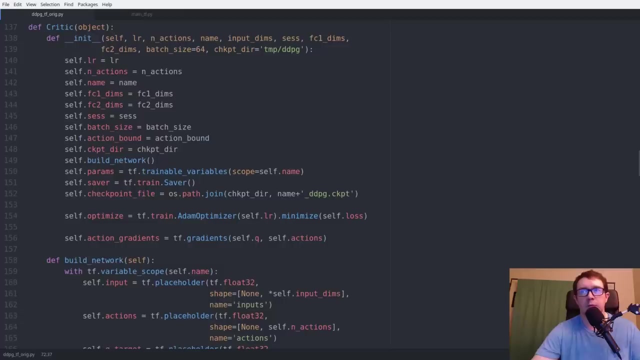 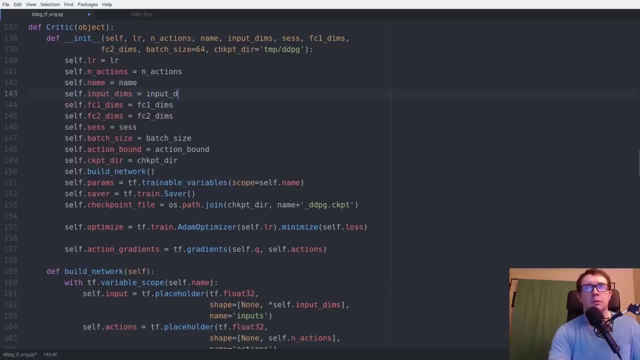 it just means i forgot to save input dims, and that probably means i forgot it in the kritik as well, since i did a cut and paste. uh, yes, it does. all right, now we'll go back to the terminal. hopefully that's the last one. all right, momentary. 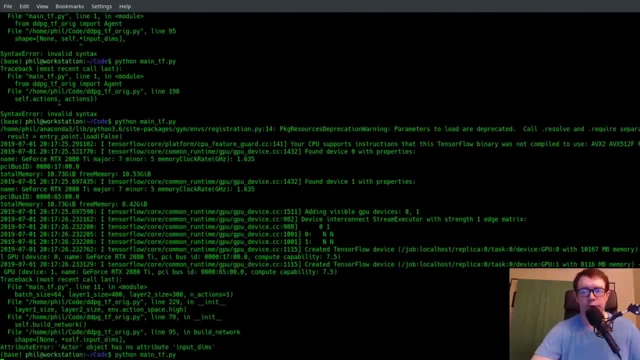 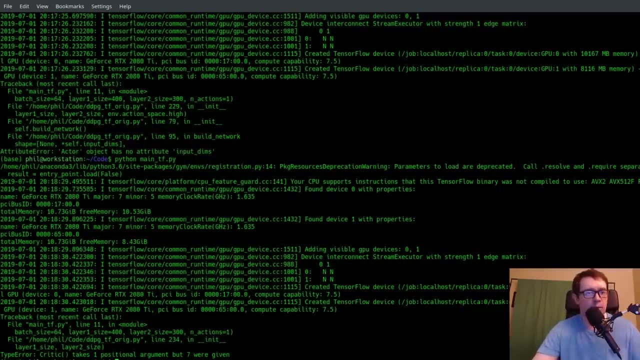 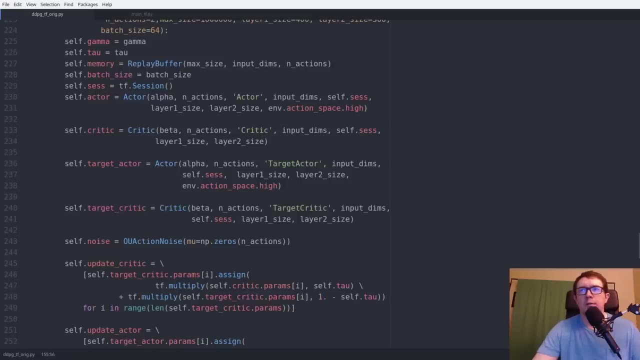 salvation dawn error. error table: возвращado a la poderasa. Moment of truth: Critic takes one positional argument, but seven were given Good grief. Okay, one second. So that is of course in the agent function. So I have line 234. 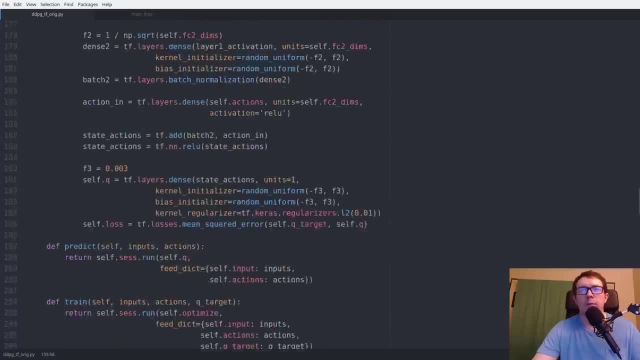 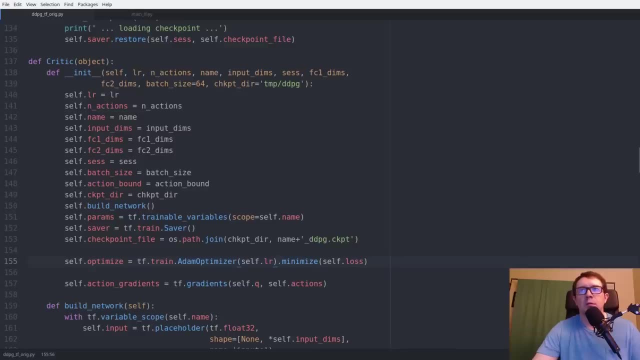 One, two, three, four, five, six, seven parameters indeed. So critic takes learning rate. number of actions. name input, dim session Interesting One, two, three, four, five, six, seven. What have I done? 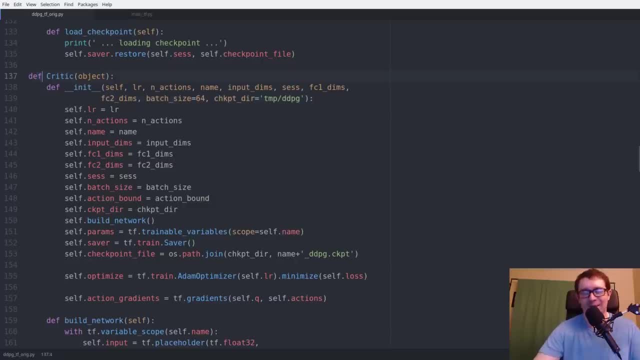 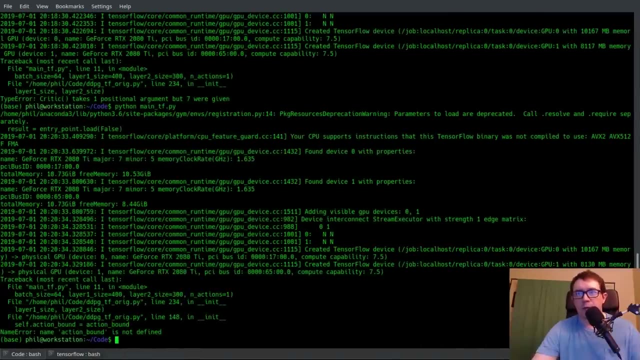 Oh ha, that's why It's class critic, of course. All right, let's go back to the terminal and see what happens. Name action bound is not defined And that is in the line 148.. Okay, line 148.. 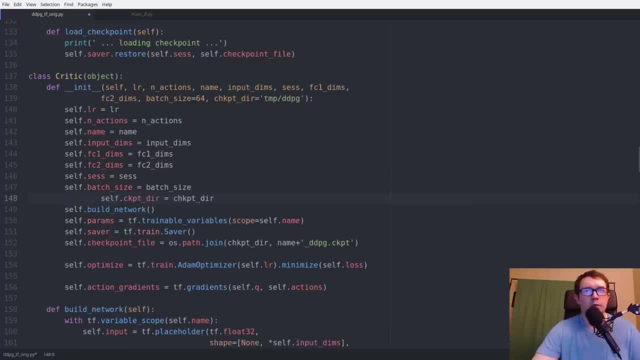 That is in the critic. Ah, that's because I don't need it there, Let's delete it. That was just for the actor. It's because I cut and pasted- Always dangerous. I tried to save a few keystrokes to save my hands. 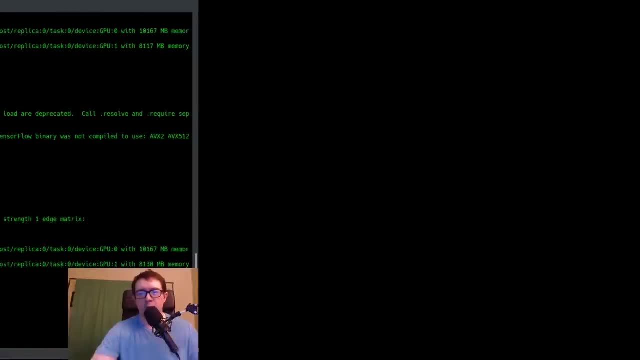 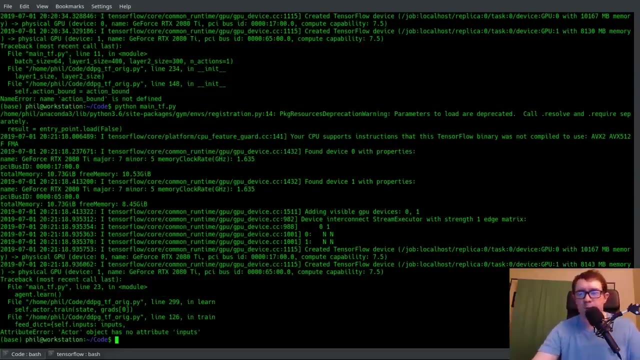 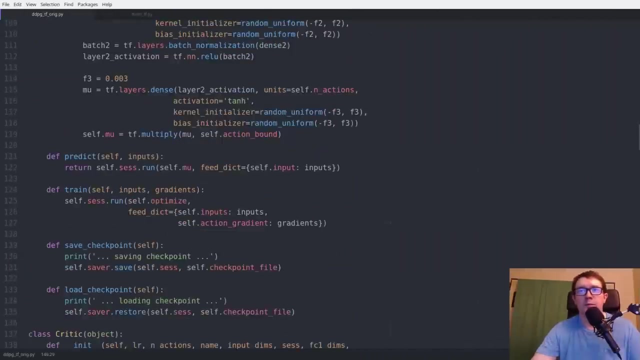 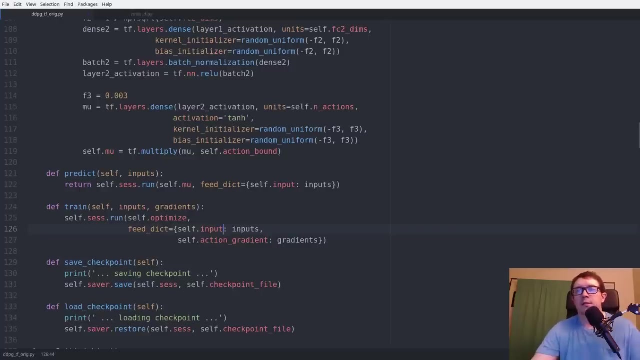 and ended up wasting time instead. All right, let's go back to the terminal. All right? Actor has no attribute inputs. That is on line 126.. Selfinputs- Selfinputs. It's probably selfinput. Yes, That's why. 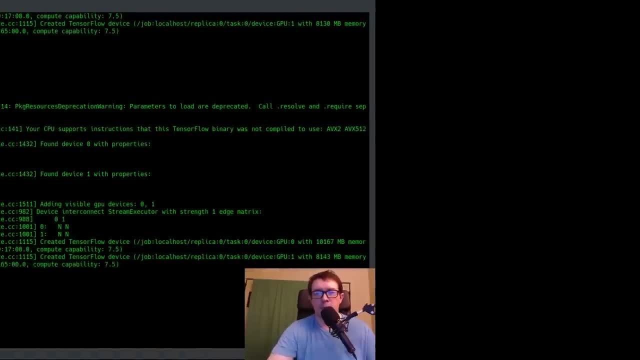 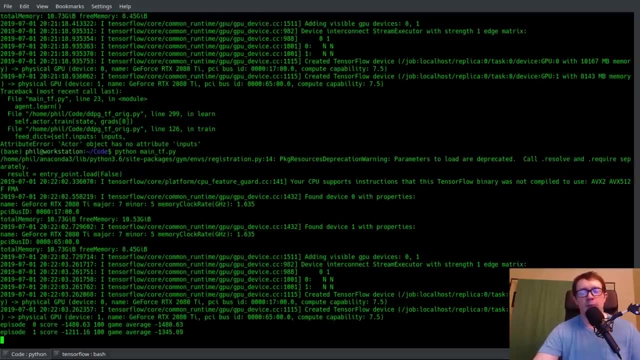 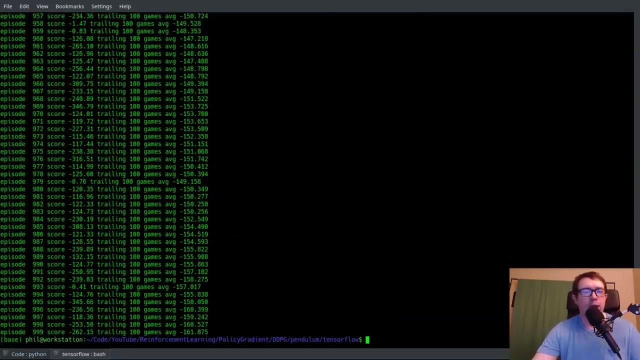 I do the same thing here. Okay, Perfect, and it runs. So I'll let that run for a second, but I let it run for 1,000 games earlier and this is the output I got Now. keep in mind it's with slightly different parameters. 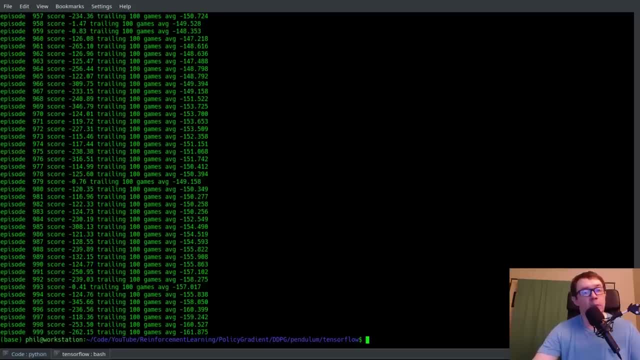 The point here isn't that whether or not we can replicate the results, because we don't even know what the results really were, because they express it as a fraction of the performance of a planning agent, So who knows what that really means. I did a little bit of hyperparameter tuning. 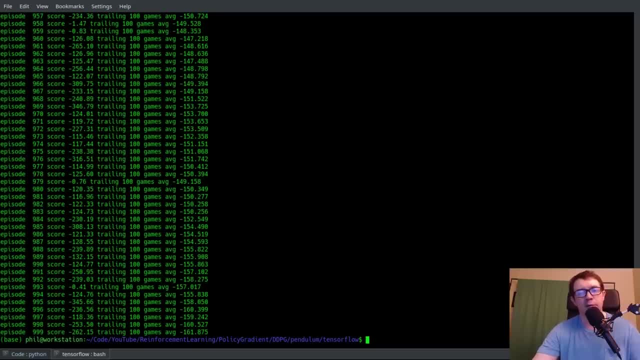 All I did was double the number of input units and halve the learning rate and I ended up with something that looks like this, So you can see it gets around 150 or so steps. It gets around 150 or so steps to solve. 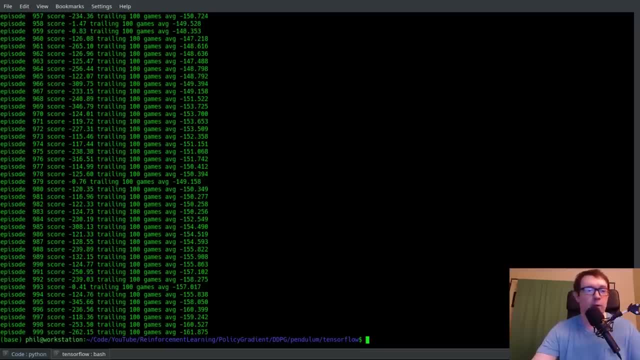 and if you check the leaderboards it shows that that's not true. That's actually a reasonable number. Some of the best environments only have 152 steps. Some of them do a little bit better. Sorry, best agents solve it in 152 steps. 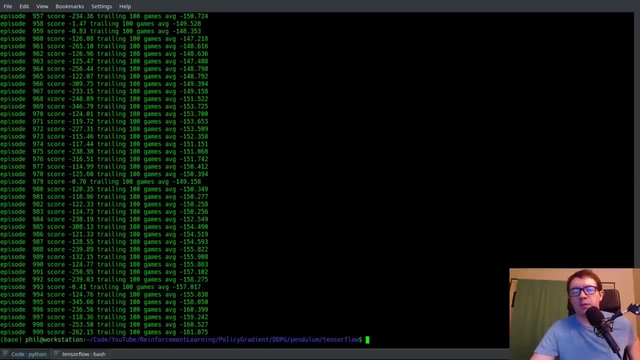 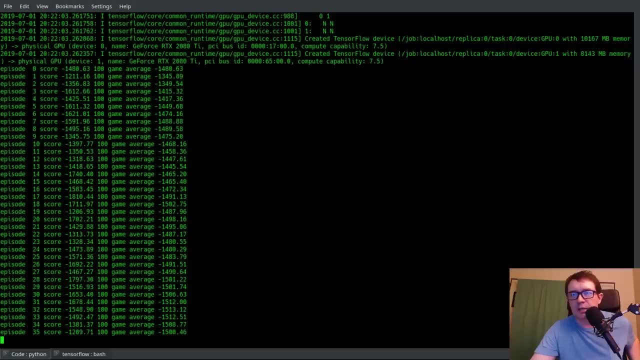 or achieve a best score of 150 steps, but it's pretty reasonable. So the default implementation looks like it's very, very slow to learn. You can see how it kind of starts out bad, gets worse and then starts to get a little bit better. 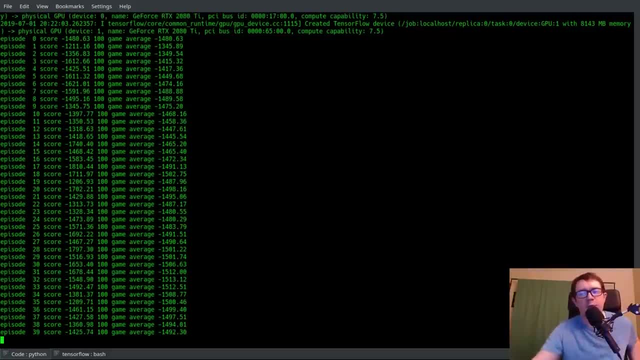 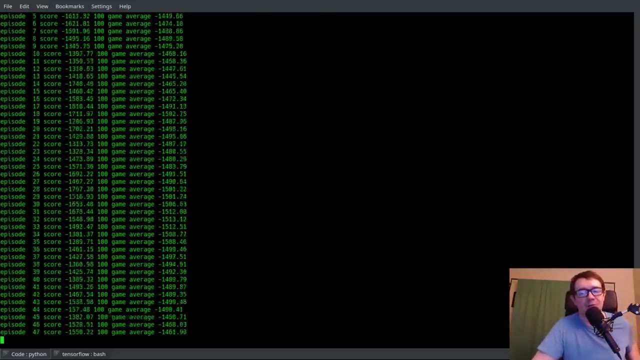 So that's pretty typical. You see this oscillation in performance over time pretty frequently, but that is that. That is how You go from a paper to a full implementation in about two hours. Of course, it took me many times to get this set up for you guys. 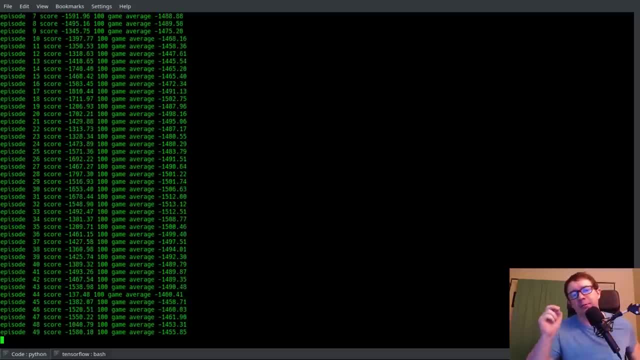 but I hope this is helpful. I'm going to milk this for all it's worth. This has been a tough project, so I'm going to present many, many more environments in the future. I may even do a video like this for PyTorch. 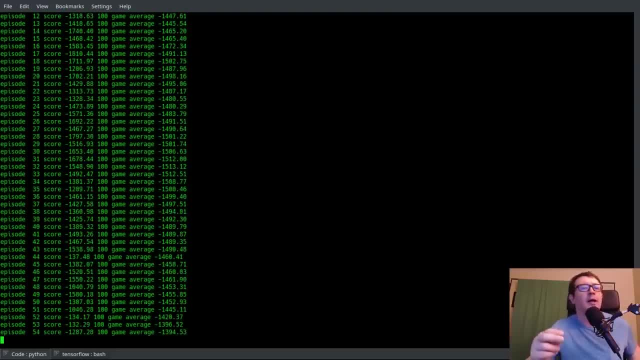 I have yet to work on a Keras implementation for this, but there are many more DDPG videos to come, so subscribe to make sure you don't miss it. Leave a comment. Share this if you found it helpful. That helps me immensely. 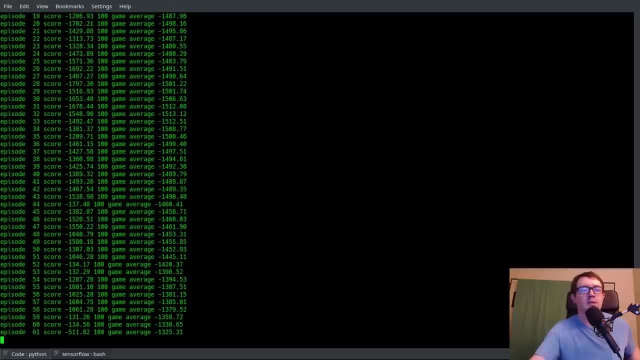 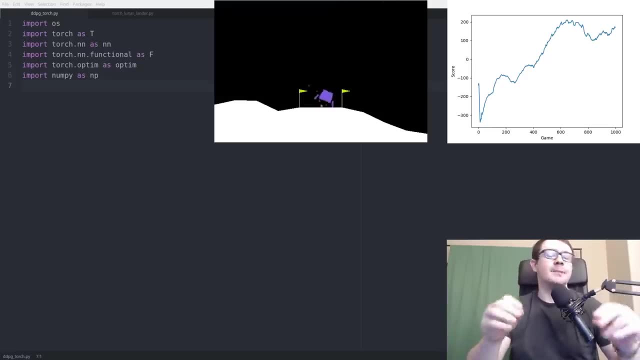 I would really appreciate it and I'll see you all in the next video. Welcome back everybody. In this tutorial you are going to code a deep deterministic policy gradient agent to beat the continuous lunar lander environment in PyTorch. No prior experience needed. 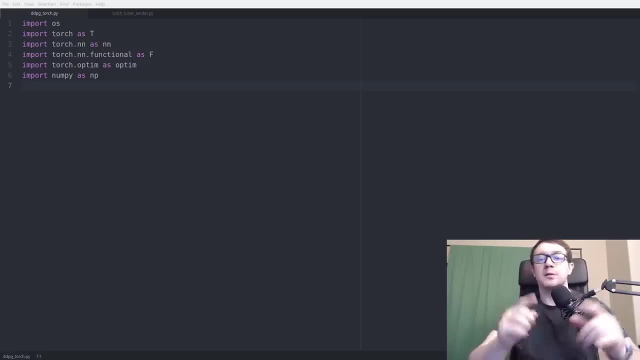 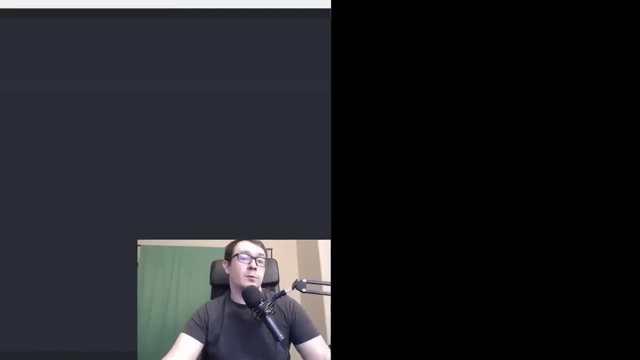 You don't need to know anything about deep reinforcement learning, You just have to follow along. Let's get started. So we start, as usual, with our imports. We'll need OS to handle file operations and all of the stuff from Torch that we've come to expect. 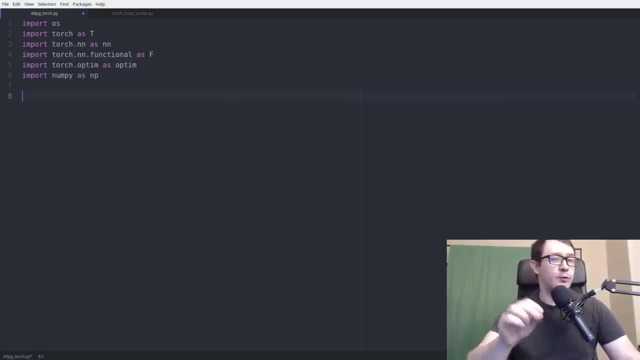 as well as NumPy. I'm not going to do a full overview of the paper. That will be in a future video where I will show you how to go from the paper to an actual implementation of deep deterministic policy gradients. so make sure you subscribe so you don't miss that. 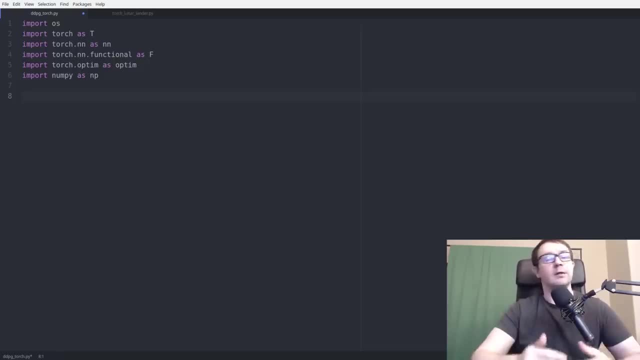 But in this video we're just going to get the very high-level overview, the 50,000-foot view, if you will. That will be sufficient to get an agent to beat the continuous lunar lander, so that's good enough. 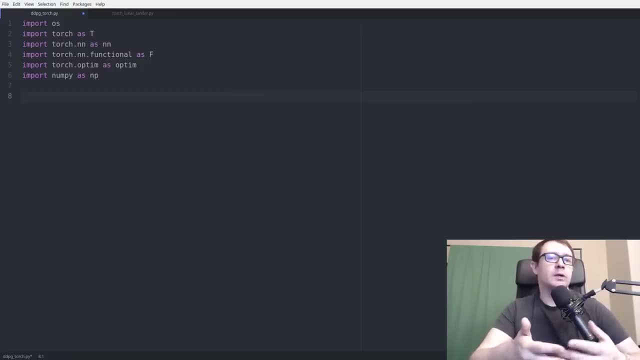 So the gist of this is we're going to need several different classes, so we'll need a class to encourage exploration, in other words, a type of noise. And you might have guessed that from the word deterministic. It means that the policy is deterministic. 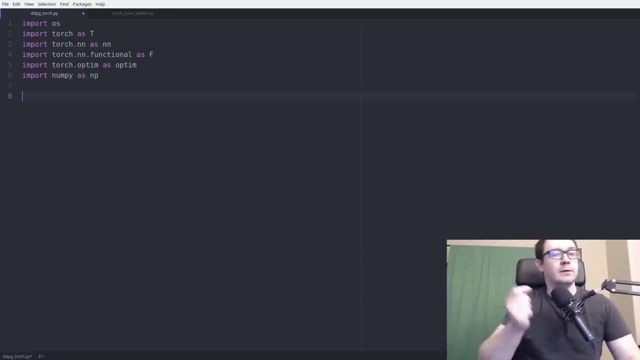 as in, it chooses some action with certainty And so if it is purely deterministic it can't really explore. so we'll need a class to handle that. We'll also need a class to handle the replay memory, because deep deterministic policy gradients works by combining the magic of actor-critic. 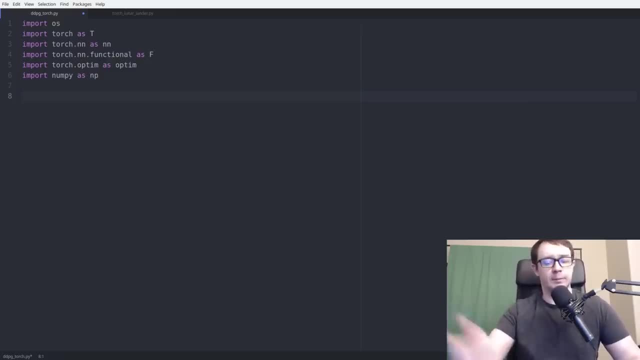 with the magic of deep Q-learning, which of course has a replay buffer, And we'll also need classes for our critic and our actor as well as the agent. So that's kind of a mouthful. We'll handle them one bit at a time. 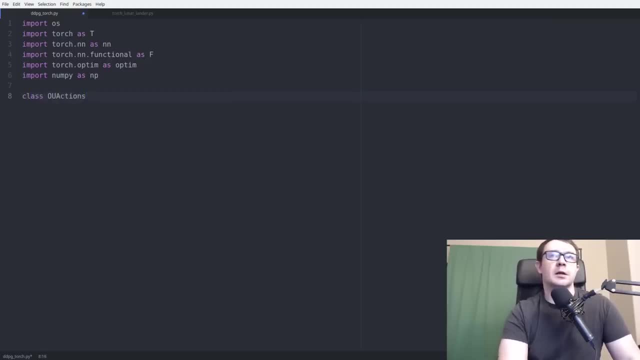 and we will start with the noise. So this class is called OU- Action Noise, and the OU stands for Orenstein-Uhlenbeck. So that is a type of noise from physics that models the motion of a Brownian particle, Meaning a particle subject to a random walk. 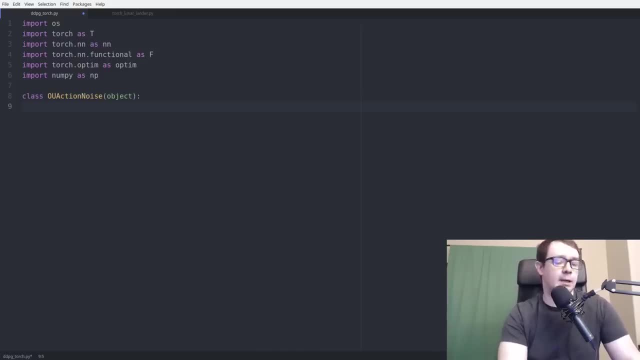 based on interactions with other nearby particles. It gives you a temporally correlated- meaning correlated in time- type of noise that centers around a mean of zero. So we're going to have a number of parameters: a mu, a sigma, a theta. 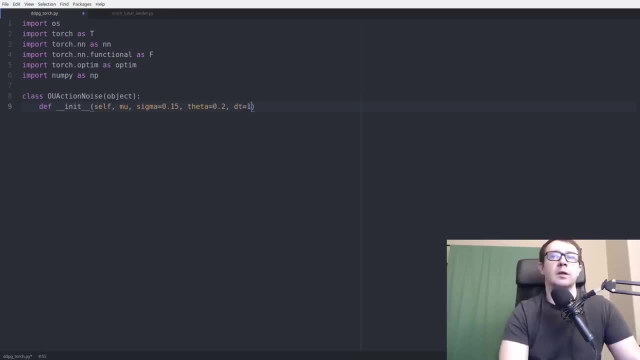 If I could type that would be fantastic- as well as a dt, as in the differential with respect to time and an initial value, that will get an original value of none. So if you want to know more about it, then just go ahead and check out the Wikipedia article. 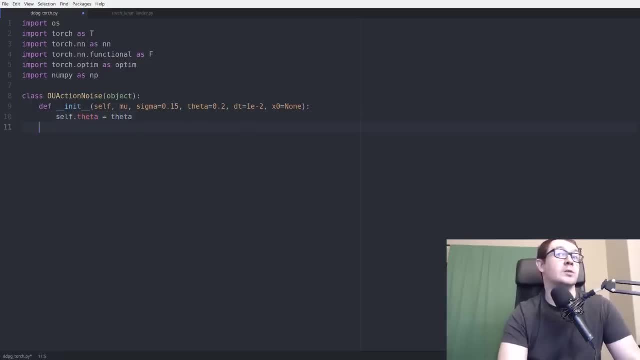 But the overview I gave you is sufficient for this tutorial. So of course, we want to save all of our values- X, zero- and we want to call a reset function. So the reset function will reset the temporal correlation which you may want to do that from time to time. 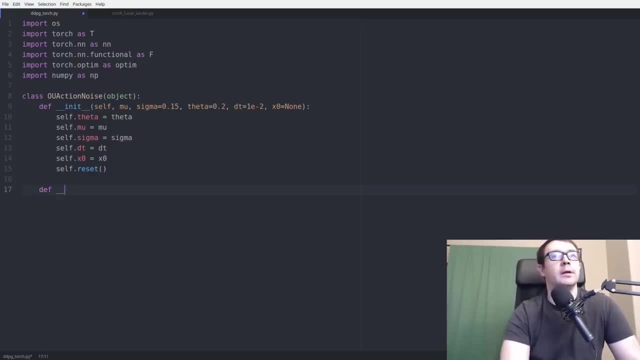 It turns out it's not necessary for our particular implementation, but it is a good function, So we're going to go ahead and do that. It's a good function to have nonetheless. So next we're going to override the call function. 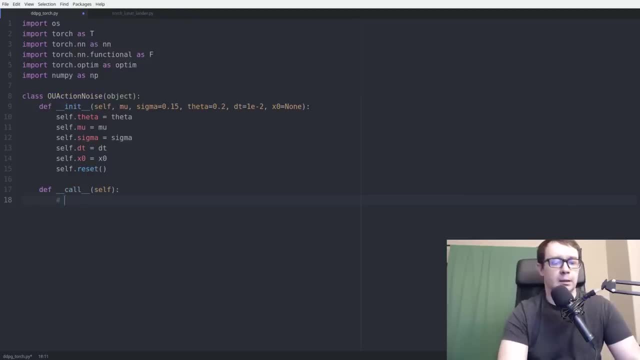 If you aren't familiar with this. this allows you to say noise equals OU, action noise, and then call noise. So that allows you to, instead of saying noise, dot, get noise, just say noise with parentheses, or whatever the name of the object is. 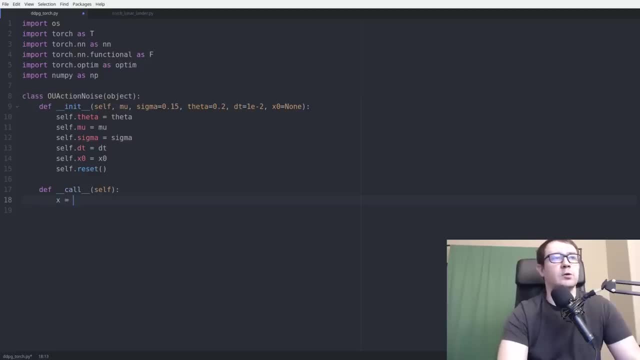 So that's overriding the call function. So we'll have an equation for that: X previous plus theta times the quantity mu minus self dot. X previous times self dot DT plus self dot sigma times numpy square root of self DT times: MP, random normal size equals mu shape. 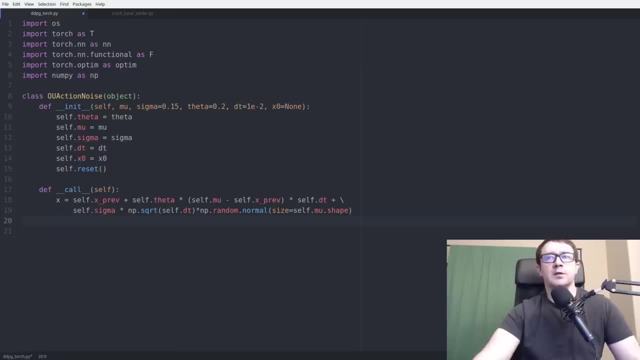 So it's a type of random normal noise that is correlated in time through this mu minus X previous term, And every time you calculate a new value you want to set the old value, the previous value, to the new one and go ahead and return the value. 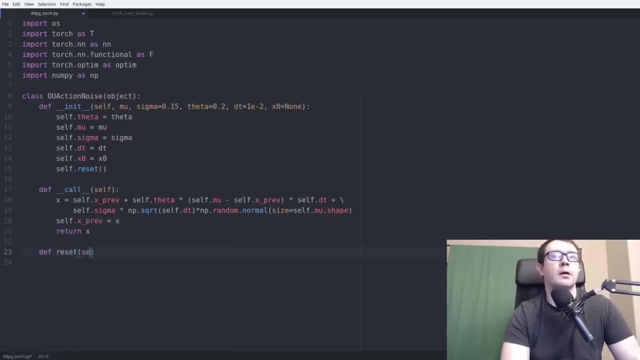 So the reset function all that does is check to make sure X zero exists. If it doesn't, it sets it equal to some zero value. So so X previous equals. so the X not if is not none else numpy zero is like in the shape of self. 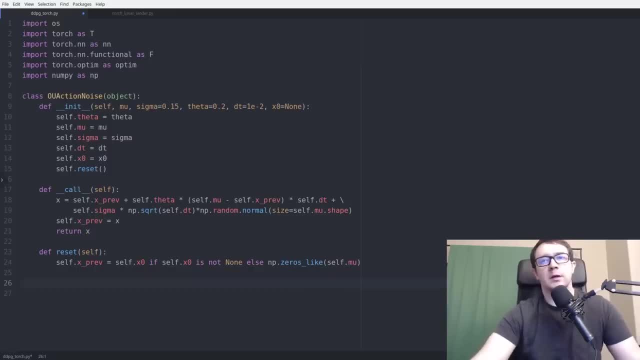 dot mu. That's it for the action noise. Again, this will be used in our actor class to add in some exploration noise to the action selection. Next we need the replay buffer class, And this is pretty straightforward. It's just going to be set of numpy arrays. 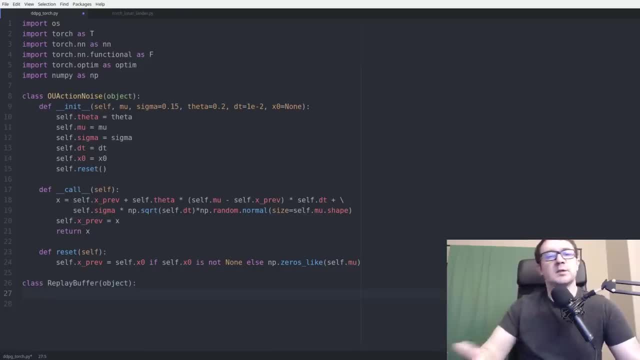 in the shape of the action space, the observation space and rewards, So that way we can have a memory of events that have happened, so we can sample them during the learning step. If you haven't seen my videos on deep Q learning, please check those out. 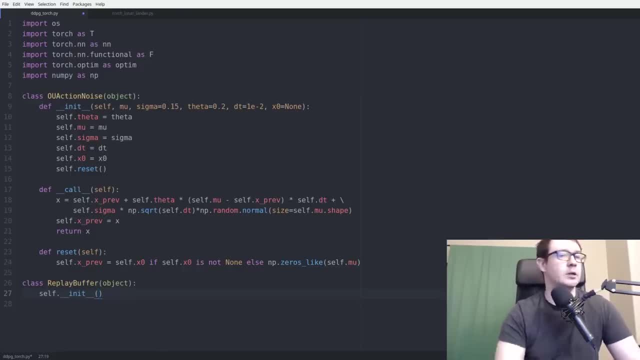 They will make all of this much more clear, as well as checking out the videos on actor critic methods, because this again, DDPG kind of combines actor critic with deep Q learning, So that will really be helpful for you. I'll go ahead and link those here as well. 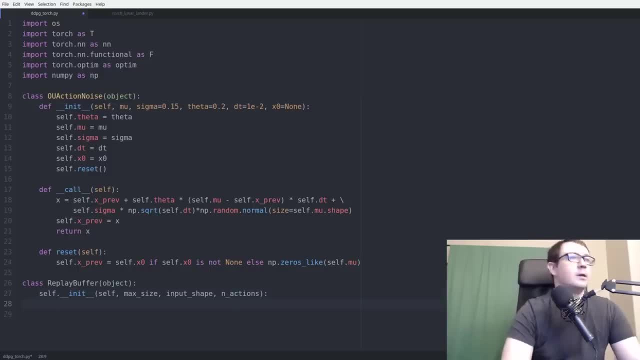 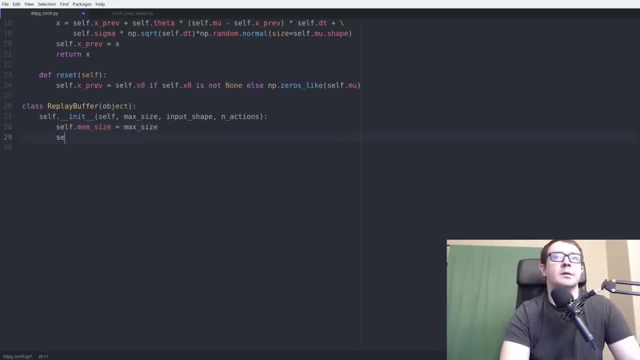 So that way you can get edumacated. So scroll down a bit. We want to save our mem size as max size, So the mem counter we'll start out at zero Again. this is just going to be a set of arrays. 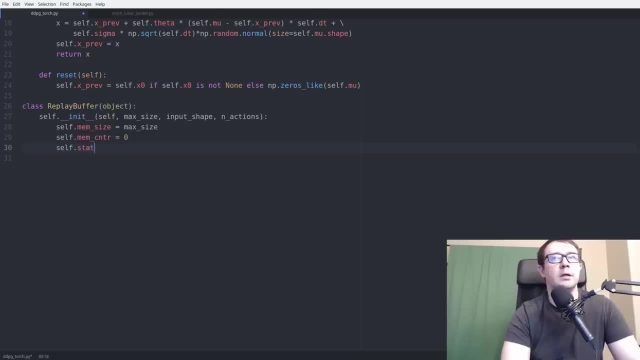 that keep track, or matrices, in this case, that keep track of the state reward, action transitions, And that will be in shape: mem size. So, however number of memories we want to store and input shape. So if you are relatively new to Python, this star variable idiom, it isn't a pointer. 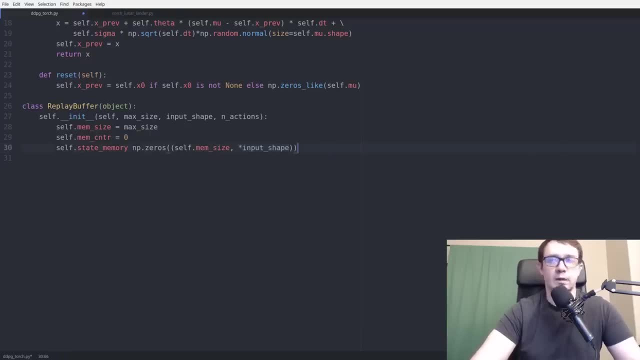 If you're coming from C or C++, it is an idiom that means to unpack a tuple. So this is going to be an idiom that means to unpack a tuple. This makes our class extensible, So we can pass in a list of a single element. 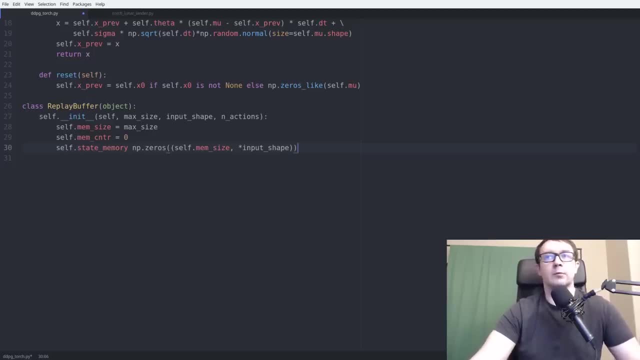 as in the case of the continuous lunar and lander environment that we'll use today Or later on, when we get to the continuous car racing environment, we'll have images from the screen, So this will accommodate both types of observation vectors. It's a way of making stuff extensible. 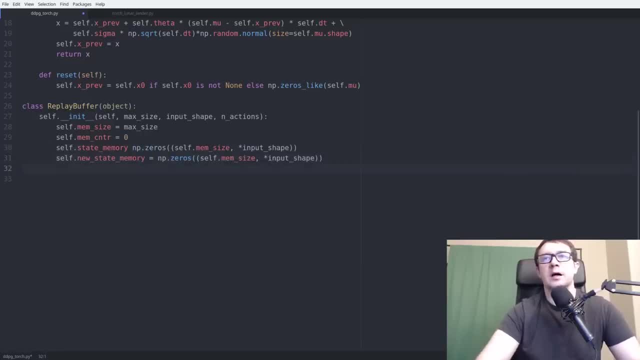 And the new state memory is, of course, the same shape, So we just copy it. It looks like I am missing a parenthesis somewhere. I guess we'll find it when I go ahead and run the program. So oh, it's not selfinit, it's def. 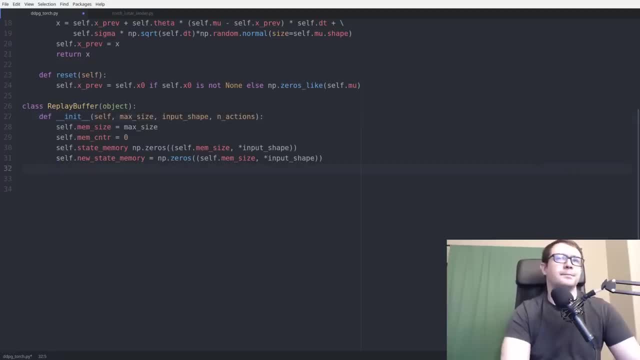 There we go: Def init perfect. So we'll also need an action memory, And that, of course, will also be an array of zeros in the shape of mem size by number of actions. I believe that means I need an extra parenthesis there. 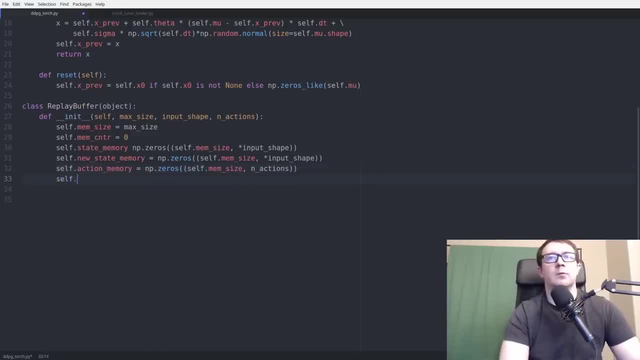 I believe that means I need an extra parenthesis there. I believe that means I need an extra parenthesis there And we'll also have a reward memory And that will just be in shape- mem size- And we also need a terminal memory And we'll also have a reward memory. 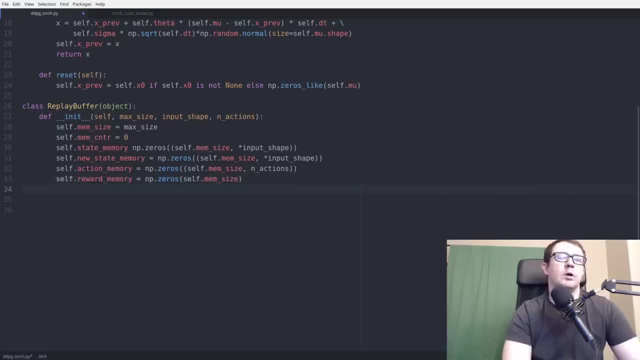 And that will just be in shape, mem size. We also need a terminal memory. So in reinforcement learning we have the concept of the terminal state. So when the episode is over, the agent enters the terminal state, from which it receives no future rewards. 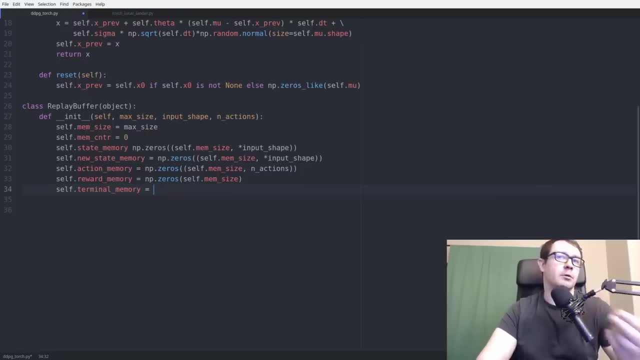 So the value of that terminal state is identically zero, And so the way we're going to keep track of when we transition into terminal states, terminal states- is by saving the done flags from the open ai gem environment, and that'll be shape numpy, uh, numpy, zeros, mem size and uh. i've called this float32. it's probably because 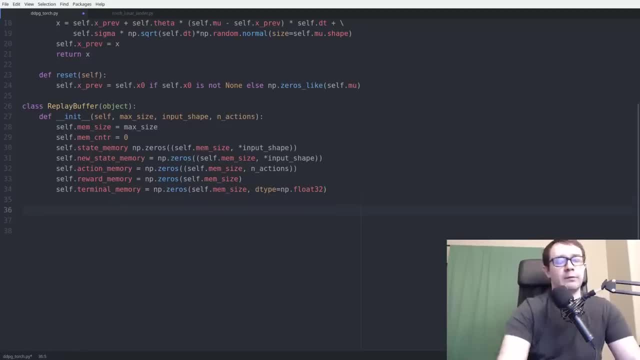 uh, torch is a little bit particular with data types, so we have to be cognizant of that. we need to function to store transitions, which is just a state action, reward, new state and done flag. so the index is going to be the first available position. so memcounter just keeps track of the 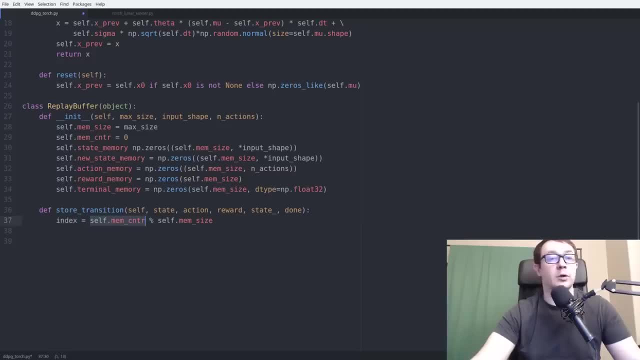 last memory you stored, it's just an integer quantity, from zero up to memsize, and so when memcounter becomes greater than memsize, it just wraps around from zero. so when they're equal at zero, and when they're equal to zero, it just wraps around from zero. so when they're equal at zero and. 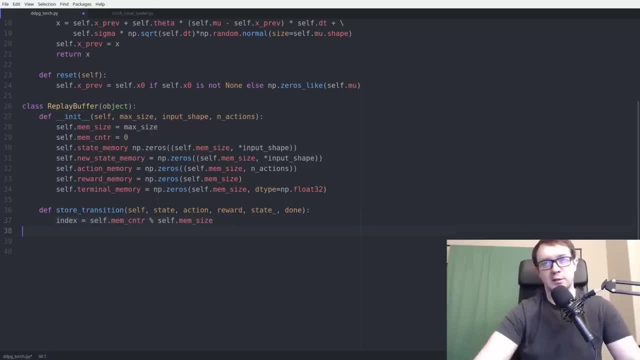 when it's equal to memsize plus one, it becomes one, and so on and so forth. so state memory subindex equals state action memory index, reward equals state underscore and the um terminal memory good grief. terminal memory index doesn't equal done, but it equals one minus done. so the reason is that when we get to 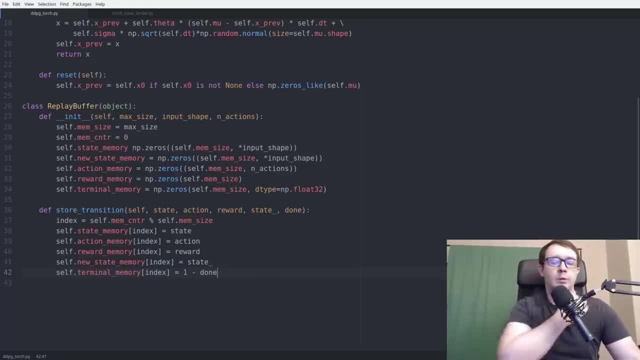 the update equation, the bellman equation, for our learning function. you'll see, we want to multiply by whether or not the episode is over, and that gets is facilitated by one minus the quantity done. just increment memcounter and next we need to um sample that buffer. so sample buffer and that will. 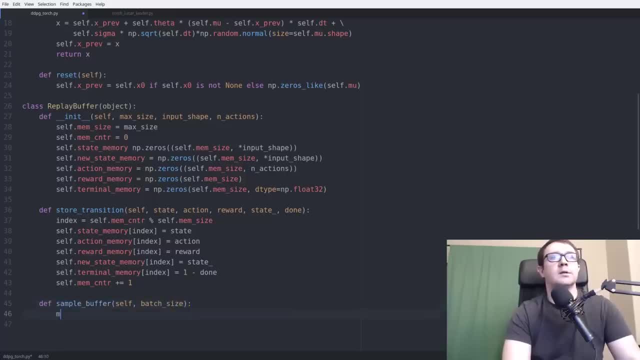 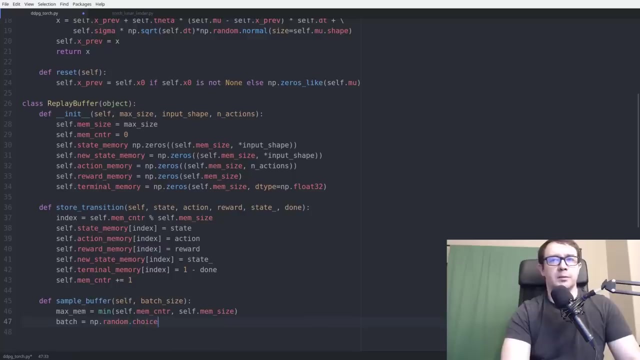 take in a batch size as input. so the max memory is going to be the minimum of either mem counter or mem size, not the max but the minimum. then match is just going to be a random choice of uh maximum index of max mem number of elements- excuse me- equal to batch size. scroll down a bit. and then we want to get a hold of. 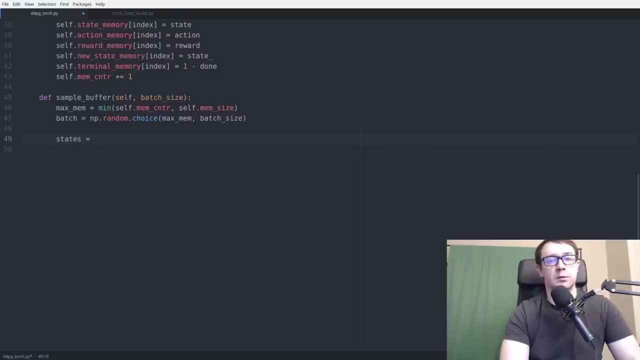 of the respective states actions, rewards and new states and terminal flags and pass them back to the learning function sub batch. new states rewards- you know it's not easy to type and talk at the same time, apparently. and let's get actions, self dot, action memory fetch and terminal good grief. so we want to return states actions. 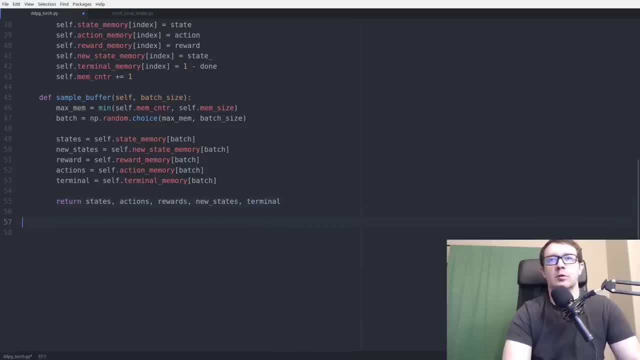 rewards new states and the terminal flags- perfect. so that is it for our replay memory. So you're going to see this a lot in the other videos on deep deterministic policy gradients, because we're going to need it for basically anything that uses a memory. 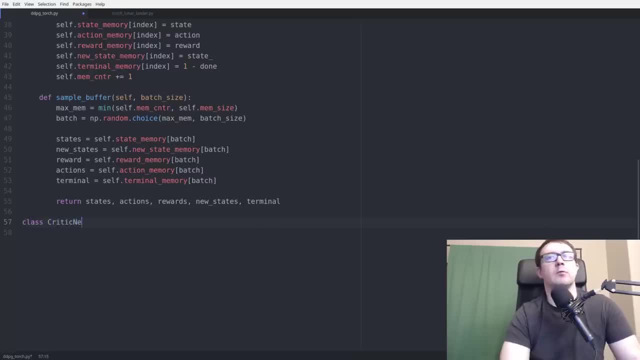 Next let's go ahead and get to the meat of the problem with our critic network. And, as is often the case when you're dealing with PyTorch, you want to derive your neural network classes from nnmodule. that gives you access to important stuff like the train and 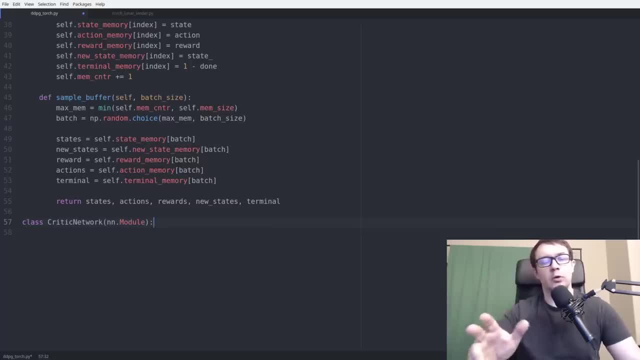 eval function, which will set us in trainer evaluation mode, very important later. I couldn't get it to work until I figured that out, So a little tidbit for you. you also need access to the parameters for updating the weights of the neural network. So let's define our initialize. 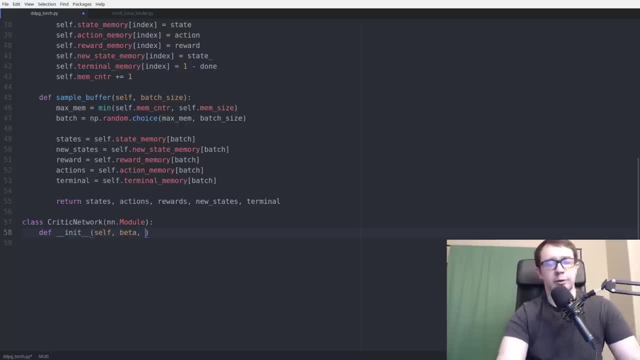 function. The beta is our learning rate. we'll need input dims. number of dimensions for the first fully connected layer, as well as second connected layer. number of actions. a name: the name is important for saving the network. you'll see that we have many different networks. 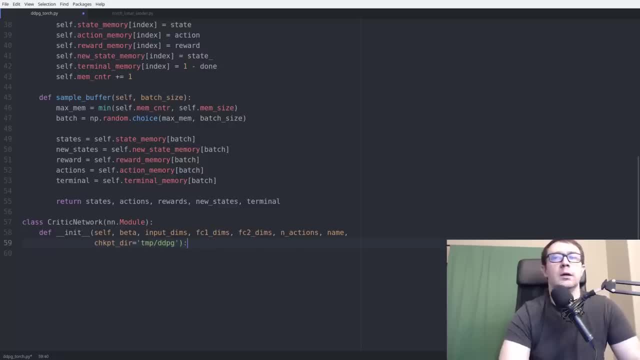 So we'll want to keep track of which one is, which very important, As well as a checkpoint directory for saving the model. They're also very important because this model runs very, very slowly, So you'll want to save it periodically And you want to call the super constructor for critic network. 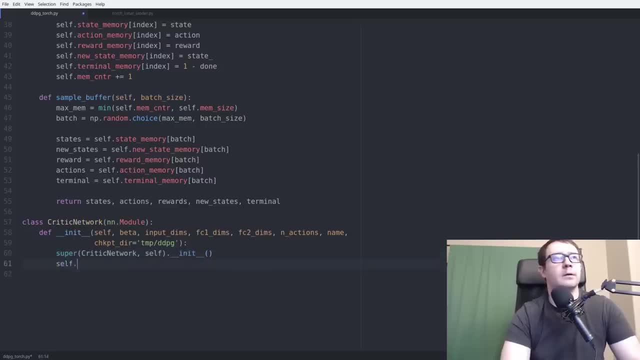 And that will call the constructor for nnmodule. I believe input dims equals input dims. I see one dims. So these will just be the parameters for our deep neural network. that approximates the value, function, the number of actions, a checkpoint file and that is OS path. join checkpoint dir with name plus underscore ddpg. 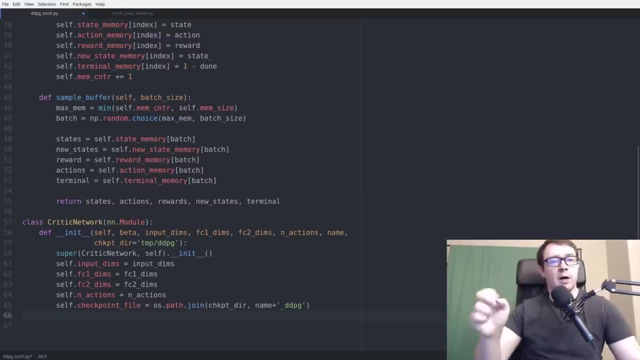 And if you check my GitHub repo, I will upload the train model, because this model takes a long time to train, So I want you to be able to take advantage of the fully trained model that I've spent the resources and time training up, So you may as well benefit from that. So next up, we need 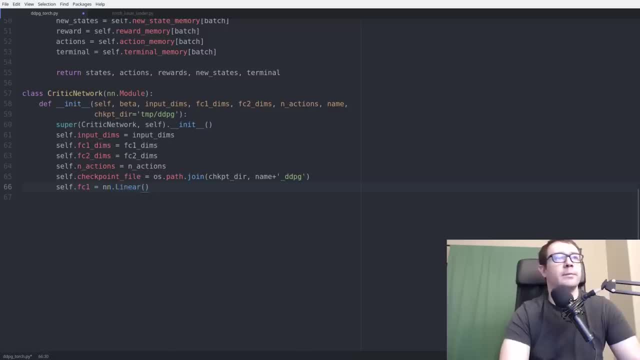 to define the first layer of our neural network, just a linear layer, And that'll take input dims and output FC, one dims. We're also going to need a number for initializing the weights and biases Of that layer of the neural network and we're gonna call that f1 is divided by one over the square. 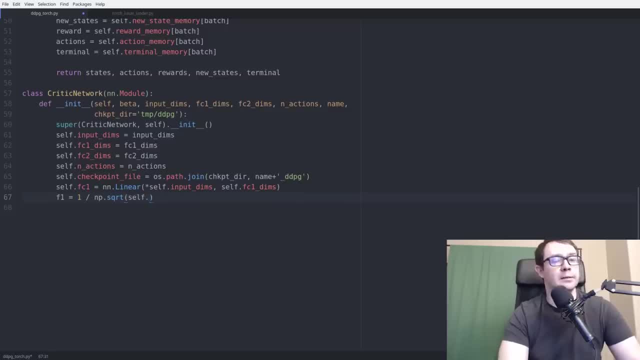 root of the number of dimensions into the network. So self dotf, c, 1 DC, weight data, that size that returns a tuple. so I need the zero element of THAT And then we want to initialize that layer by using T torch and then init, And then in here I'm going to call that the efficient city. enough, toela, Which allows me. 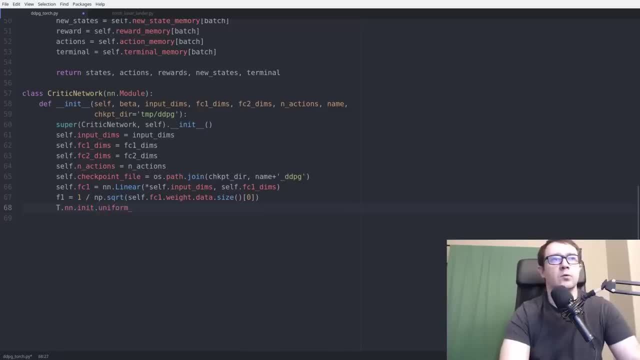 this error And thenуска a. now, Now that you've created amoment on a row, let's see what other times I many times fill Port row. all that written in can't complete those. Penn becoming сним sleeping, So dot uniform, underscore the, the tensor you want to initialize, which is fc1 weight data. 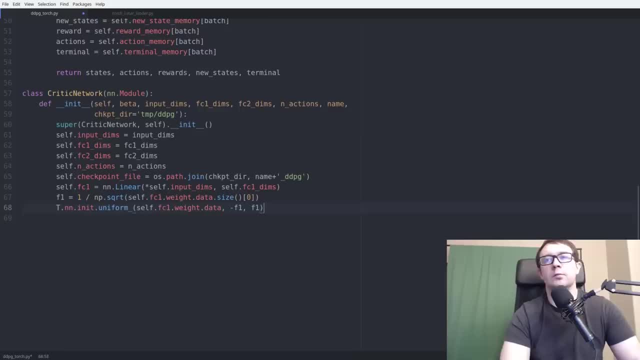 up from minus one to positive f1, so this will be a small number of order 0.1, or so not exactly 0.1, but of order 0.1, and you also want to initialize the biases, biasdata, and that gets the same number. and again in the future video when we go over. 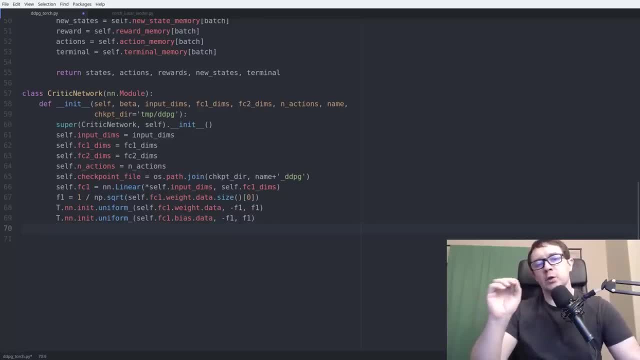 the derivation of the paper. i'll explain all of this, but just for now, know that this is to constrain the initial weights of the network to a very narrow region of parameter space to help you get better convergence. perfect, so, oh, and make sure to subscribe so you don't miss that video. 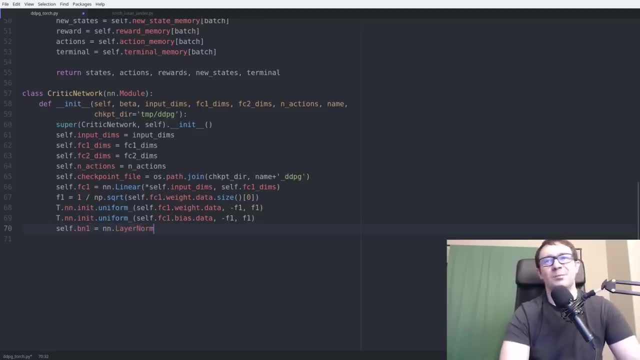 because it's going to be lit. so bn1 is a layer norm and takes fc1 dims as input. the batch normalization helps with convergence of your model. you don't get good convergence if you don't have it, so leave it in. so fc2 is a second layer. 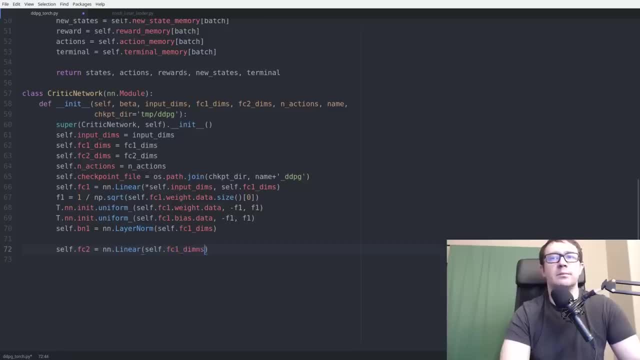 another, linear. it takes fc1 dims as input and outputs, fc2 dims- good grief, and we want to do the same thing with initialization. so it's one over the square root of fc1 dims and it takes fc1 dims as input and outputs, fc2 dims. 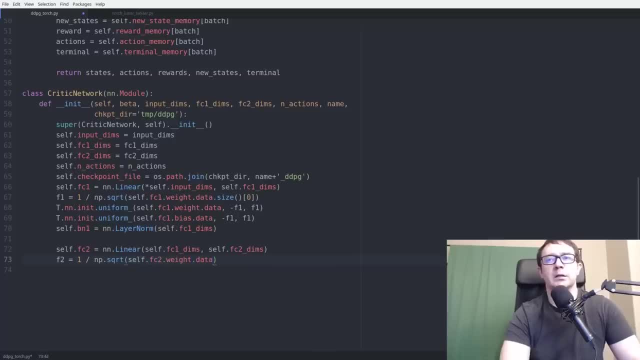 root of self dot fc2 weight data, dot size zero and you want to do tnn init uniform underscore c2 weight data minus f2 up to f2. make sure that's right so we don't screw that up, because that's important. that looks correct. the syntax here is the first parameter. is the tensor you want. 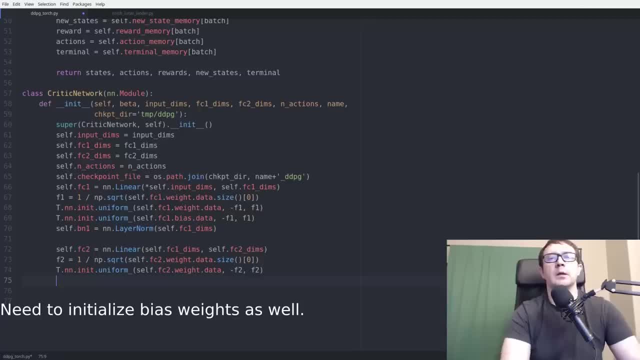 to initialize and then the lower and upper boundaries. so next we need uh bn2, which is our second batch norm layer, fc2 dims. and, just a note, the fact that we have a normalization layer, a batch norm type layer, means that we have to use the eval and train functions later. 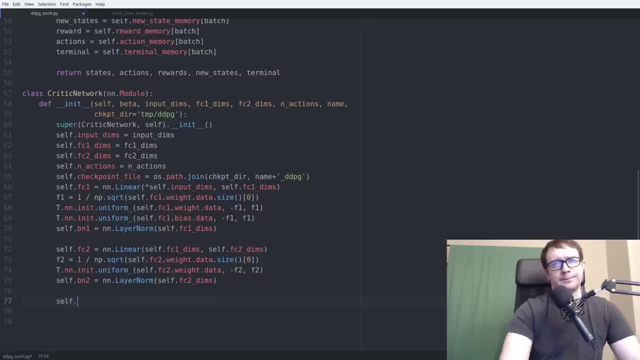 kind of a nuisance. it took me a while to figure that out. uh, the critic network is also going to get a um action value, because the action value function takes in the states and actions as input, but we're going to add it in at the very end of the network. 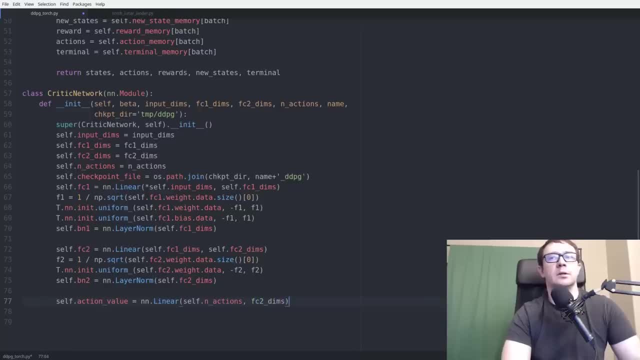 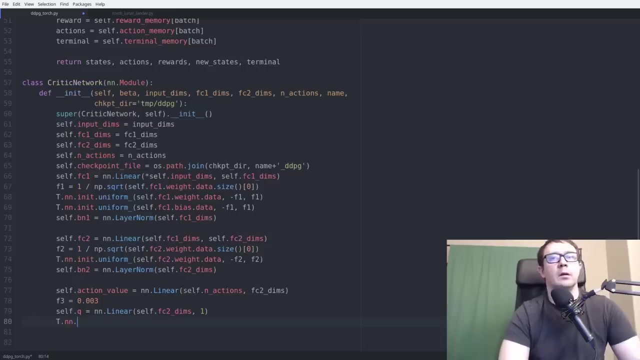 Linear actions. C2 dims and this gets a constant initialization of 003, or, sorry, the next one, the output, gets an initialization of 003, and since this is a scalar value, it just has one output and you want to initialize it again uniformly. 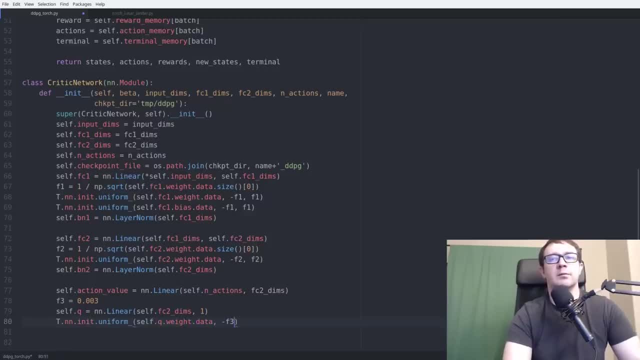 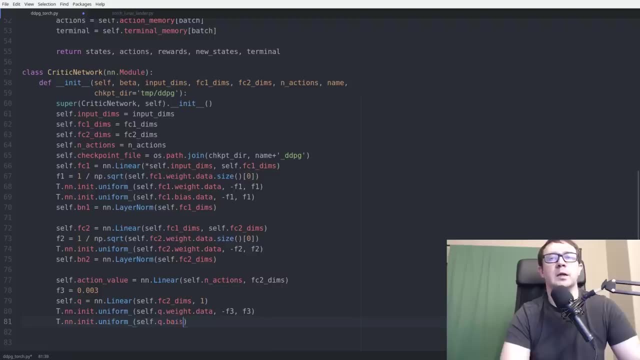 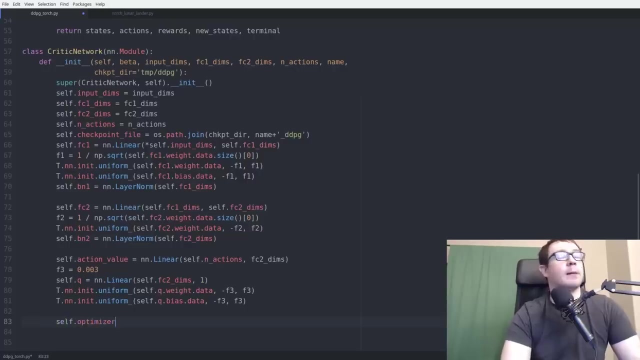 qweightdata, and that gets minus F3 up to F3, and likewise for bias data. Okay, so now we have our optimizer and that will be the atom optimizer. and what are we going to optimize? The parameters and the learning rate will be beta. 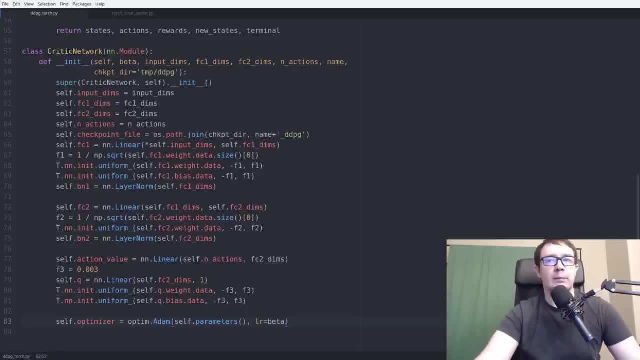 So you notice that we did not define parameters right here. right, We're just calling it and this comes from the inheritance from nnmodule. That's why we do that, so we get access to the network parameters. Next, you certainly want to run this on a GPU. 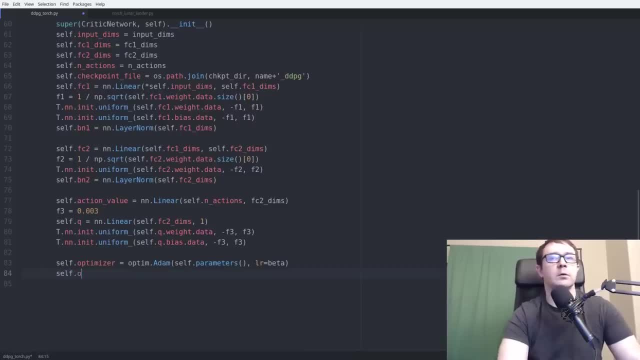 because it is an incredibly expensive algorithm. so you want to call the device so tdevice, CUDA 0 if tCUDAisAvailable, else CUDA1,. so I have two GPUs. If you only have a single GPU, it will be else. CPU. 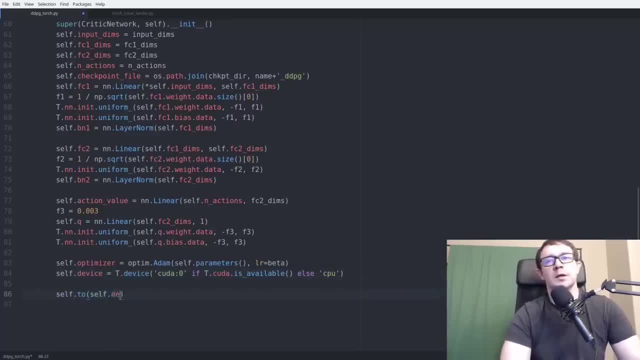 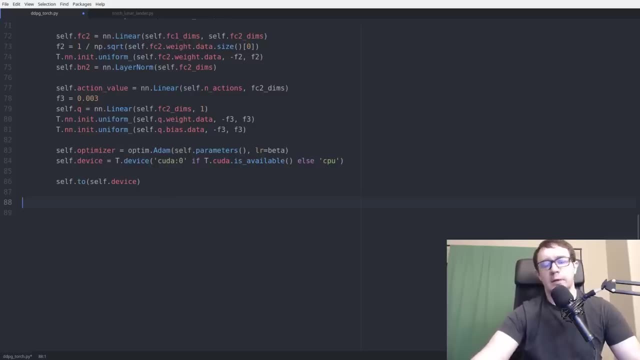 but I don't recommend running this on a CPU. So next you want to send the whole network to your device by selfto selfdevice. We are almost there for the critic class. Next thing we have to worry about is the forward function. 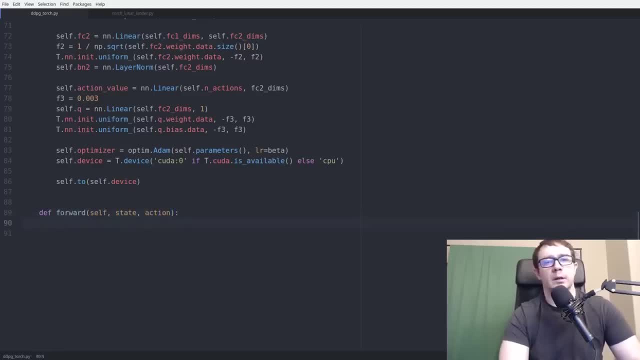 And that takes a state and an action as input. Keep in mind the actions are continuous, so it's a vector, In this case length 2, for the continuous lunar lander environment. It's two real numbers in a list or numpy array format. 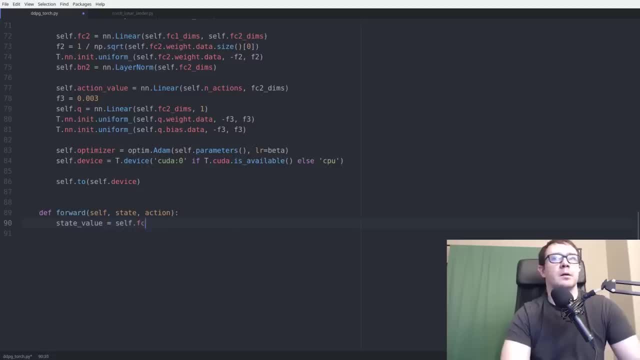 So state value: fc1 state, and then you want to pass it through bn1 state value And finally you want to activate it- frelu state. Now it is an open debate whether or not you want to do the relu before or after the batch normalization. 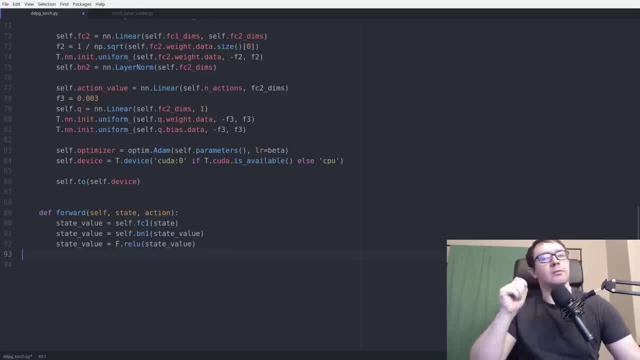 In my mind it makes more sense to do the batch normalization first, because when you are calculating batch statistics, if you apply the relu first, then you're lopping off everything below zero, right? So that means that your statistics are going to be skewed toward the positive end. 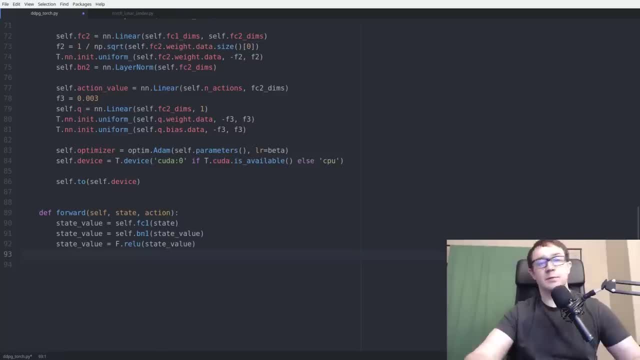 when perhaps the real distribution has a mean of zero instead of a positive mean, or maybe it even has a null. So that means that your statistics are going to be skewed toward the negative mean, which you wouldn't see if you used the relu function. before the batch normalization. 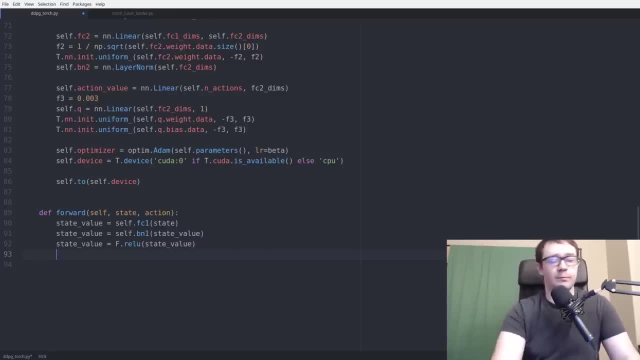 So just something to keep in mind. You can play around with it. Feel free to clone this and see what you get, But that's how I've done it. I did try both ways and this seemed to work the best. So next we want to feed it into the second fully connected layer. 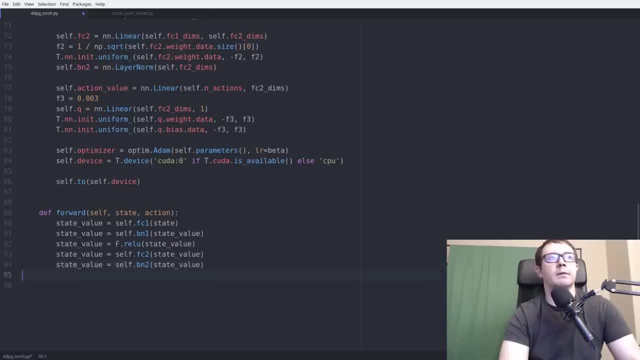 Bn2 state value And then we want to bn2 that. Sorry, I already did that One second, let me let the cat out. So we've already done the batch normalization. We don't want to activate it yet. What we want to do first is take into account the action value. 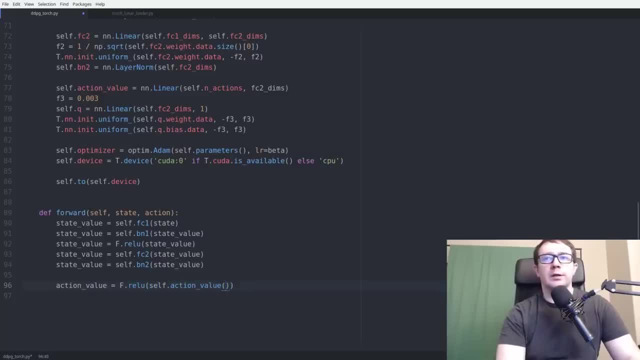 And what we're going to do is activate the action through the action value layer and perform a relu activation on it right away. We're not going to calculate batch statistics on this, so we don't need to worry about that, But what we want to do is add the two values together. 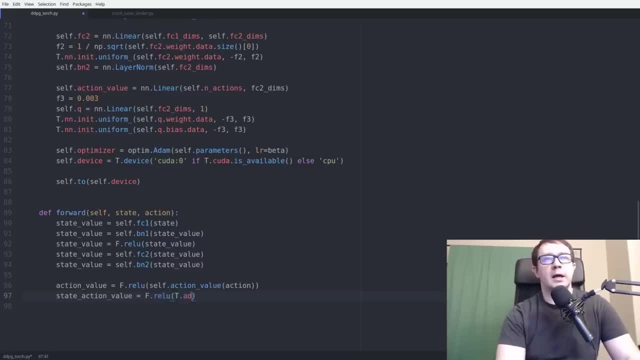 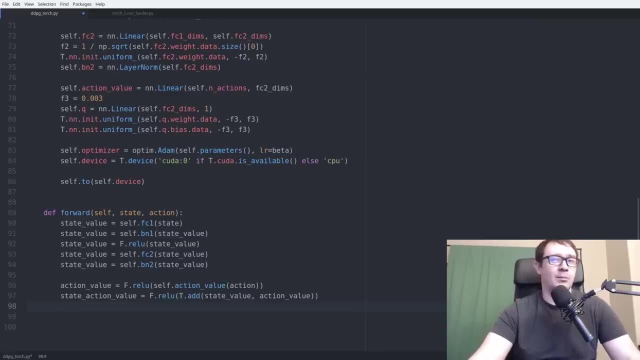 So state action value, frelu tadd, state value and action value. Other thing that's a little bit wonky here- and I invite you to clone this and play with yourself- is that I am double reluing the action value function. 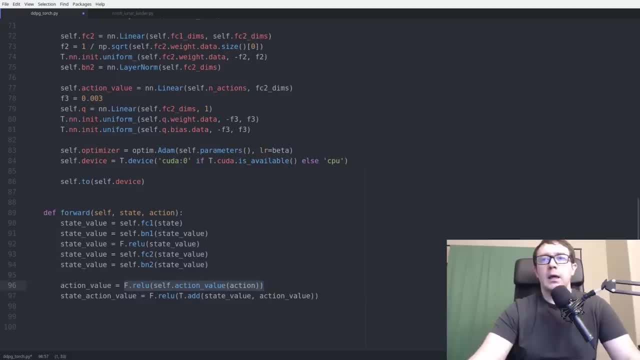 so the action value, quantity. So I do a relu here and then I do a relu on the add. Now, this is a little bit sketchy. I've played around with it and this is the way it works. It works for me. 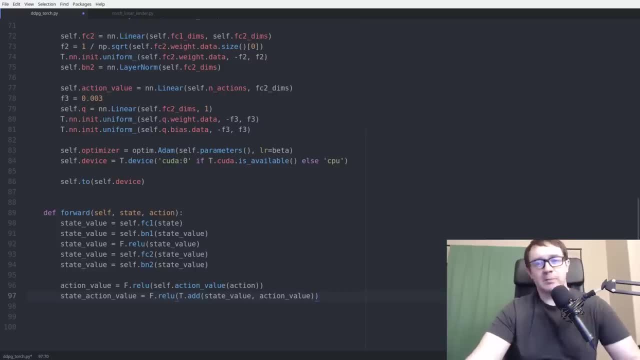 So you can clone it and get it to work a different way. The other possibility is that you don't do this relu here, but you do the relu after the add. So relu is a non-commutative function with add. So what that means is that if you do an addition first and then a relu, 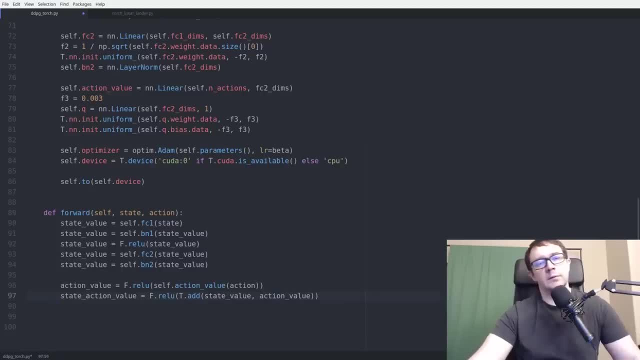 that's different than doing the sum of the two relus, right? So if you take relu of minus 10 plus relu of 5, you get a relu of minus 10 is 0 plus relu of 5 is 5, so you get 5.. 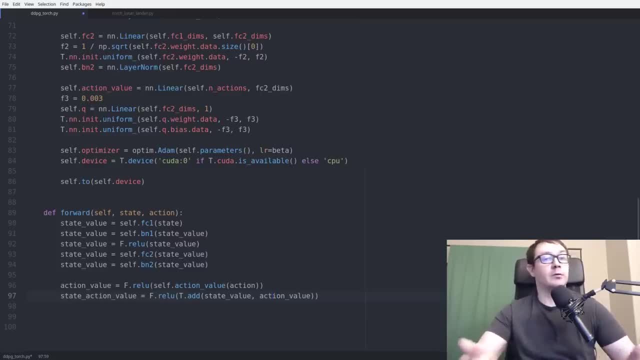 If you take the relu of minus 10 plus 5, then you get a relu of minus 5 or 0. So it's a non-commutative function. so it does matter the order, But this is the way I found it to work. 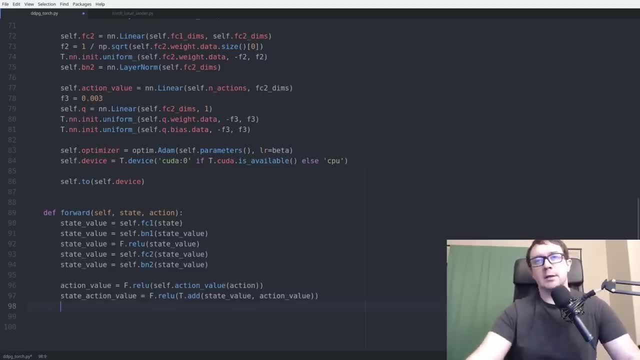 I've seen other implementations that do it differently. Feel free to clone this and do your own thing with it. I welcome any additions, improvements or comments. So then, we want to get the actual state action value bypassing that additive quantity through our final layer of the network. 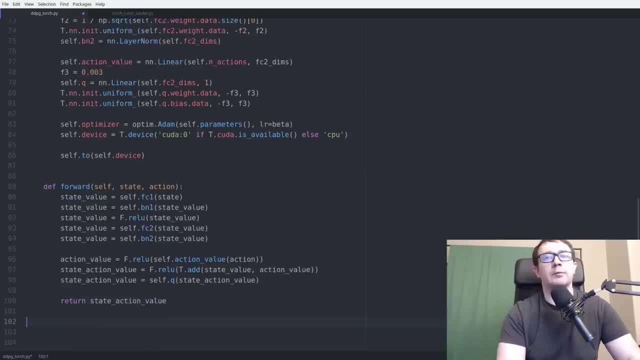 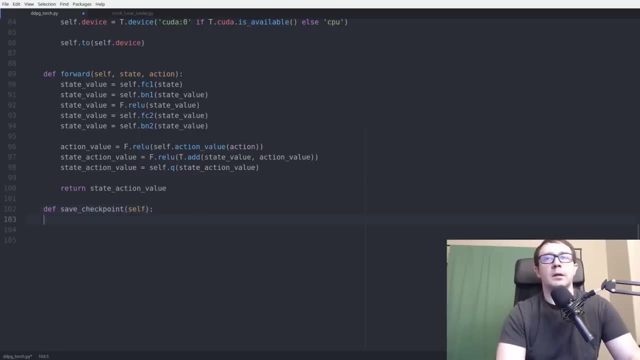 And go ahead and return that little bit of bookkeeping. We have a check save, checkpoint function and we'll say print. And then you want to call tsave selfstate dict. What this does is it creates a state dictionary where the keys are the names. 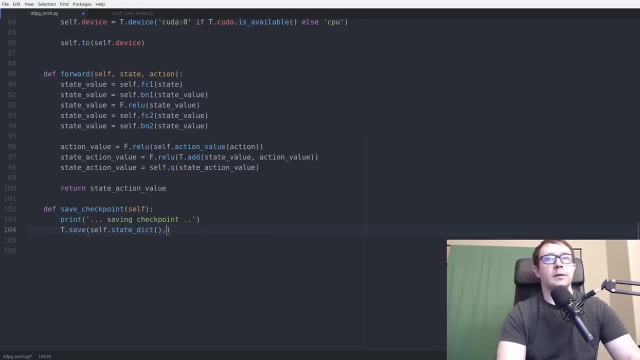 of the parameters and the values are the parameters themselves. And where do you want to save that? You want to say that in the checkpoint file. Then you also have the load checkpoint, good grief checkpoint function And that does the same thing, just in reverse. 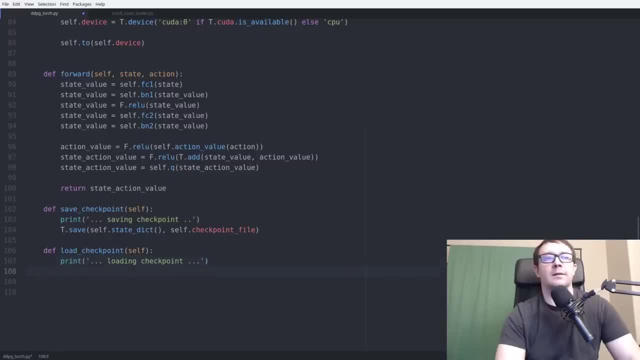 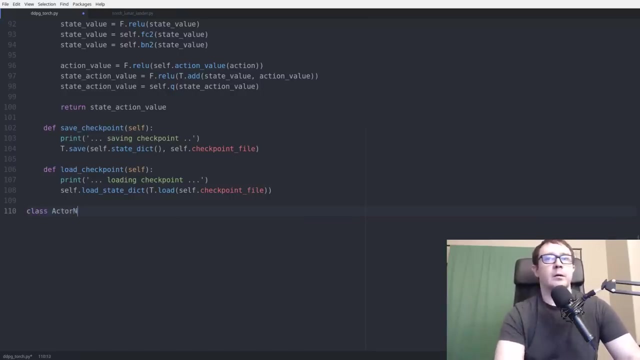 Loading checkpoint and you want selfload state dict. tload selfcheckpoint file. So that is it for our critic network. Now we move on to the actor network, And then, of course, it derives from NNmodule. We have an init function. it takes alpha. 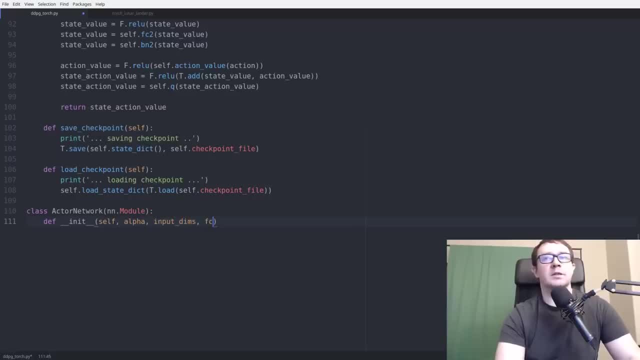 If you can spell correctly: input dims, FC1 dims, FC2 dims. This is pretty similar to the critic network. It will just have a different structure. In particular, we don't have the. we don't have the critic network, but we have an input dims. 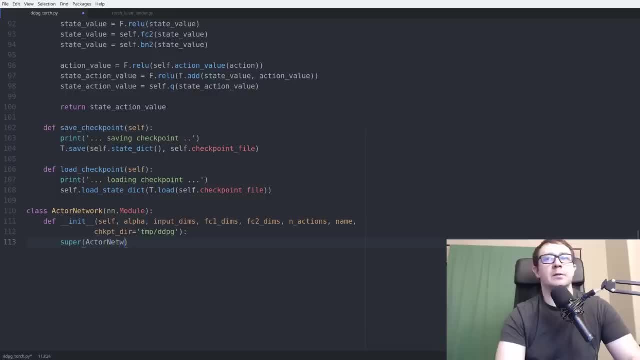 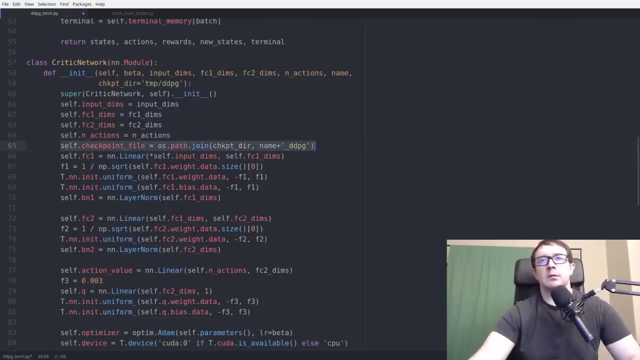 actions. I can't type and talk at the same time, but it's pretty similar nonetheless. so input- dims- you want to save- and actions- see one dims- and FC- two dims- same deal. let me go copy the checkpoint file function, just to make life easy. perfect, I like to make life easy, so we have our first fully. 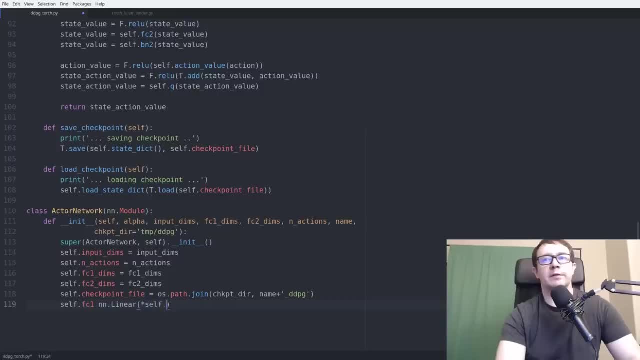 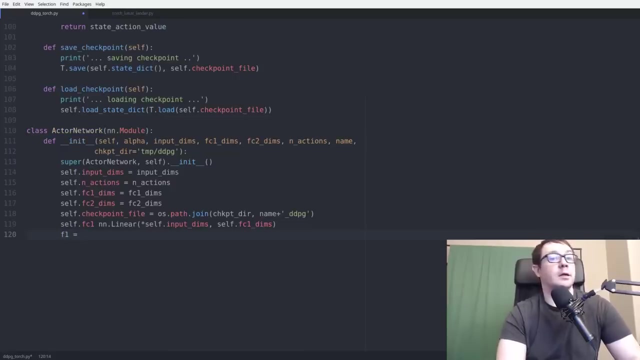 connected layer and end out linear. takes self input dims as input and FC one dims and of course that operates in the same way as I discussed in the replay buffer, where it will just unpack the tuple. next we have the initialization value, very similar: 1 over MP square root self. 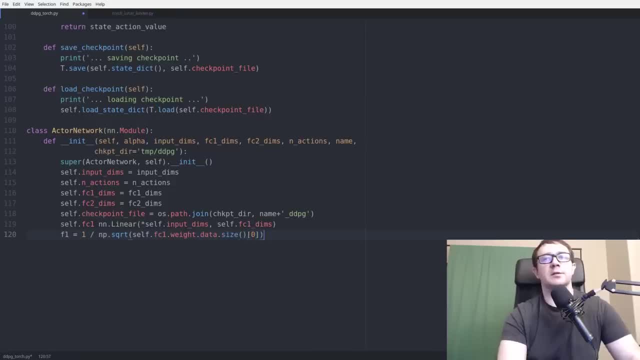 dot FC, one dot weight data size, zeroth element and you want to initialize the first layer uniformly within that interval in its uniform underscore se 1 weight data minus f1 and f1 copy that that will be a, a, a, a, fc1 bias data. fc2 is another linear layer. takes fc1 dims as inputs and outputs, fc2 dims as you. 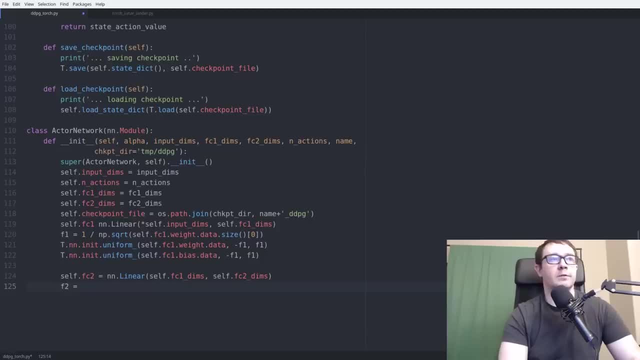 might expect, and the initialization for that will be basically the same thing, except for layer two. so fc2, weight data and then you know what? let's just copy this paste and make sure we don't mess up: fc2, f2- oh good grief. and plus minus f2, and that is all well and good. other thing we forgot: 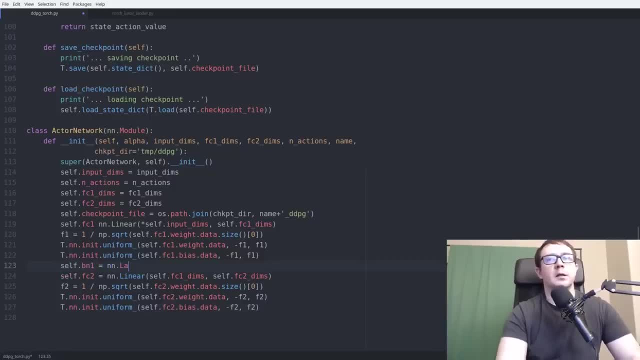 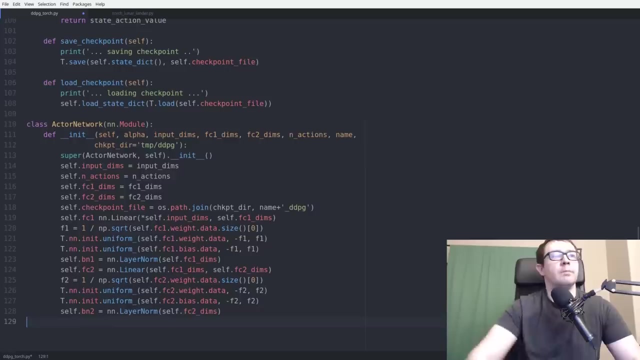 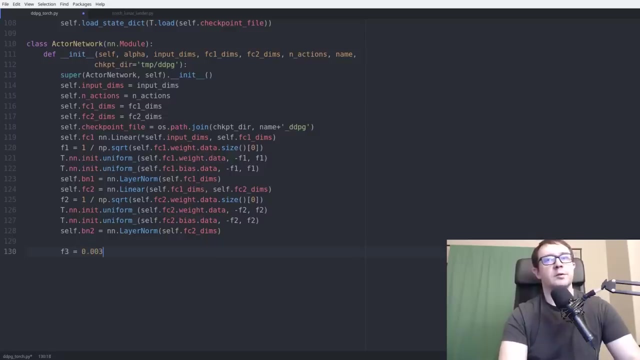 is the batch norm and that is nn layer norm and that takes fc1 dims as input. likewise for layer two, that is another layer norm, takes fc2 dims as input shape and that doesn't get initialized. but we do have the f3 and that is 0 0 3. this comes from the paper. we'll go over this. 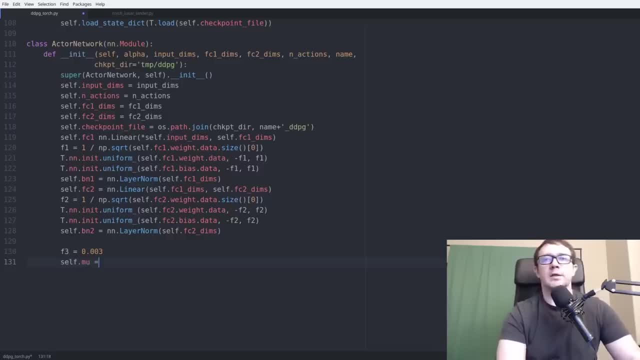 in a future video, but don't worry about it. selfmu mu is the representation of the policy in this case, and that's the representation of the policy in this case, and that's the representation of the policy in this case. it is a real vector of shape and actions. it's the actual action, not the. 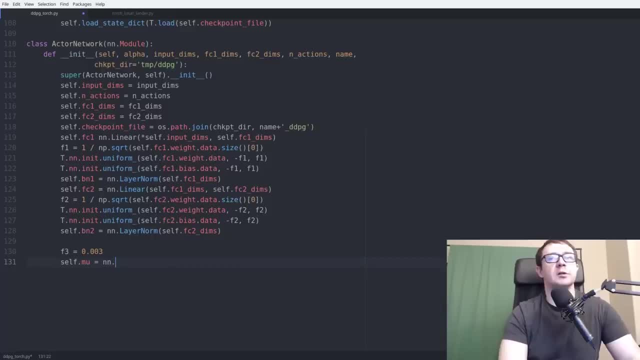 probability. right, because this is deterministic, so it's just a linear layer. takes fc2 dims as input and outputs the number of actions. and we want to do the same thing where we initialize the weights. let's copy paste, and instead of fc2 it will be mu and instead of f2 it is. 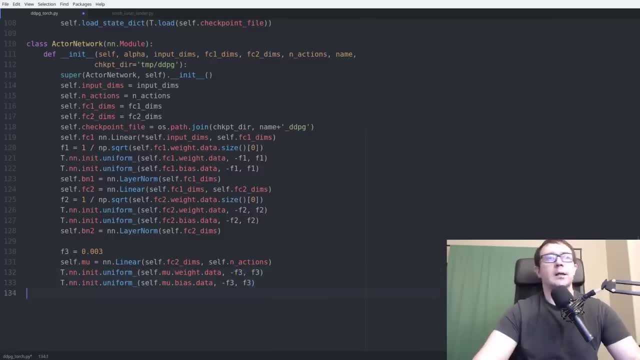 f3, as you might expect. am i forgetting anything? i don't believe so. so, finally, we have an optimizer, and that's again optimadem: selfparameters and learning rate equals alpha. we also want to do the same thing with the device tdevice, cuda zero, if tcudais available else. 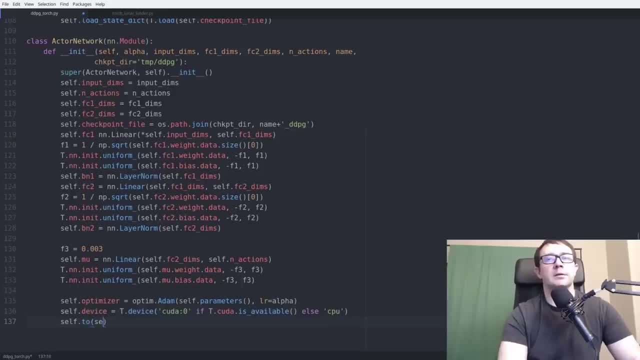 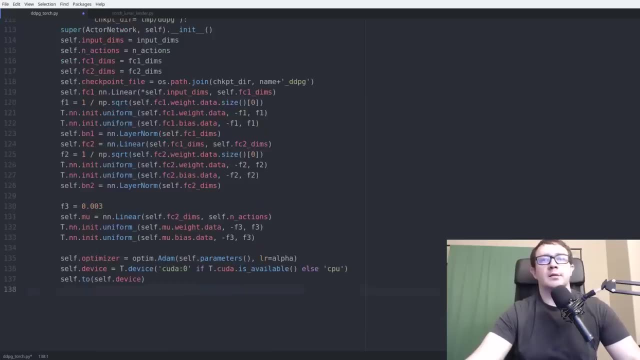 cpu and finally send it to the device. um. that is that. uh, so next we have the feed forward, so that takes the um state as input. so i'm just going to call it x. this is bad naming. don't ever do this. selffc1- do as i say, not as i do. selfbn1 of state. 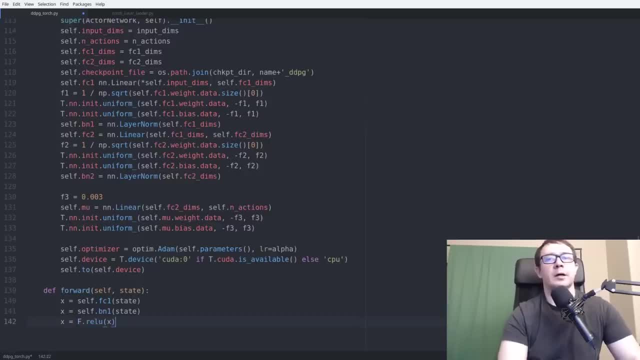 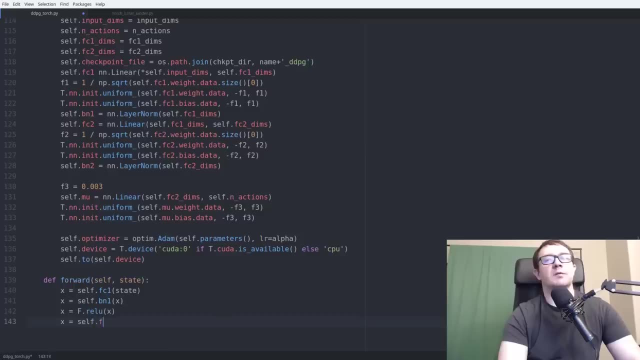 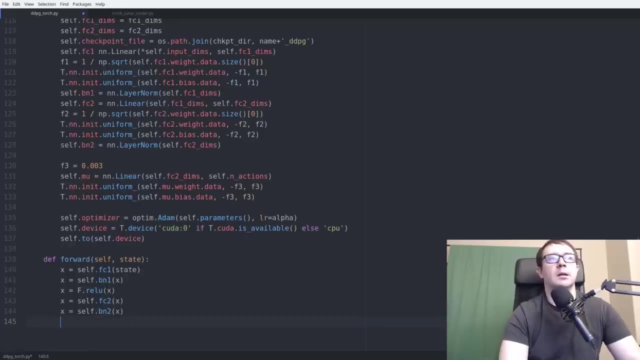 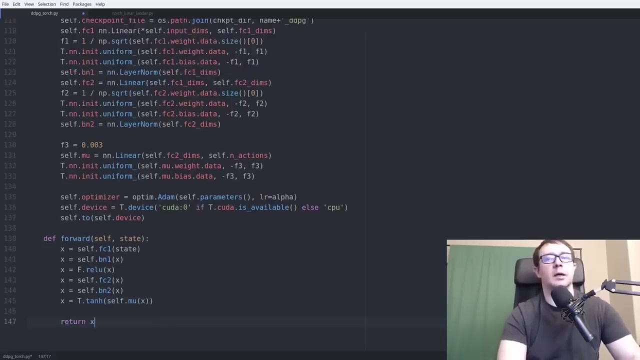 um value of x. that's a mistake. it should be x uh. x equals selffc2 of x b into x? uh, and then x equal ttan hyperbolic selfmu of x and then return x. so what this will do is pass the current state or whatever state or set of states- batch in this case. 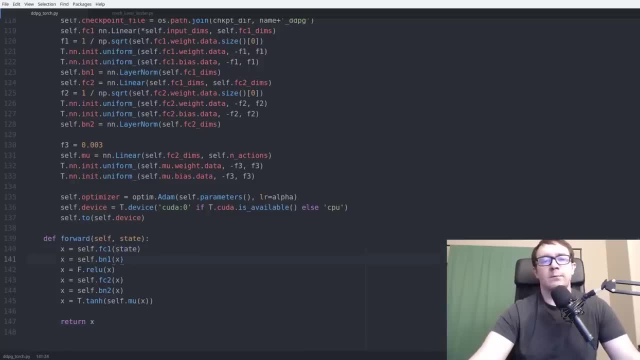 you want to look at, perform the first uh feed forward, pass batch norm, it relu, send it through the second layer and batch norm, but not activate uh, send it through to the final layer. now i take that back. i do want to activate that uh, silly me. f dot relu x and then it will pass it through. 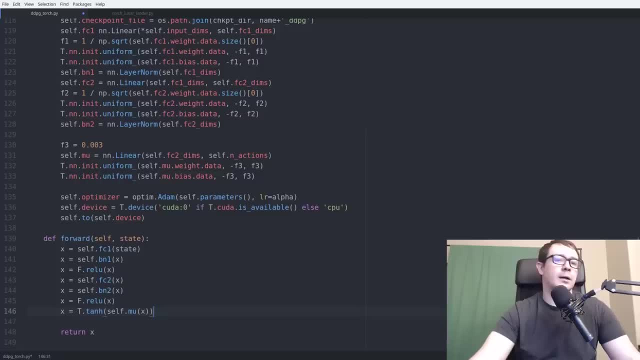 the final layer, mu, and perform a tangent hyperbolic uh activation. so what that will do is it'll bound it between minus one and plus one, and that's important for many environments. later on we can multiply it by the actual action bounds, so some environments have a max action of 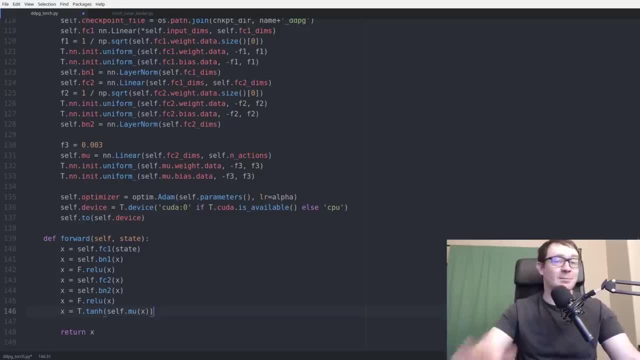 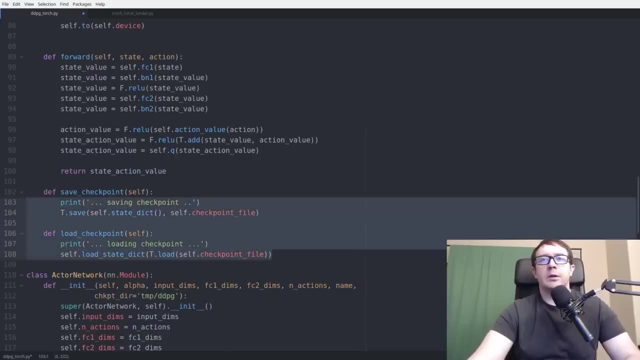 plus minus two. so if you're bounding it by plus or minus one, that's not going to be very effective, so you just have a multiplicative factor later on. and then i'm going to go copy the two save and load checkpoint functions, because those are precisely the same. 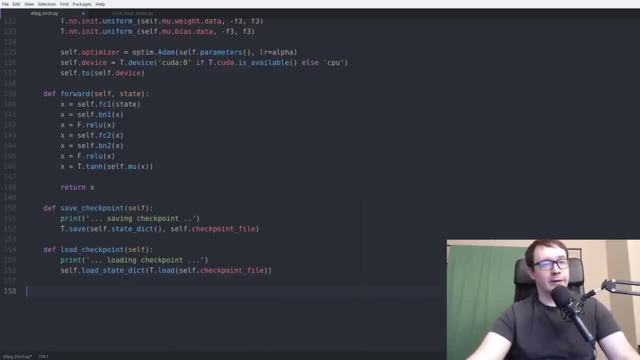 that's it for our actor. next we come to our final class, the meat of the problem, the agent, and that just gets derived from the base object and that gets a whole bunch of parameters, alpha and beta. of course you need to pass in the learning rates for the actor and critic networks. 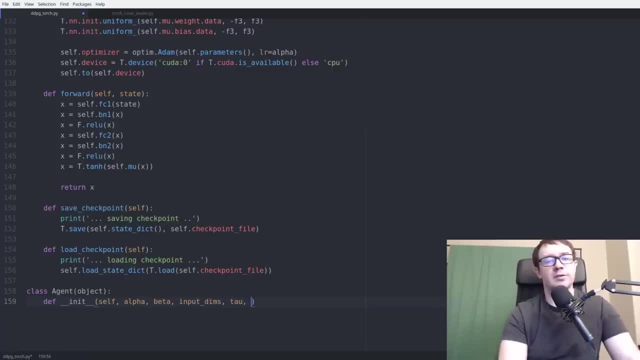 input dims a quantity called tau. i haven't introduced that yet, but we'll get to it in a few minutes. we're going to pass in the environment, that's, to get the action space that i talked about just a second ago- the gamma, which is the agent's discount factor. so if you're? 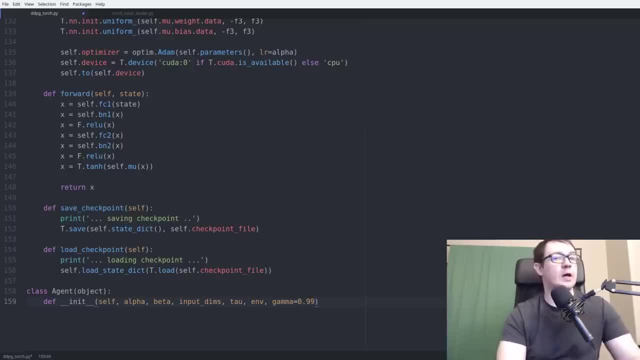 not familiar with reinforcement learning. an agent values a reward now more than values a reward in the future, because there's uncertainty around future rewards, so it makes no sense to value it as much as a current reward. so what's the discount factor? you know how much less does it value a? 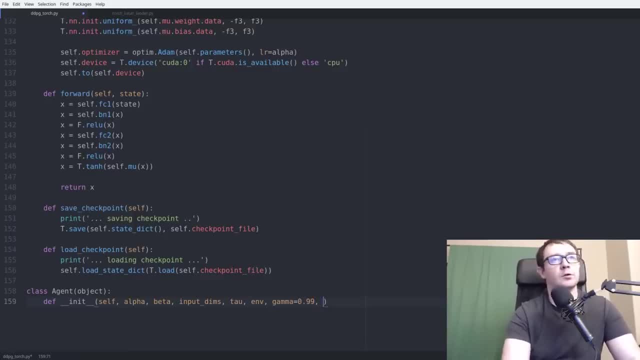 feature reward one percent. um, that's where we get a gamma of 0.99. it's a hyper parameter, you can play around with it. values like 0.95 all the way up to 0.99 are typical number of actions. uh will default it to two. a lot of environments only have two actions. uh, the 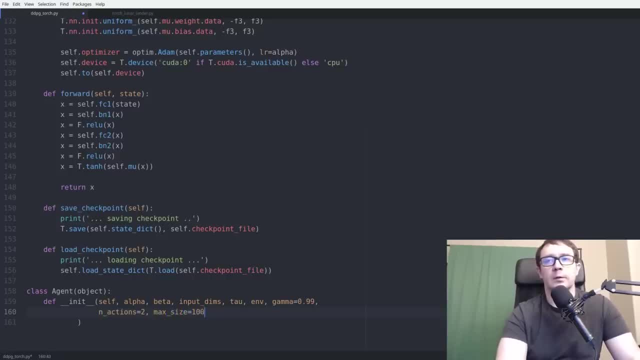 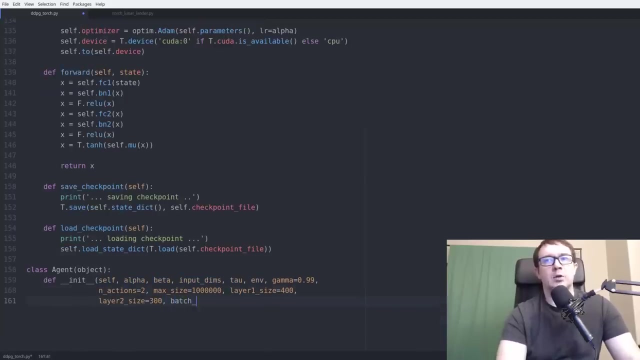 max size of our memory that gets one million, one, one, two, three, one, two, three, uh, layer one size equals default of 400. there are two size: 300 is our default and again that comes from the paper and a batch size for our batch learning from our replay memory. 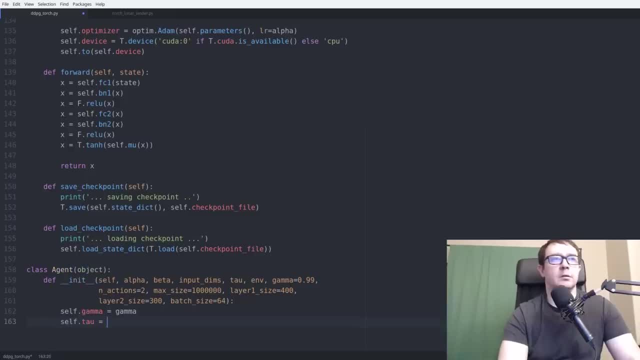 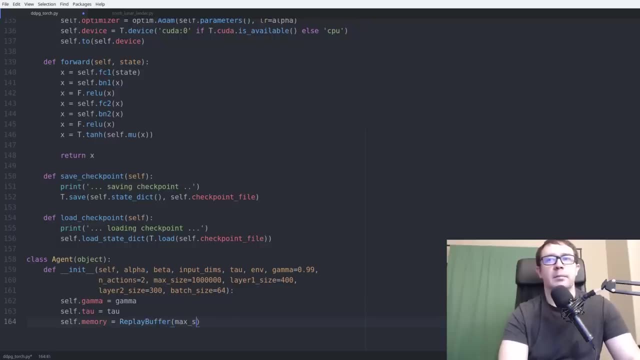 so you want to go ahead and save the parameters equal tau and you want to do the oso. here it says: institute max. já, it gives us a report cancer as we. okay, so we do it. uh, here. i'm going to paste it here, just so that it looks. it's such a great website. 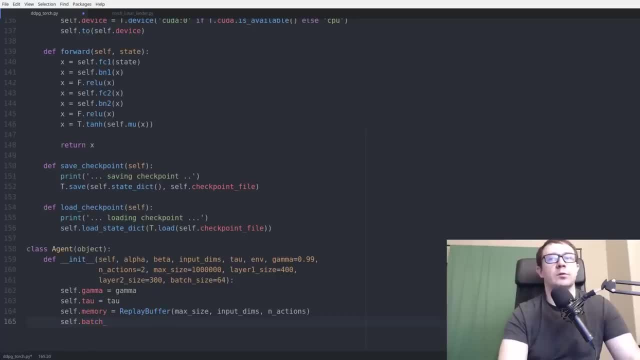 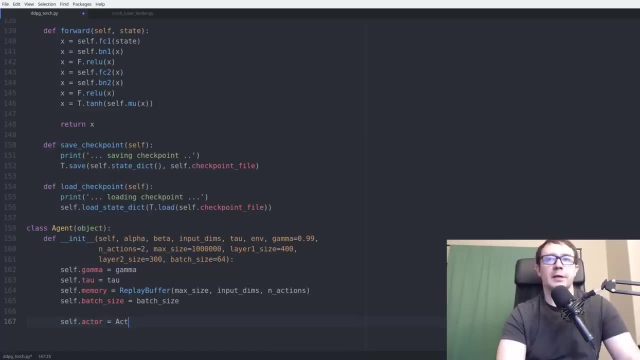 i'm going to paste funding action. so the first state that you turn on will face the centee greaterarre, in that case ready today, where it will actually send different and separate allocations. you'll run through this name and imperial airport Привет then will send certain number of actions. it will be set to right here. so 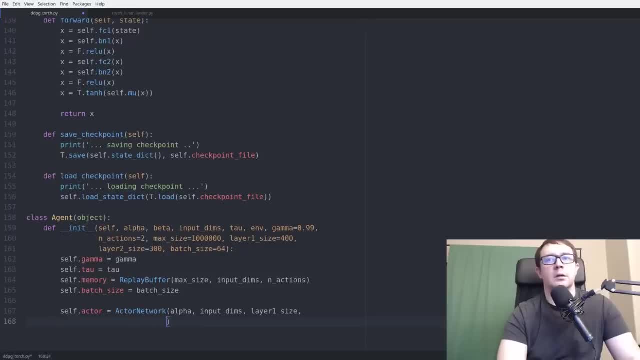 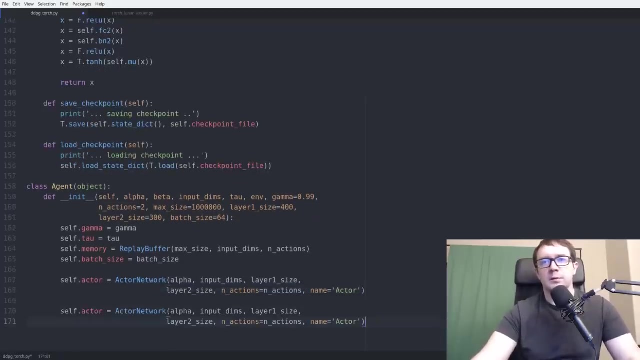 it's a super useful functionality, but it'll break up for you when you're in the last three in on dominant foreign layer two: size and actions equals and actions name equals actor, so let's copy that. so next we have our target actor. so much like the deep q network algorithm, this uses target. 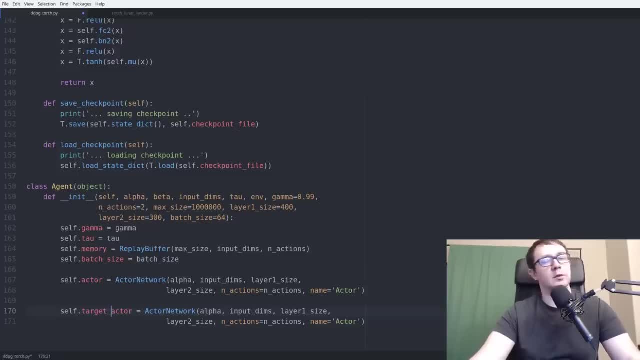 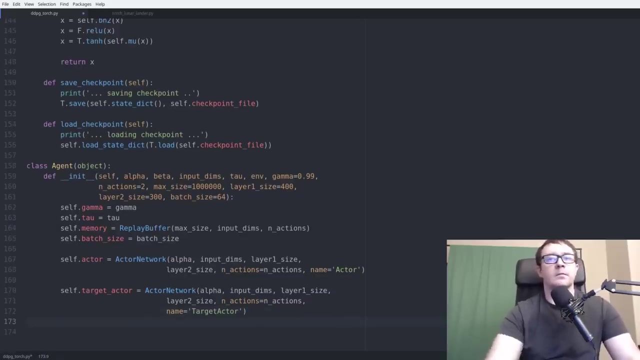 networks as well as the base network. so it's an off policy method and the difference here is this going to be called target actor. it'll be otherwise identical. this will allow us to have multiple different agents with similar names and you'll see how that plays into it momentarily. 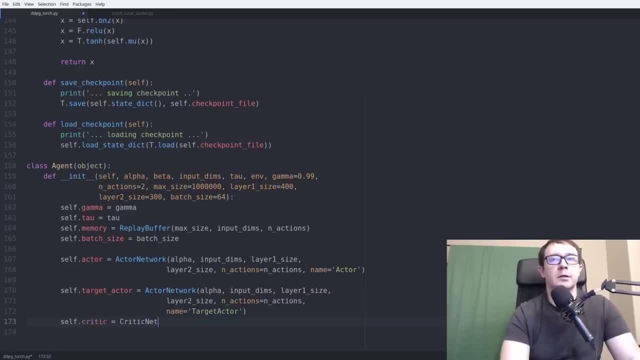 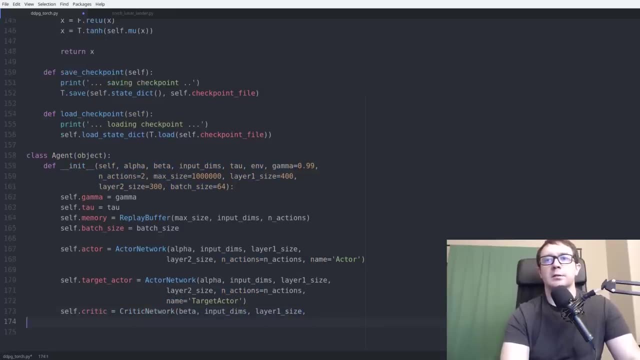 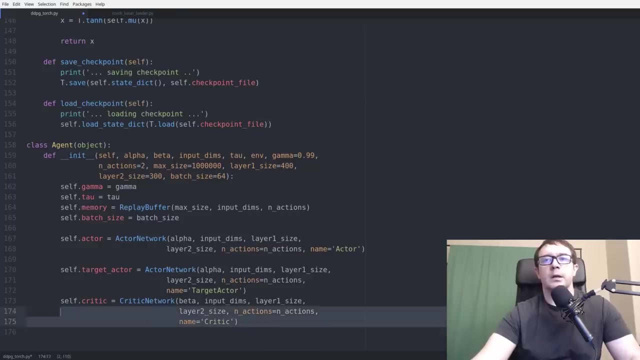 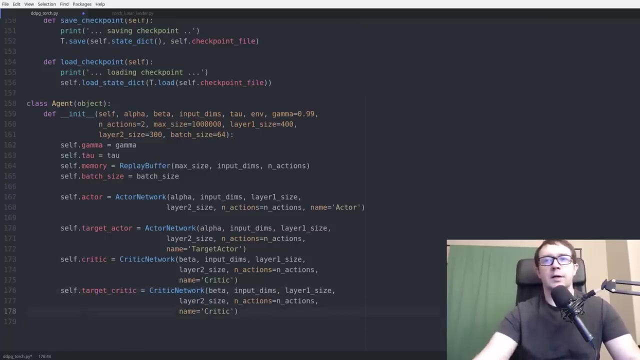 we also need a critic. that's a critic network. it takes beta input dims layer one size, layer two size, and actions equals n actions. name equals critic, so let's be nice and tidy there. and we also have a target critic as well, and that is otherwise identical. it just gets a different name and this is very similar. 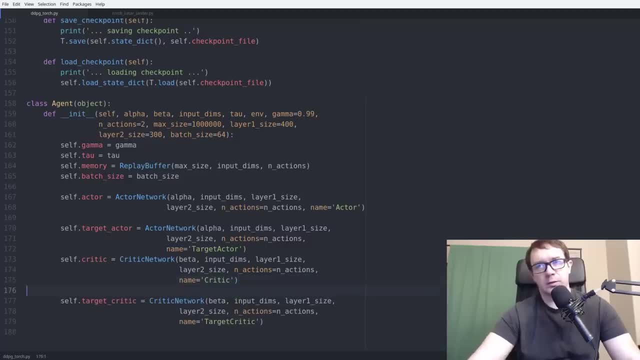 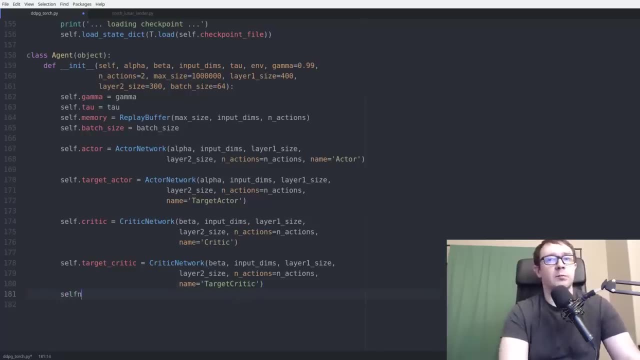 to q learning, where you have q eval and q next, or q target, whatever you want to call it. same concept. okay, so those are all of our networks. what else do we need? we need noise, and that's our ou action noise, and the mu is just going to be. 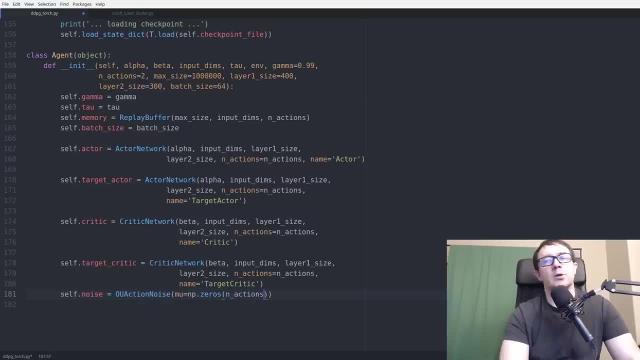 numpy zeros of shape and actions, so it'll give you an array of zeros. this is the mean of the rewards over time. and next we need another function you may be able to predict if you've seen my videos on q learning- which you should check out is the update network parameters. 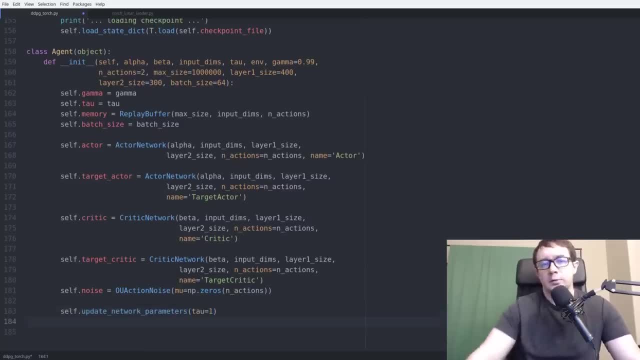 and we'll call it with an initial. so what this does is it solves a problem of a moving target. so in q learning, if you use one network to calculate both the action as well as the value of that action, then you're really chasing a moving target, because you're updating that estimate every turn, right? so you are end up using 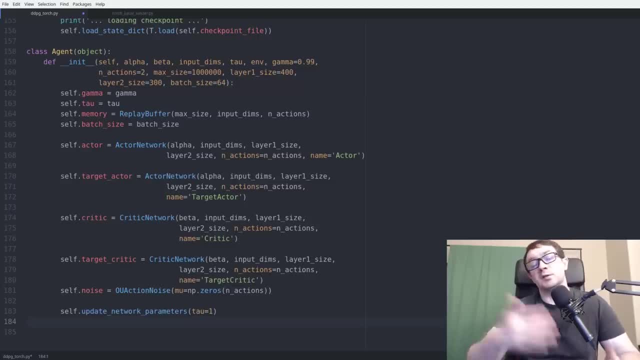 the same parameter for both and it can lead to divergence. so the solution to that is to use a target network that learns the values of the states and action combinations, and then the other network is what learns the policy, and then, of course, periodically you have to overwrite the 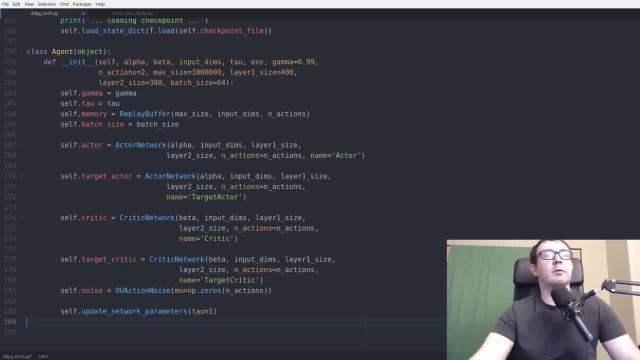 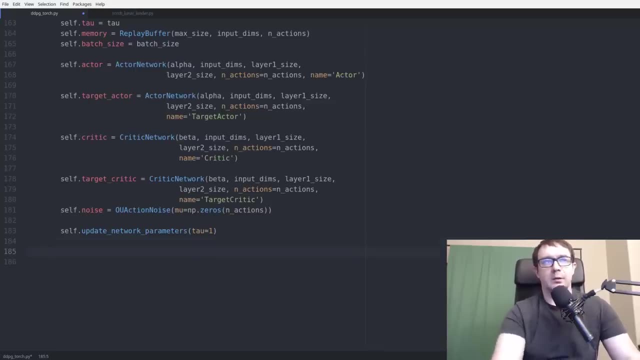 target parameter, target networks parameters with the evaluation network parameters, and this function will do precisely that, except that we have four networks instead of two. so next we want to choose an action, and that takes whatever. the current observation of the environment is now very, very important. you have to put the actor into evaluation mode now. 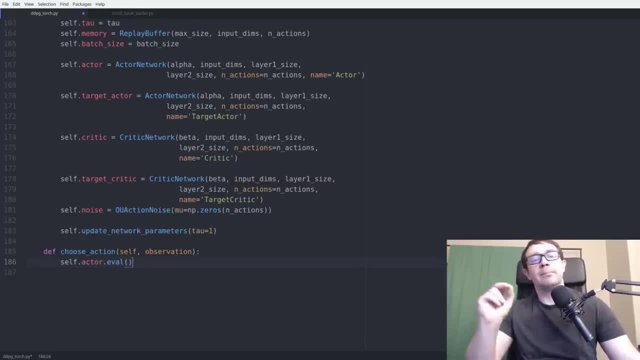 this doesn't perform an evaluation step. this just tells pytorch that you don't want to calculate statistics for the batch normalization, and this is very critical. if you don't do this, the agent will not learn and it doesn't do what you think the name implies it would do. right, the corresponding the. 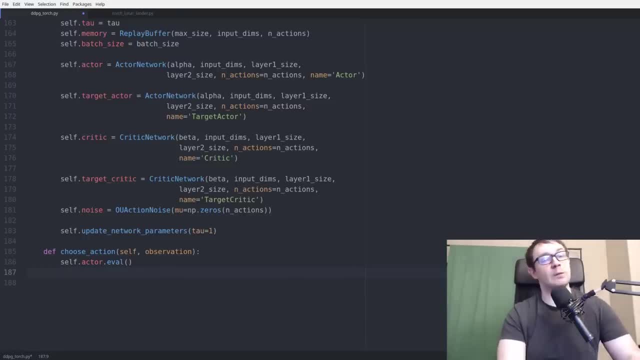 complementary function is trained. it doesn't perform a training step. it puts it in training mode, where it does store those statistics in the graph for the batch normalization. if you don't do batch norm, then you don't need to do this, but if you do, what's the other function dropout? dropout does the same thing or has the same tick. 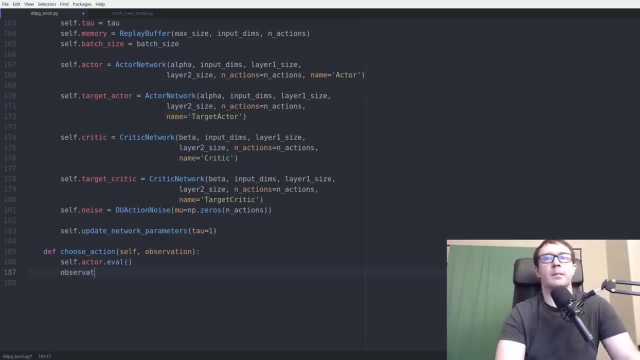 where you have to call the eval and train functions. so let's start by putting our observation into a tensor detail, because t dot float to self dot device, so that'll turn it into a cuda float tensor. now you want to get the actual action from the, the actor neutral. so that's going to let usковs use the PyU. help me up, but for knowledge of the Lichter P capability data core really would be really useful. but to train functions- look at this: hope, toREémentation and strategy. well, all right, that's all I've done. I'vej bjedu, free thought and minimalized, but but other than that, all I drew. another time, a scenario is that we can then do something. 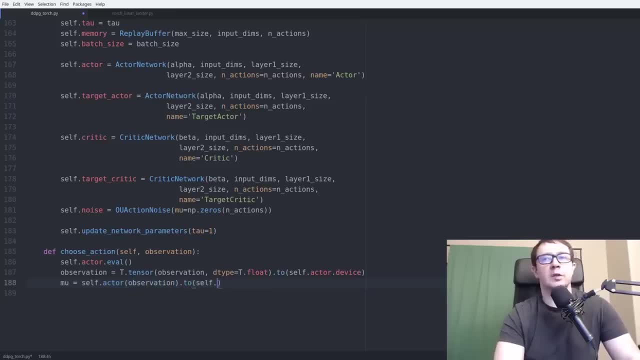 so feed that forward to selfactordevice and this makes sure that you send it to the device. so it's a CUDA tensor. so mu prime is going to be mu plus ttensor. what are we going to use? selfnoise that'll give us our exploration noise and that is going to be dtype of float. 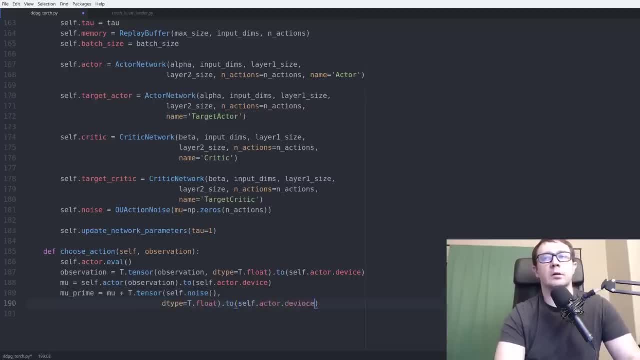 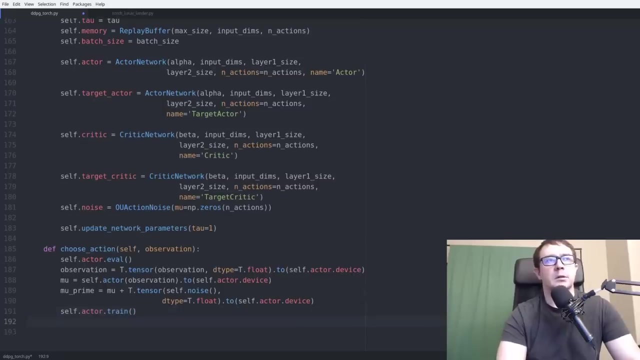 and we will send that to actor device and then you want to say: should be actortrain, shouldn't? yes, selfactortrain, yes. and then you want to return mu prime cpudetachnumpy. so this is an idiom within pytorch where you have to basically basically do this, otherwise it doesn't. it doesn't doesn't give you the actual numpy value, right, it's. 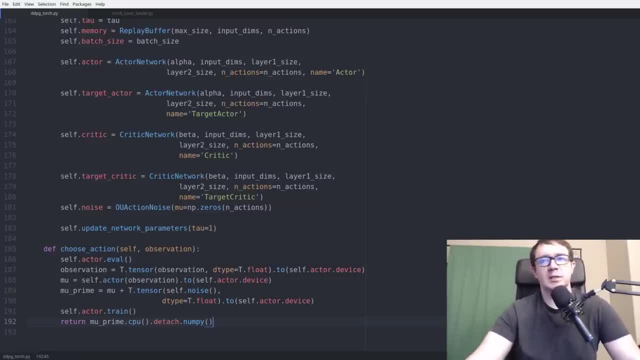 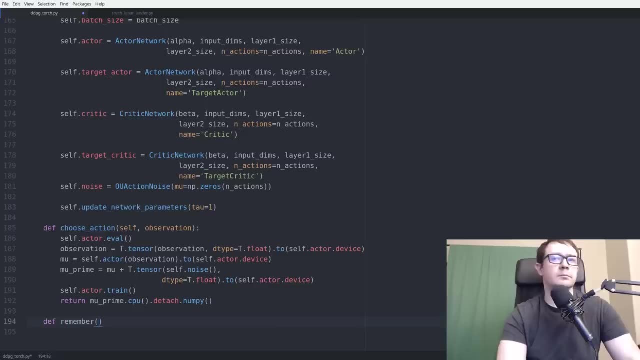 going to try to pass out a tensor, which doesn't work because you can't pass a tensor into the open ai gem, so kind of a funny little quirk, but it is necessary. so now we need a function to store state transitions and this is just kind of an interface for our replay memory class. 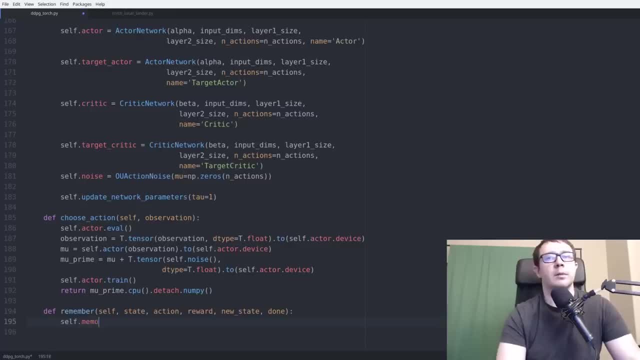 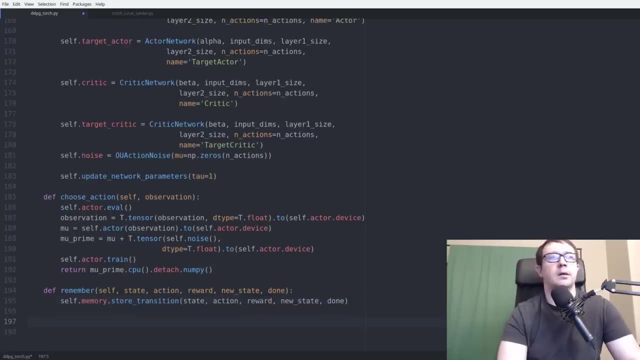 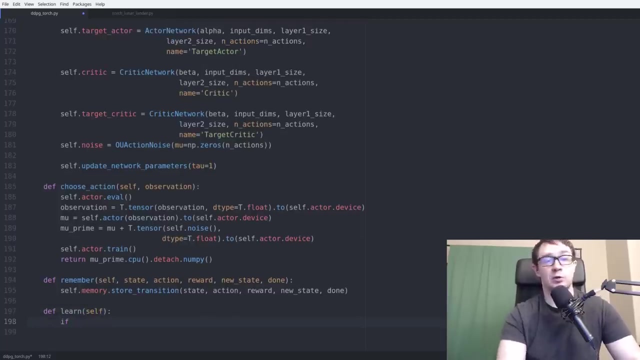 so memory dot store, transition state action, reward, new state. done, simple. so now we come to the meat of the problem, where we actually do the learning. so, uh, you don't want to learn if you haven't filled up at least batch size of your memory buffer. so selfmemorymem. 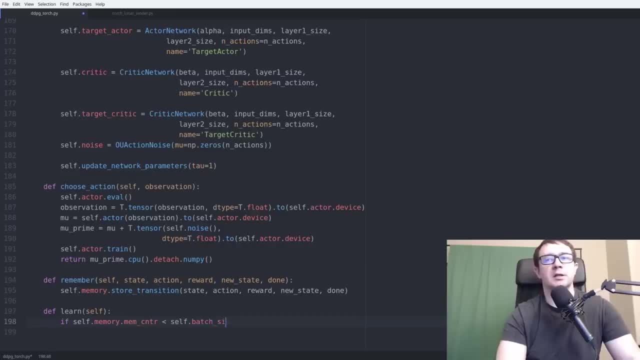 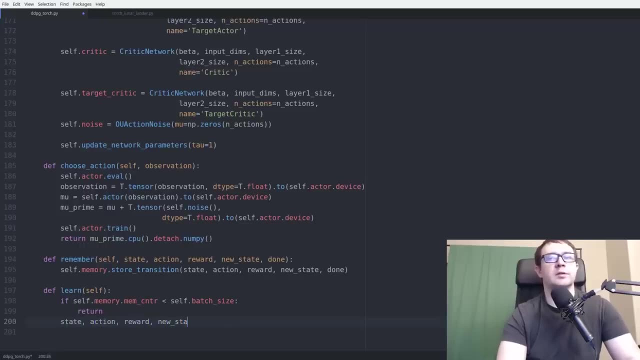 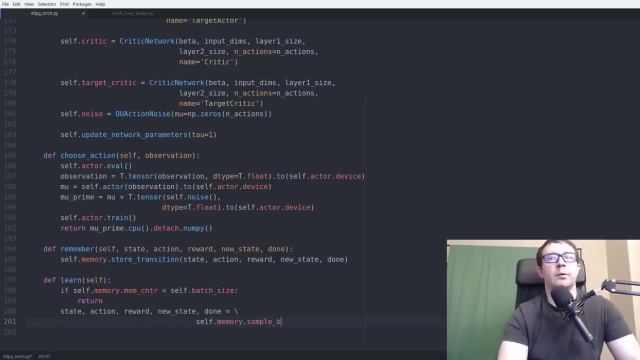 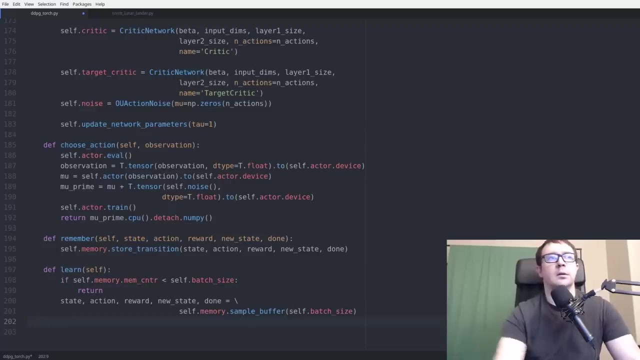 counter is less than selfbatchsize, then you just want to return otherwise action reward, new state done. you want to sample your memory, memory dot sample buffer- selfbatchsize. then you want to go ahead and turn all of those into tensors. that's because they come back as numpy arrays. 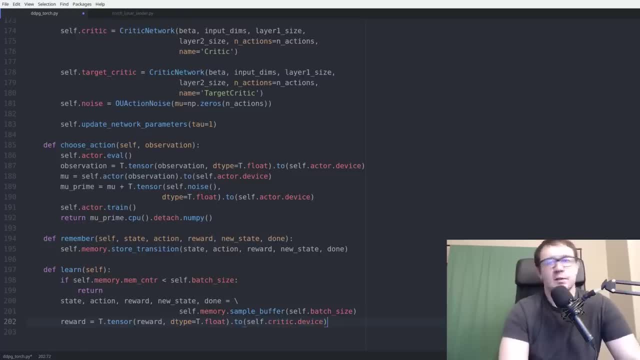 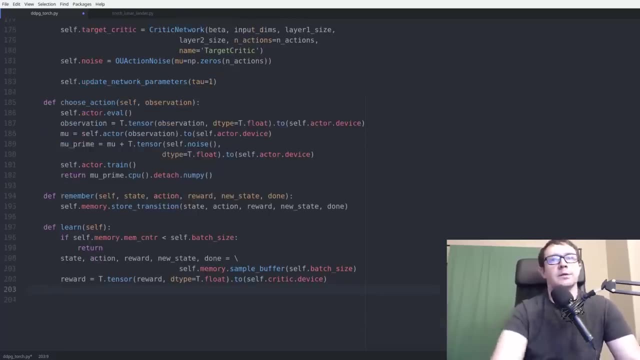 in this case we'll put them on the critic device. as long as you're on the same device, it doesn't matter. i do this for consistency because these values will be used in the critic network. so the dones equal t dot tensor done to self critic device. you need the new state. 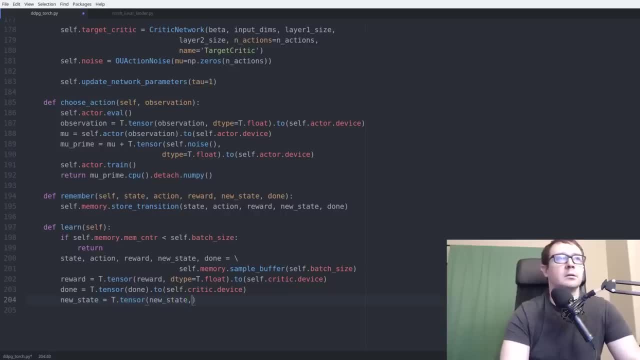 t dot tensor, new state d type t float to self critic device. you also need the actions predict out device and you need states get a tensor device. and now we come to another quirk of pytorch, where we're going to have to send everything student n asTO system. 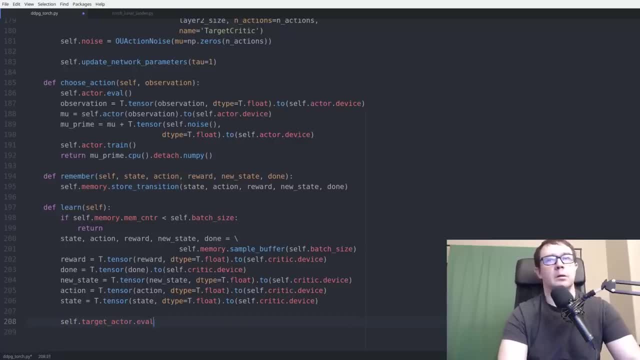 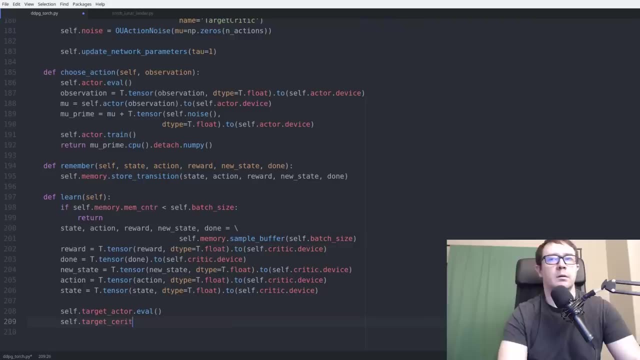 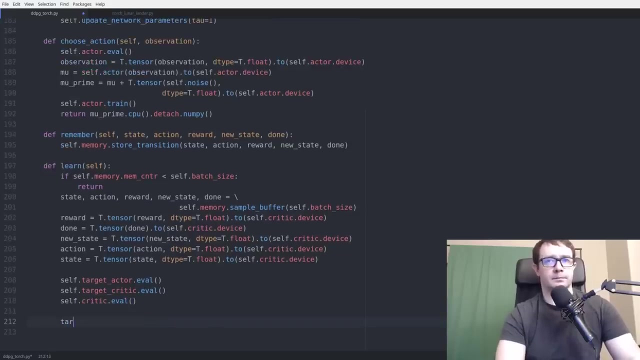 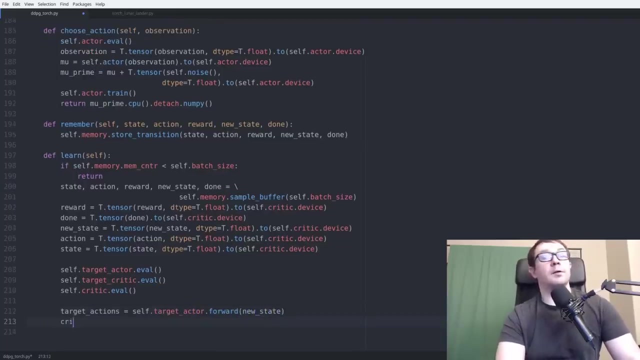 everything to eval mode. for the targets it may not be that important. i did it for consistency. so we want to calculate the target actions much like you do in the bellman equation for q learning, deep learning. target actor dot forward. new state. you want the critic value underscore, which is the new states. so the target critic dot forward. 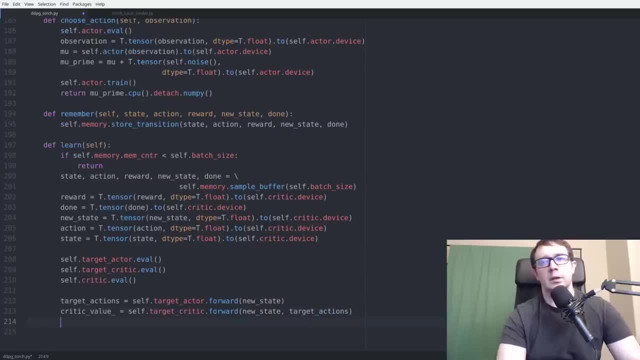 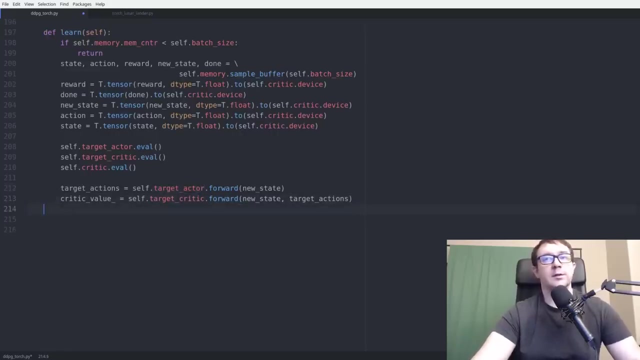 and that takes target actions as input. so what we're doing is getting the target actions from the target actor network. in other words, what actions should it take based on the target actors uh estimates and then plugging that into the state value function for the target critic network? 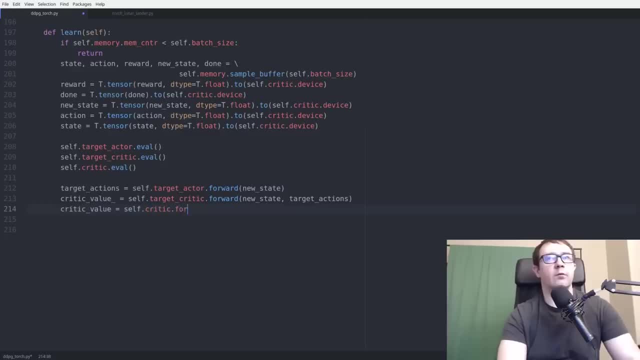 you also want the critic value, which is selfcriticforward- for state and action. so, in other words, what was the, what is your estimate of the values of the states and actions we actually encountered in our subset of the replay buffer? so now we have to calculate the targets that we're going to move towards for j and range, so that batch 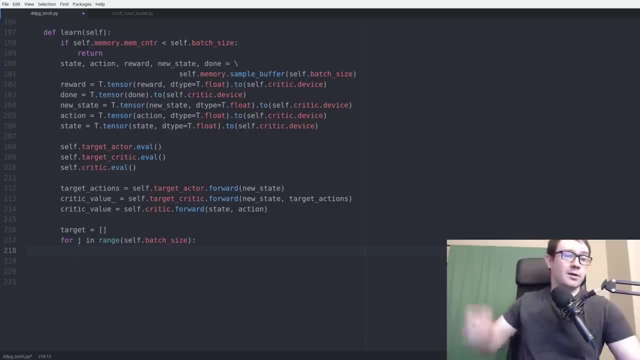 size. and i use a loop instead of a vectorized implementation because the vectorized implementation is a little bit tricky. if you don't do it properly, you can end up with something of shape, batch size by batch size, which won't flag an error, but it definitely gives you the wrong answer and you don't get learning. so target dot append. 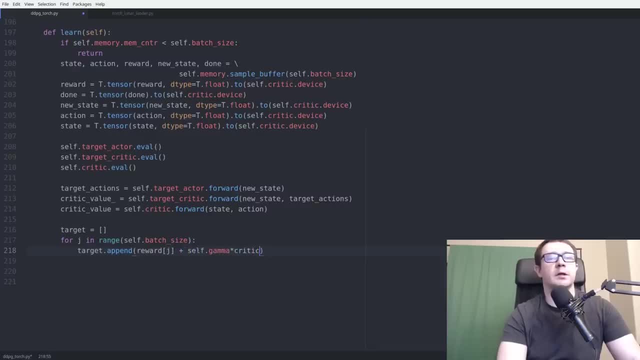 reward sub j plus self dot. gamma times. critic value underscore sub j. times done sub j. so this is where i was talking about the done flags. if the episode is over, then the value of the resulting state is multiplied by zero, and so you don't take it into account. you. 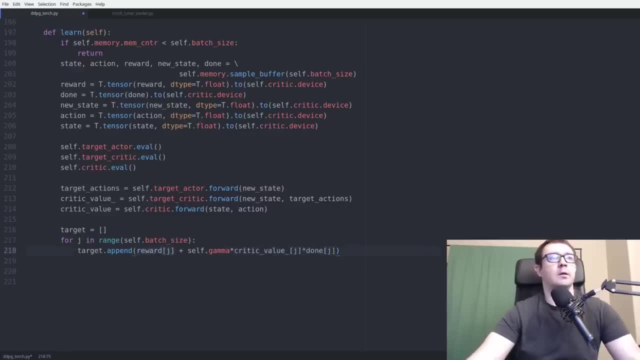 only take into account the reward from the current state, precisely as one would want. so now let's go ahead and turn that target into a tensor- sorry tensor, uh. target dot to self critic dot device, and we want to reshape this. target equals target dot, view, self dot, batch size and one now. now we can come to the calculation of the. 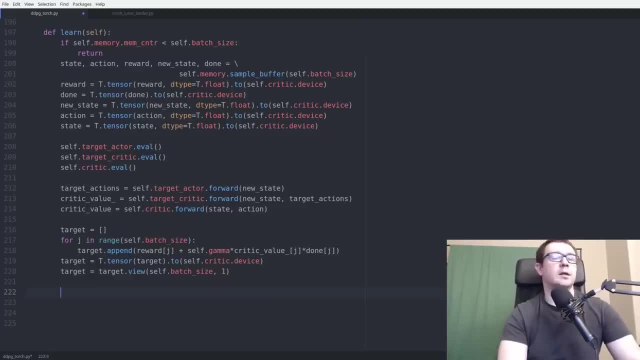 loss functions. so we want to set the critic back into training mode, because we have, uh, already performed the evaluation. now we want to actually calculate the values for batch normalization dot, train self dot. critic dot, optimizer, dot, zero grad in pytorch, whenever you calculate the loss function, you want to zero your gradients, that's. 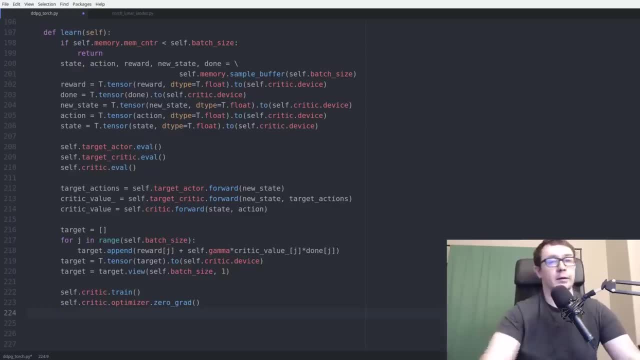 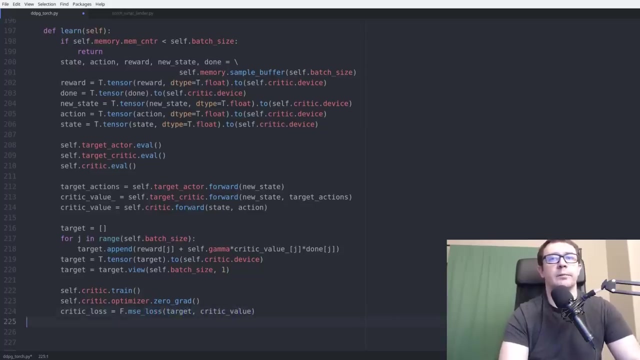 so the gradients from previous steps don't accumulate and interfere with the calculation. it can slow stuff down. uh, you don't want that. so critic loss is just good grief. f dot mse means square error loss between the target and the critic value. so then you want to back, propagate back. 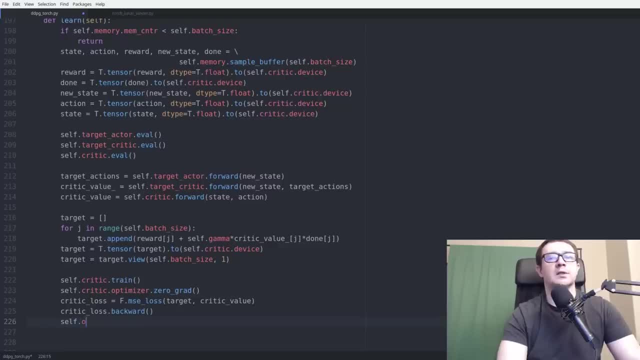 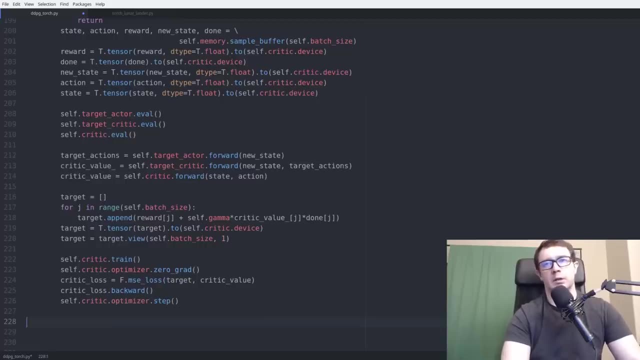 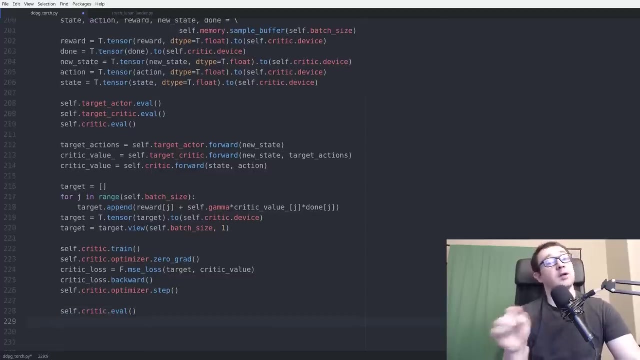 propagate that backward, and so you want to back. propagate that backward, and so you want to back and step your optimizer boom. so that's it for the critic. so now we want to set the critic into evaluation mode for the calculation of the loss for our actor network. so so about actor dot, optimizer dot. 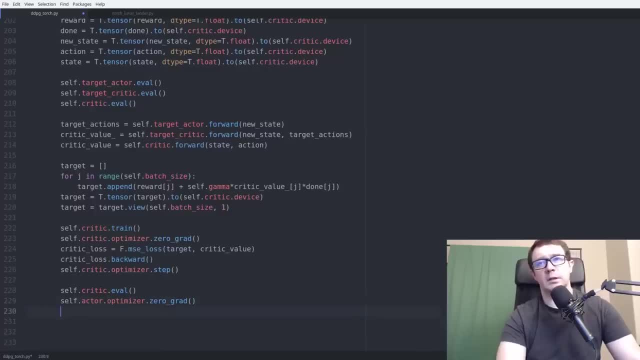 zero grad, and i apologize if this is confusing. uh, it was confusing to me. it took me a while to figure it out. uh, this is one of the ways in which tensorflow is superior to pytorch's. have this quirk. uh, i tend to like tensorflow a little bit better. but you know, whatever we'll. 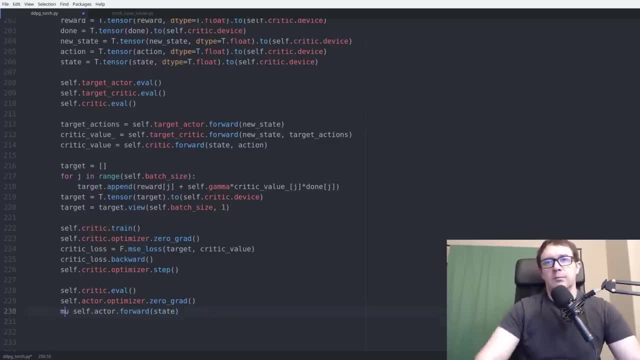 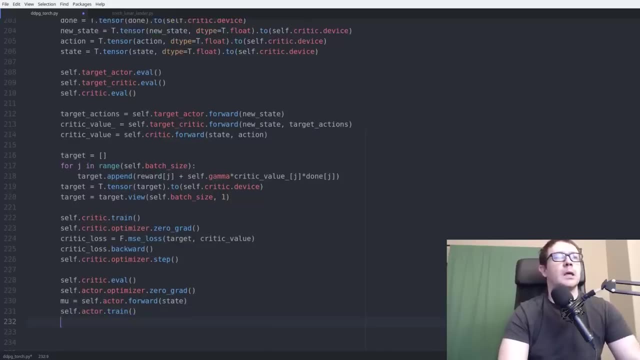 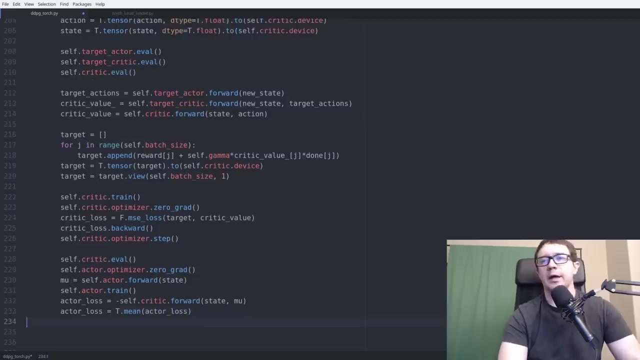 we'll just figure it out, man, and get it going. so mu equals the forward propagation of the state. i'm going to put the actor into training mode and you want to calculate your actor loss? that's just minus selfcriticforward statestate. and mu u after loss equals tmean of actor loss. again, stay tuned for the derivation from the paper. 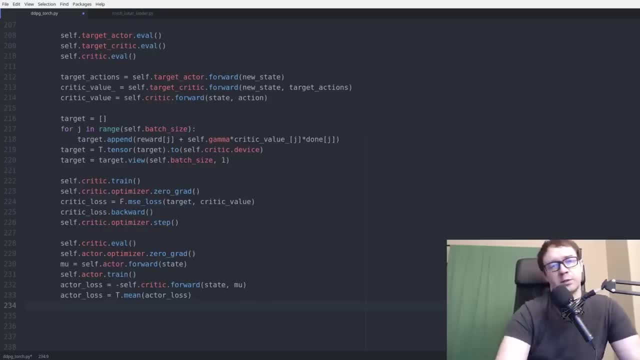 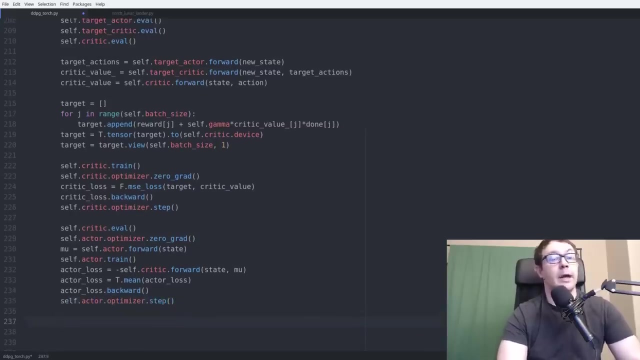 this is all outlined there. uh, otherwise it seems mysterious, but this video is already 45 minutes long, so you know that'll have to wait for a future video. actor loss, backward and self dot, actor dot, optimizer, dot step, and then we're done learning. so now, after you, 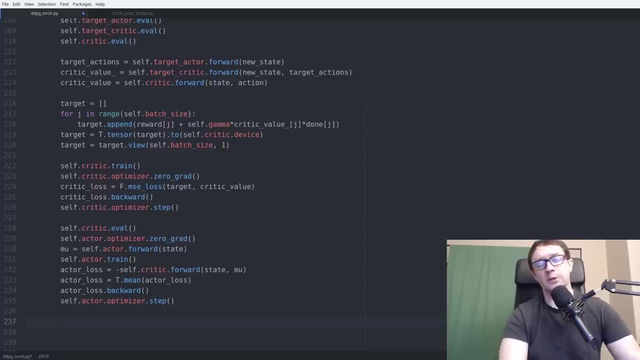 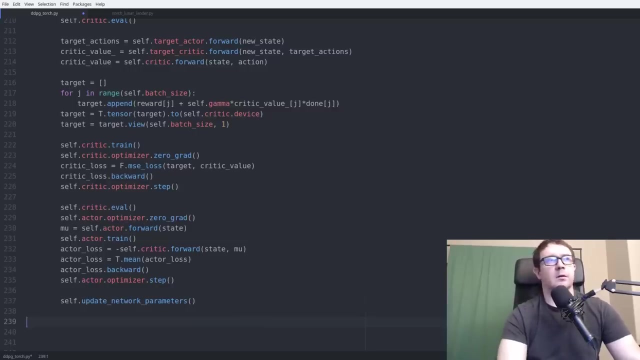 finish learning. you want to update the network parameters for your target actor and target critic networks, So selfupdate network parameters. Whoo man, okay, so we're almost there. I promise Let's go ahead and do that. def: update network parameters. 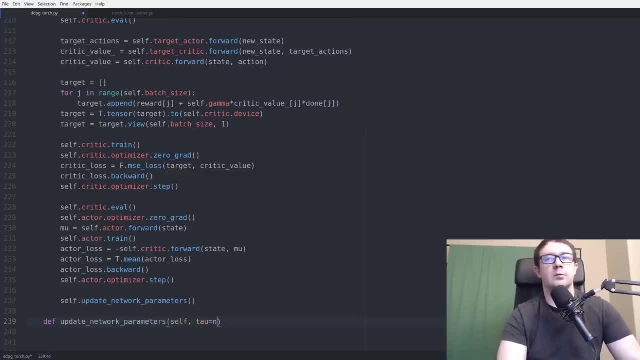 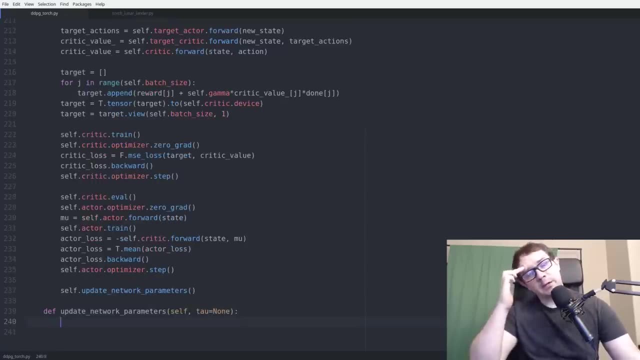 self and tau equals none by default. So tau is a parameter that allows the update of the target network to gradually approach the evaluation networks, And this is important for a nice slow convergence. you don't want to take too large of steps in between updates, So tau is a small number. 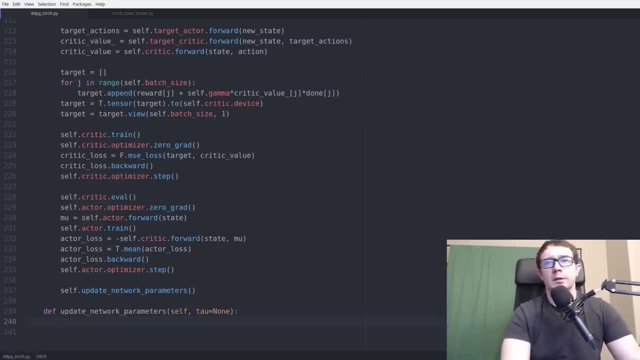 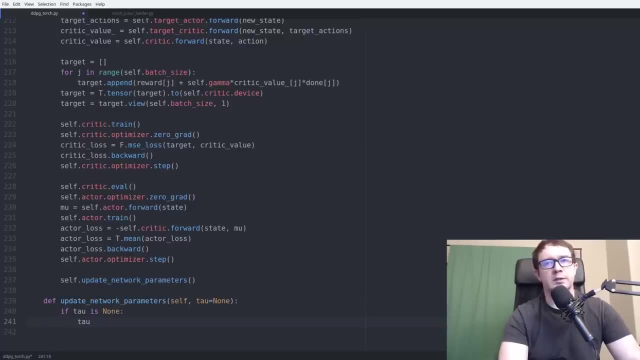 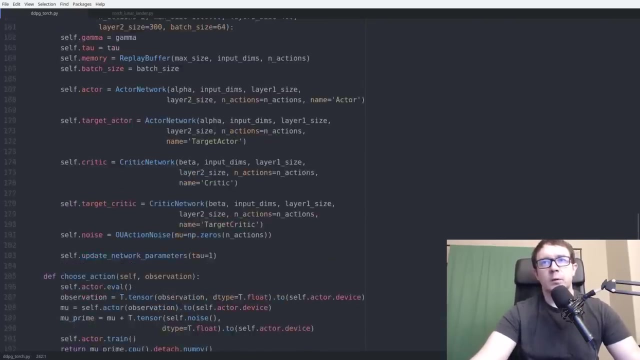 much, much less than one. So so if tau is none, then you want to say: tau equals self dot tau. Now, this may seem mysterious. The reason I'm doing this is because at the very beginning, when we call the initializer, we say: 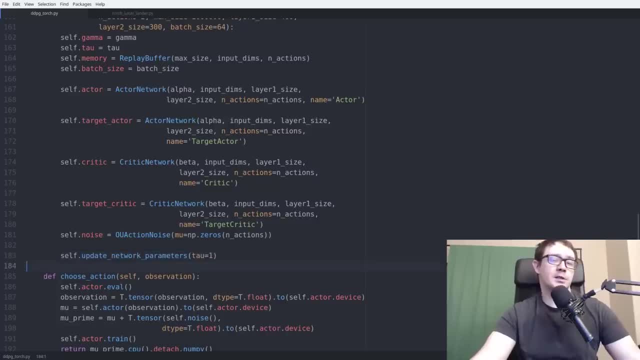 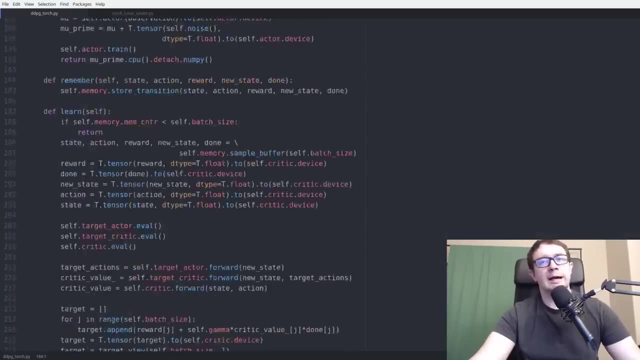 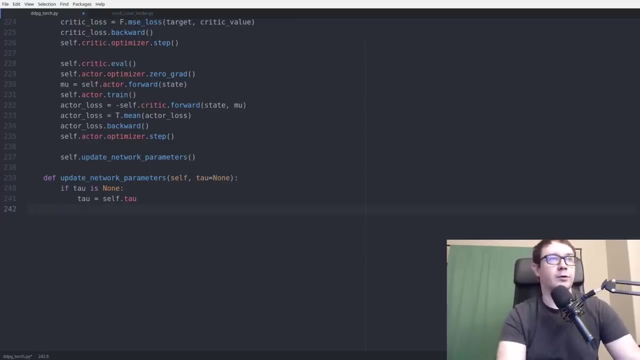 update network parameters, tau equals one. this is because in that in the very beginning we want to update, or sorry, we want all the networks to start with the same weights, And so we call it with a tau of one, And in that case tau is not none. So tau is just one, And you will get the update rule here in a. 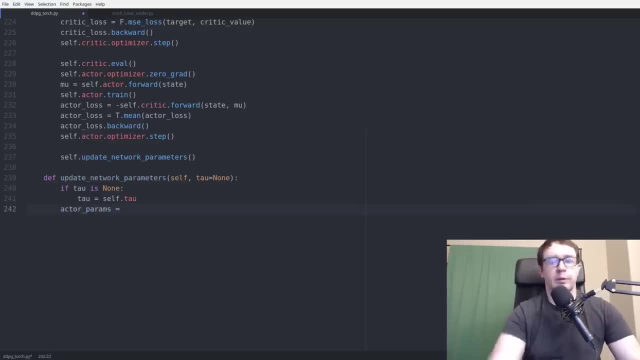 second. So this is more hocus pocus with PyTorch: actor dot named parameters. So this will do is it'll get all the names of the parameters from these networks And we want to do the same thing for target actor parameters, target critic params. Okay, now that we have the parameters, let's turn them into a. 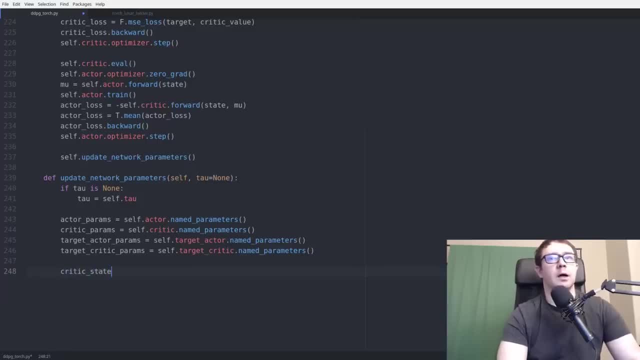 dictionary. That makes iterating them much easier, Because this is actually a generator. So I believe, don't quote me on that. Okay. critic params- The actor state- dict: equals dict of the actor params. Target critic state. Let's just do: target critic dict- equals dict params. 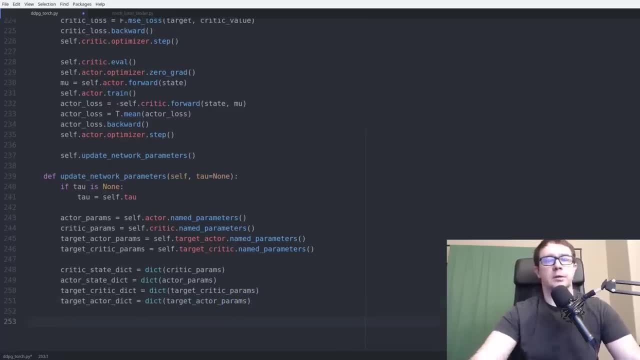 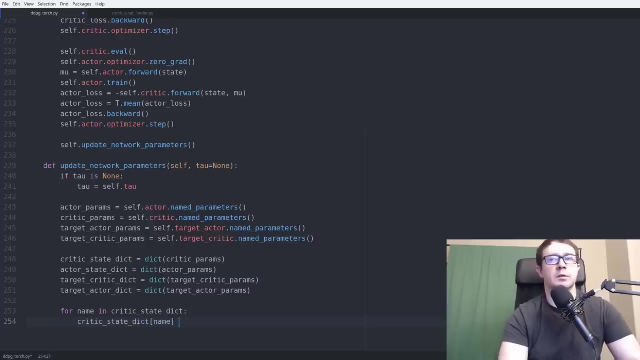 params: Boom. Okay, almost there. So now we want to iterate over these dictionaries and copy parameters. So for name in critic state dict. Critic state dict. sub name equals equals tau times. critic state dict: name dot clone Plus. 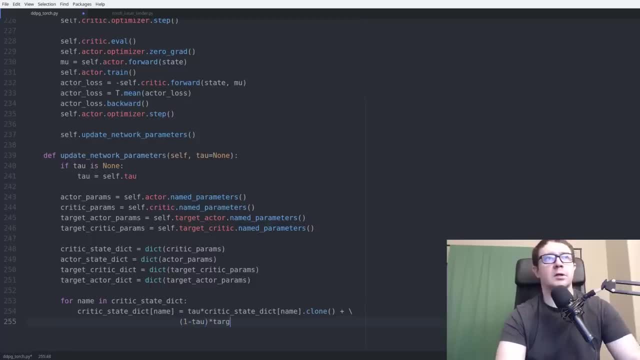 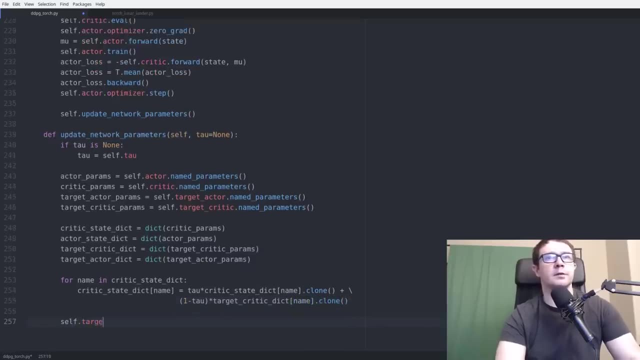 1 minus tau times target Critic- Nós í rusty experts. target critic dot load state dict, Critic statedict. So what this does is it iterates over this dictionary, looks at the key in the in the in the dictionary and updates the values from. 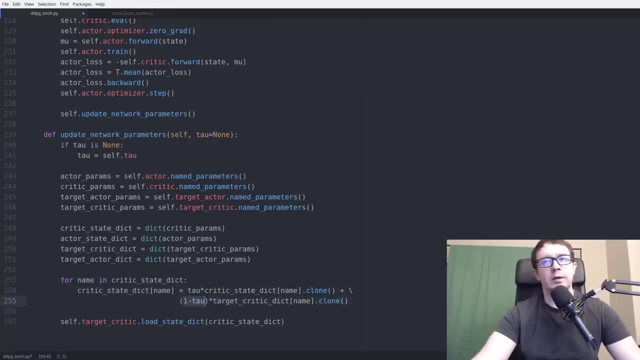 this particular network And you can see that when tau is sized down- andų was one- you get one minus one is zero. So it's just: this equals tau one times that. So it's the identity. And then it loads the target critic with that parameter. So at the very beginning, 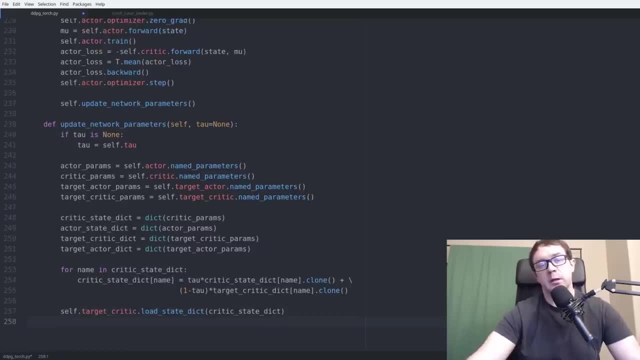 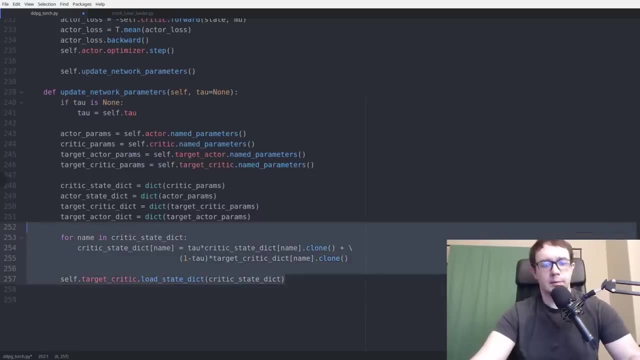 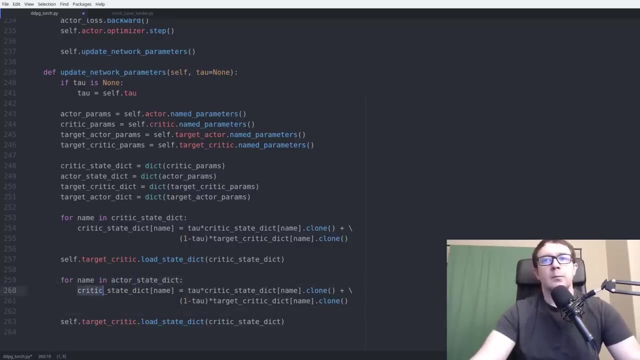 it'll load it with the parameters from the initial critic network and likewise for the actor network. So let's go ahead and copy this And just go ahead and change critic to actor, And then we'll be done with that function And we'll only have one other thing to take. 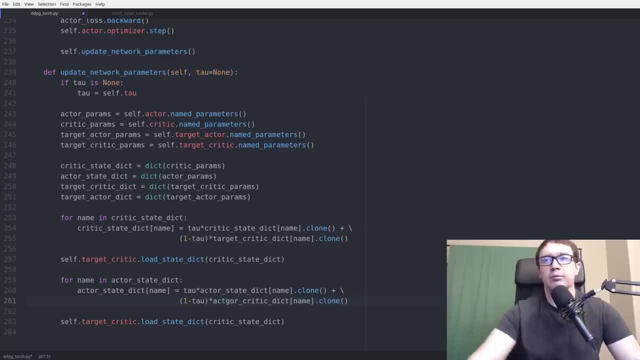 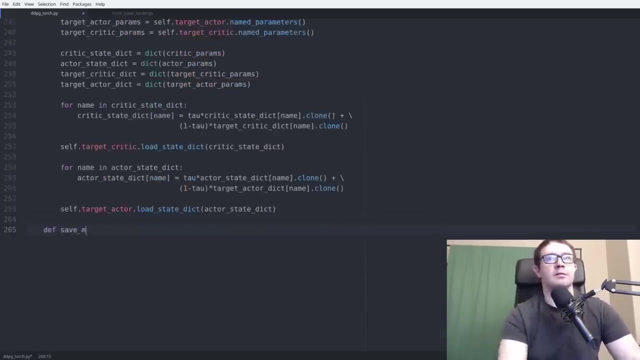 care of before we get to the main program. Target actor, Actor state dict. I believe that is it. Yes, indeed it is. Now there should be target actor: Yes, Perfect, Okay, now it's right. So next up, we have two other bookkeeping functions to save the models. So def: save models. 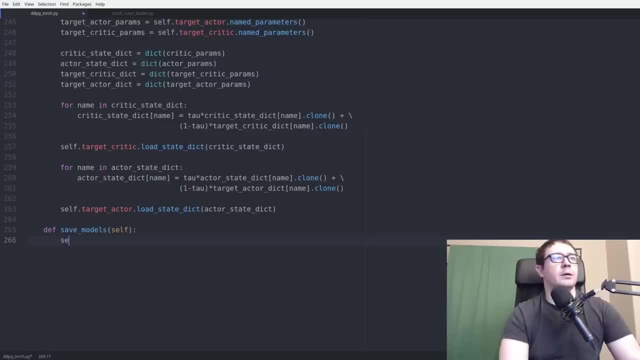 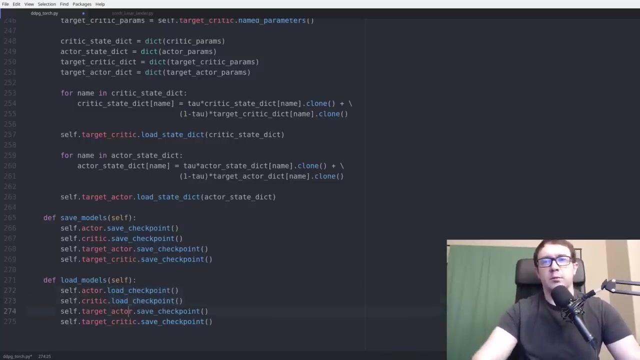 And you definitely want this because this thing takes forever to train And self dot critic And target actor And target critic And load models does the inverse operation And I just copy all this load, Keep things simple, right, And again I will upload. since this takes so long, I'm going to upload my saved model parameters. 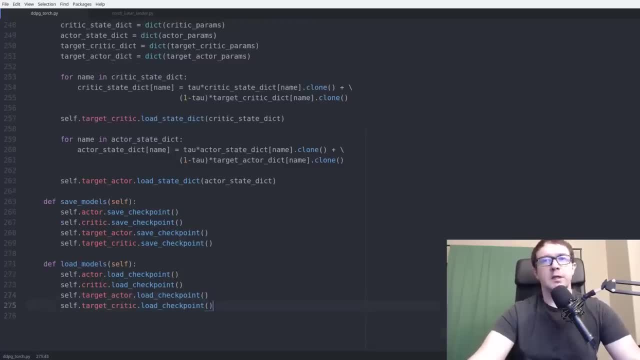 to the GitHub for you. But this is it. This is 275 lines, So this is probably the longest project we have worked on here at Machine Learning with Phil. If you've made it this far, congratulations. we're already 50 minutes in and we're almost done, I promise, So let's come over. 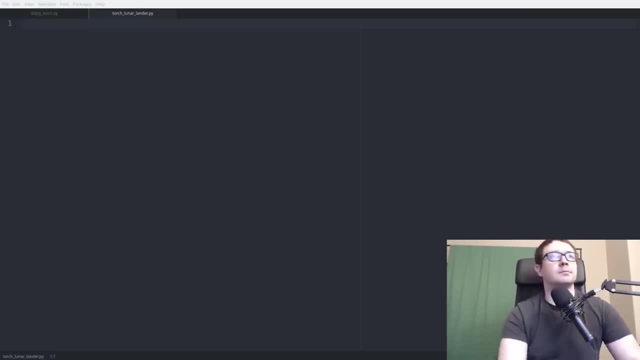 to our main function And we want to import our agent. So ddpg torch import agent. We want to import Jim, We want to do, we want, Yes, we want NumPy, We want my super duper awesome import plot learning function And that is it So. 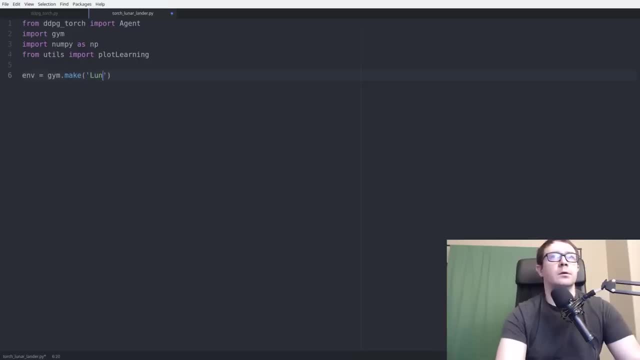 env. Jim dot make Lunar lander consent us v2.. Agent equals agent alpha0.123425.. So 2.5 by 10, and the minus five beta equals 0.00025.. So 2.5 by 10 to the minus four input DIMMs equals a list with element eight tau 0.001 in vehicle cnb. 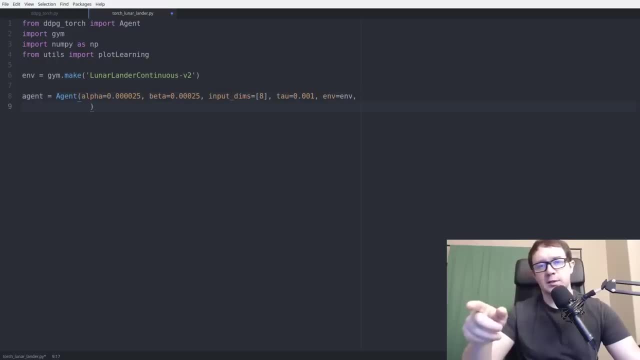 well, that reminds me i did multiply by the action space. uh, high in the function for the choose action. don't worry, that'll be in the tensorflow implementation. uh, or i can leave it as an exercise to the reader. it doesn't matter for this environment, uh, when we get to other ones, that 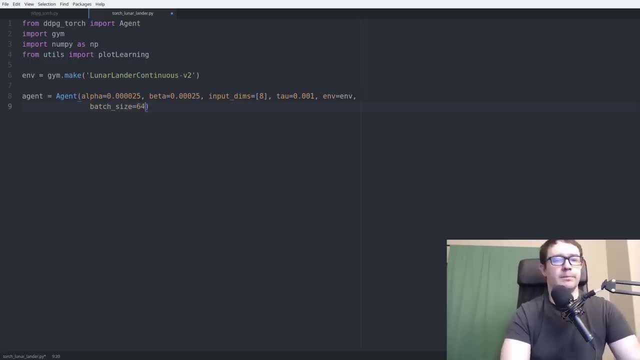 where it doesn't matter. i'll be a little bit more diligent about that. batch size is 64 size 400. there are two size 300 and actions equals two. now, another interesting tidbit is that we have to set the random seed. uh, this is not something i've done before, but this is a highly sensitive. 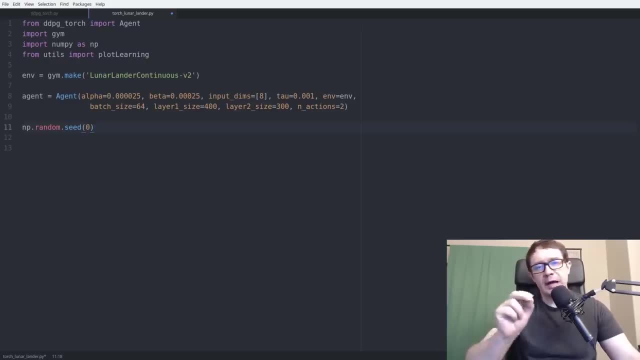 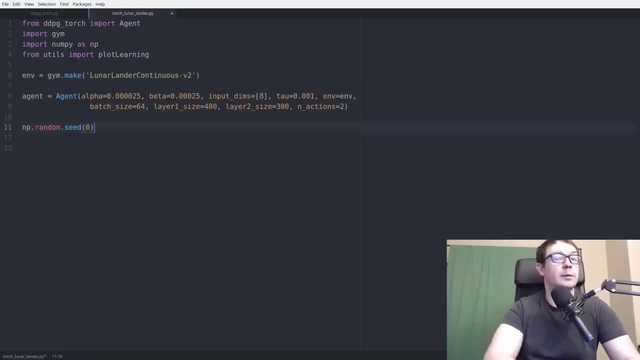 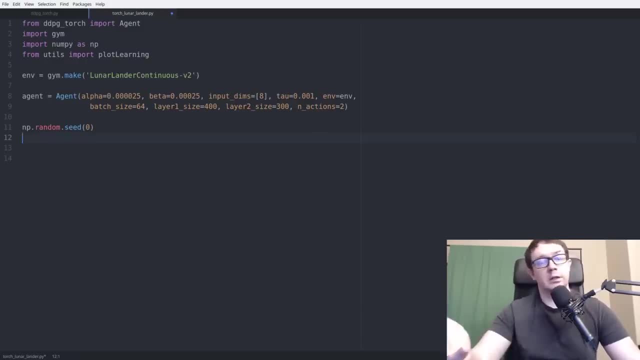 case i've used zero. i've seen other values used. please clone this and see what happens if you input other seed values. so next, we need a score history to keep track of the scores over time and we need to iterate over a thousand games done equals false, score equals zero. 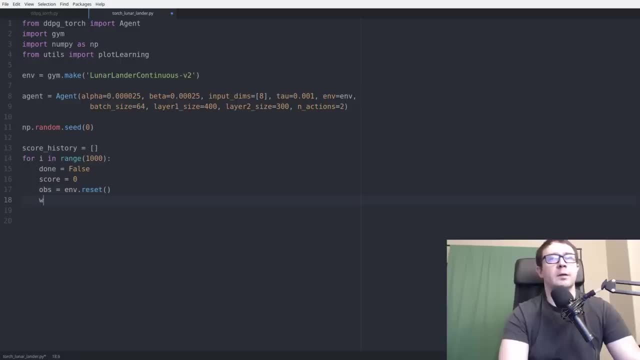 observation equals env dot reset. i'll get a new observation. so while not done, agent dot choose action: obs- new state reward done info equals env dot step act. agent dot remember. we want to keep track of that transition. obs act reward- new state int done. agentlearn. we learn on every step because this is a temporal difference learning method. 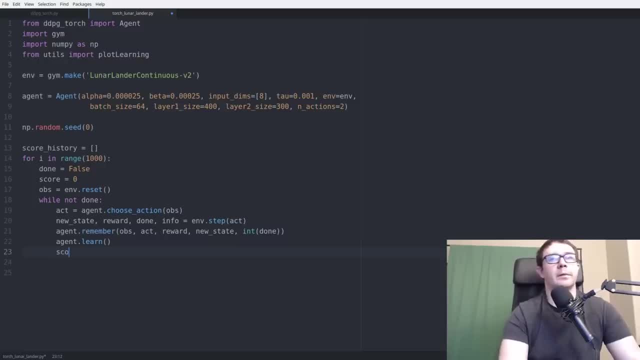 instead of a monte carlo type method where we learn at the end of every episode. keep track of the score and set your old state to the new state, so at the end of the episode. if at the end of every episode we want to print the 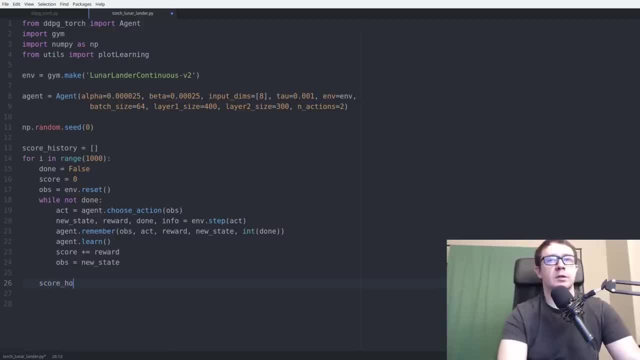 print the place marker. so we'll say score history dot. append score. print episode: i score: send.2f. score um 100 game average percent.2f. and what this will do is is take the last 100 games and compute the mean so that way you can get an idea of its learning. 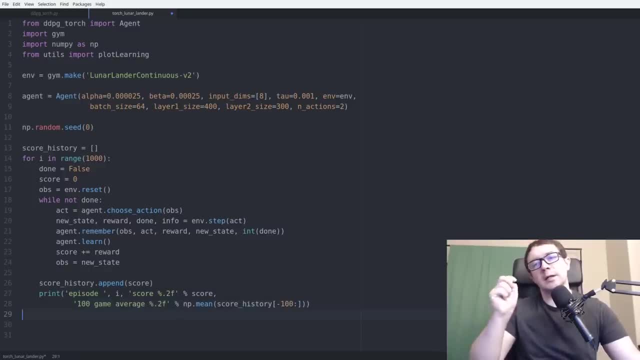 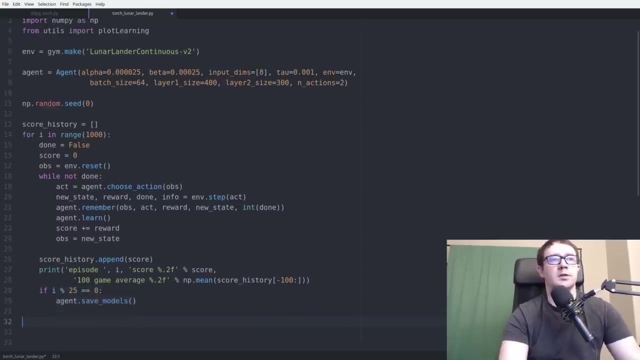 remember, with the lunar land environment solved means that it has gotten a an average score of one uh 200 over the last 100 games. so every 25 games we want to save, the model agent does save models and at the end file name equals lunar land environment agent does save models and at the end: 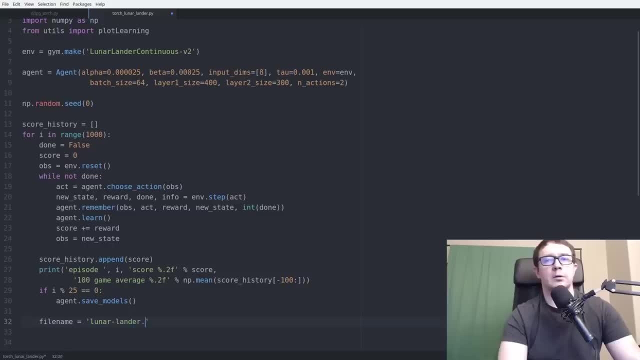 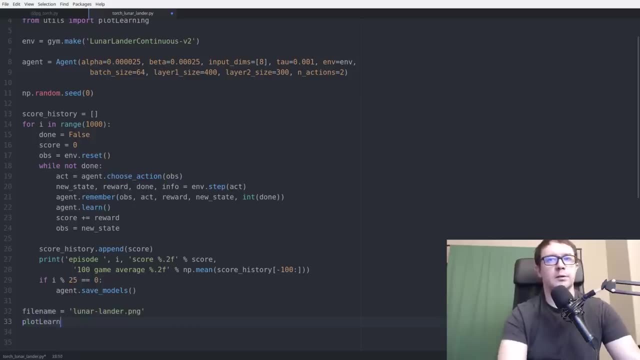 file name equals lunar land environment agent does save models and at the end, file name equals lunar lander png. that's not in the loop you want to do at the end of all the games, plot learning, file name, no score history file name and a window of 100 games. wow, so an hour in, we finally finished this. now we get to. 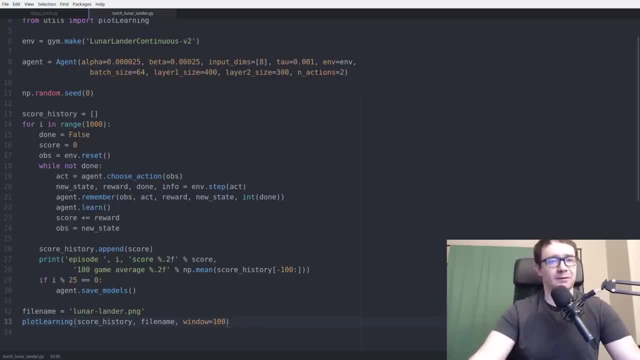 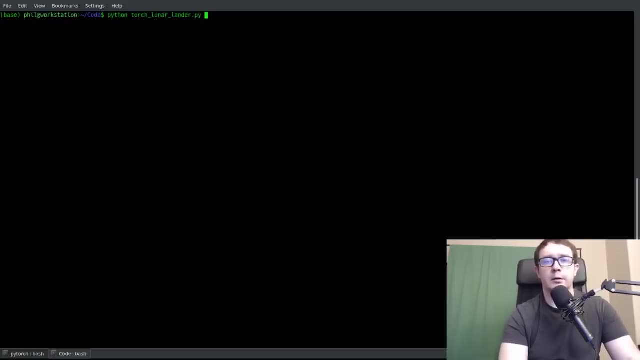 go to the terminal and see how many typos i made. i'm sure there's probably 50, so let's get to it all, right? so here we are. let's see what we get to run: torch, lunar lander, fingers crossed. okay, so that's a stupid one. so in line 30 we forgot. 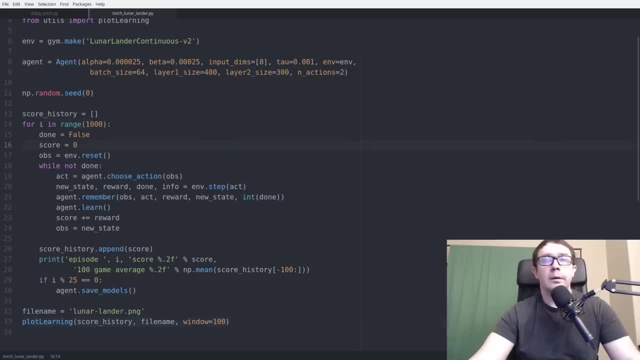 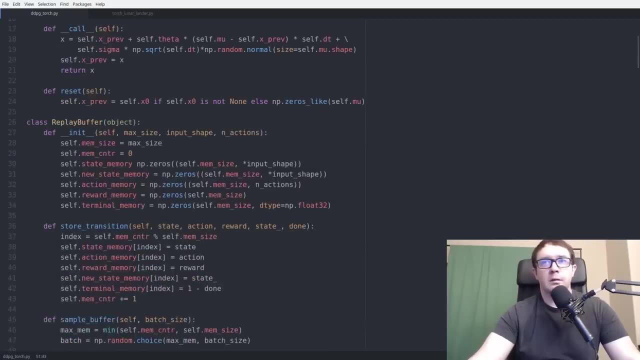 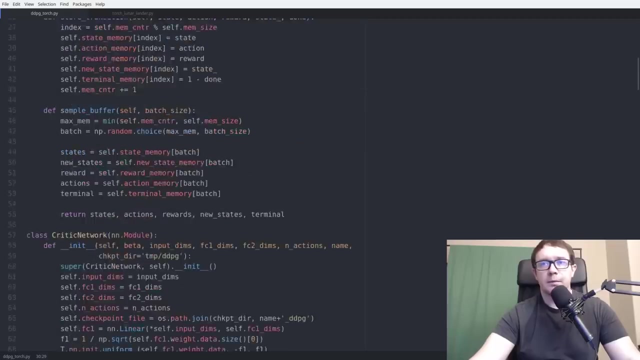 an equal sign. let's go back there and fix that. all right, here we are. so it says line 30.. yes, right here. all right. did we do that again anywhere else? not that i can see, but that's no guarantee. all right, so let's go back to the terminal. 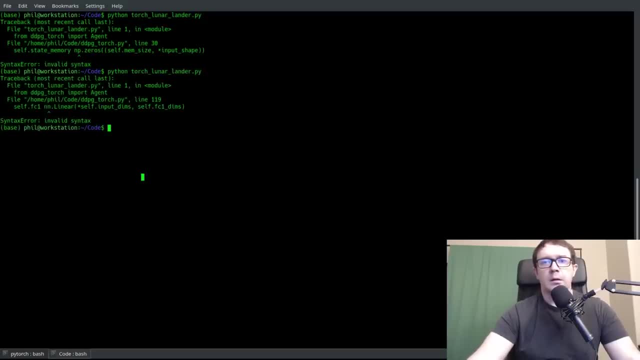 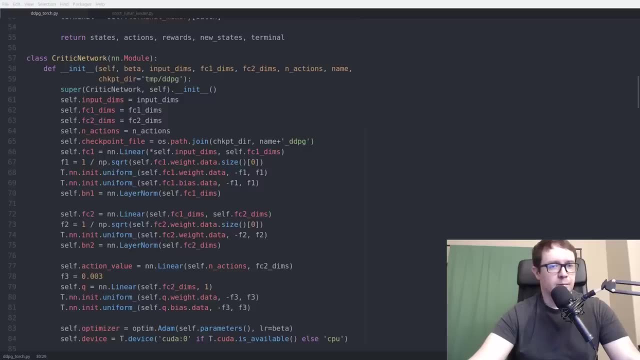 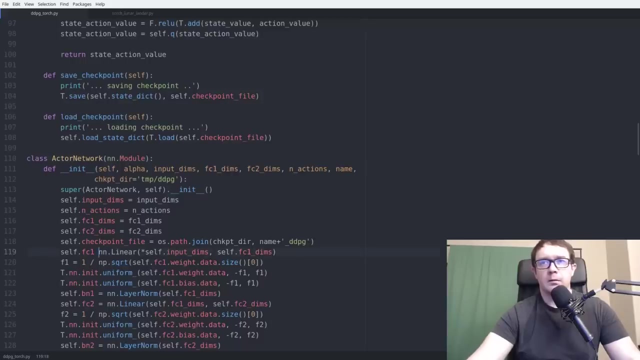 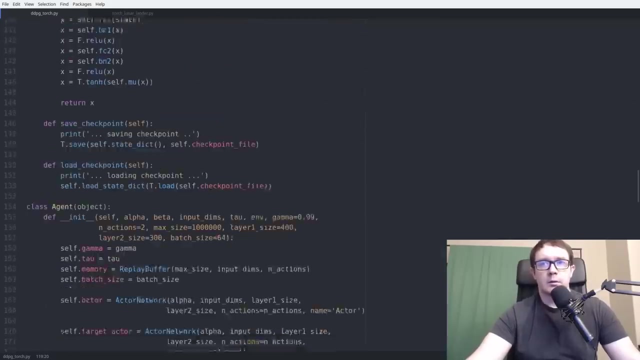 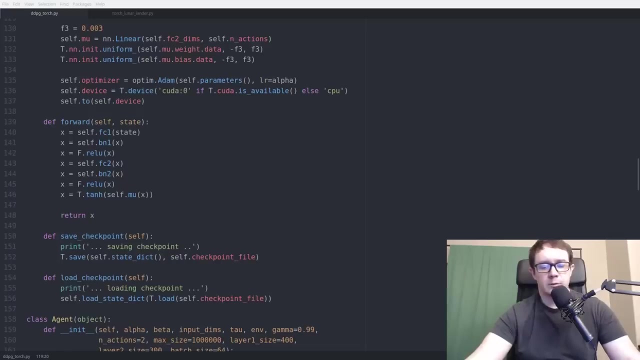 all right, let's try it again. uh, line 119. okay, uh, typical, all right, so 119. uh, right there. so that's in the actor. let's just scroll down. that's the agent class. all think i did it there. all right, i'm going back to the terminal. 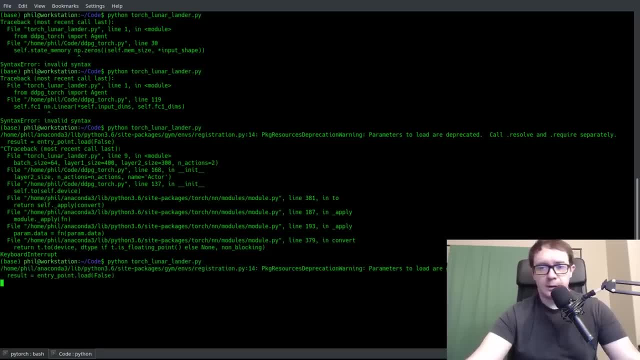 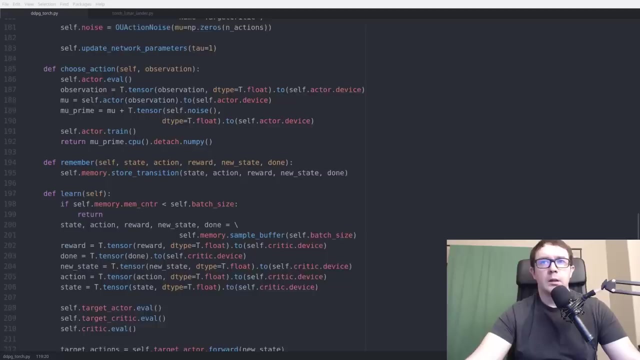 all right. so i started it and it ran. so let's see: built-in function has no function or method has no attribute numpy. all right, that's an interesting bug. let's fix that. so that is on line 192 in our choose action function and mu prime. 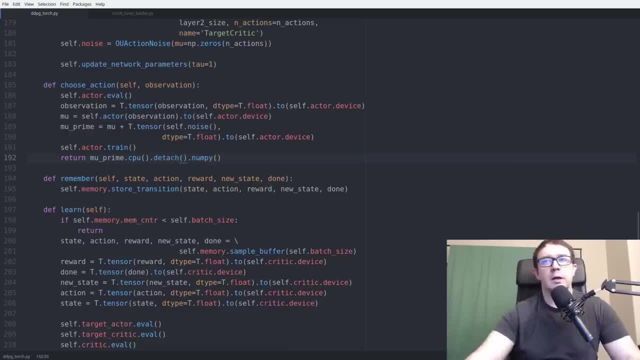 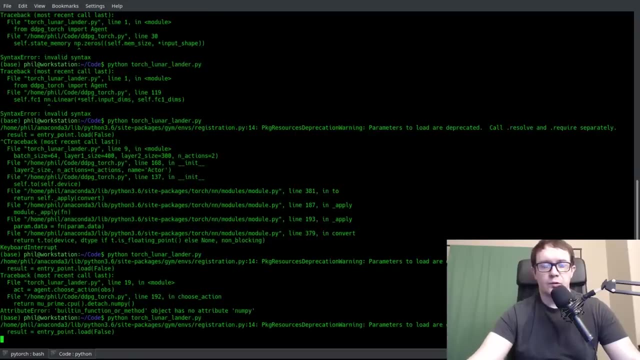 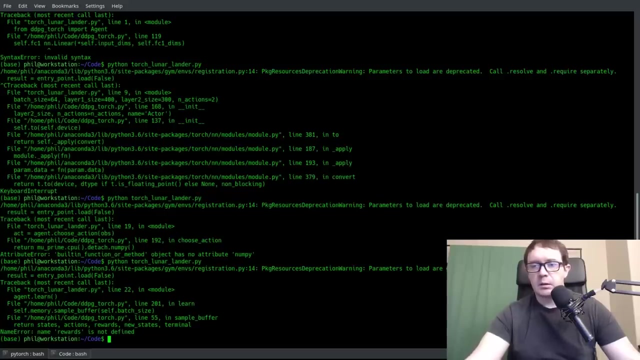 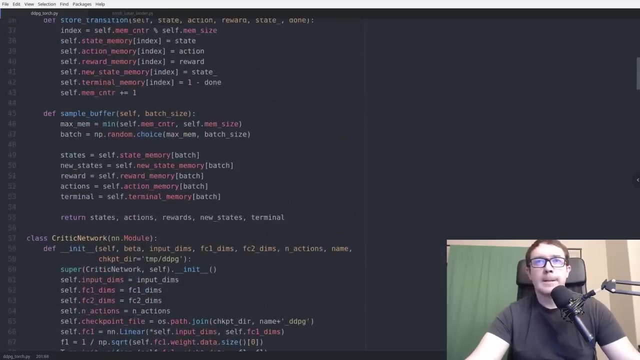 oh, that's why it detaches a function, not an object. that should fix it. let's head back to the terminal. rewards is not defined, so that is in line 55. okay, ah, it's just called reward. there we go, add the s and back to the terminal. 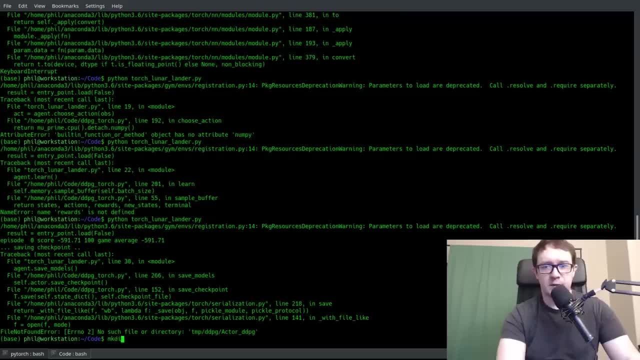 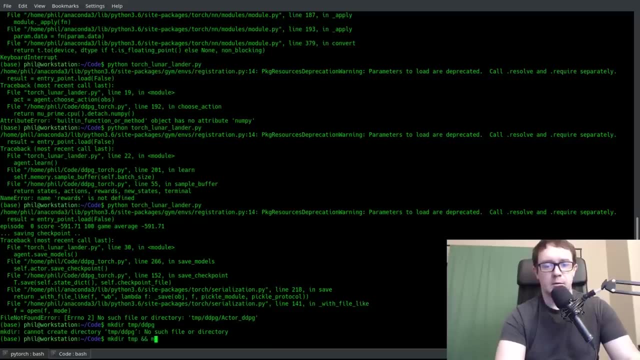 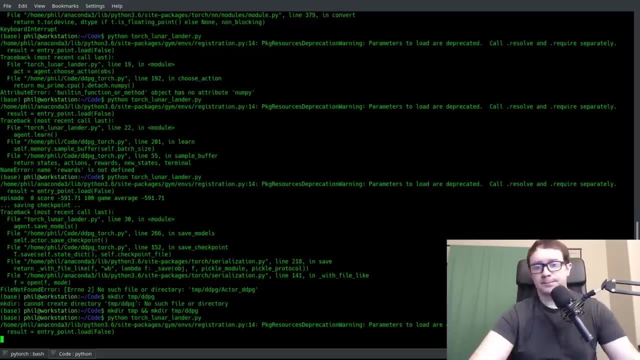 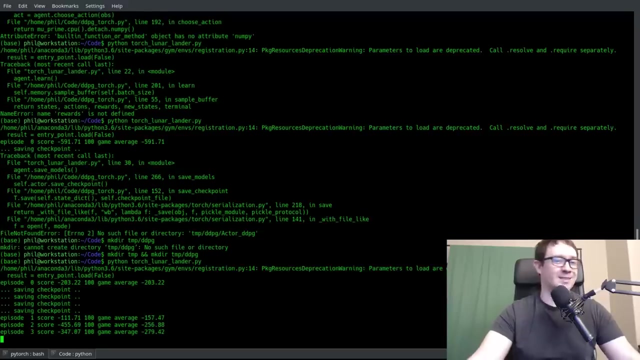 ah, perfect, that's easy to fix. mictor temp slash gdpg. because i didn't make the directory first. that's easy to fix. so i'm not going to let this run all 1000 games because it takes about a couple hours or so. instead, let's take a look here. so i was running this earlier when i was making the. 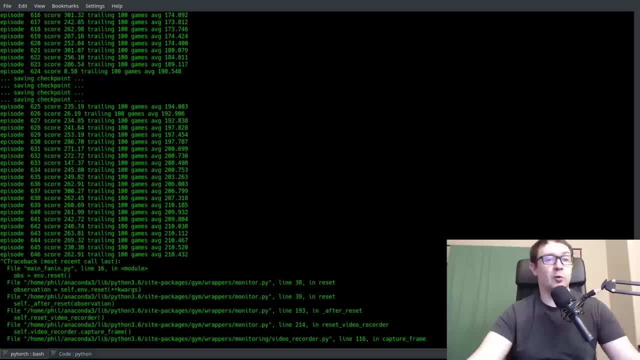 uh videos for the- uh sorry, the recording the agents play while making for this video and you can see that within under 650 games it went ahead and solved it. so when you print out the trailing average for the last hundred games, we get a reward of well over 200.. i'm going to go ahead and do that. 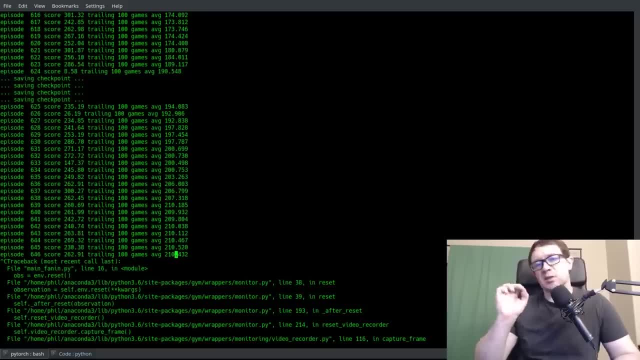 um, now, keep in mind. uh, one interesting thing is that this is still, uh, actually in training mode. it's not, excuse me, it's not in full evaluation mode, because we still have some noise. right, if you wanted to do a pure evaluation of the agent, you would set the noise to zero. 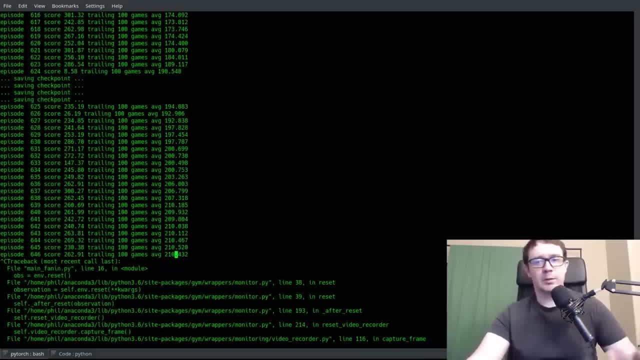 we'll do that in a set of future videos. there's a whole bunch of stuff i can do on this topic, uh, but just keep in mind that this is an agent that is still taking some random actions- the noise is non-zero, and so it is still taking sub-optimal actions and getting a score of 260- and 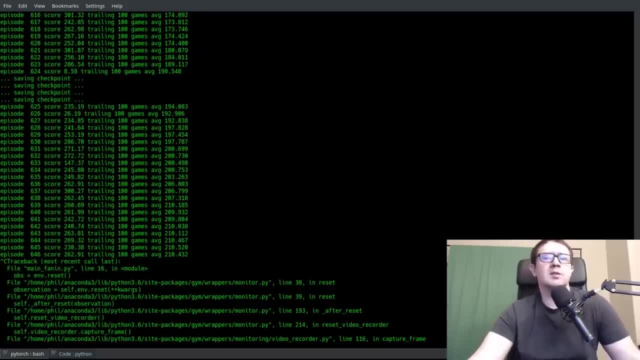 still beating the environment, even though that noise is present, uh, and you can see it in, uh, like episode 626, where it gets a score of 26, so, and then in episode 624, where it does, you know, 8.58 points. so, uh, that is pretty cool stuff. so this is a very powerful algorithm and keep in mind this was 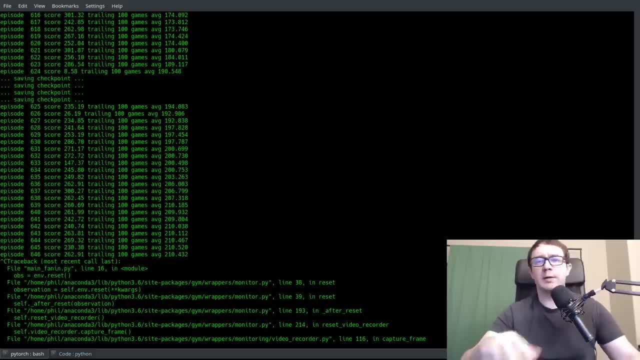 a continuous action space, totally intractable for q learning right. that is simply not possible. uh, it's an infinitude of actions. so you need something like ddpg to handle this, and it handles it quite well. in future videos, i'm going to go ahead and show you how to do that and i'll see you. 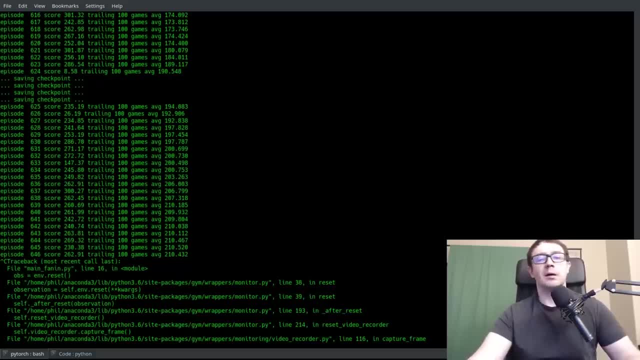 in future videos. we're going to get to the walker, the bipedal walker, we're going to get to the learning from pixels, where we do the continuous racing environment, and we'll probably get into other stuff from the robo school of the open ai gym. so make sure to subscribe so that you can see.